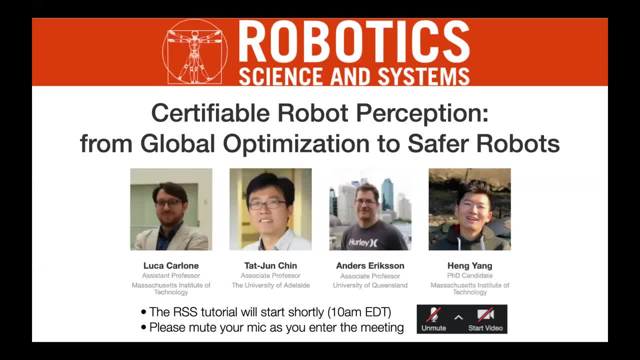 Thank you, All right, I think we can start. Hi everyone, Welcome to the tutorial. RSS tutorial on certifiable robot perception: from global optimization to safer robots. I'm Luca Carlone. I'm assistant professor at MIT and I'm one of the co-organizers of the workshop, together with TJ Chin. 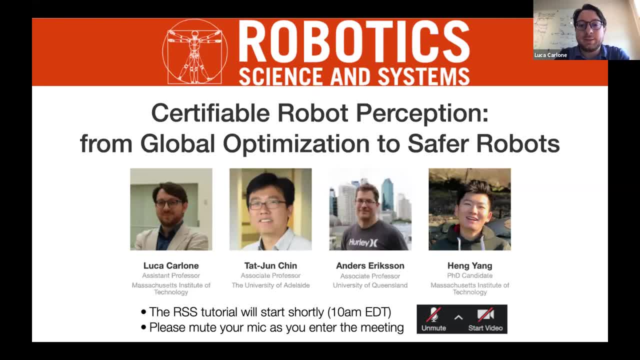 with associate professor at the University of Adelaide, Anders Eriksson, associate professor at the University of Queensland, and Han Yang, who is a PhD candidate at MIT. So, before starting, I want to thank you for tuning in to this workshop. I hope that you. 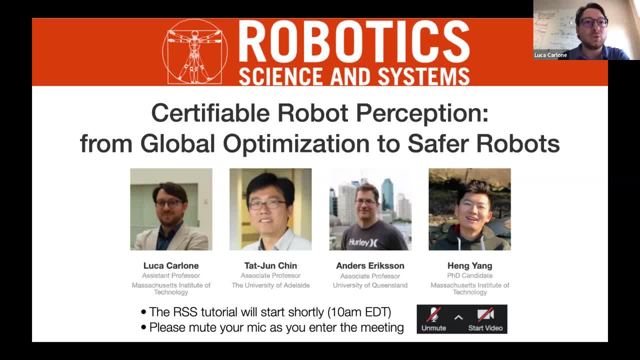 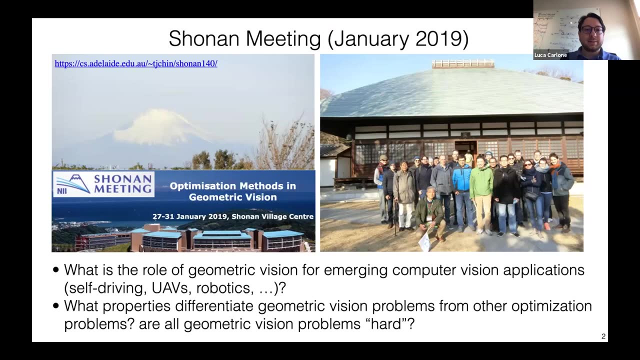 and your loved ones are doing well, And I also wanted to thank two of our co-organizers who are tuning in from Australia and for them it's essentially midnight at this point, So let's get started. So this meeting actually started the idea of organizing this tutorial. 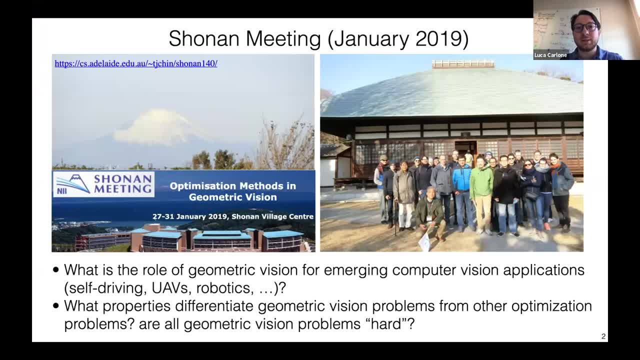 started from another meeting, which was in January 2019.. It's called the Shonan meeting, So the Shonan meeting is a particular format in which essential researchers come together in small groups to have focused and intensive discussions about specific topics. And in this, 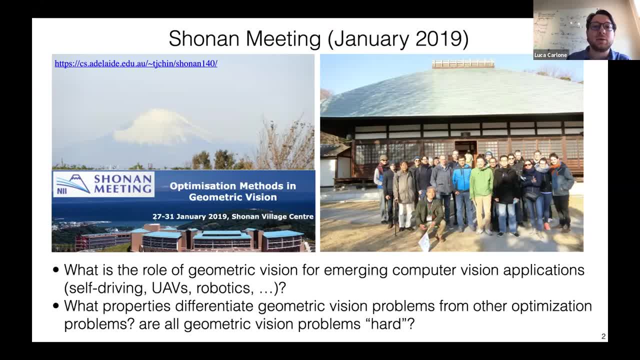 case, TJ in 2019, he was the first to come to the workshop. And he was the first to come to the workshop. And then, TJ in 2019, organized the Shonan meeting on optimization methods in geometric vision, discussing what is the role, for example, questions such as what is the role? 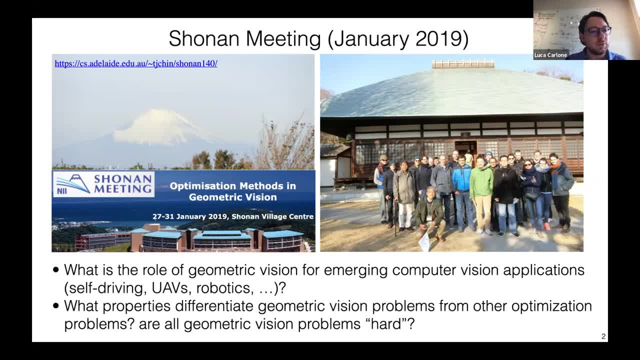 of geometric vision for computer vision applications, including self driving, UFVs, robotics and so on, understanding what properties differentiate geometric vision problems from other optimization problems and understanding how hard it is essentially to solve geometric vision problems. So through this meeting we realize that there is a lot. 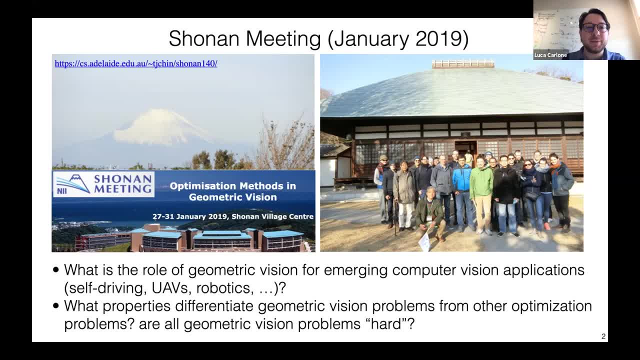 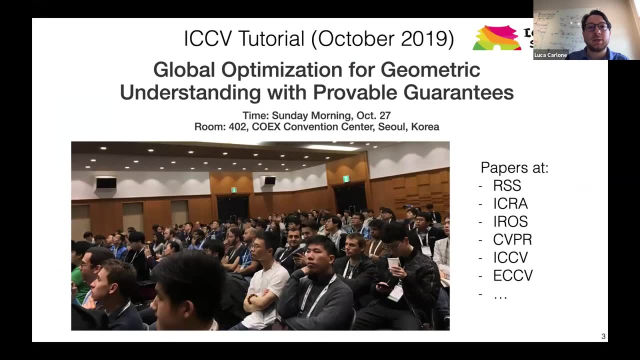 to be done in this area and is really an area which is at the boundary between multiple research fields, including computer vision and robotics. So after this meeting in January 2019, we organized a previous event which is kind of a twin event compared to this RSS tutorial. 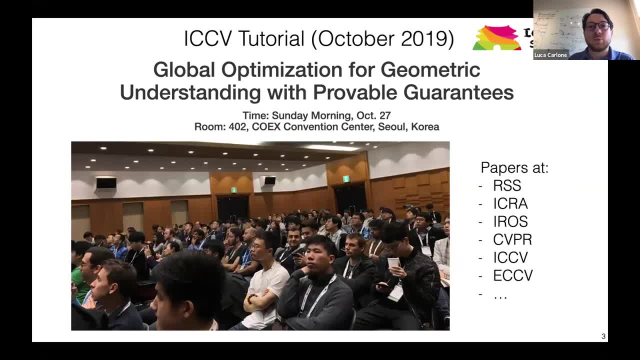 So the previous event was an ICCV tutorial in October 2019, just called Global Optimization for Geometric Understanding with Provable Guarantees. At ICCV in Seoul in Korea, we got around 200 participants. You may remember these nice times. 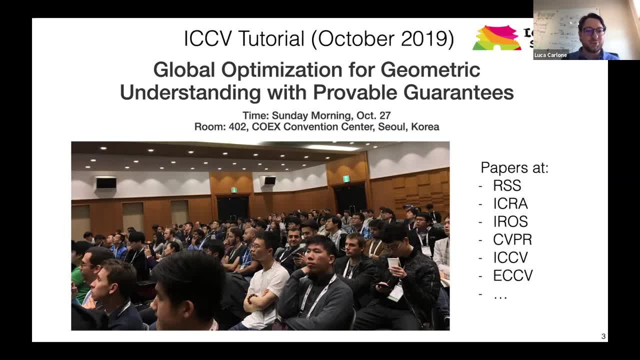 in which conferences were in person and you were going to other places to enjoy the conference with your colleagues. But I guess the message here is that the topic we're going to discuss this morning is of broad interest across multiple research communities, And indeed you'll find papers dealing 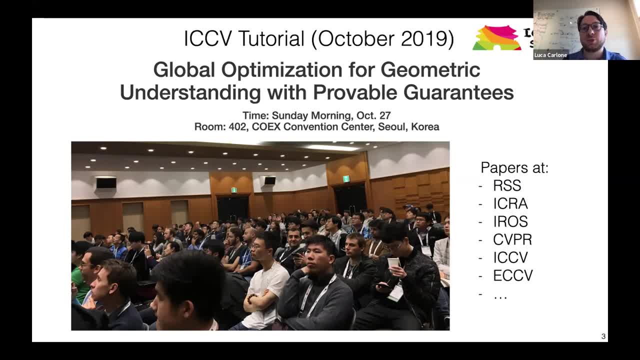 with the global optimization, certifiable perception, perception with global guarantees in many venues across robotics, computer vision. I'm listing here RSS, ICRA, IRIS, CVPR, On the computer vision side, CVPR, ICCV, ECCV. 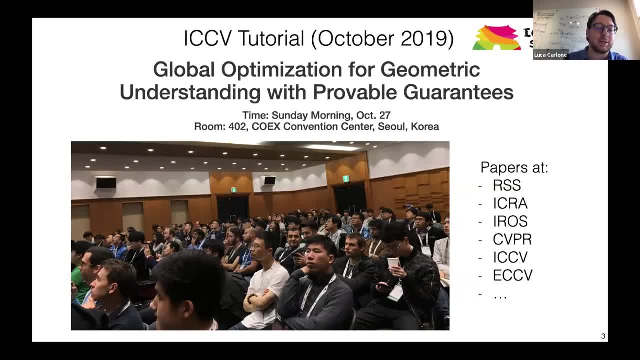 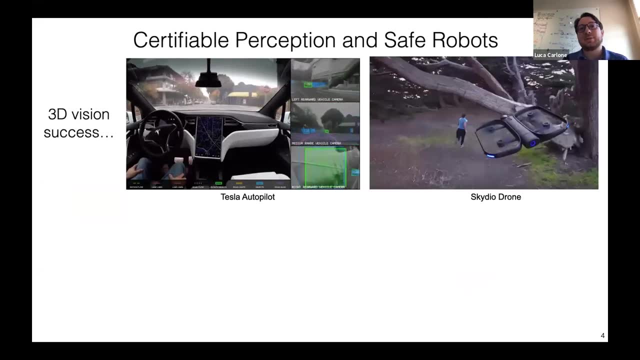 And not only. You will find papers along these research lines also in applied math venues and across multiple communities. So what is the topic of today's tutorial? Today, we want to talk about certifying, about certifiable perception, And we want to stress the importance 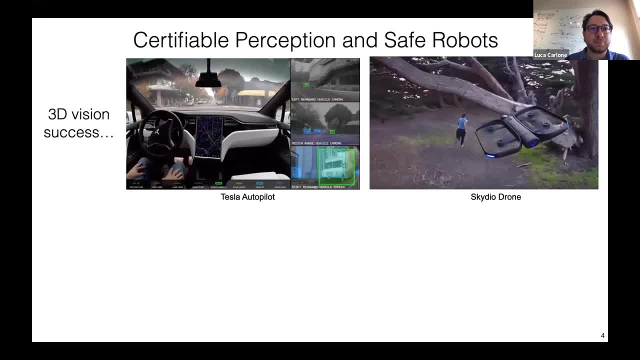 of certifiable perception for safe robots. So why do we care about perception? Well, it turns out that you should not be surprised that perception right now is a great moment for robotics in general, but also perception technologies are essentially playing a huge role in many robotics applications. 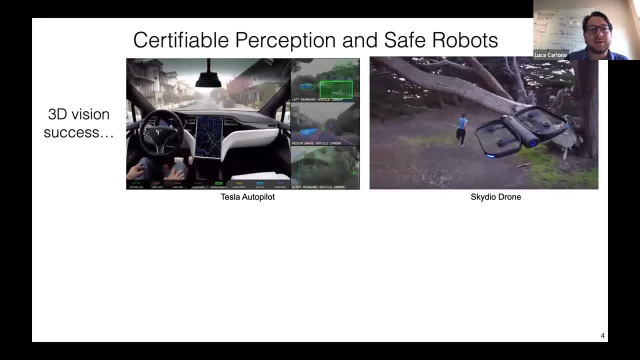 Here I'm showing a couple of very, very good examples. Here I'm showing a couple of very, very good examples. Here I'm showing a couple of very, very good examples. On the left, you see the self-driving car, the Tesla. 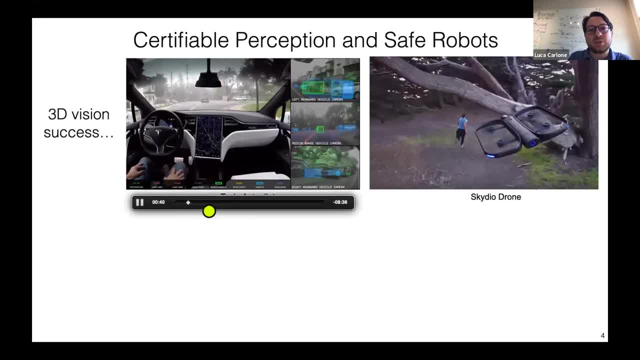 autopilot, And you can see that there is. in this demo, which at this point is a few years old, you can see that there is a lot of computer vision and perception going on. You can kind of understand that there is some object detection. 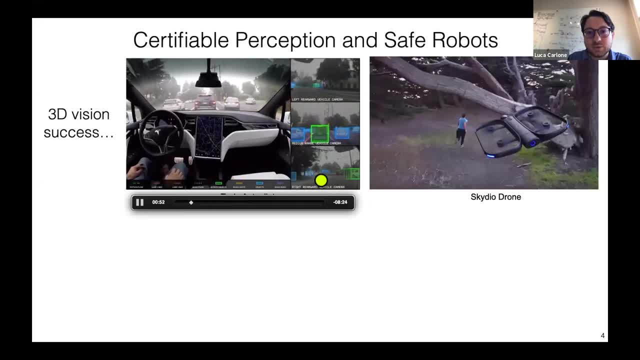 There is some lane detection, road detection And also, I think in some of the images there were some features that were tracked In the scene. you can look at some of the images. You can look at other applications, like drones, for example. 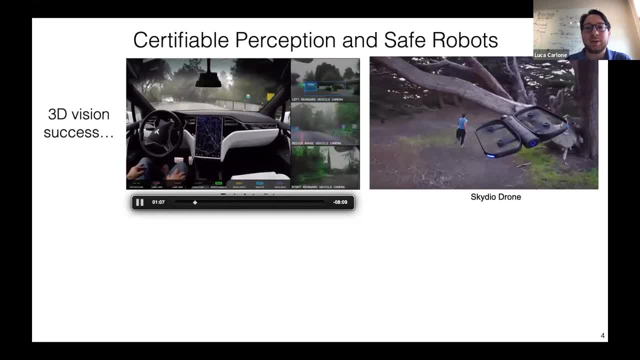 And perception is playing an important role for drone in enabling obstacle avoidance and navigation in unknown environments. While perception is positioned to be a very important technology for the future of robots, the broad adoption of this technology is also showcasing fundamental limits of the algorithms that you are working on right now. 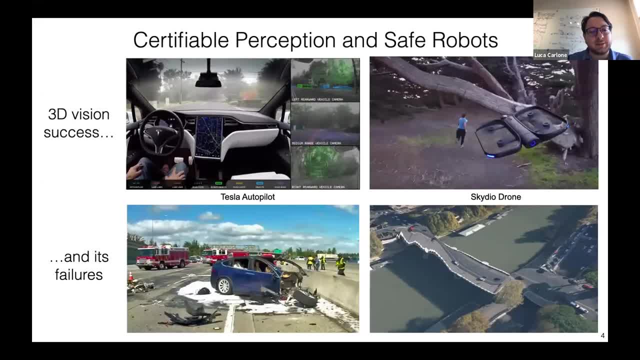 And, in particular, the message that I want to give here is that perception algorithms are increasingly used for safety-critical applications, such as self-driving cars. In these applications, failures of the algorithm can have catastrophic consequences. So here is an accident from a Tesla from a couple of years. 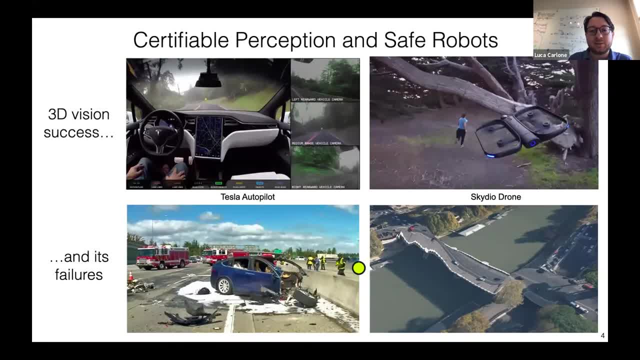 ago, in which the vision system misdetected this concrete obstacle on the left of the car and decided to turn into it, killing the passenger. And these are other examples of failure of well-engineered, well-engineered systems such as Google Earth. 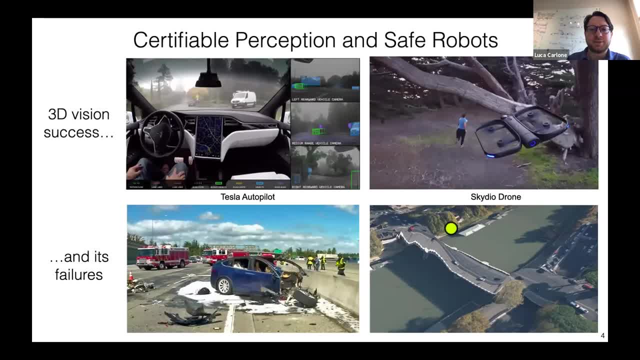 in which you can see that even like an engineer, system will have failure modes in which the reconstruction of a bridge in this case- is completely off. So message so far is that certifiable perception in general is important And doing it right is even more important. 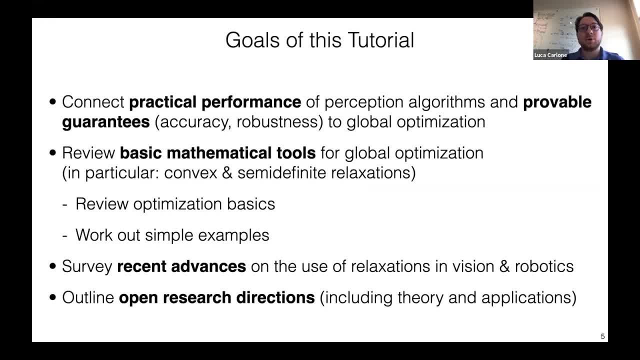 for safety-critical application, And this brings me to the goal of this tutorial. So the goals we have are these four that I'm listing here. We want to connect practical performance of perception algorithm and provable guarantees of these algorithms, including accuracy and robustness. 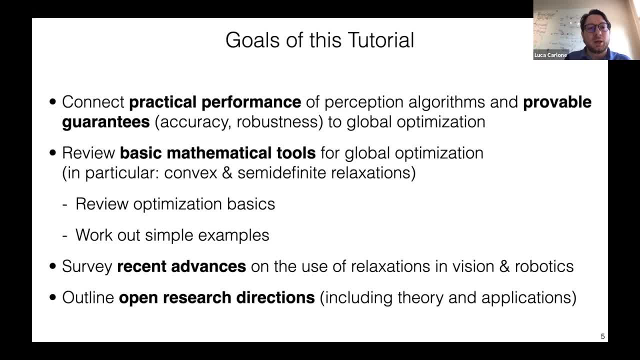 two ideas that go back to global optimization. We want to review basic mathematical tools. This is supposed to be a tutorial. We want to review basic mathematical tools for global optimization and, in particular, convex and semi-definite relaxations. So we are going to start with a review of basics. 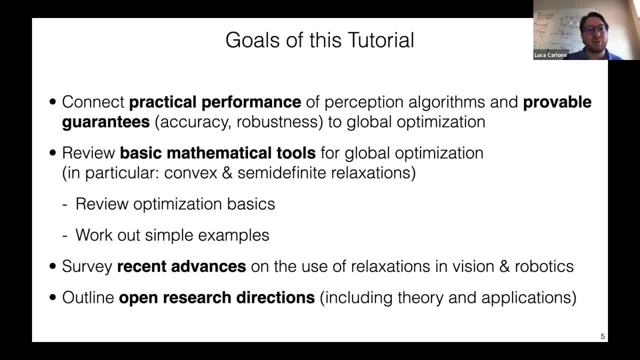 of optimization and we're going to work out a simple example. I'm saying simple but actually a pretty advanced robotics example. We want to offer you a survey of recent advances on the use of relaxation in vision and robotics and we want to outline open research direction. 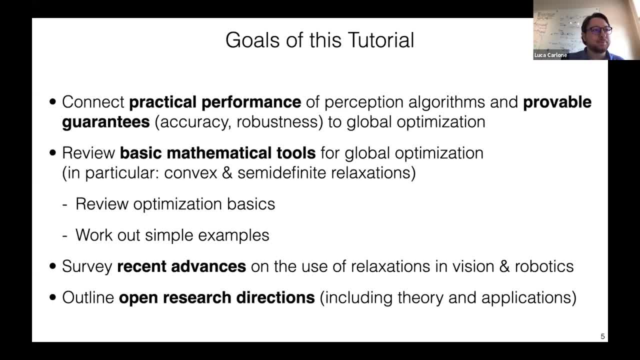 All the research that we're going to discuss has been booming in the last few years. There is plenty of work to do and we want to make sure that, as you walk out from this tutorial, you have some good idea about the open research. 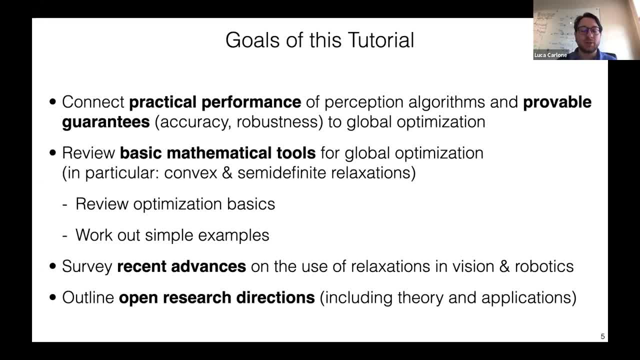 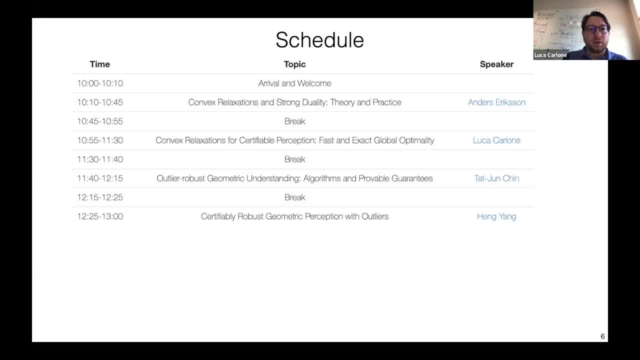 So we want to be able to provide you with some of the information that you need to go to the next step, which is to bring you to the next step of the research that you need to go to. So we want to talk about the. The plan for this morning is as follows. 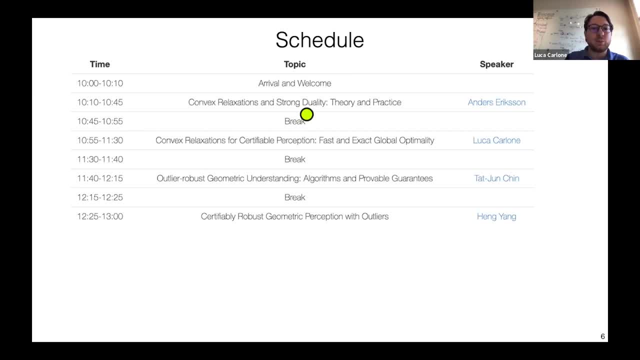 We are right now in the middle of the introduction here and we're going to have four presentations. The presentation is around 35 minutes and there is a little bit of a break of 10 minutes after each presentation. We are going to be flexible. so if you guys have lots of time, see you next time. bye, bye. 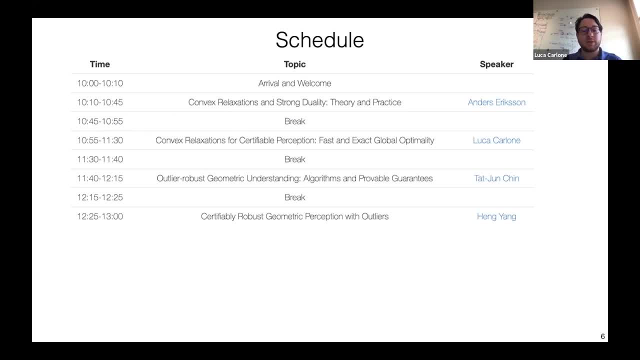 lot of questions- you can take a little bit of the break time to answer more questions- And the four presentations are essentially trying to cover, to sample this space which is, like you know, this idea of certifiable algorithms, and it's going to sample this. 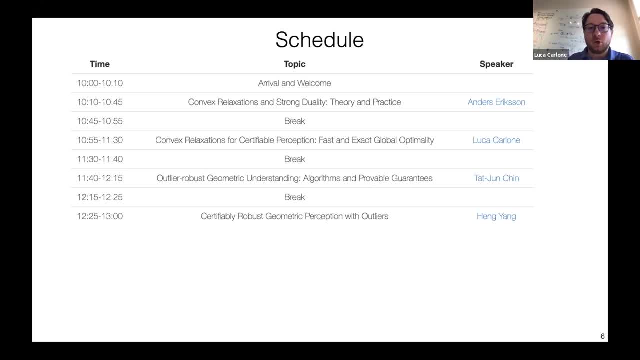 space to give you an overview of different aspects of interest. Anders is going to start with the first presentation. he's going to talk a little bit about history, but mostly he's going to cover, like you know, the notion of optimality and how that. 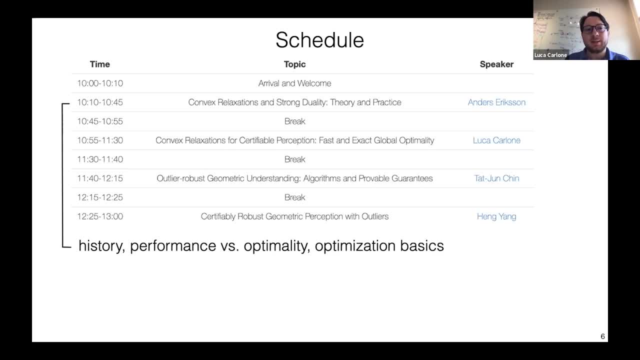 impacts, performance in robotics and vision application, and the key role of the first presentation is just to give you the basic concepts about optimization, which we're going to mention again and again in the other talks. I'm going to give the second presentation and the second presentation we're going to 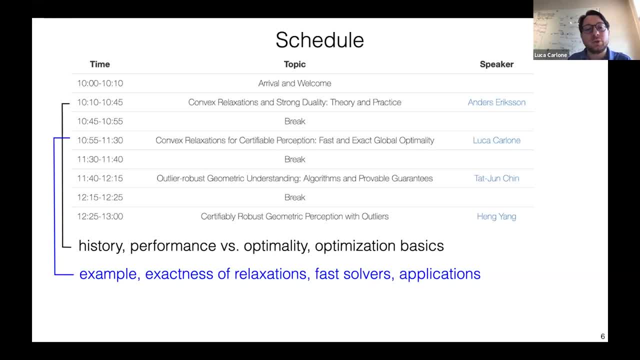 jump on the use of focus, on the use of convex relaxation, And I'm going to work out an example which is related to simultaneous localization and mapping in robotics. I'm going to show you that, despite the name, relaxations can be often exact, you know. 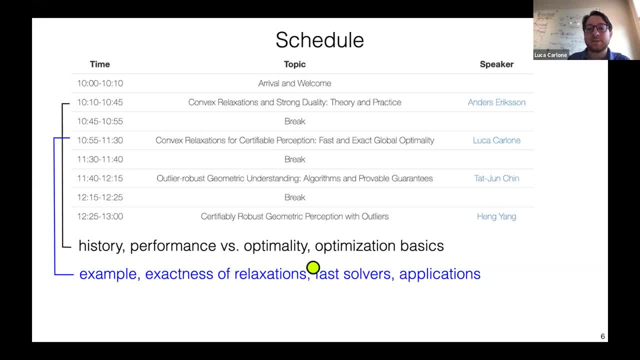 can not entail any approximation. We can develop fast solvers and I will review a bunch of cases in which our groups and other researchers in the community were able to develop successful relaxations in geometric perception. TJ is going to talk about another important aspect in real-world application, which is 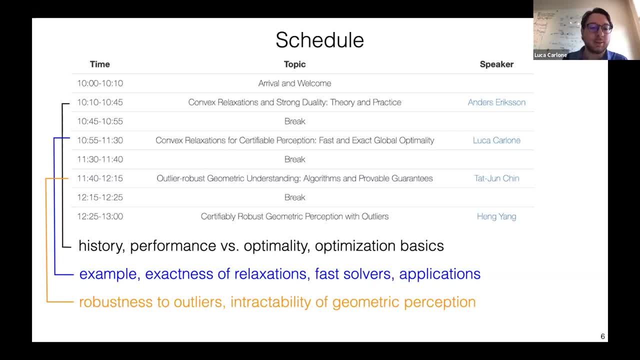 robustness of outliers. Outliers will always be present in robotics and computer vision and he's going to stress very fundamental results about intractability of geometric perception without outliers, And Hank is going to close the tutorial with some very decent idea about how to use convex. 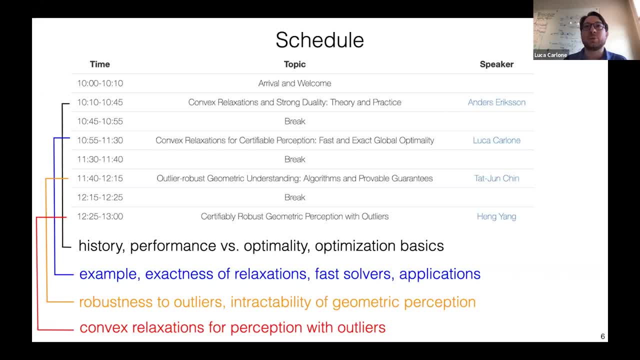 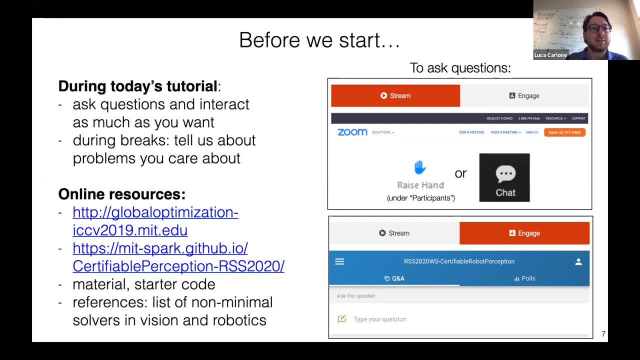 successfully use convex relaxation for perception without outliers. Thank you. So before we start, I have one final slide here, which is giving you a little bit of the rules of engagement for this morning. First of all, we want you to ask as many questions and interact as much as you want. 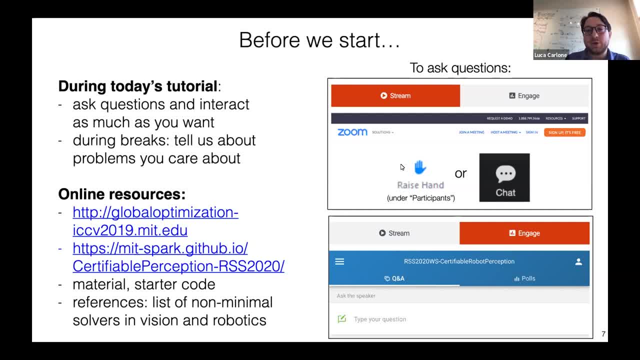 There are two main ways to do that. At this point, you're most likely connecting from the RSS portal, so you should see in front of you an interface like this, But if you don't, you're not going to be able to interact. 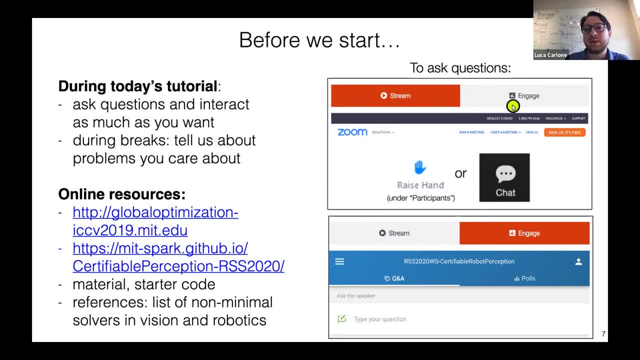 You will see two buttons: One is stream and the other one is engage. Right now you're looking at me, so most likely you're on the stream tab, And inside the stream tab you should see an interface which is essentially Zoom. 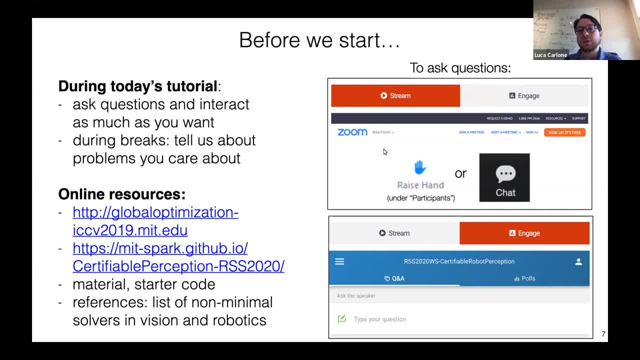 And within Zoom. there are two ways that we suggest using to ask questions. The first one is just use the chat. You can write your question in the chat and we are going to monitor that. The other one is that if you click under participants, there should be a function which is called 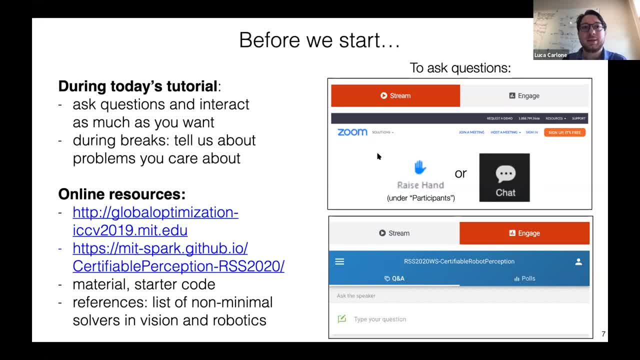 raise hand And we're going to monitor that as well. If you raise your hand, we're going to call on you for asking the question directly, The other approach. so these are the two approaches that you can use. There is another approach, which is clicking on the engage tab on the RSS portal. 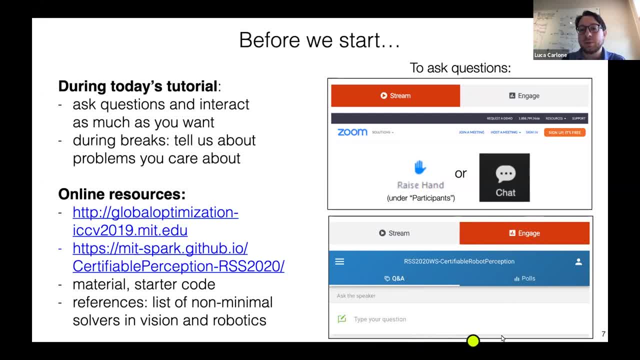 If you click on the engage tab, you're going to see Slido, which is just this interface in which you have a tab, essentially, in which you can type any questions you want, And then you can click on the engage tab. And then you can click on the engage tab. 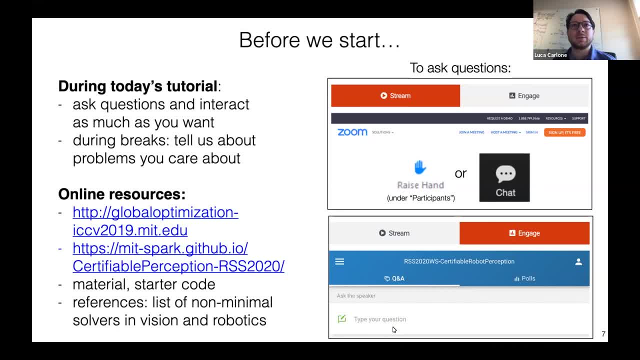 And then you can click on the engage tab, And then you click on the engage tab. You can also use the question you have, And you can also decide whether the question is anonymous or whether you want to put your name next to the question. 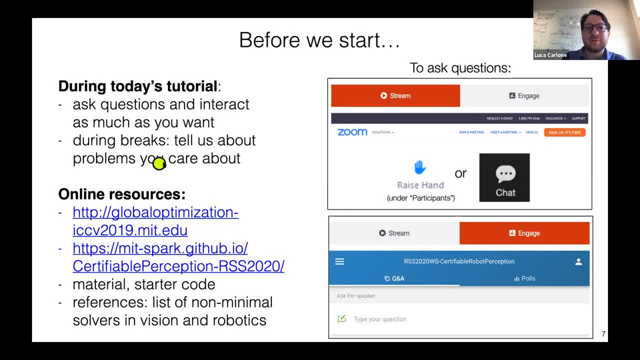 The breaks. as I mentioned, we're mostly going to stay online for the breaks. Feel free to stay online as well. Feel free to ask questions and to tell us about the problems that you care about. As we go, we're going to release more and more online resources. 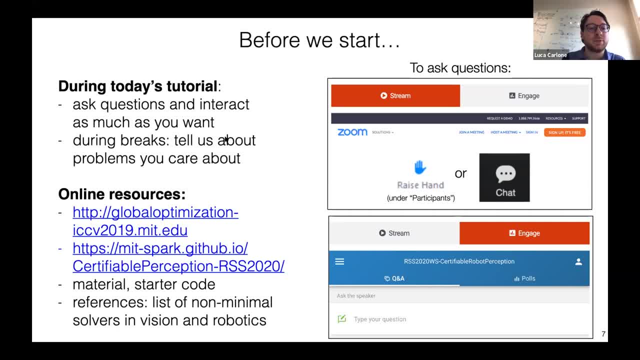 Right now you're going to find already plenty of online resources at the SCCV tutorial from last year, as well as on the website of this RSS tutorial, and these resources include some material. we're going to release slides. we're going to release a little bit of code references. 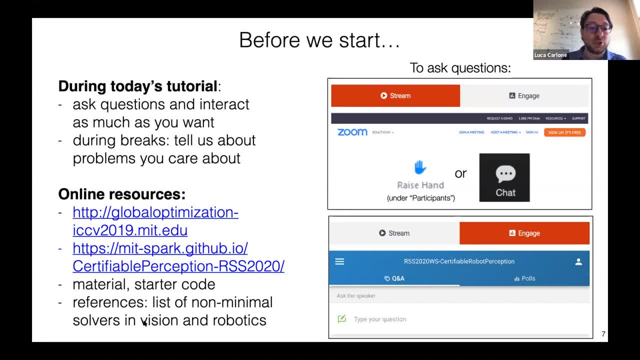 listing pretty much all the approaches that we're going to cover in this, this tutorial proposed in both vision and robotics, and not only i would say so. with this, i would say that we can get started, and i just wanted to see if there are any more comments from from the other organizers. 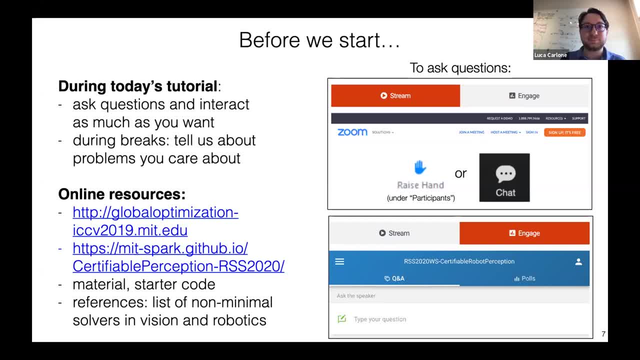 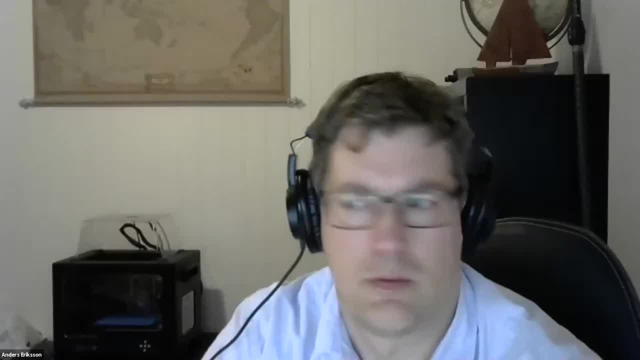 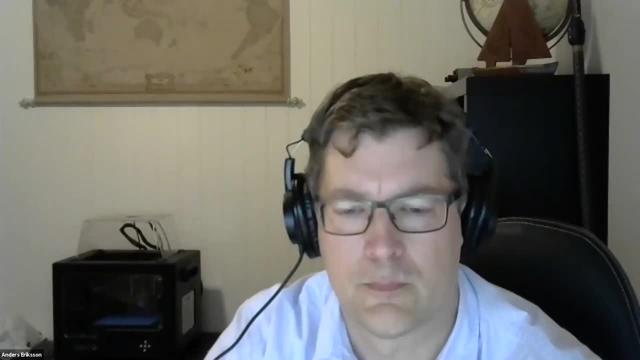 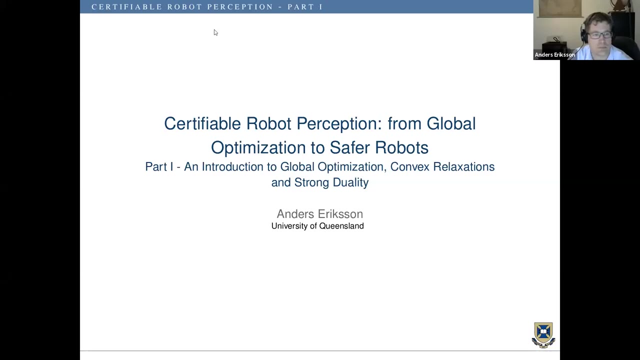 otherwise we'll get started with Anders. yeah, i'm ready, see you, can you can see that, okay, i hope me too. um, okay, well, first of all, good morning everyone. well, not really, it's, it's just past midnight down here in australia, so, um, me and tj might be struggling a little bit, not yawning. 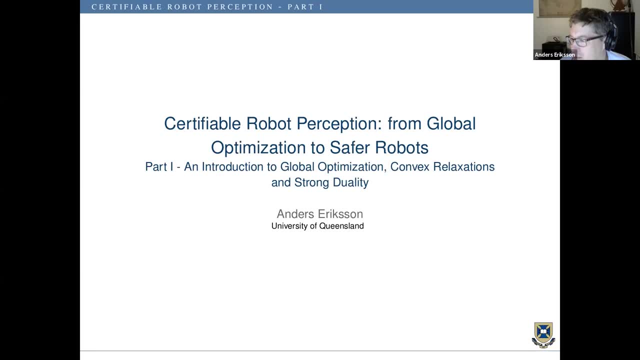 um, anyway. so, um, yes, my name is Anders Eriksson. i'm an associate professor at the university of queensland here in brisbane. um, and my talk is going to be. well, the aim of it is to try and give a, i guess, a gentle introduction to global optimization, but the topics that i'm 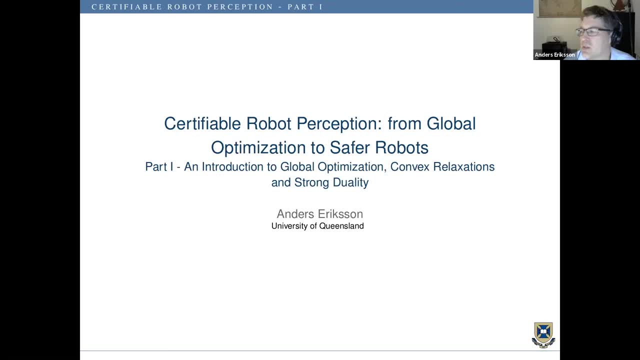 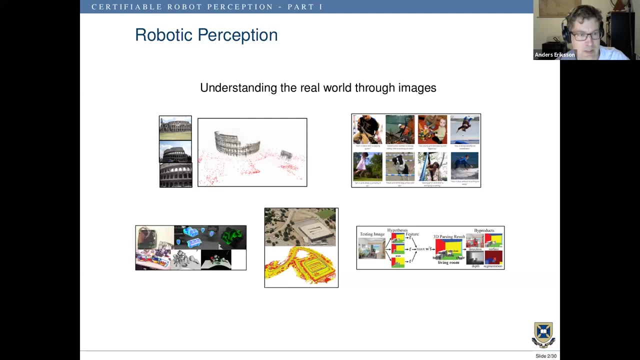 going to be touching on specifically are the ones relating to convex relaxation and a concept known as duality or strong duality. so the motivation behind this, behind this talk, and i guess i guess this whole entire line of research, relates to the fact that robotic perception or robotic vision, or computer vision or whatever you're going to call. 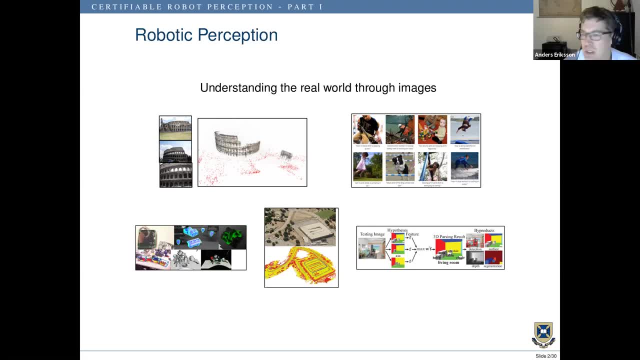 it. it's something that concerns itself with the, with understanding the world through images with a wide range of different applications. so here, for instance, you can see, we have the problem of 3d reconstruction. we have something like image processing understanding. on the bottom left we look. 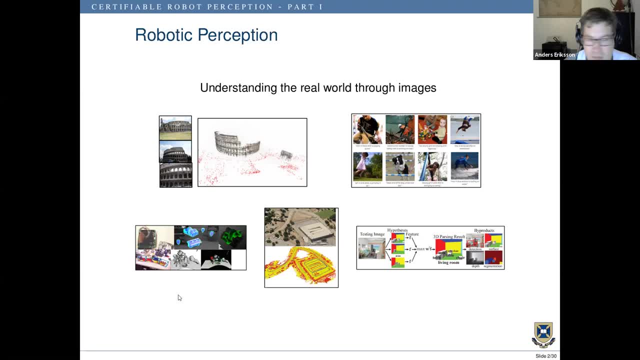 we have an example of of six degree of freedom: pose estimation, perhaps in the middle there, robotic localization and mapping and slam and perhaps something like image segmentation or semantic segmentation. but what is common, uh, is that these problems typically leads to some form of an optimization problem. in the first one, there we 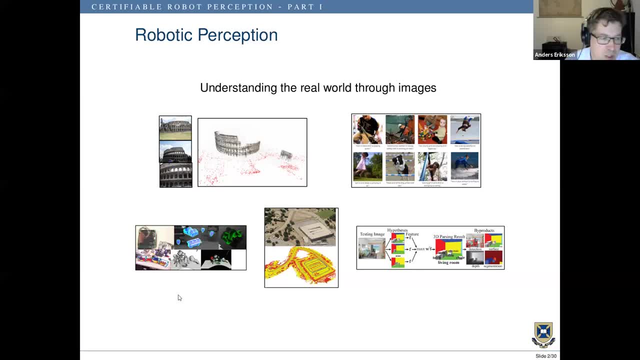 have 3d reconstruction. you look at minimizing some form of reprojection error in the image understanding task. you look at perhaps learning through minimizing some related loss function in training. the pose estimation problem might be formulated as minimizing some form of model fitting error, geometric errors in the slam example for instance, and so on. 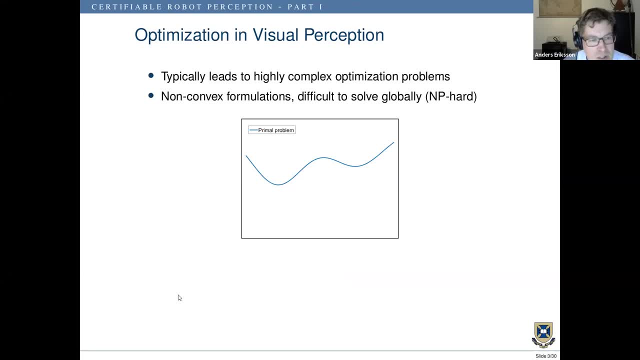 and what is also common is that, in the majority of these applications, the the resulting, this resulting optimization problem is highly complex: um, the non-convex formulas, formulations typically that are very difficult to solve globally. um, so, typically, what you do in this, in these settings, is that you, you pick some. 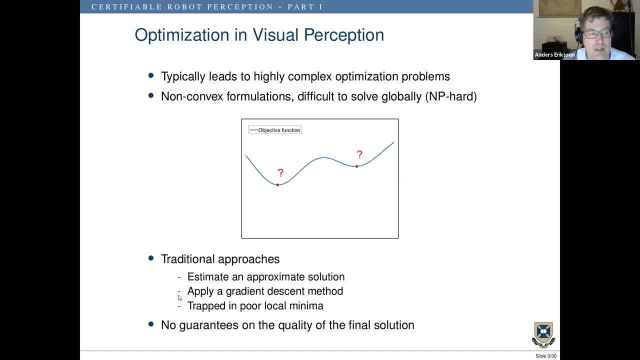 starting point and you start moving downhill until you can't any longer. and that is the solution to your problem, or at least you hope so. um. the issue with this approach, uh of this um steepest descent, uh minimization type approaches, is that you can really be certain of the quality of the resulting solution. 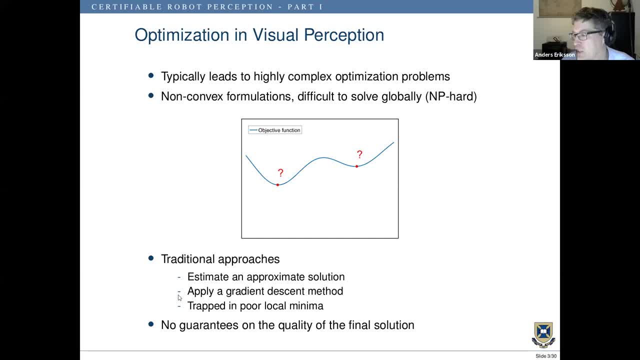 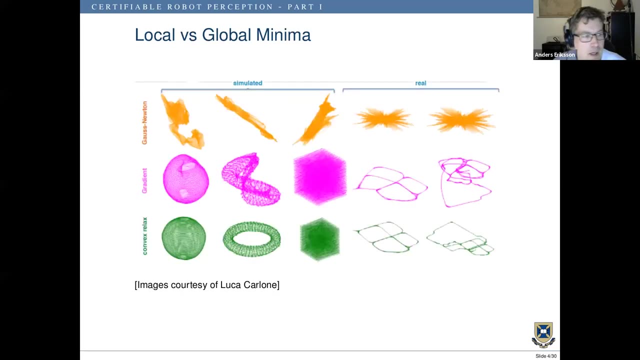 so in this image here, if you have that approach, you don't really know which which of these two local minimas, uh, you ended up in. or one is the global one that you want and one is a local one that is not desirable, um and um. here you can see some examples of the 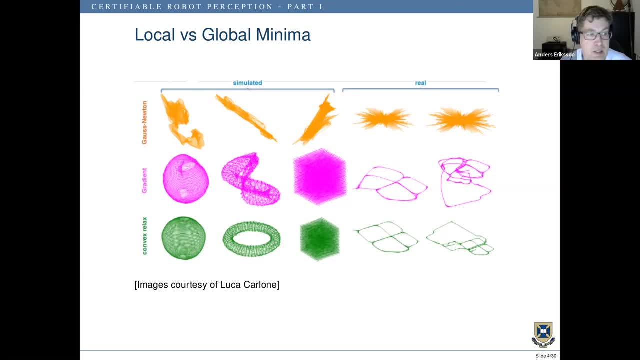 difference between local and global solutions might look like. this is the task of postgraph based slam in 3d, and each column here denotes different local optima for and each- sorry, each row- different local optima. each column here is a different problem. the first three columns are simulated. 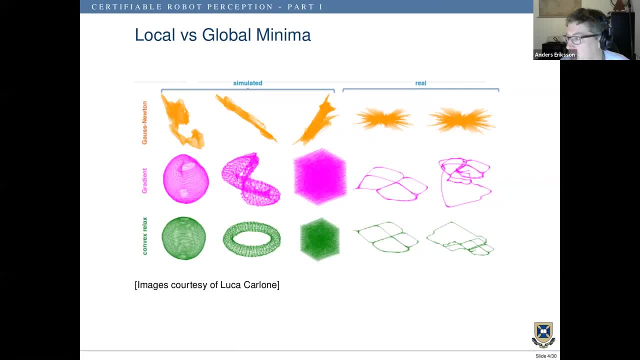 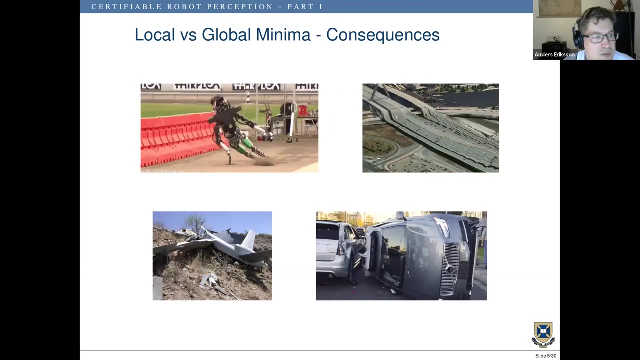 settings, and the two rows are simulated and the right, most ones are from real, real applications and the true one is one at the bottom. so, as you can see, they differ quite, quite drastically and, as luca mentioned, the consequences of failing to distinguish between a local minima and a global minima. 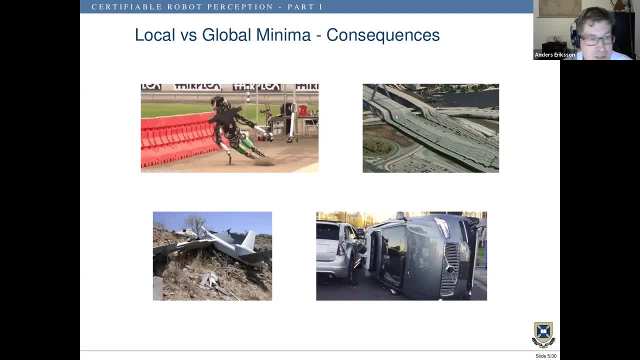 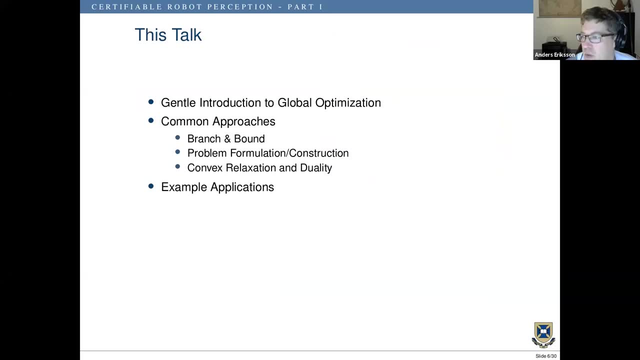 can be quite significant, from from comical to very serious and potentially lethal outcomes. so in this talk then, um, my aim here is to, like i said to, to give, to give a bit of a introduction to global optimization, hopefully a gentle one. i'm going to talk about a couple of a. 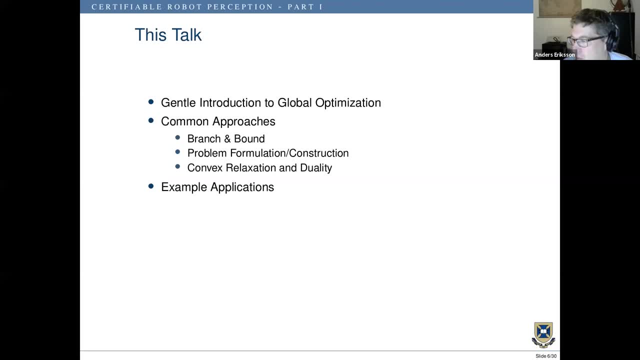 couple common approaches to solving these problems. uh, the three ones i'm going to discuss is a method called branch and bound. i'm going to discuss a little bit about an approach um called, i suppose called problem formulation or construction, and then i'm going to spend perhaps the majority of the time. 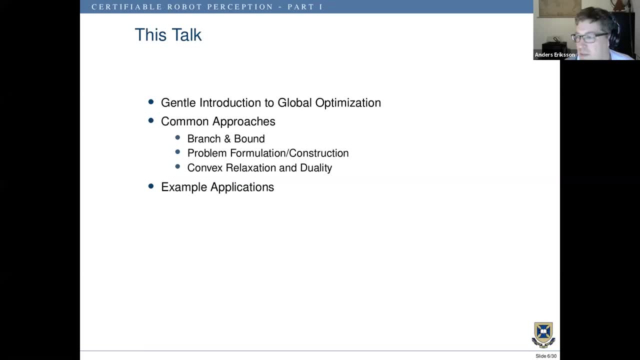 talking about relaxation, convex relaxation and duality, and then end up with just showing a couple of example applications. um, but before we get going, i thought i'd start a bit easy by quickly going through the necessary basics. uh, just to sort of: so we're on the same page, instead of you guys perhaps, and it's late for me. 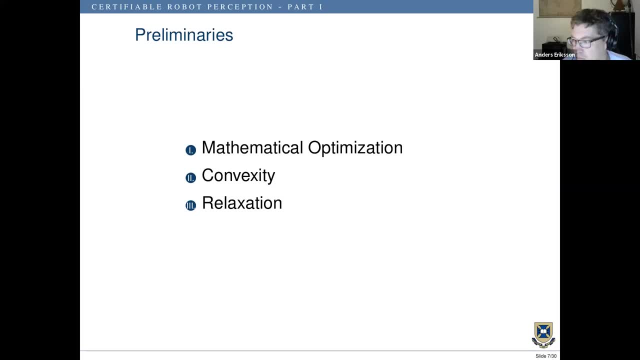 um, so i'm just quickly going to go over these three. um, just mathematical optimization: how, what is it? how do we define it? um, then talk a little bit about convexity. it's a very, very important concept in optimization. and lastly, uh, i'm gonna introduce the concept of relaxation. 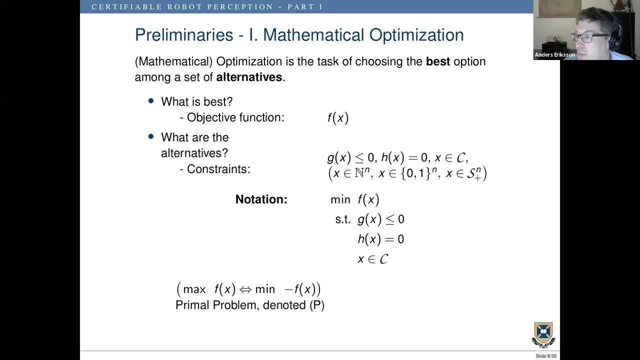 um, so the first one, uh, mathematical optimization, or optimization. um, what do we? what do we mean when we say that? well, one way of defining is it is to say that it's a task of choosing the best option among a set of alternatives. so what do we mean by best? well, that's. 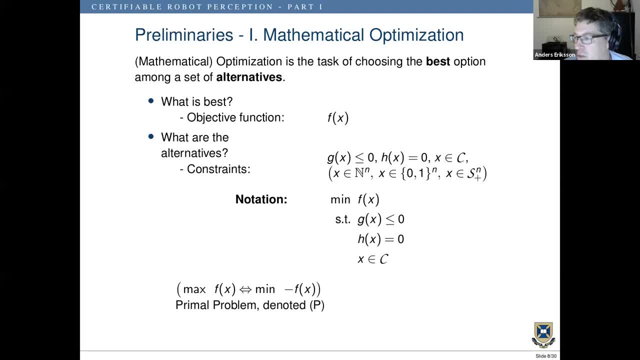 typically measured by some form of objective function. this might be some, some error that we want to minimize, with some loss function that we're going to minimize um, but it's the, the, the um. this is described by the objective function. uh, then the alternatives, um, are described by constraints. this is limits. this is what limits your choice. 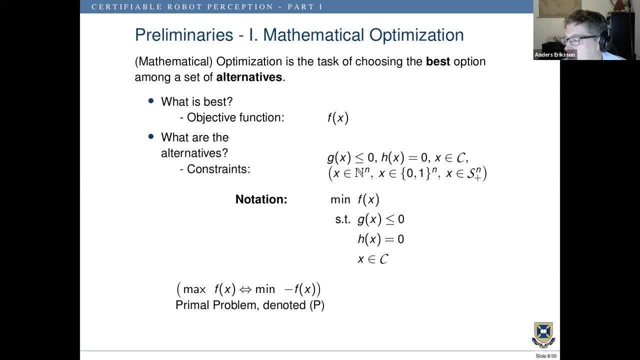 and how you can choose. these are typically given in a number of different ways you can be given, you can have them as inequality constraints. equality constraints- uh, perhaps some kind of set notation. um, it's a depends a little bit on on the problem and the author of that uh paper. 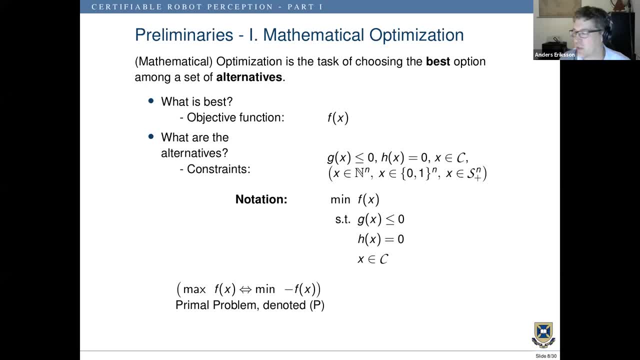 it's not entirely um consistent annotation here, but normally when you, when you, when you um, define an optimization problem, you, you, you write it like this: so you minimize your objective function: uh, st, or such that these list your constraints and again these can be given as as inequality constraints, equality constraints or with some form of. 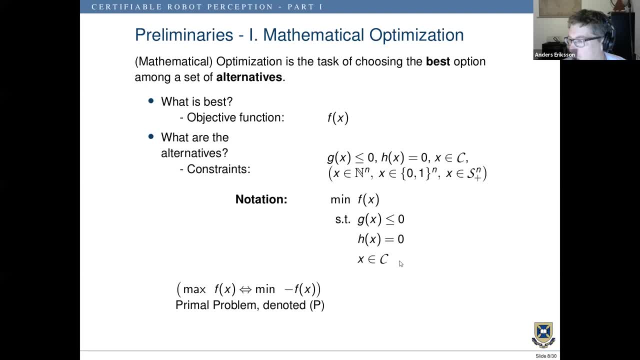 set notation. you often talk about, uh, optimization, as always, minimizing things. this is not always consistent, again, but, um, sometimes it might be more intuitive to say that you want to maximize something, you want to maximize some kind, you perhaps maximize some energy or maximize some form of, some measure of similarity. 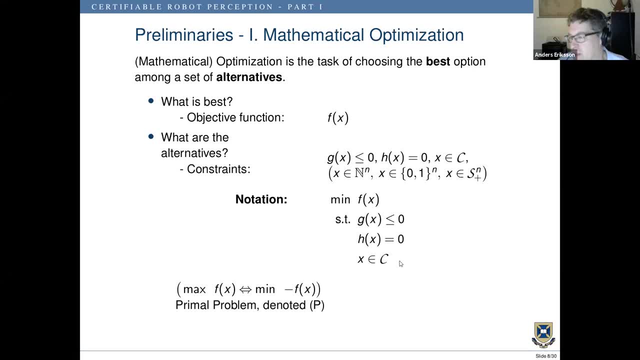 we can always rewrite the maximization problem as a minimization problem. they're equivalent in this sense that maximizing f of x is equivalent to minimizing minus f of x. uh, lastly, uh, this problem here, the problem that we want to solve, is sometimes, uh, sometimes, called the primal problem. 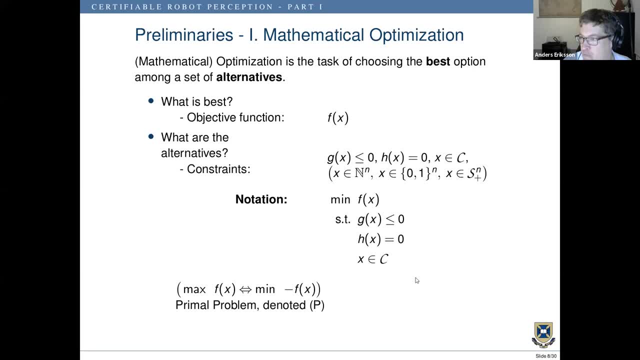 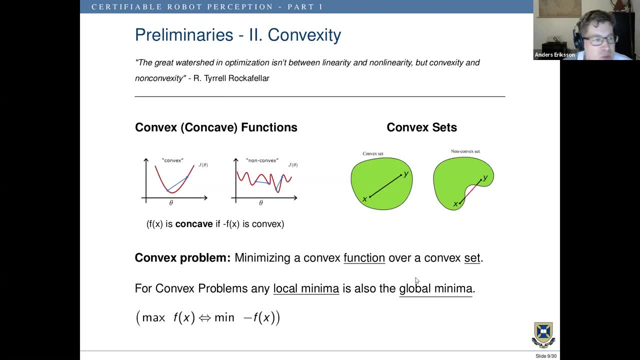 also denoted by capital p um. next, we have convexity um, and this is perhaps one of the most important concepts in optimization, much more so than, say, linear versus non-linear. this is really famous quote by a mathematician called terry rockefeller saying something like that: the great watershed in optimization is in between. 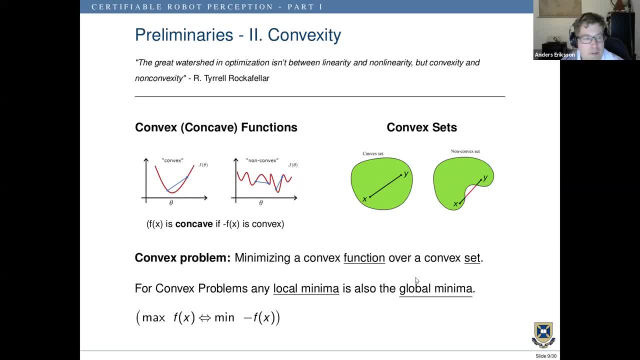 linearity and non-linearity, but convexity and non-convexity. so when you talk about convexity you can sort of talk about convexity in two different ways, with two different, two different meanings. perhaps the first one is you talk about convex functions. a convex function is a function that is. 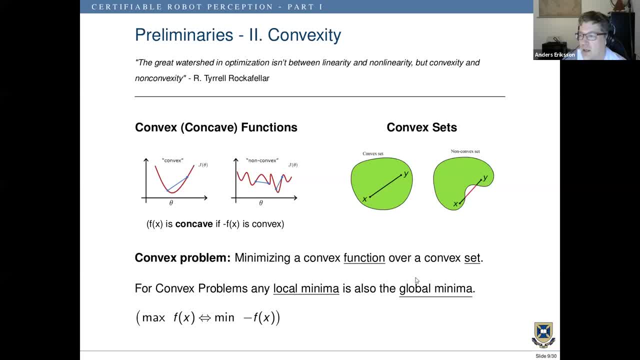 well behaved doesn't have any any. uh, only has one single minima and that's the global minima. like you see on the left here, a non-convex function is a little bit more messy. uh, the um formal definition of a convex function is that if you pick two points on the curve of the function, the line, 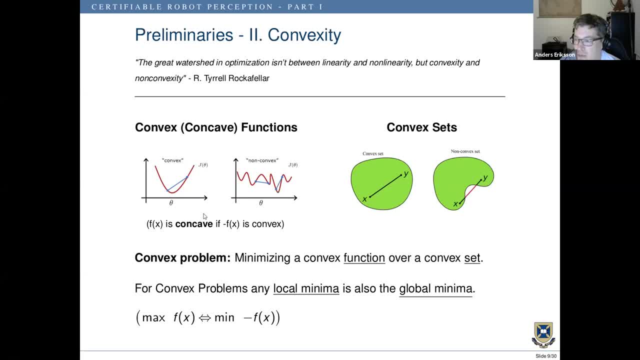 segment that you draw between those two points will always be above or on on the function itself. so this is true for for here on the convex function on the left, but it's not necessarily true for the non-convex function. you also sometimes talk about con cave functions. um, the definition of that is. 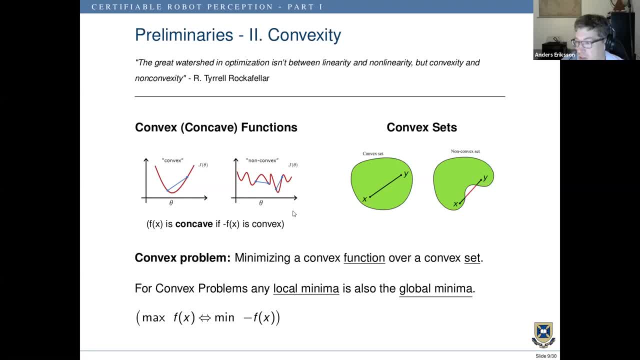 basically f of x is concave if minus f of x is convex. so sometimes you use these two terms a little bit, um inconsistently perhaps, but sometimes you talk about minimizing a convex function and sometimes you talk about maximizing call like concave functions, but they're sort of the same property because you can turn. 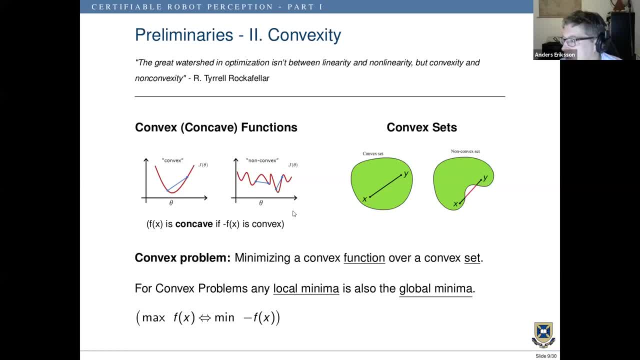 turn one into the other. the second concept in convexity is that of convex sets as a similar definition. so you can hear certain convex sets. the convex set is the one on the left and the non-convex one. this is set on, this is set on the right and the 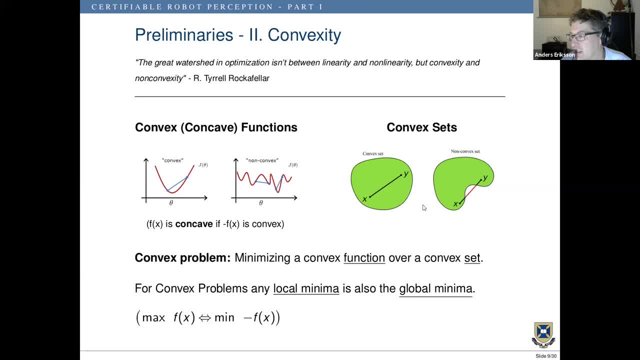 definition is here is that if you pick any two points in the set, any line segment you draw between the two needs to be completely within the set as well. so that holds for the convex set on the left but not for the numbers convex set on the right. 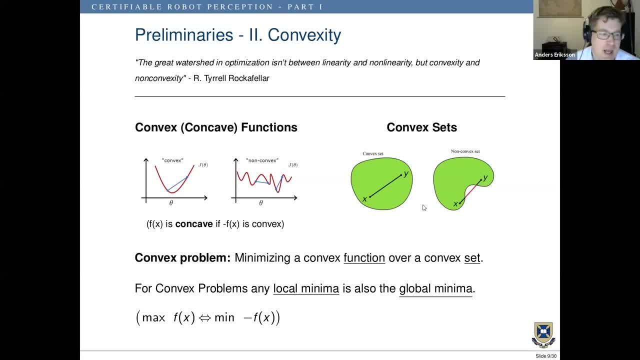 so when it comes to to optimization, it turns out that having a convex objective function is not enough. the constraints must also define a convex set. so we put these pieces together. it means that if you have a convex objective function over a convex set, it's called a convex. 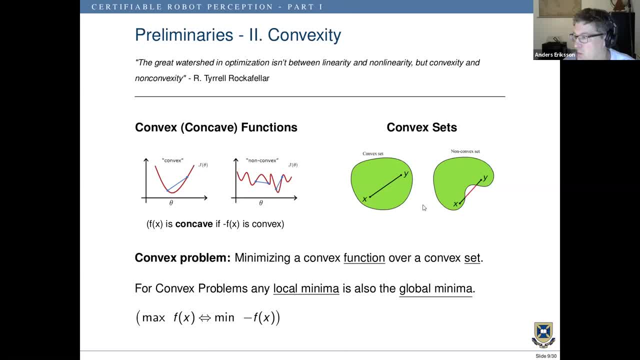 problem- and these are very, very nice problems to have, it turns out they're they're easy to solve. no local minimas. you can always, you're always guaranteed to find the global optimal. in fact, it turns out that if you solve the local- sorry, a convex- problem and you find a local minima, it's also always the global minima. 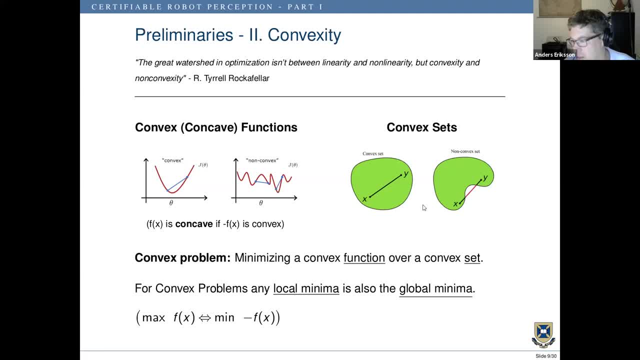 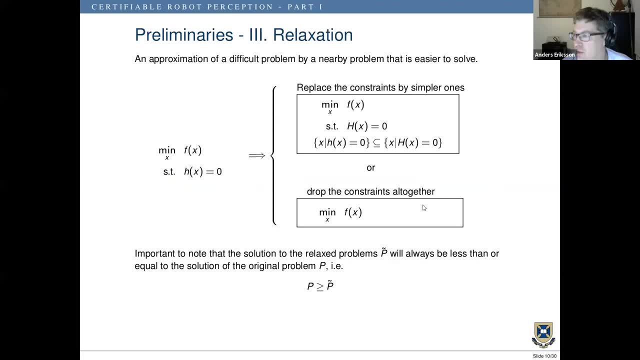 and again: maximizing concave function and minimizing convex function. sometimes you've used interchangeable. so then the third concept, that of relaxation. the idea here is basically that if your problem is too difficult, just try to place it with a simple one. you can always do this stereotypically. 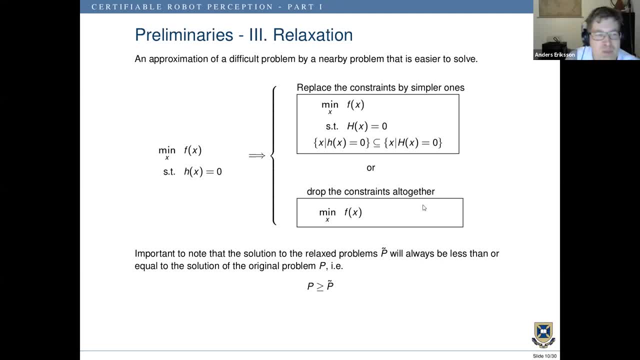 more, more formally, perhaps it's an approximation of a difficult problem by a nearby problem that is easier to solve. um? so, for example, if we want to solve this problem here on the left, that's the problem we want to solve. that's a primal problem that for some reason, is too difficult perhaps. 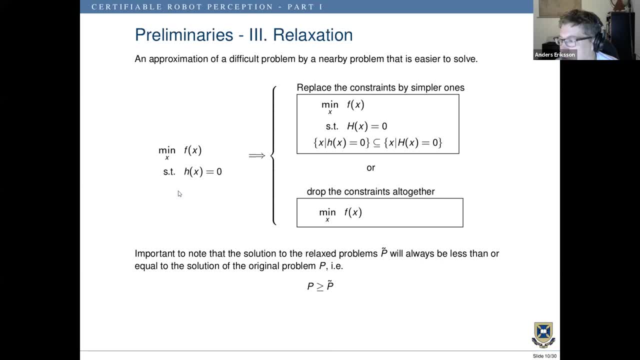 let's assume that the that the constraints, are particularly difficult to deal with here. one approach we can have is just um: replace the constraints, Replace them with constraints that are more manageable and, in this case, denoted uppercase H of X. Or, if you want to, you can just drop the. 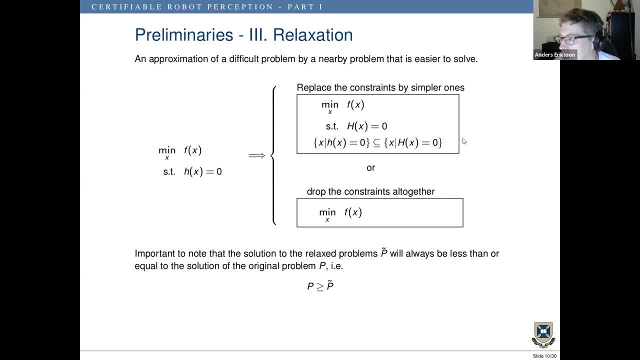 constraints altogether. That results in a relaxed version of your original problem. So for this, in this setting, it's important to note that the solution of the relaxed problem will always be less than or equal to the solution of the original one. That's important to remember because we're going to get back. 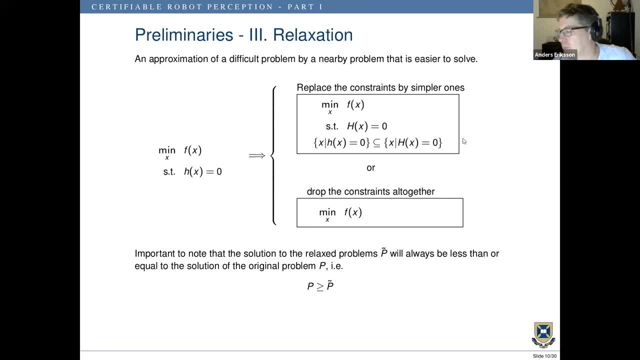 to that. Of course, a requirement for that to work is that when you do your relaxation, your relaxed set is bigger than the original one and it contains the original constraint set as well. But as long as you do that, the relaxed problem will always be less than or equal to the 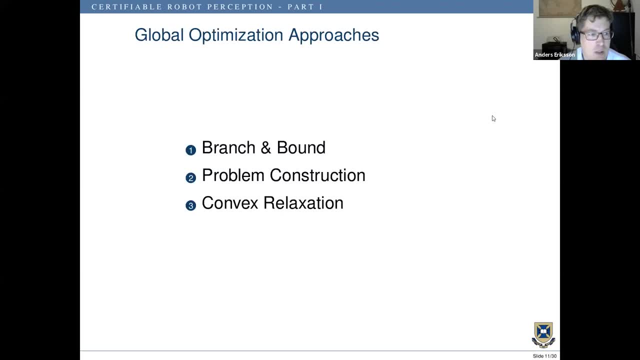 solution. So that is it. Those are the basics and we're now ready to start talking about global optimization And, as I mentioned before, I'm going to go through three different concepts. The first one is an algorithm called branch and bound. The second one is this approach of problem construction and the 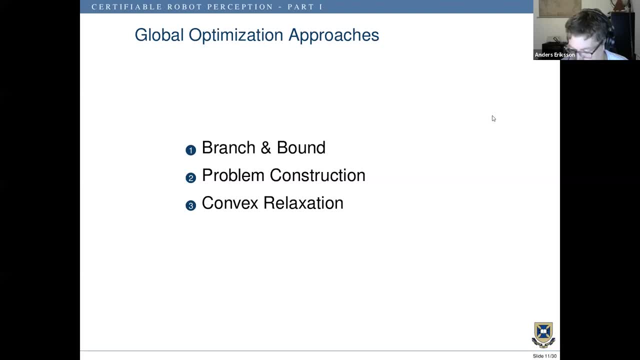 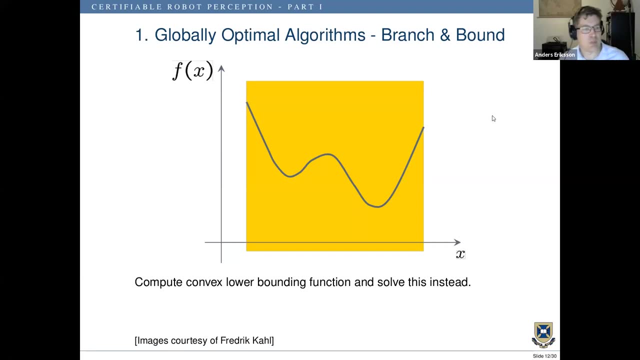 third, one is using something called convex relaxation, So starting with the branch and bound. So this is a very classical method in global optimization. It's been around for a while. It was first introduced back in the 60s. It's also a very general algorithm. You can find global solutions to discrete. 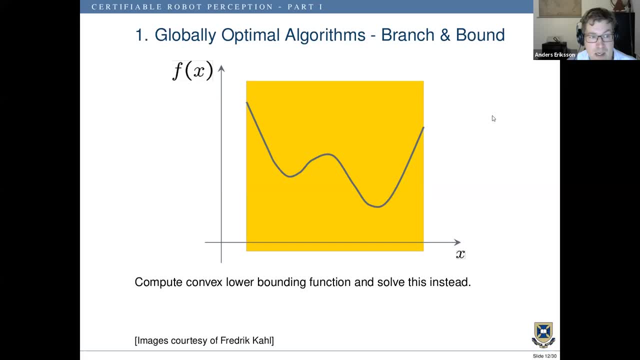 combinatorial as well as continuous optimization problems. And it's not. it's quite simple. It's a quite simple idea, but it's quite a clever one at the same time, And it's not too difficult to to understand what's happening. So let's, for example, say we want to find 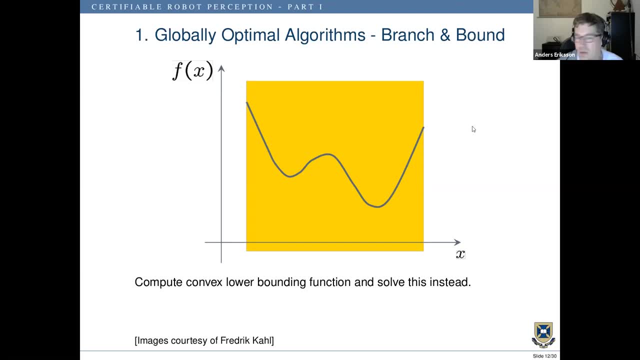 the global minima of this clearly non-convex function over some interval. Here the interval is shown in yellow. Now, instead of- and we assume that this problem is difficult to solve- This is called a plus or minus. This is a trivial illustration of it. 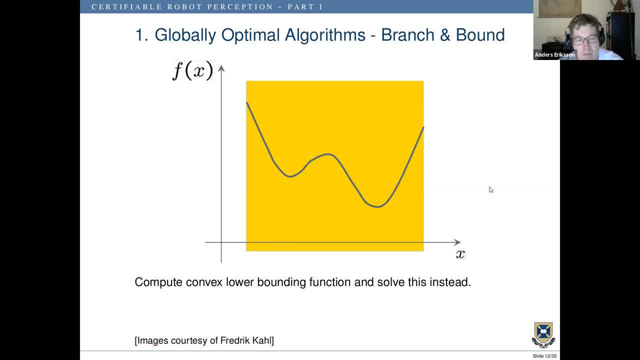 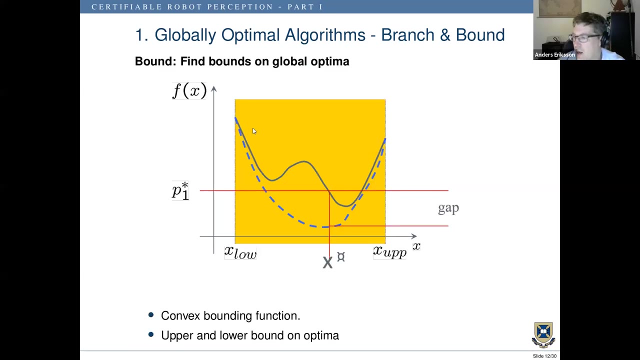 But the idea here is to find a lower bounding function to this blue function, Ideally a convex one or one that's easy to solve, and solve that one instead and then build on from there. So it might look something like this: This is our original objective function. We still have the same interval. 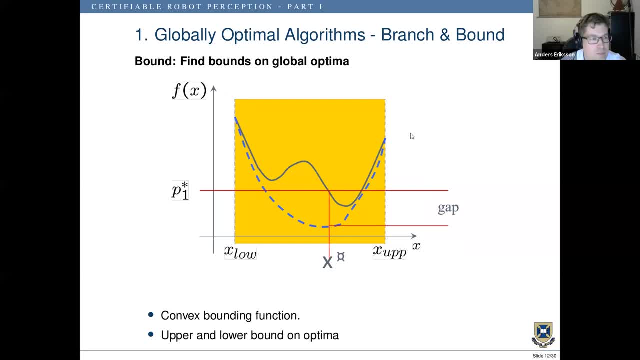 Let's say, somehow we're given this lower bounding function. This is a much easier one. As you can see, it's convex, And we solve that one instead, And if we do that, we might end up finding the minimum, which is down here somewhere. 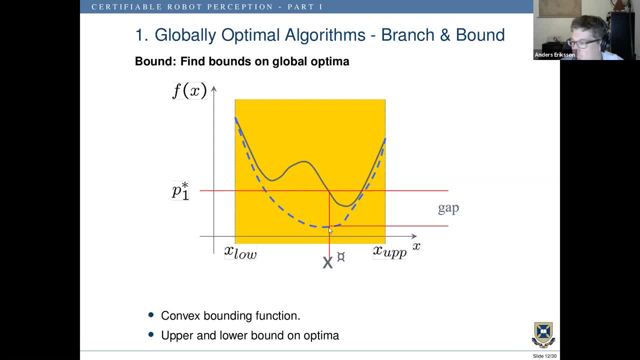 Again, we know, since this is a lower bounding function, this will give us a lower bound on the global optima. We can also evaluate the original objective function at the same point. That gives us that function value. So by doing this now, we've now found an upper bound and a lower bound on the global optima. 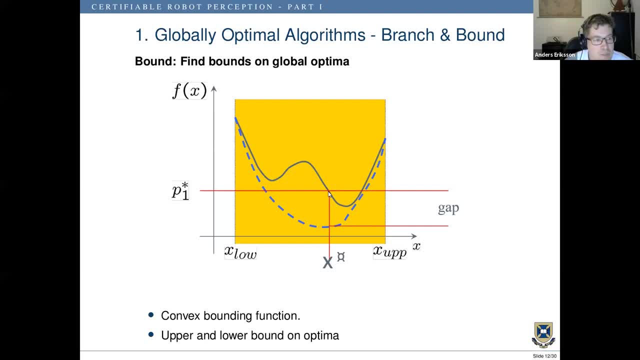 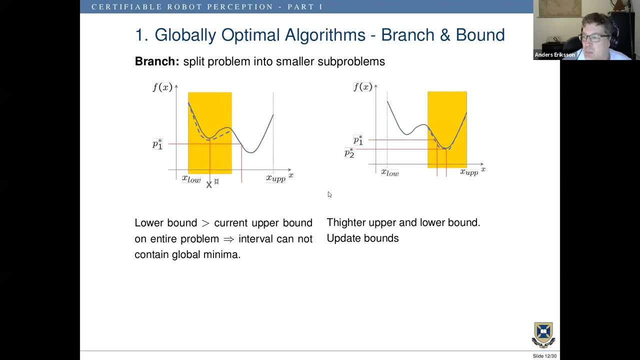 We know that the global optima has to be somewhere between those two. So what we then do is that we take our original interval and we split it or we branch it, We divide the problem into smaller subproblems. Here we use two intervals. 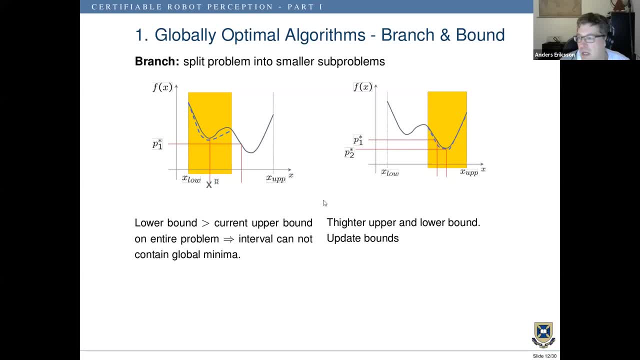 So we split into a left part and the right part And then we repeat the first step again. We do that individually for each of the subproblems. So if we look at the left interval, we find this lower bounding function and we solve that. 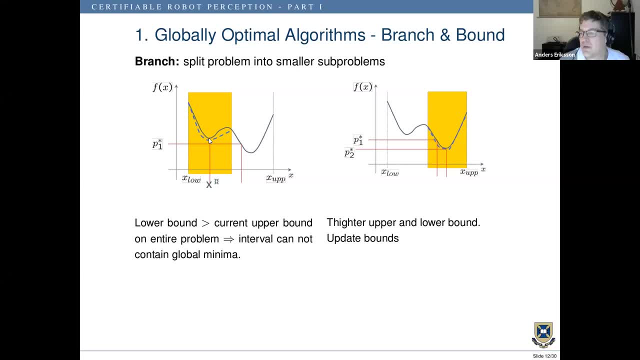 And then we also evaluate the function, the original function, at the same point. And then we do the same thing for the right side of the interval. We solve or we minimize the lower bounding function. Instead we also again for the left- sorry for the right interval- we get a lower bound and an upper bound. 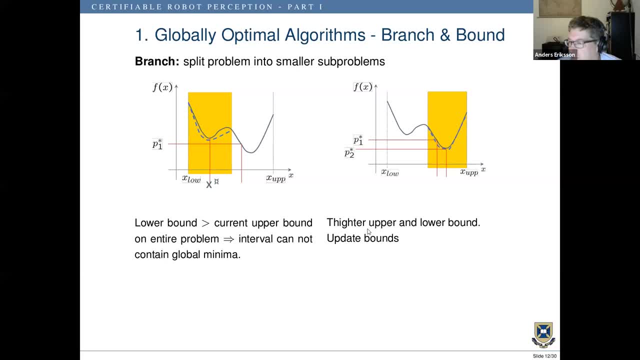 Now, if you take another look at this, especially if we're starting on the left interval, you can make the following observation: That the lower bound we get on the left interval is higher than the upper bound. we got on the previous step When we did the bounding on the entire interval. 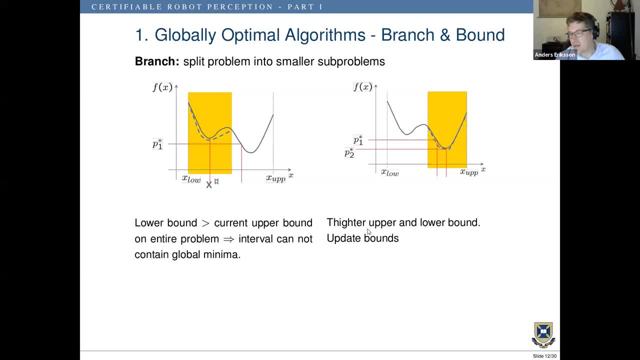 If you think about that a little bit more, that means as well that the global optima cannot be in that left interval And we can actually remove it altogether. We can focus our efforts on the right interval. On the right hand side. you can't do the same. 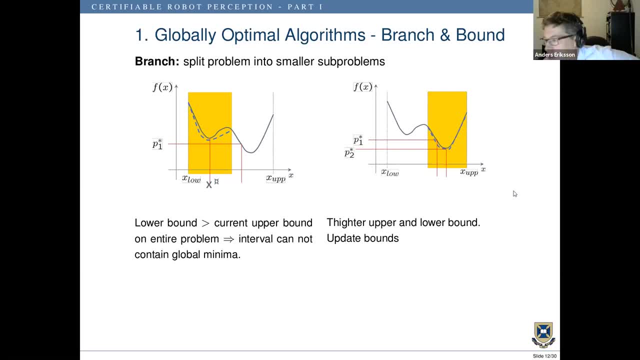 You can't exclude it because the bounds that we get are in between the old bounds. But we can do. since we know, now that we discarded the left side of the interval, We can now update the bounds. We now get tighter bounds on the way the global optima lies. 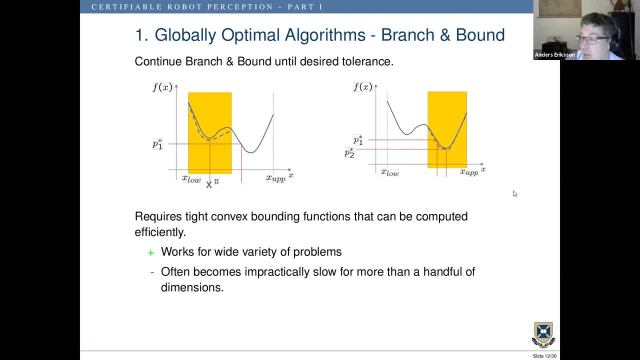 And then the idea is that you do that. Those are the only two steps you do. You bound and you branch, And you keep doing that until you manage to eliminate and discard enough intervals Or that the difference between the upper and lower bound is small enough and within some desired tolerance. 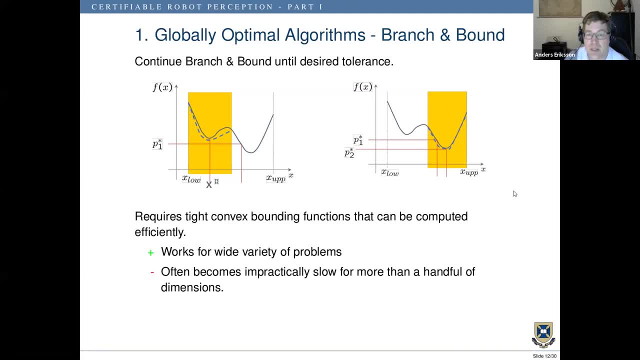 And then you stop, And that's essentially the idea behind this approach. You do this. It's sort of a clever way of doing your state-based search. The only thing that it requires- and I didn't really touch on too much- is that it requires this tight, convex bounding function. 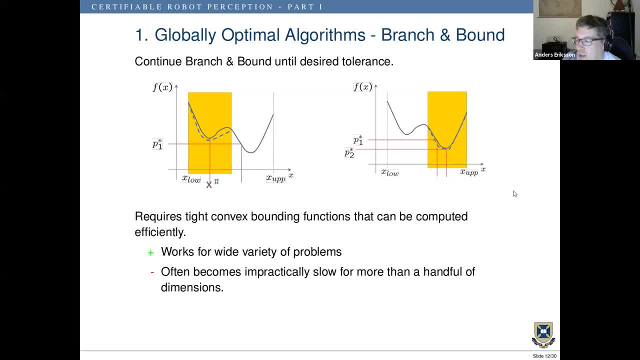 Some technical details run on the properties of such a function, Exactly how to find that function. It's not entirely trivial. It depends highly on the problem and the setting. But if you manage to find such a function, you can apply branch and bound. 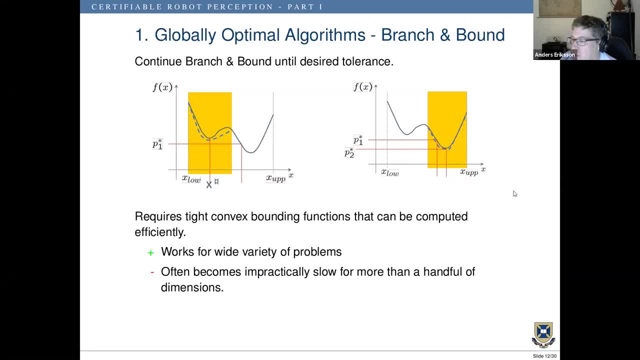 And there are some standard methods. you can try to do this, And the good side with this is that it works for a very, very wide variety of problems. The downside of it is that it can be quite slow and often becomes impractically slow for more than a handful of dimensions. 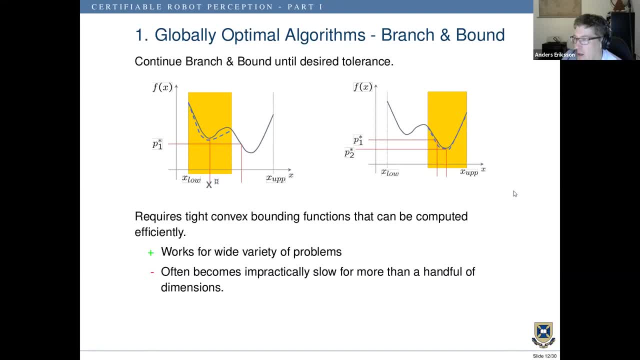 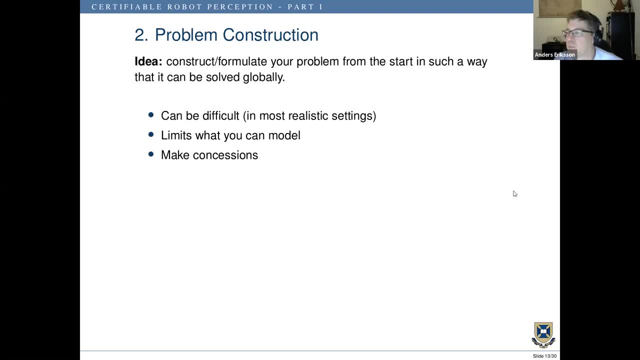 But it's worth mentioning. It's one of the more famous methods for doing global optimization. The second approach to global optimization is the one of problem construction, And this is actually the idea behind this one is that just construct your problem, formulate it in such a way that it can be solved globally. 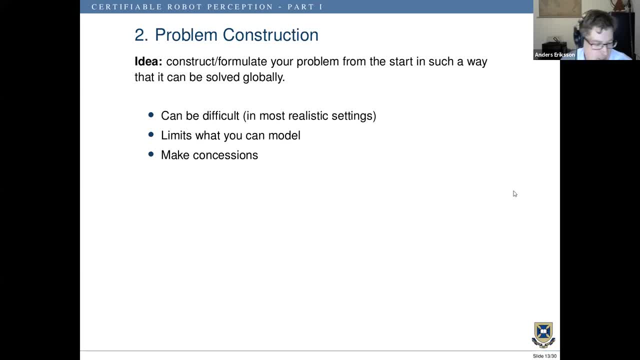 Unfortunately, this is not always that Difficult and it's not always possible. It requires, I suppose, a fair bit of experience in optimization and convex optimization and global optimization. It also limits what you can model And also you have to make concessions. 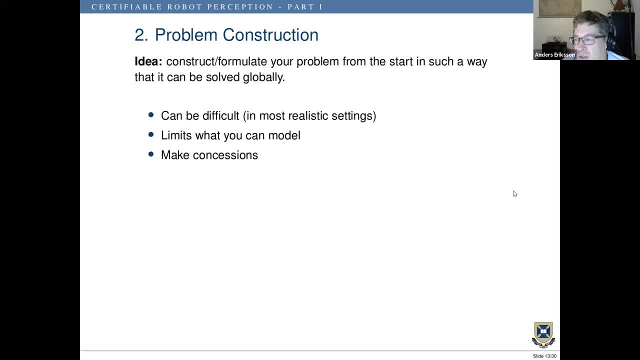 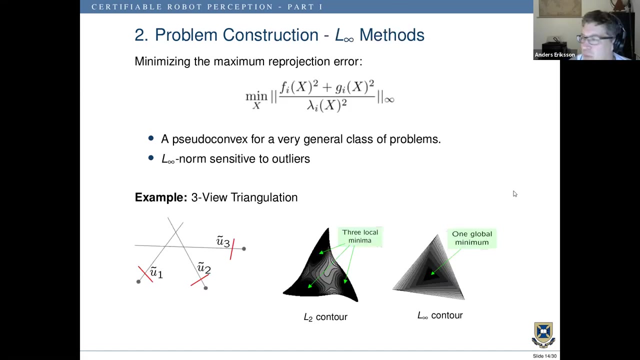 You have to make trade offs, You have to exclude certain things from from your problem formulation in order to be able to compute the To solve the resulting problem globally. And an example of this, perhaps the most well-known example from from at least from the computer vision community, is that of the L of infinity, or the max norm methods. 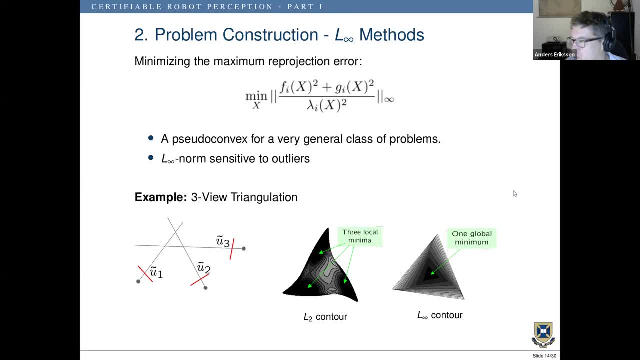 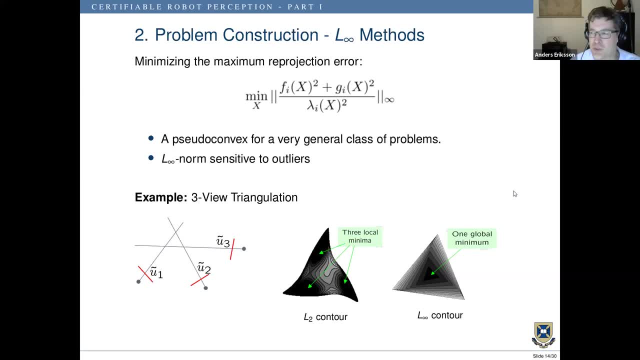 The norm on the residuals. If you choose that carefully, The problem is in fact solvable globally. There are no local minimums in such problems, And the norm, The norm that you normally would use in this situation, is the L2 norm. 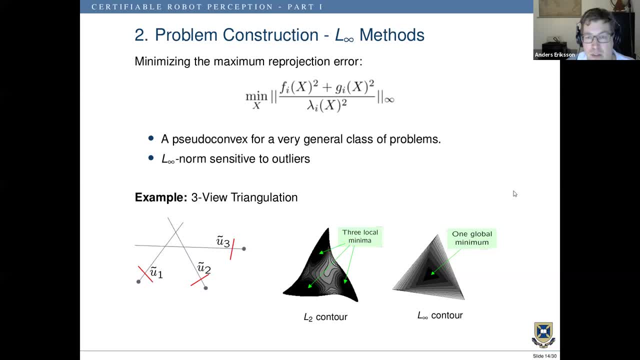 But that has been shown to be to be non-convex And it's also resulting in many local minimums. So here on the bottom, here you can see this, an example of three view triangulation. So here we have three cameras in 2D. 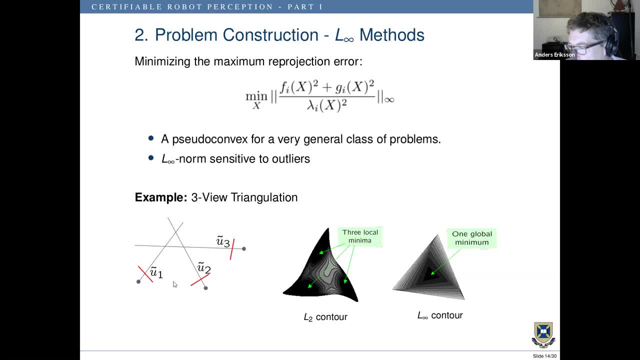 U1, U2 and U3 with known positions and known image points, And you want to find what 3D point gave rise to these, to these images, And you can then go on to show that if we measure those errors in the reprojection error using the L2 norm. 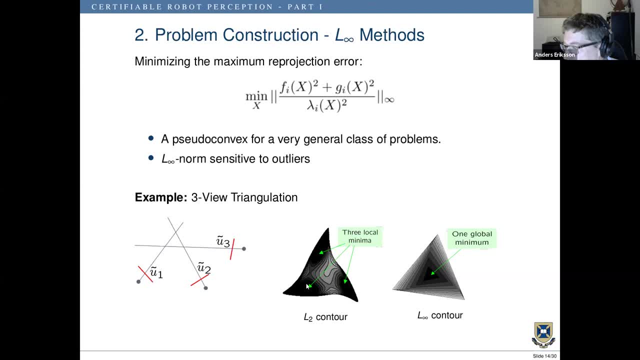 The landscape. In this case This is a 2D landscape. Looks something like this: We have three local minimums, But if you instead change the L2 norm to the L infinity norm, It turns out that problem only has one global minimum. 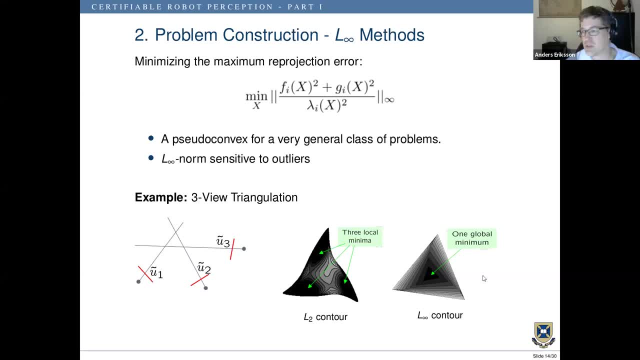 So this is all good, I suppose, But here the trade off of the concession that you have to make is that you're now dealing with a norm that is known to be very, very sensitive to our bias, So that's the price you have to pay here. 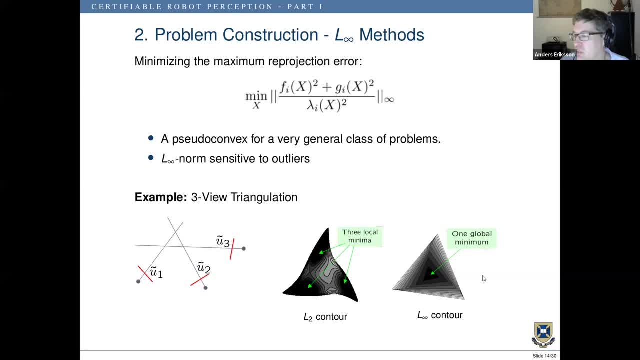 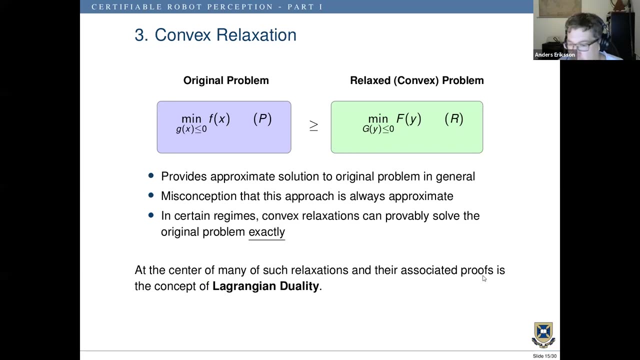 But this is- this is perhaps a good example of where you construct your problem From the get go To be one that you can solve globally. Then the next one I'm going to spend perhaps most of my time on is that of convex relaxation. 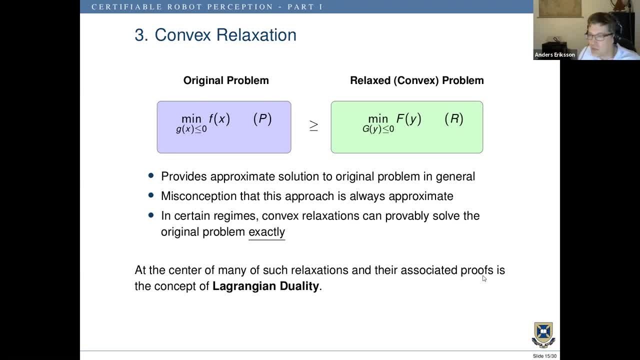 The idea here is again similar to that of relaxation that I mentioned before. So you have some original problem here, Our primal problem P, But for some reason it's too difficult to solve globally When I try and find some relaxed problem, ideally convex. 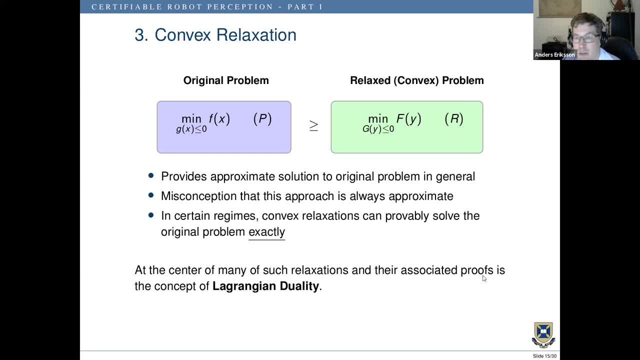 2M will solve that instead. Now, in general, an approach like this normally only provides approximate solution to the original problem, But it's a misconception that this approach is always approximate. It turns out that in certain situations convex relaxation, such as this: 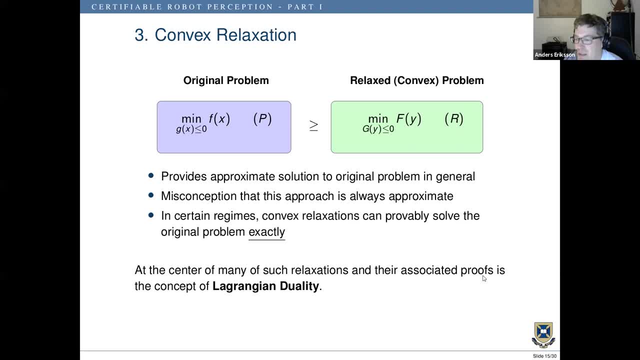 can provably solve the original problem exactly. And at the center of many such relaxation and associated proofs is a concept of Lagrangian duality, And because of this I'm going to try and take a few moments and explain Lagrangian duality in a bit more detail. 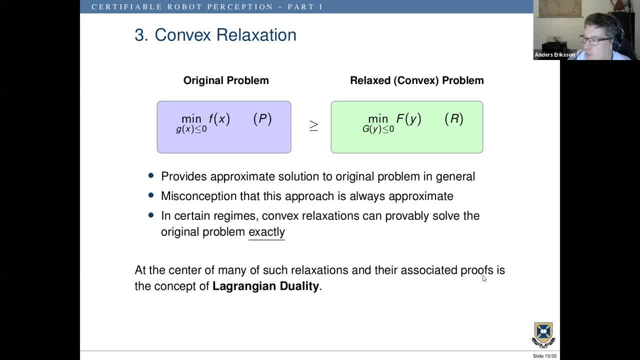 And since Lagrangian duality can be somewhat an abstract concept, the aim is mainly to be towards giving an intuitive understanding of what it is and how it works. And it turns out that all the concepts we need to understand Lagrangian duality are the ones we just went through in the preliminaries, a few slides back. 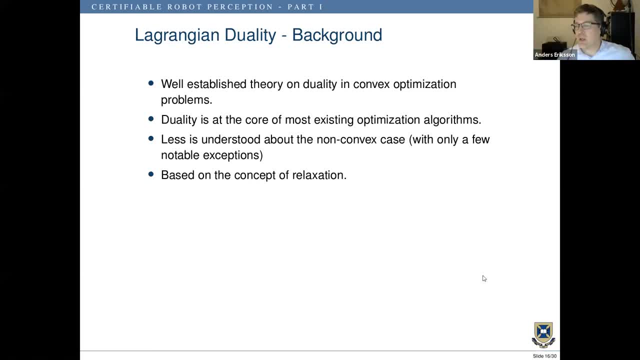 So the background of Lagrangian duality. It's a well-known concept. It's a well-established theory on duality, especially relating to convex optimization problems. Duality is at the core of most existing optimization algorithms, But less is understood about the non-convex case. 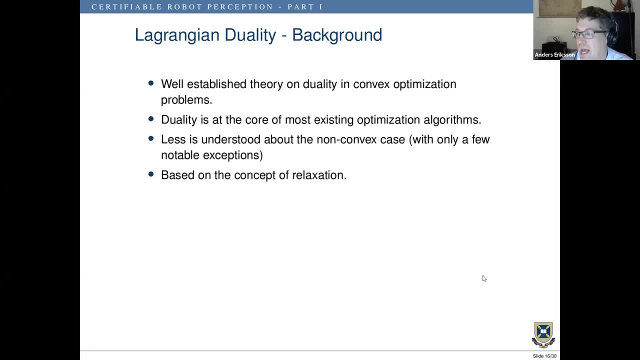 There's a few notable exceptions to this And it can be viewed as being based on the concept of relaxation And to try and illustrate that, we're going to start off with looking at this problem here. So again, this is our setting. 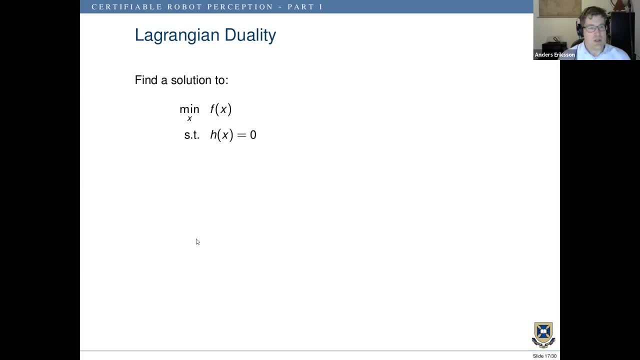 Let's say this is the problem we want to solve. I'm just going to use equality constraints for simplicity. You can do exactly the same thing using inequality constraints as well. It just makes the notation a little bit messier. So again, let's say we have this problem. 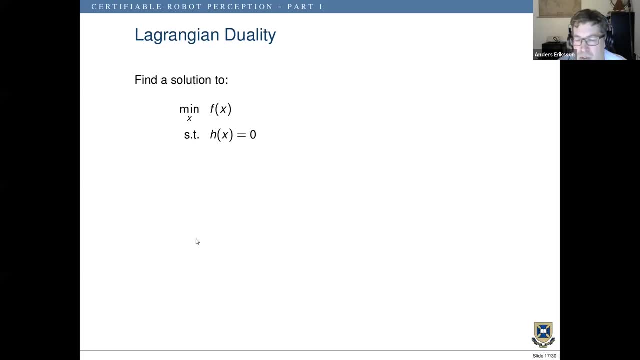 It's difficult to solve, And let's further assume that the issues we have with this are that the constraints are making it difficult. So what we can do is do what we did before, Using relaxation. we just say, well, OK, well, let's just remove the constraints and solve that resulting problem. 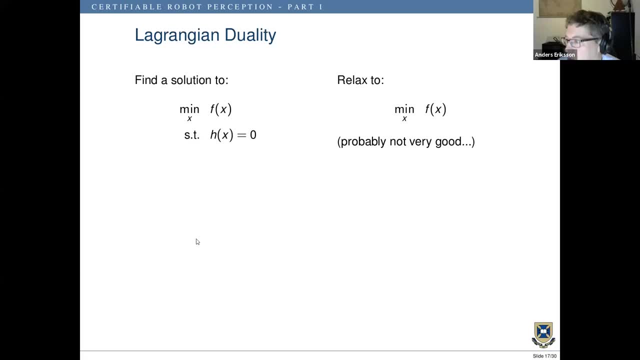 And the assumption here again is that if we do that, we can solve this relaxed problem much more easily And we can solve it globally. Now the downside here is that's probably not a very good thing to do, But let's do it anyway. 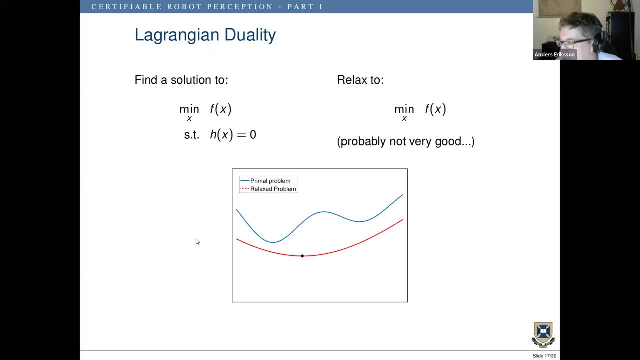 So let's say we have the following situation. This is sort of an attempt to illustrate the problem. We have the blue curve supposed to represent our primal problem And the red curve is supposed to represent the relaxed problem, the problem on the right. 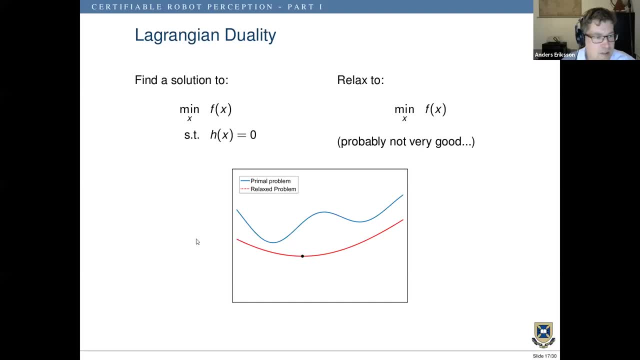 Now, this notation here isn't entirely technically correct, since our primal problem involves constraints And the blue curve. there are no constraints involved there. But again, this is mainly aimed at trying to correct the problem And to provide an intuitive picture of what's going on here. 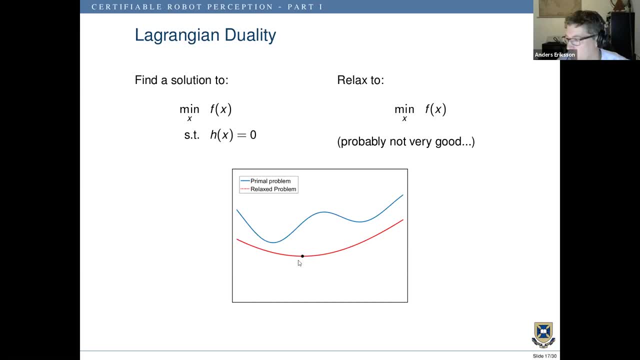 So let's say: we do this, We relax our problem And we solve this, And we arrive: We solve the red one, We solve the relaxed problem, We arrive at that solution there. It's not great, but it's not too bad either, I suppose. 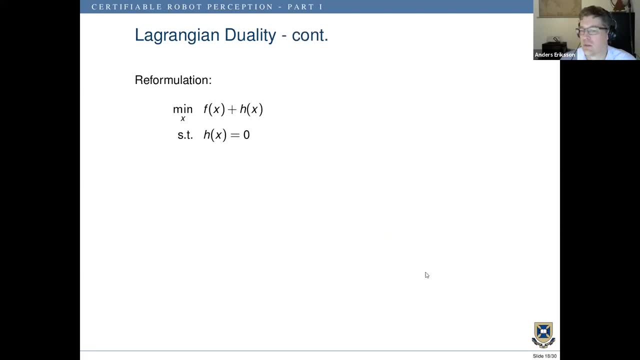 So what else can we do? Well, we can do the following thing: We can take our original problem and we can add h of x to the objective function, And we can add constraints to the objective function, Since h of x is always 0, we haven't really changed anything. 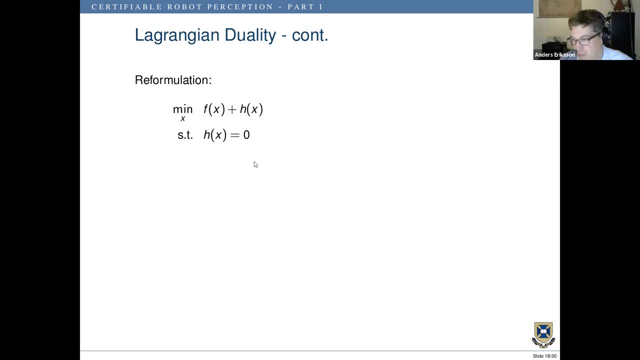 The problem is still the same problem. If we manage to find a global solution to that problem, it still will be the same. We haven't made things any easier by doing that, But the observation that we should make here is that the relaxation we get by removing the constraints is now a different one. 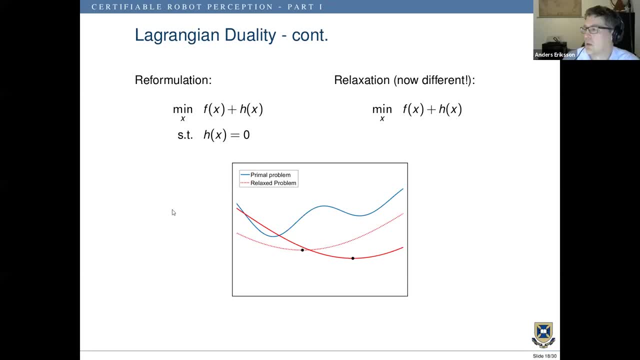 And if we do the same thing, We solve this relaxed problem. We'll get a slightly different one. So if we solve this one, we might look something like this And we arrive at a slightly different relaxed solution. We can do the same thing. 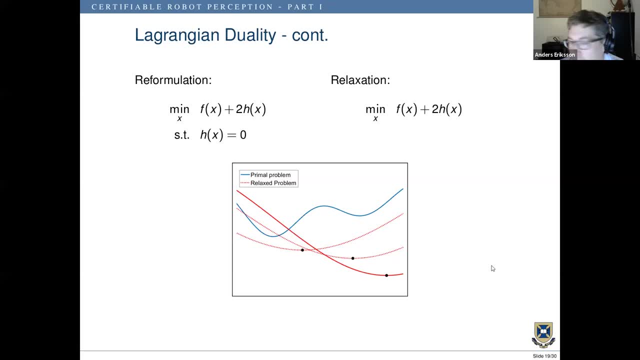 We can add something similar. We can add 2 times h of x to the objective. Relax that, And we arrive at yet another relaxed version of our original problem. And we can solve that, And we arrive at yet another solution. In fact, you can do this for any multiple of the constraint function that you want. 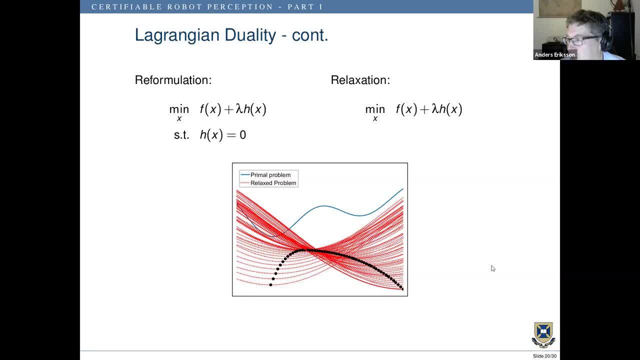 And if you do that for a whole range of relaxation where you denote different values that you multiply h of x with by lambda, it might look something like this: So, depending on the lambdas, you get a whole suite or a whole family of relaxed solutions. 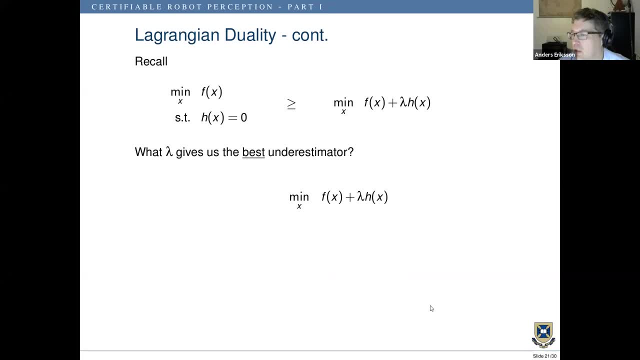 Now again, if you recall from the slide on relaxation is that since we're viewing this, what we're doing, as a form of relaxation, we also know that the resulting problems will always be underestimated. So lower bounds on the original problem. 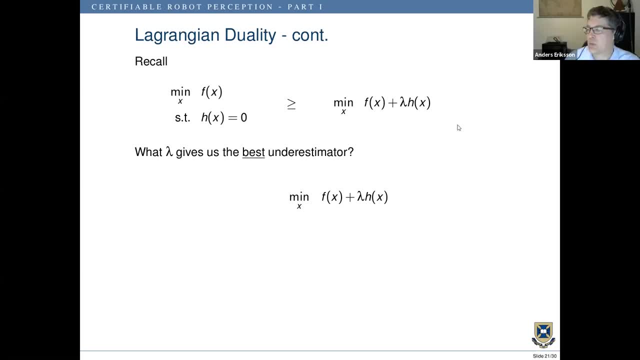 So we know it doesn't matter which lambda we put in there, the resulting solution will always be a lower bound on the original one. Now, the natural next question would then be to ask ourselves what lambda gives us the best underestimator. 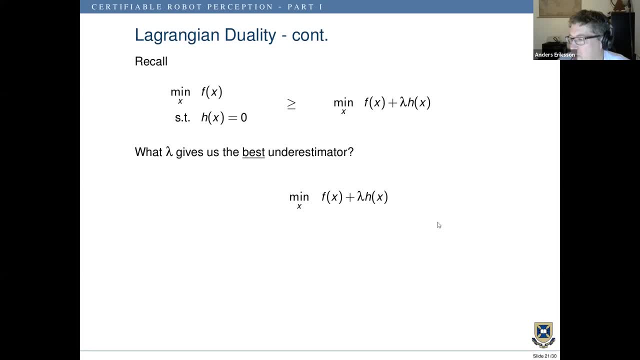 So which lambda gives the largest value of this expression here? So we want to maximize the minimization of f of x plus lambda h of x. Now some of these terms in this expression are so common that they've given them names. The first part, the f of x plus lambda h of x. 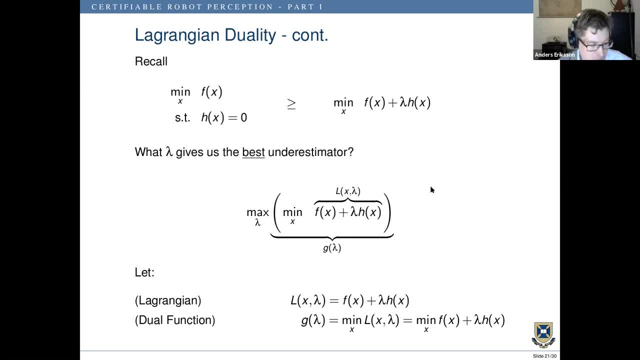 is denoted normally by L, And it's also called the Lagrangian or the Lagrangian function. The minimization with respect to x of the Lagrangian function is called the dual function, denoted g, of lambda. Again, this is a function of lambda. now, 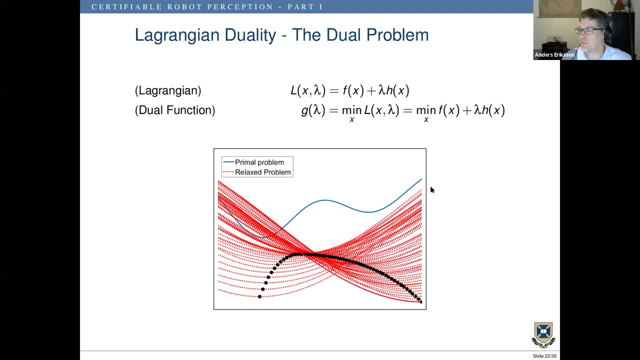 Yes, And that leads to sort of the following image, I suppose: When we have a Lagrangian, we have a dual function and we try different values of lambda and solve those functions, and the situation looks something like this: You remove the red bits, maybe something like that. 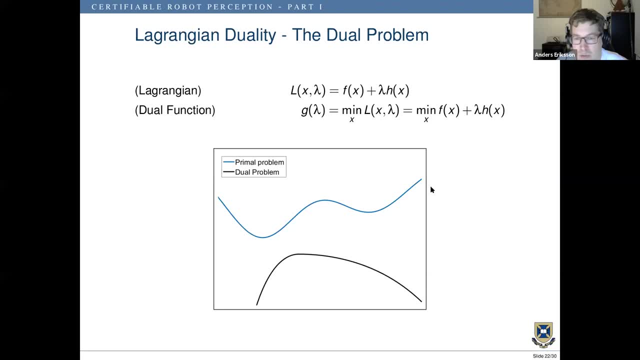 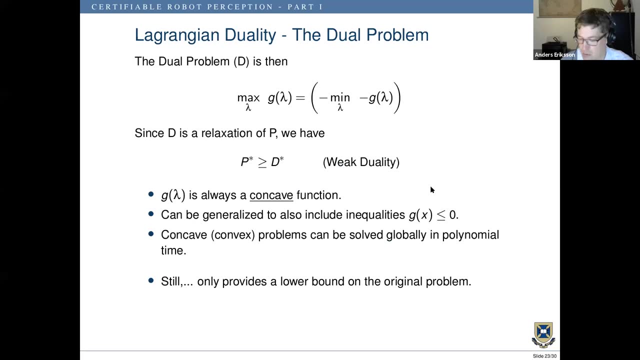 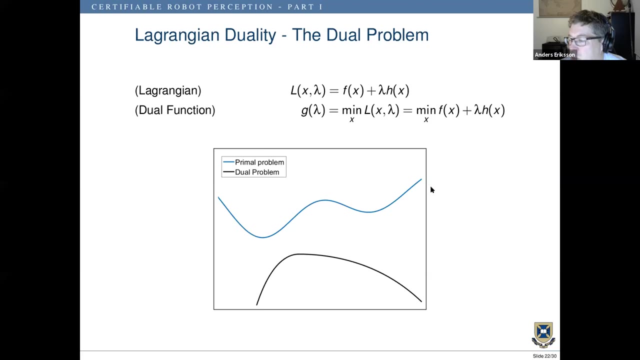 And this is then what is called the dual problem To finding the best underestimator to maximize the dual function. that is the dual problem to maximize the dual function to maximize g of lambda, to find the best underestimator of our original problem. 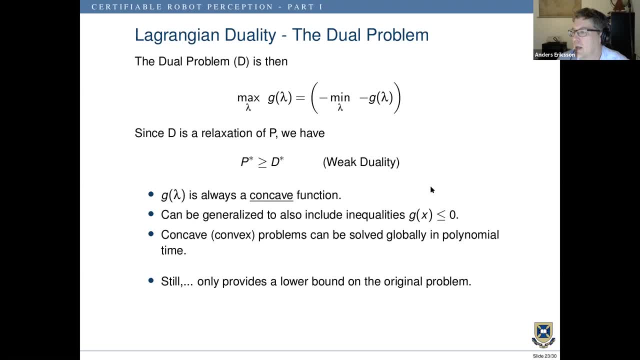 And again, since this dual problem is a relaxation, we have that the optimal value of the primal problem is always greater than or equal to the optimal solution of the dual problem. What's also interesting is that, as you saw, the dual function here is shown as a concave function. 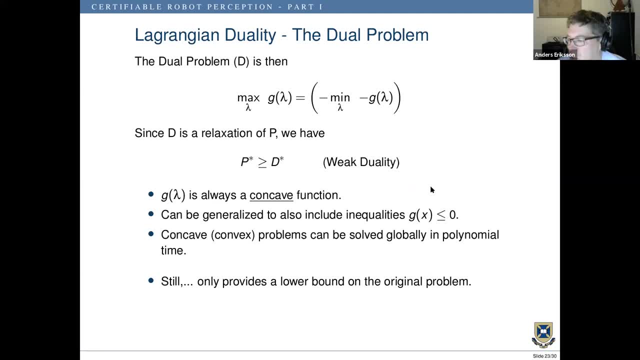 And that's not by accident, It turns out- you can actually show that g of lambda is always a concave function. Even if the original problem is not a convex problem, the dual function will always be a concave one, And maximizing a concave function is something that we can do efficiently. 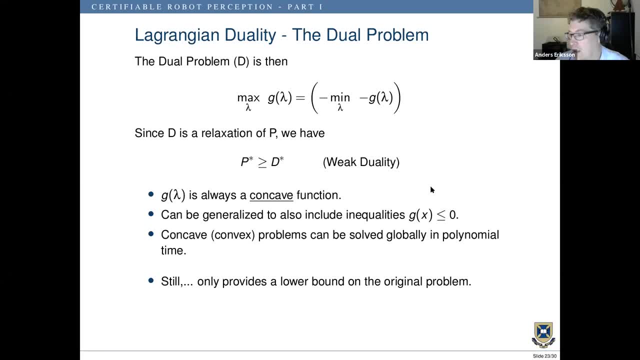 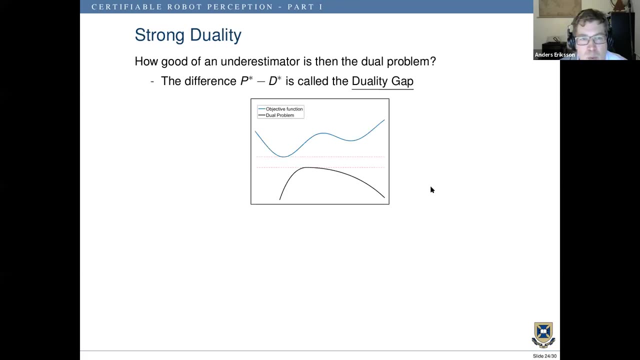 and do it globally. And again, like I said before, you can generalize this to also include inequalities. Now, this still only provides lower bounds to the original problem. So a natural question then is to ask how good of an underestimator is? then the dual problem. 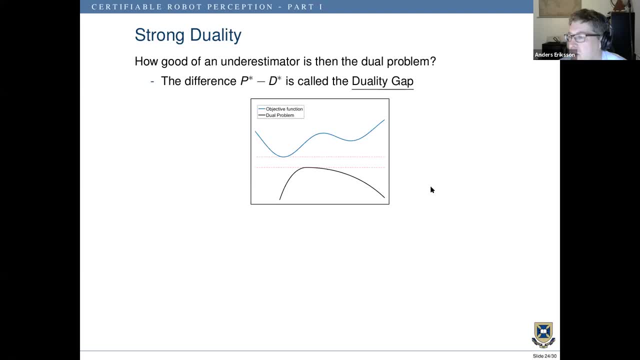 The difference between the solution of the primal p star and the solution of the dual d star is called the duality gap, And it might look something like this in our problem. it did, But sometimes this happens That p star and d star coincides. 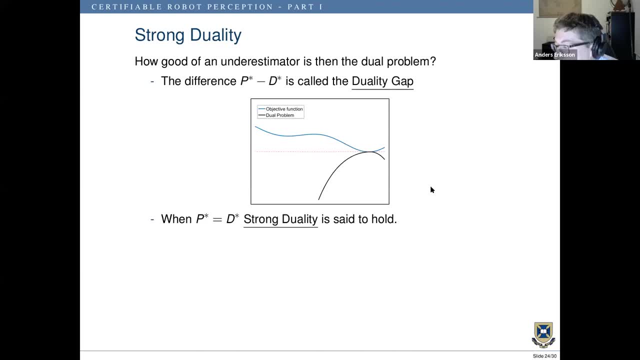 So p star is equal to d star and the duality gap is zero. When that happens, we said that strong duality holds And again, there's a lot of established theory has been for a long time on how and when this happens. 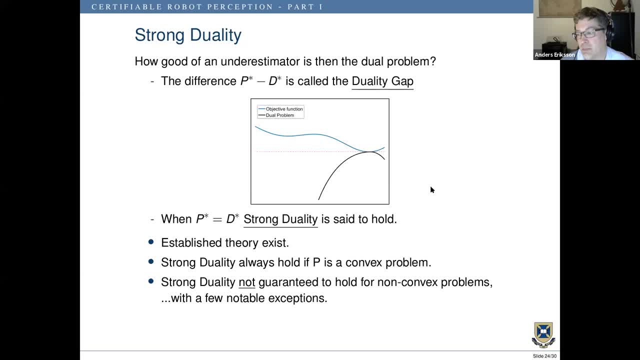 But, for example, strong duality always holds if the primal problem is a convex problem. There's some technical details around that, But in general that's true. But strong duality is not guaranteed to hold for non-convex problems, with a few notable exceptions. 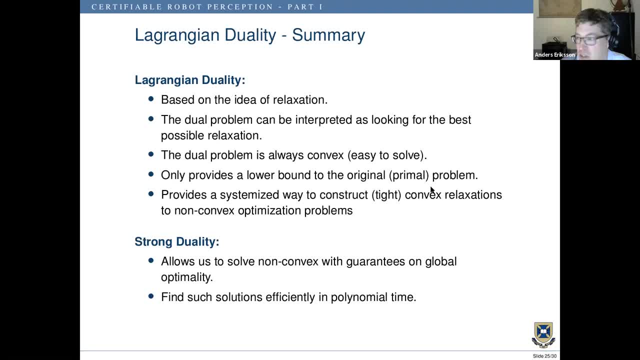 So just a quick summary of Lagrangian duality. Yeah, and that is essentially it. That is the idea behind Lagrangian duality And, to just quickly summarize it, it's based on the idea of relaxation. The dual problem can be interpreted. 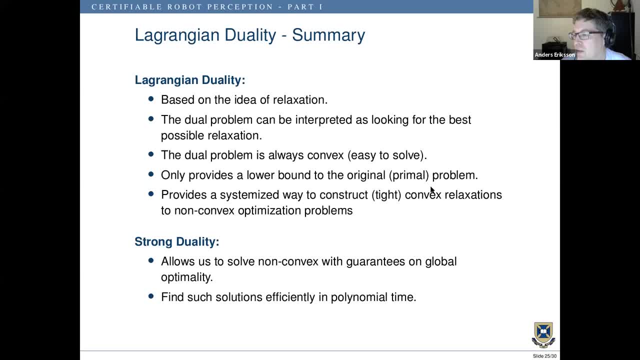 as looking for the best possible relaxation. The dual problem is always convex, so it's easy to solve. But it only provides a lower bound to the original primal problem. But it does provide a systemized way to construct tight convex relaxations to non-convex optimization problems. 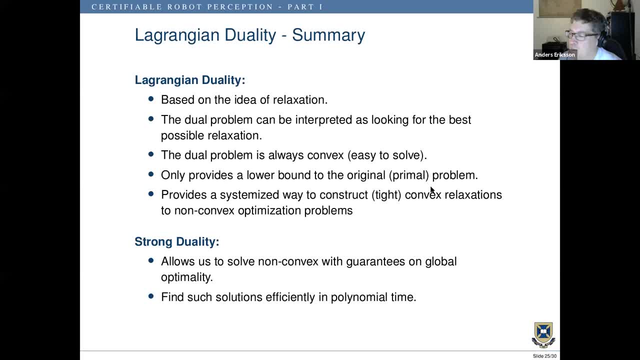 In addition to that, if we have strong duality, if we can show that that property holds, it then also allows us to solve non-convex problems with guarantees and global optimality, And you can find such solutions and do it efficiently. 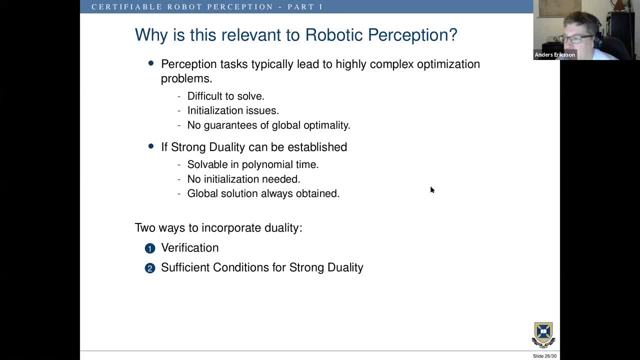 So why? Why is this then relevant? Again, like I said in the beginning of the talk, that most of the problems that we're looking at in perception or vision lead to complex optimization problems, ones that are difficult to solve, But if we can establish this property of strong duality, 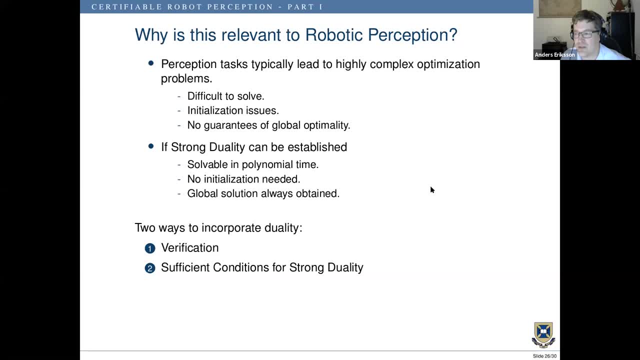 at least in some form. we gain a lot, And I guess the most important one is that if that holds true, we're always guaranteed to find a global solution to that problem. We don't have to worry about initialization. It might affect sort of runtime. 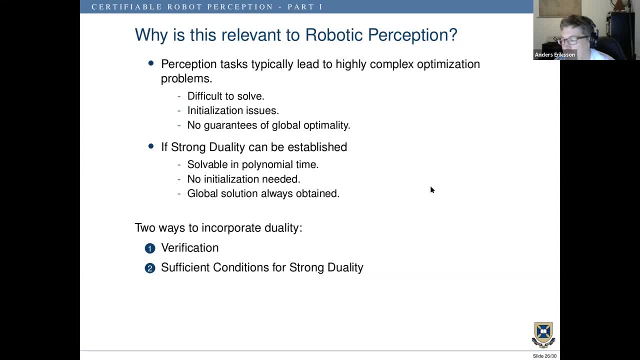 but as far as global optimality goes, it's not, It's not important, And you can also solve the resulting problem efficiently And at the moment there are two ways, I suppose, to try and incorporate duality or essentially strong duality. 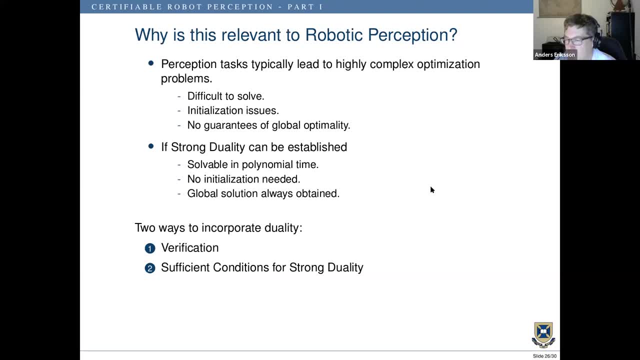 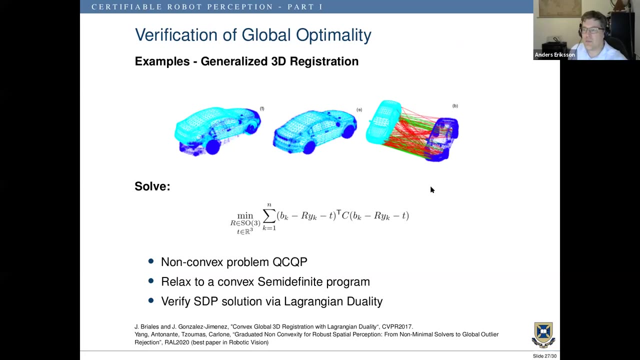 in robotic vision and computer vision. One is called verification or certification of solutions, The other one sufficient conditions for strong duality. An example of the first one is this problem: here It's called generalized 3D registration. Here you want to register. 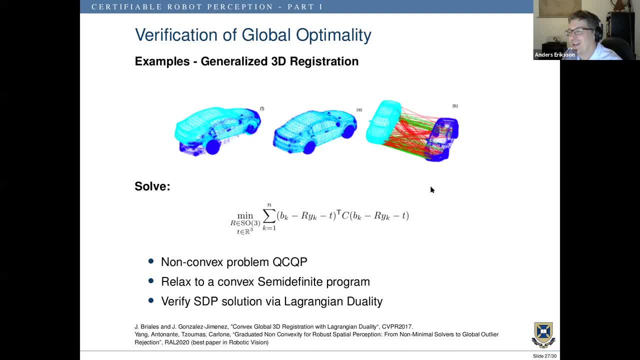 two 3D shapes with each other. You want to find the rotation and the translation that aligns them as well as possible, And you do it in such a way that it does not only involve points, but it might also involve lines and planes. 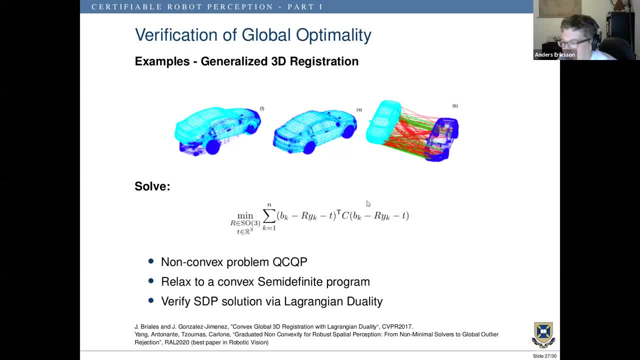 That problem itself. you want to solve something that looks a little bit like this. You can formulate that as a quadratically constrained, quadratic program, denoted QCQP. It can easily be shown that those- Especially in this case there's a non-convex problem. 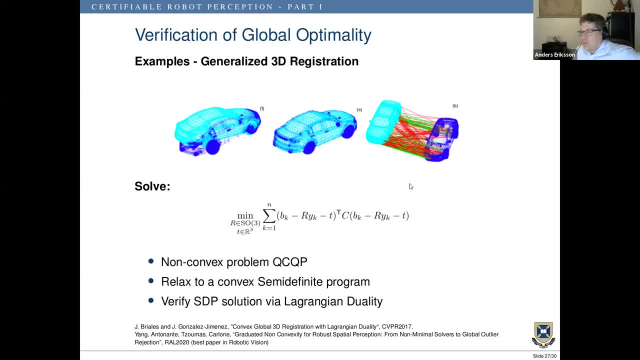 And what they do in this example is that they relax this using semi-definite program and kind of solve the dual and hope for the best- Well, not hope for the best, but they solve it anyway- And once they find the global solution to the dual problem, 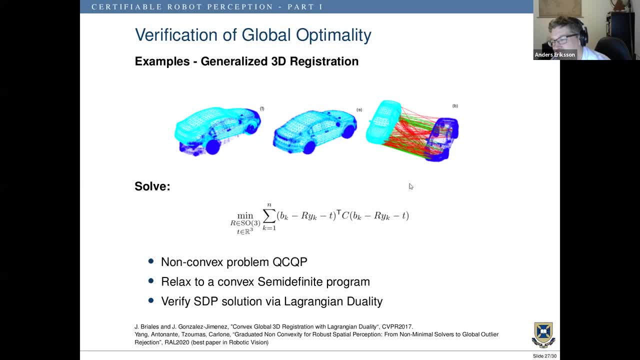 then you can try and construct a feasible primal solution from that dual solution. And if you then manage to show that the duality gap between those two solutions is zero, then you don't have to do anything more. You're basically certified that the solution that I have 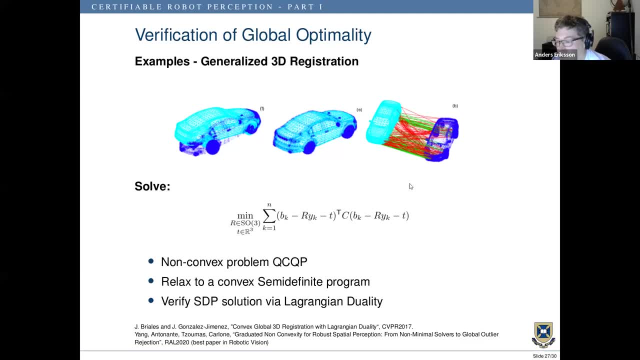 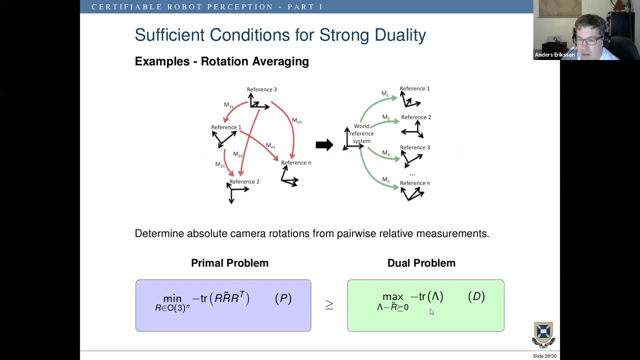 is the global one. There is no better solution. So there's two papers here that are reference to: One is from Brialis et al and one is from Yang and Calone, published only a few months ago, I think. And then the second example. 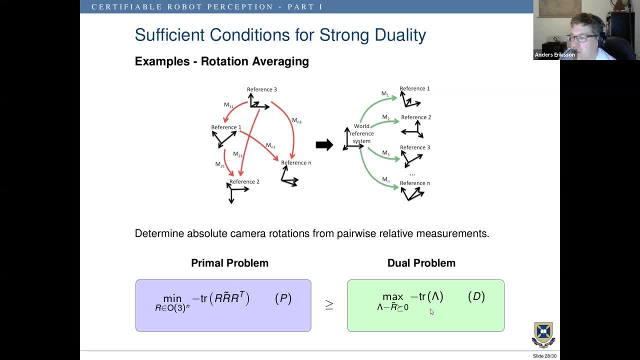 here is the problem of rotation averaging. This is the problem of determining absolute camera rotations from pairwise relative measurements. So here we have, for example, four cameras and we know their relative rotations and we now want to find what are their absolute rotations. 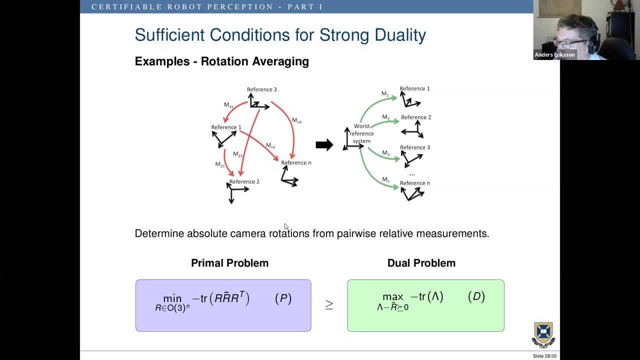 at least up to some global world reference system. And similarly here you can show that the primal problem is can be written as it is done on the left here, And the associated dual problem looks like that It's a semi-definite problem as well. 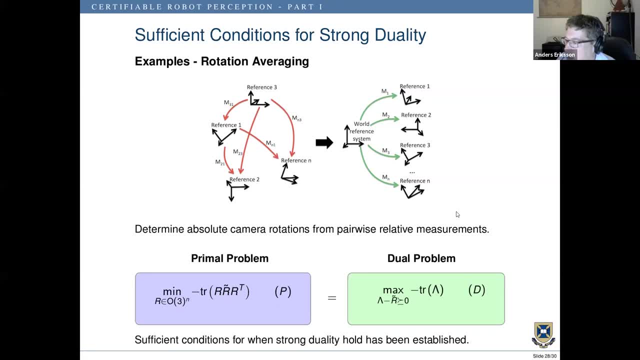 But for this problem you managed to show something slightly different. You can actually show beforehand. You don't have to check each individual solution, but you can actually try and provide sufficient conditions for when strong dualities always will hold. So in this case, 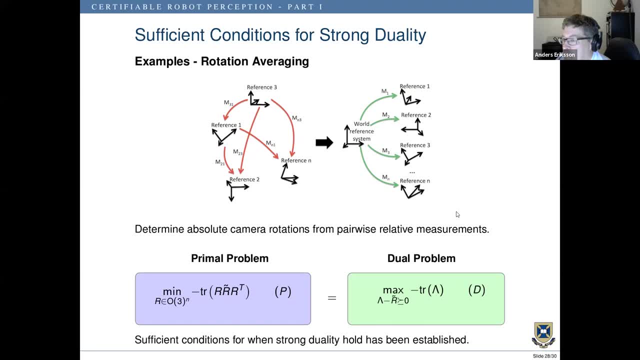 you can actually show that if the noise levels are sufficiently small, strong duality will always hold, which means that if that is true, if those noise measurements are small enough, you can solve the dual problem and you're guaranteed to always find the global minima. 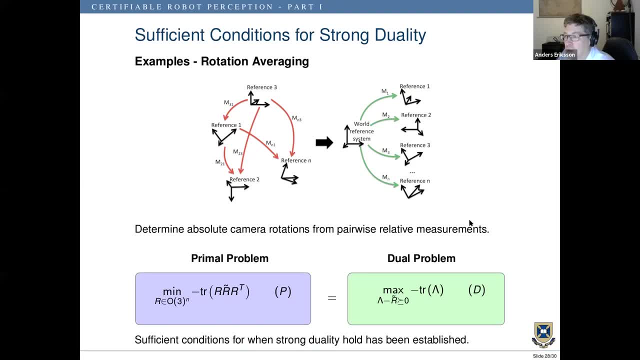 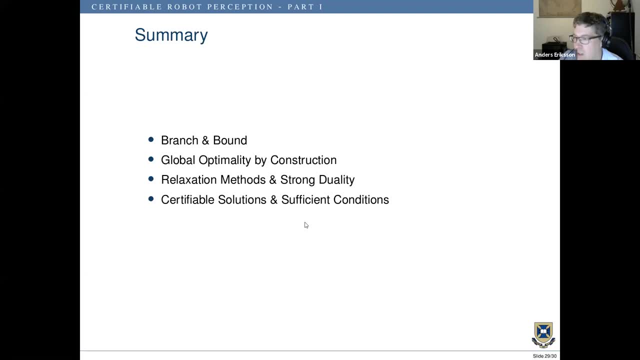 You don't have to check anything, You don't have to verify anything. Yeah, So that's basically it for my talk. I think I went over a little bit on time, so I might just finish there. See if there are any questions. 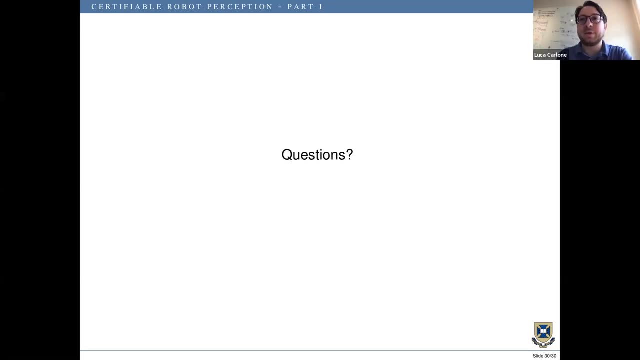 Thanks. Great presentation, Very, very clear. I think we have a question about. So what's the use of moving into the dual view if it is guaranteed to find the global minimum only for convex problems For which we cannot really use existing solver? 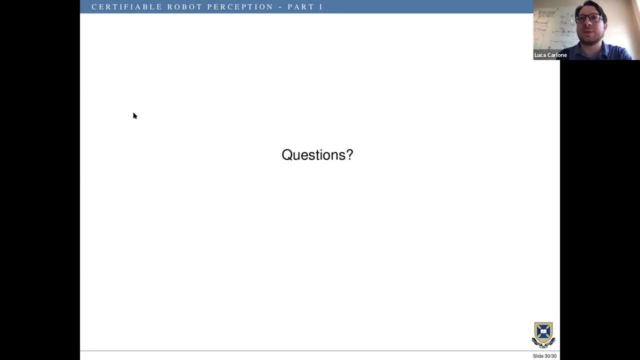 So I guess the question is: how should we use the dual in non-convex? Why do we care about duals in non-convex problems? Well, I guess you can. It all comes down to if you're able to show. 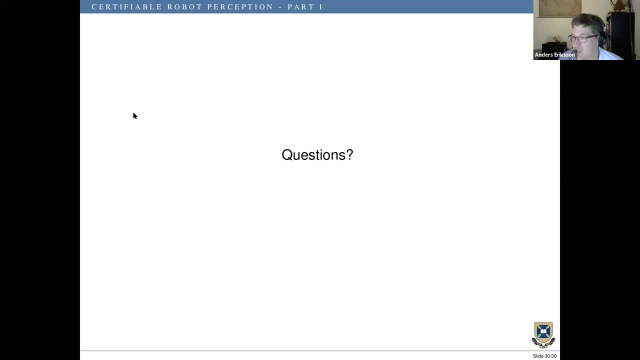 that this property of strong duality holds. it essentially gives you the answer. So it is guaranteed to hold for non- Sorry For convex problems, And again, but for non-convex ones. it's not entirely clear, But it is a tool. 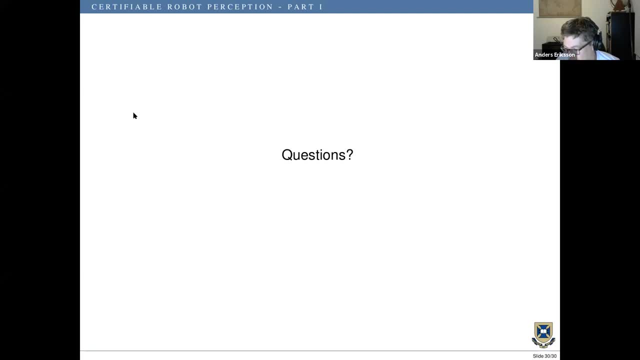 that can be used to to verify your solutions or show that the solutions that we give are always the global ones. Did that make sense? That was a very good answer. I think It does. I would make the statement even stronger. I would say that the reason why 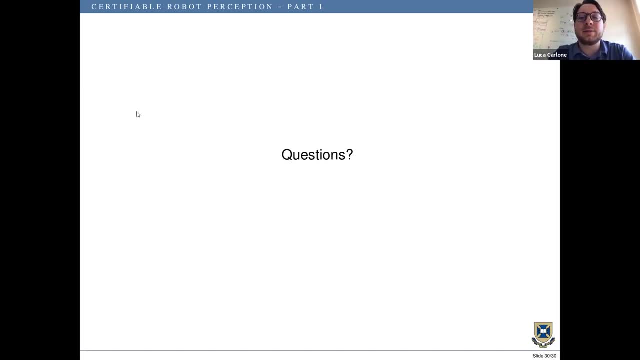 we are so concerned about strong duality in this tutorial is that indeed many non-convex problems showing up in geometric perception. they have strong duality. They are non-convex but they have strong duality. Yes, Yeah. And to make that statement, 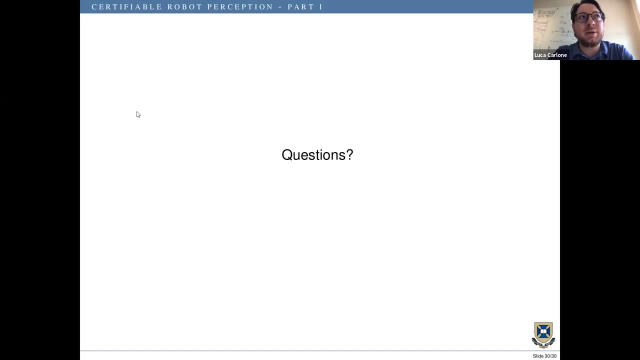 a little bit more precise. they have strong duality, typically when the noise in the measurements is not huge, in the sense that you know at some point strong duality will break. But the important thing is that it breaks in a setup which is too extreme. 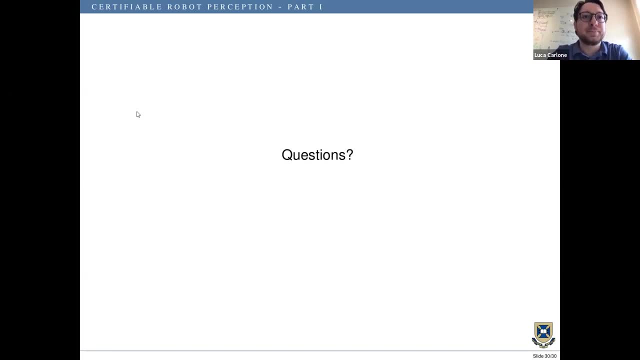 to show up in practice. Yes, Yeah, No, I definitely agree with that. I mean to me as well. what I find interesting with it: it provides a very formalized way of answering the question of: is my solution the global one? 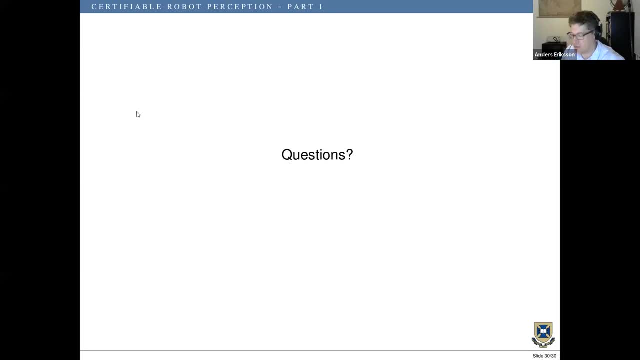 And then exactly what approach you take around it, if you do it either as a sort of certification approach after the fact, or if you try to say something before, even before you start your optimization. I guess that depends on the problem itself and how amenable they are. 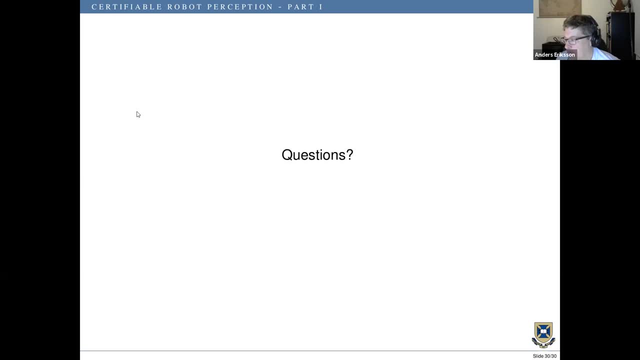 to each of those approaches. Cool. There was another question before which I think was partially answered by TJ in the chat, But I think Maolin was trying to get a little bit more insight about why the L-infinity norm was a better choice. 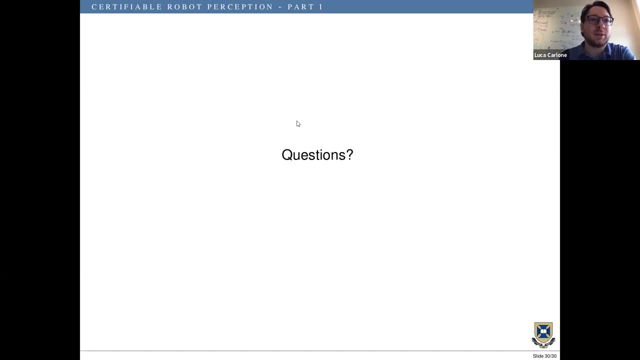 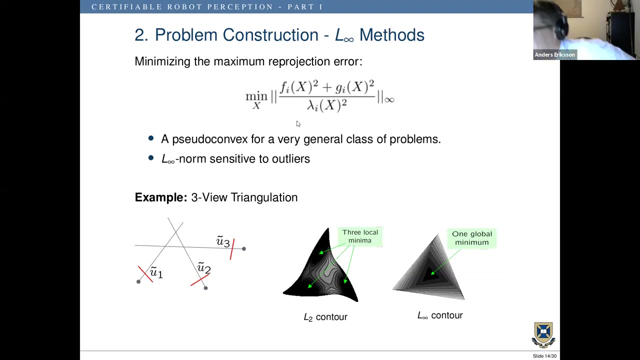 Like you know why you got convexity, or you get a unique global minimum if you have the L-infinity norm. Ah, that's It turns out if you really dig in under the hood and look at the very deep into the mathematics. 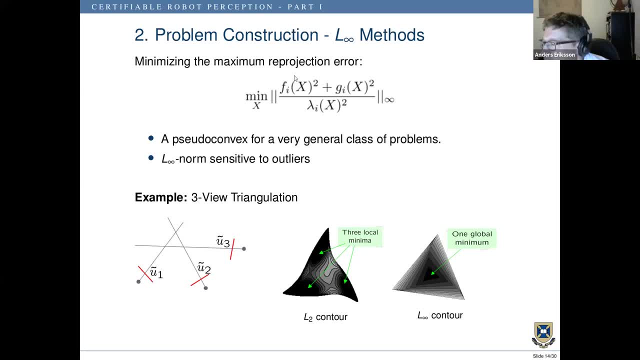 it turns out that if you do this, if this function, You can still see my sharing right here. So you want to minimize these residuals and these. It turns out that this term here is something called a pseudo-convex function, And it turns out that the maximum of 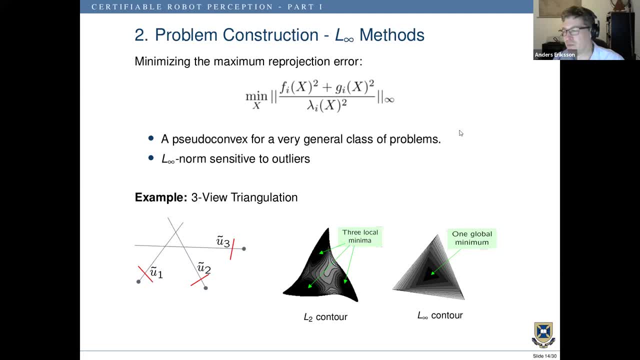 A number of pseudo-convex functions is still pseudo-convex, But unfortunately the sum of squares of pseudo-convex functions is not pseudo-convex. That's the thing that differs the two. Very interesting, Okay, At this point. 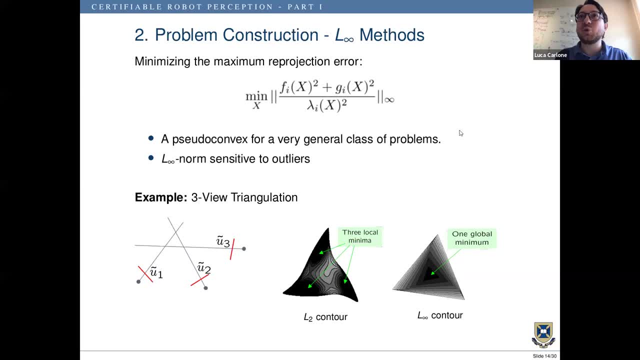 I think we have Our 10-minute break became a 2-minute break, So I suggest that. Well, there is another question. So I think let's take the other question and we'll do without the break. So the other question is: 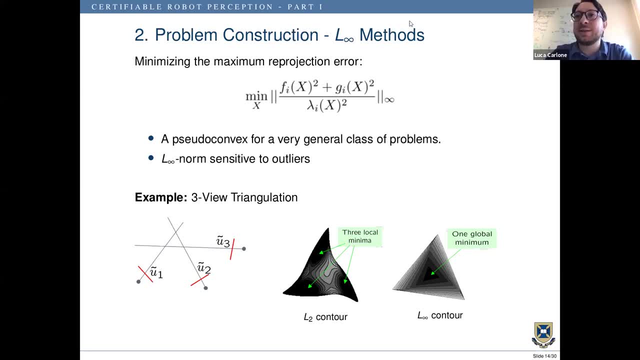 Lagrangian, duality seems to be a particular way of constructing convex relaxation. Is there proof that the resulting relaxation is the best you can get? Yes, there is. You can show that the The convex relaxation you get using duality is the tightest one. 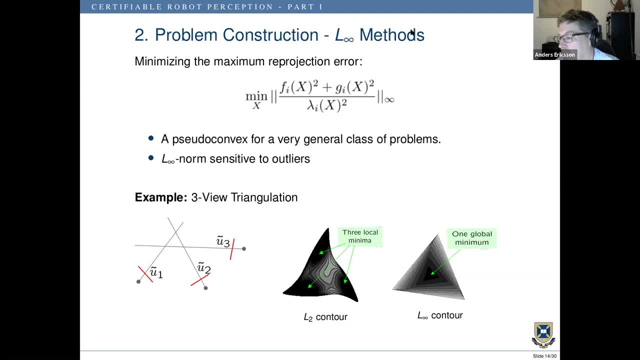 So it's the one, that's? Yeah, It's the best possible convex relaxation of that particular problem. Cool, I think we have, I don't know, the reference off the top of my head. I think I will show an example exactly of that. 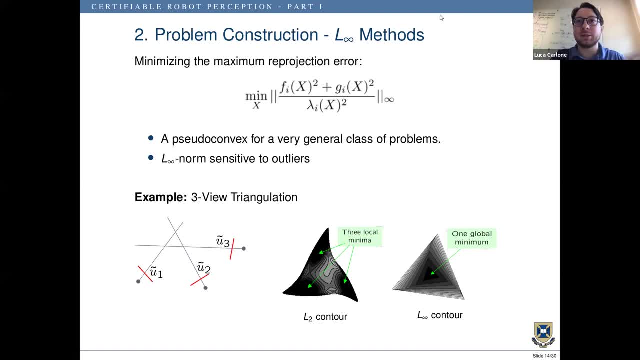 and the relation between Lagrangian duality and more traditional view of convex relaxation in my talk as well. Yeah, Thanks, Anders. At this point it should be like, you know, a standing ovation or something. Unfortunately, like you know, with Zoom, 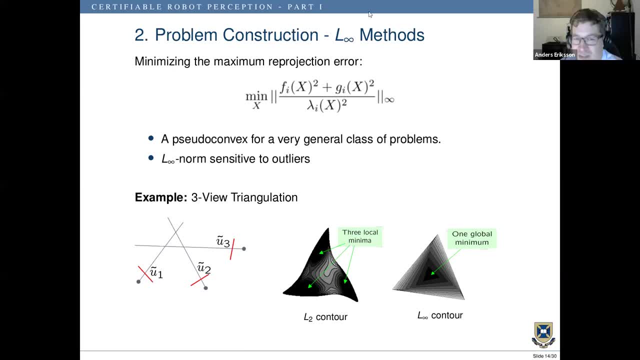 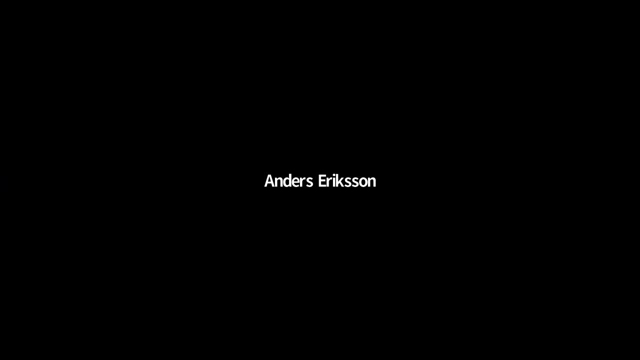 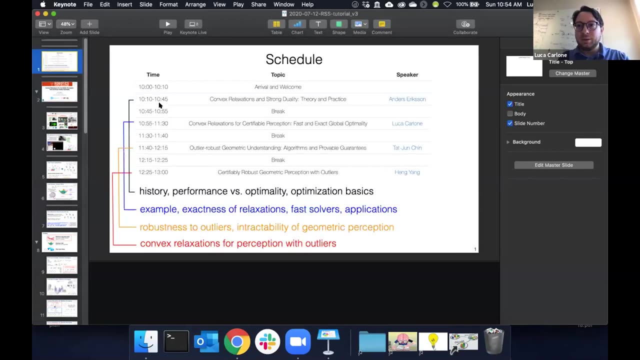 we cannot do that, But thank you so much for the talk. Yeah, Thanks for your time. Thanks for listening. I think it's pretty much time to start directly with the second talk. I will try like to stay, like you know. 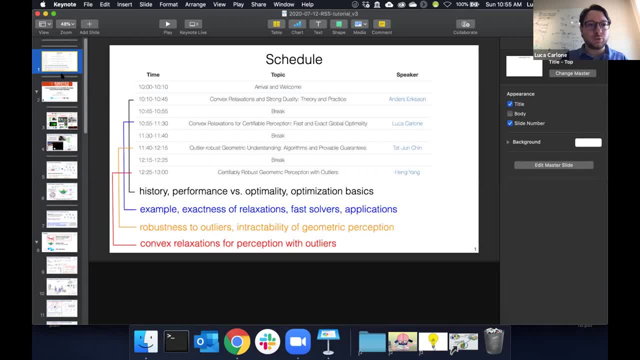 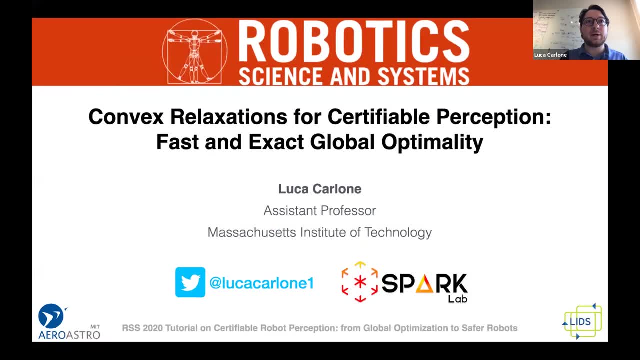 and to make sure that there is a break after this talk. The talk is supposed to be 35 minutes And let me start. Okay, So hi again, everyone, And, as I mentioned, I'm Luca Carlone, assistant professor at MIT. 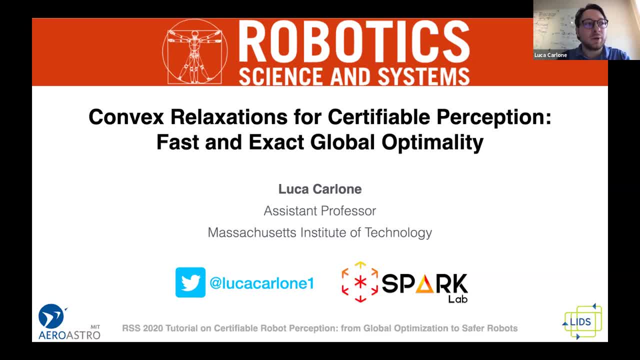 With this second presentation, I want to essentially leverage the basic notion that Anders gave us in the first talk and try to show how to apply this in practice. I will consider examples which are practical. They are robotics examples, so they are directly applicable to your research. 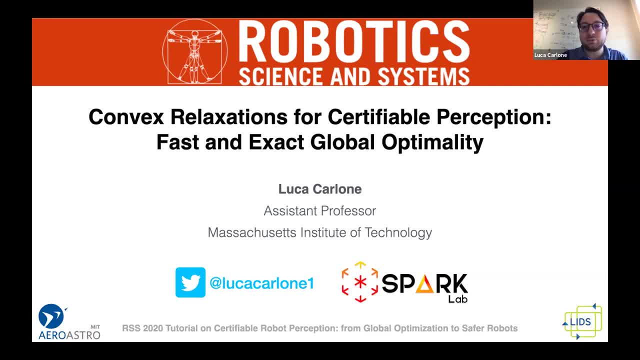 in SLAM and so on, But at the same time they're easy enough to just showcase how easy it is in some cases applying this notion of convex relaxation, duality and so on. So the goal of the presentation is to show that. 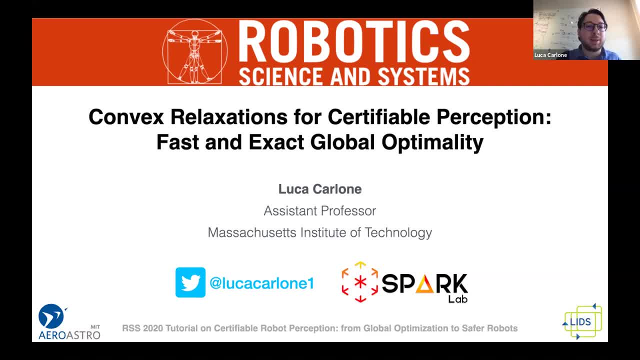 in many of these robotics problems- in particular, I'm going to talk about SLAM- these relaxation are exact. So, in the words of Anders, there is strong duality for these applications And, if you get lucky enough, you can also design very fast solvers. 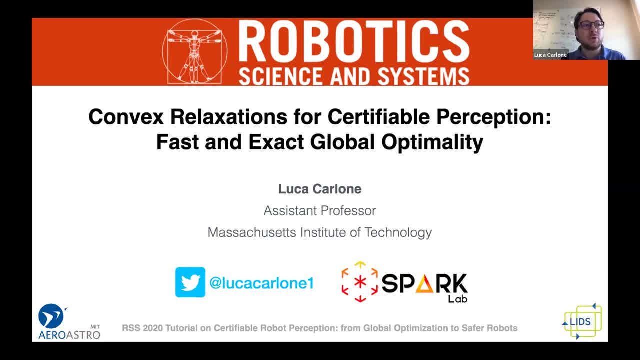 for these specific problems, And I will conclude with a few pointers to other applications which are still close to robotics and computer vision, in which the same is true Strong duality holds. Most of this presentation is about problems without outliers in which essentially, 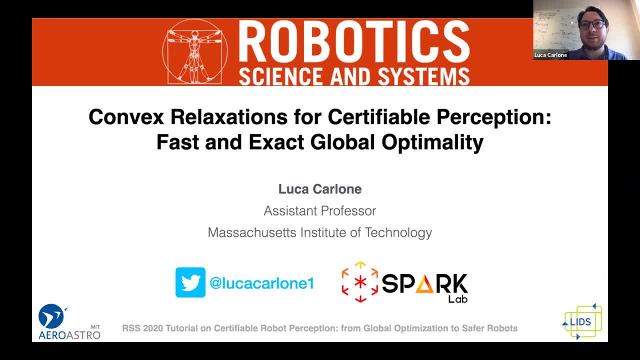 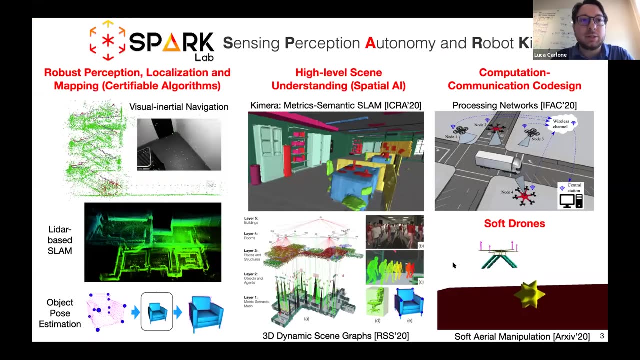 you have some least squares cost And I think the following presentation will focus on problems without outliers. So let me just say, like you know, I'm Luca Carlone. I'm the director of the Spark Lab. In my lab, in general, we are doing robotics research. 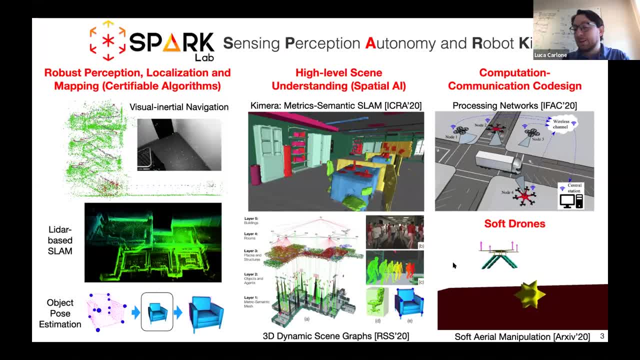 and we are particularly concerned about perception for robotics. This is one slide overview of the work we do before we enter in the details of, like you know, the topic of this talk. So in the past we have been working Okay. 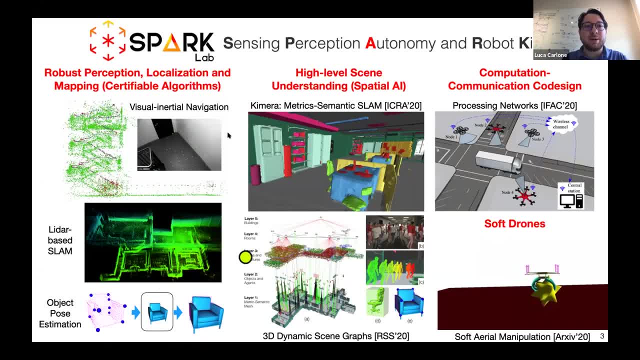 So we're working a lot on robust perception, localization and mapping and this idea of certifiable algorithms. You're going to hear a lot about these today in this tutorial. We are also concerned about problems which are a little bit farther, like you know. 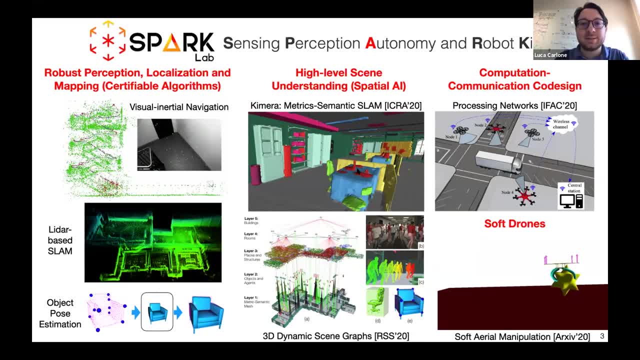 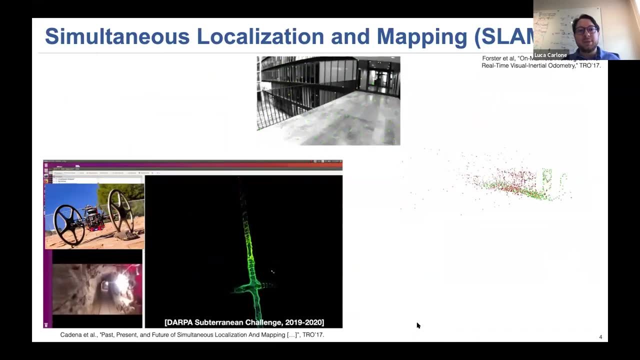 a little bit away from the topic of this tutorial, including high-level scene understanding and metric semantic reconstruction In other topics which are even, like you know, away from perception, including processing networks and drone manipulation. So the truth is that I started this investigation. 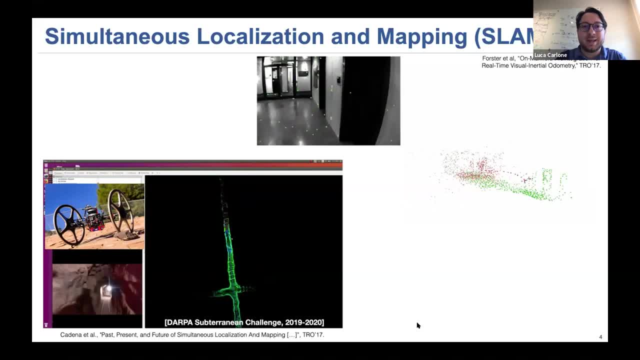 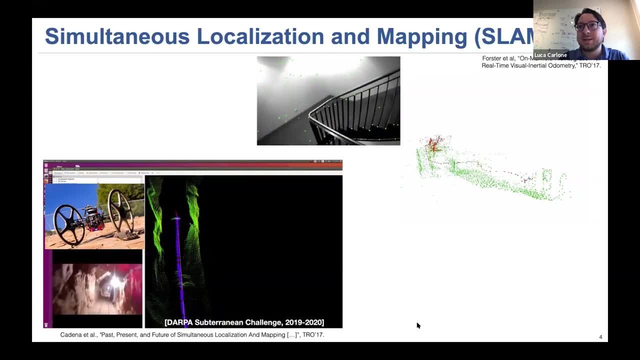 as a student and at the time I was working a lot on SLAM- simultaneous localization and mapping- And we're going to try to use for this talk. we're going to use SLAM as a running example to show how easy it is to use this idea of relaxations. 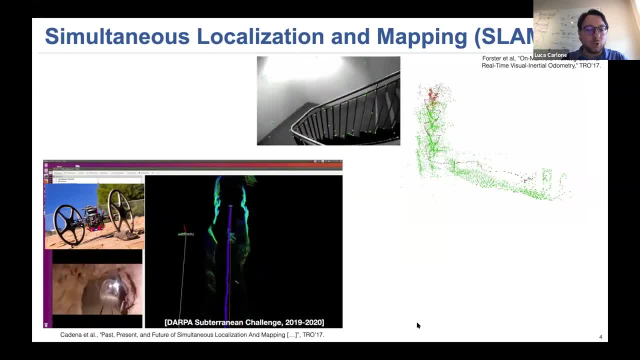 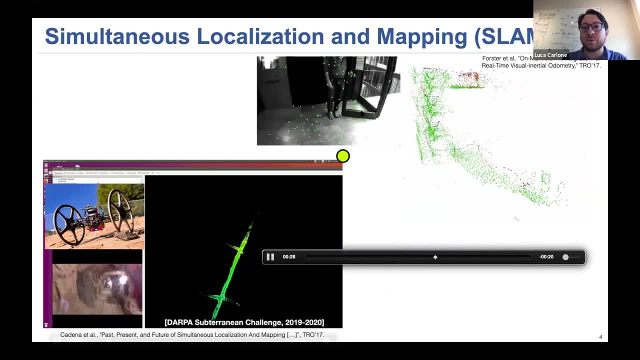 So these are some of the things that we're working on. So these are two examples of SLAM that we have worked on over the last few years. This is back 2017.. It's visual inertial navigation in which you're using information from cameras. 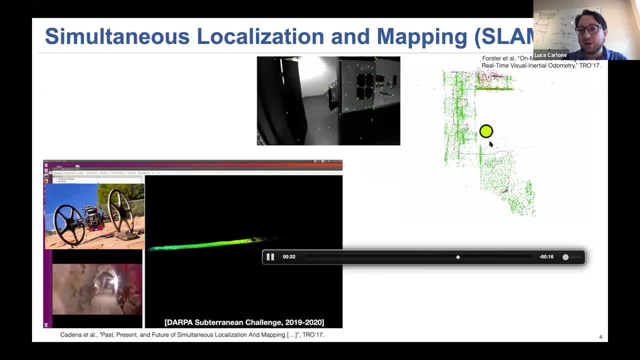 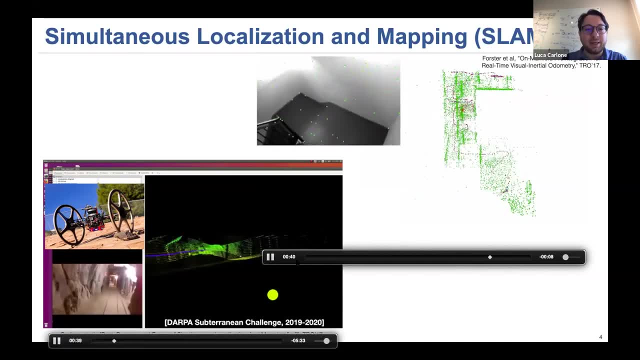 inertial sensor to build 3D reconstruction of the environment and an estimate of the trajectory of the robot that you see in red here, And this is a more recent example. This is about cave exploration. It's about LiDAR-based SLAM. 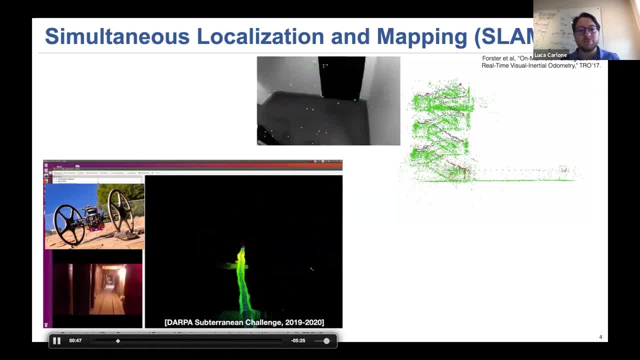 in the context of the DARPA Subterranean Challenge. So this is a project we're involved in right now. We just won the competition, the DARPA Subterranean Challenge, the second event of the competition, which was last February. But for the sake of this presentation, 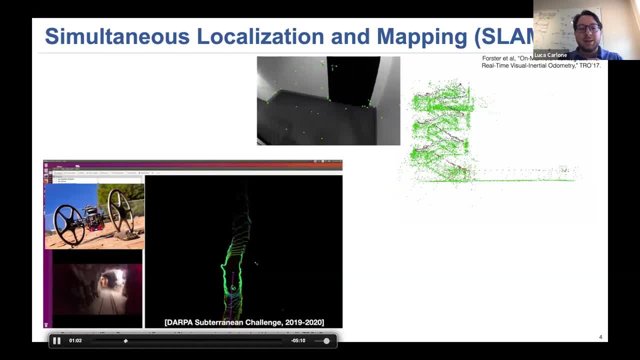 the message I want to give in this slide is that, despite the apparent complexity of these SLAM problems- that are complex sensor data, LiDAR cameras, inertial measurements- this message is that SLAM, at the very core, is solving an optimization problem. 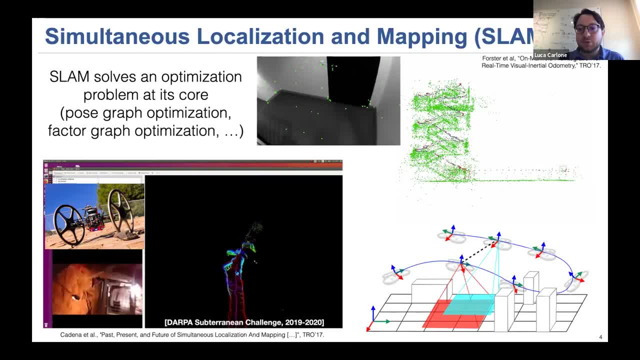 And this optimization problem in its most common form is about using sensor data to figure out the trajectory of the robot. So in SLAM, the robot is moving in a completely unknown environment And what you want to do is to process sensor data to figure out its own trajectory. 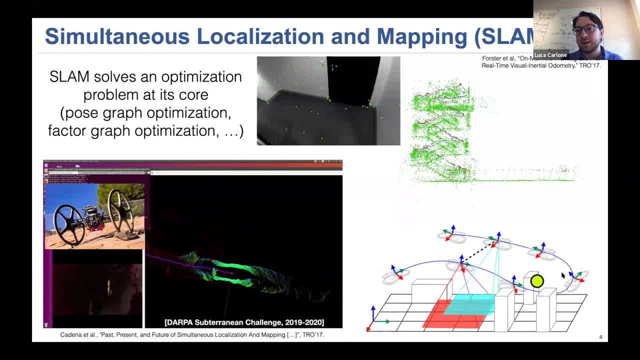 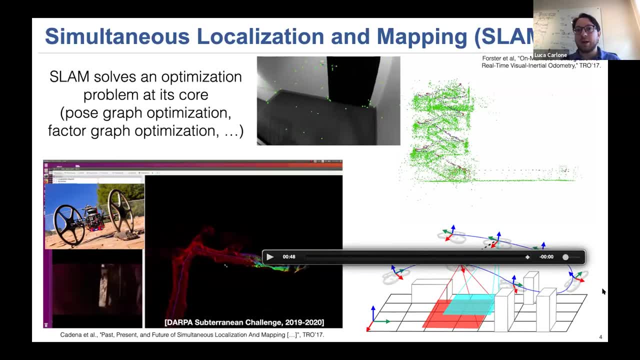 the trajectory from time zero to the current location of the robot And typically, after you figure out the trajectory, it's fairly easy to do a 3D reconstruction of the environment, which is the mapping part. So the optimization problem showing up in SLAM. 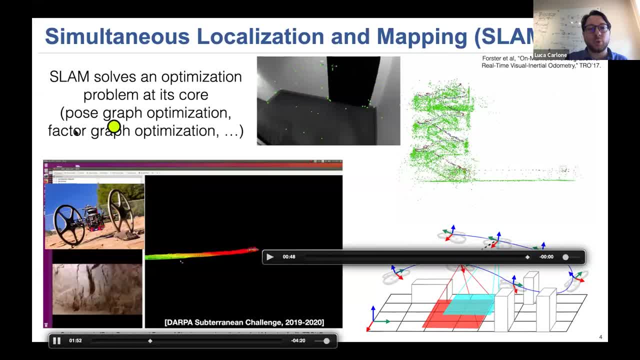 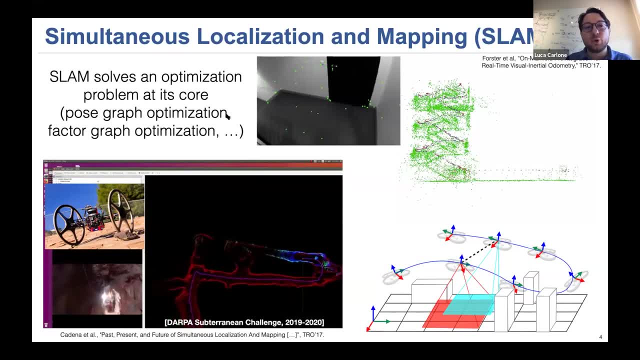 is typically called one of the most popular. which we're going to look at today is post-graph optimization. I'm going to tell you in the next slide what this is about, And in its more general form, it's called factor graph optimization. 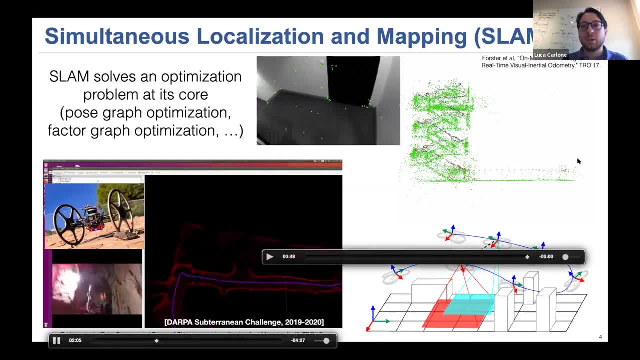 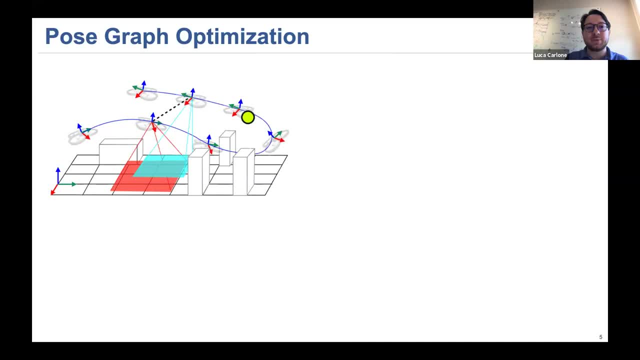 which is slightly more general. So what is post-graph optimization? Again, like you know, we want to in SLAM, we want to figure out the trajectory of the robot given sensor data, The basic idea behind modern SLAM system. 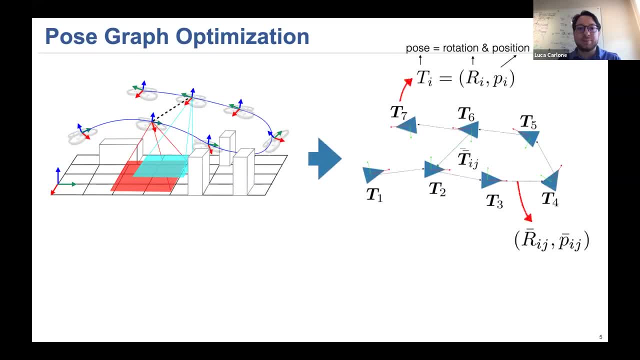 is to abstract away this problem into a simpler one or, like you know, abstract away the sensor measurements and move from the original problem of the robot model, the original problem of the robot moving in the unknown environment as a graph. okay, So here you want to estimate the trajectory of the robot. 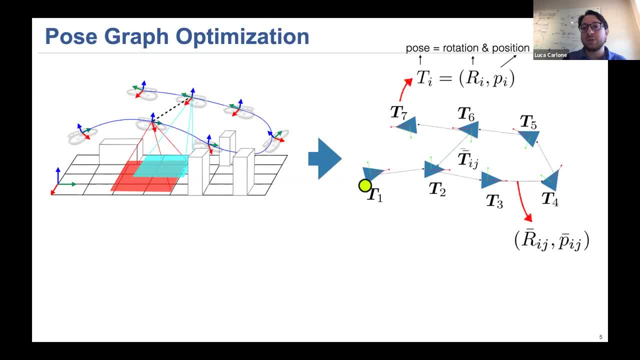 The basic idea is to model the trajectory as nodes in a graph. So T1 is the pose at time one, T2 is the pose at time two, and that's exactly what you want: to reconstruct the poses of the robot over time. 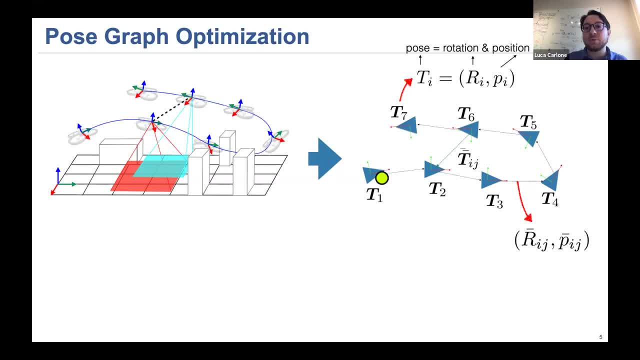 And in this graph the ages corresponds to measurements within two poses. okay, So there is, for example, an odometric measurement between pose T1 and T2, because we're able to measure the odometry between the two poses And, in general, it's true that every age in this graph 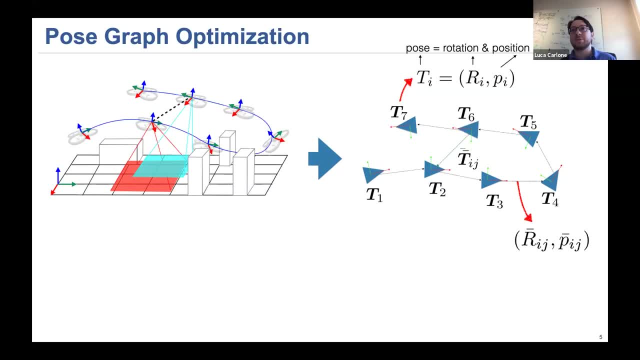 is obtained by some pre-processing of the sensor data. So there is something that's called the SLAM front-end which is going to pre-process the sensor data to create these ages in the graph. So on the mathematical side we abstracted away a very complicated problem. 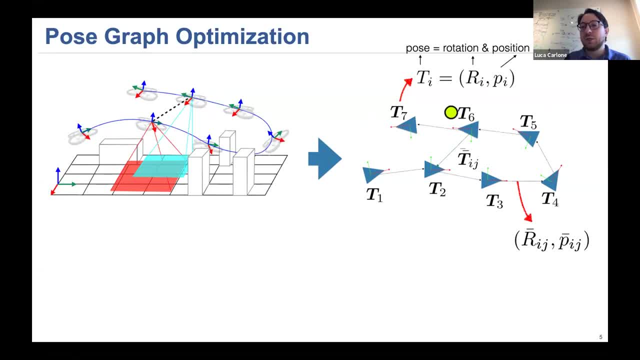 into a very nice and simple mathematical formulation in which essentially we want to estimate poses attached to nodes in a graph. So these are the T1,, T2, T3, and so on, And remember that each pose by definition is just a rotation array in a position pi. 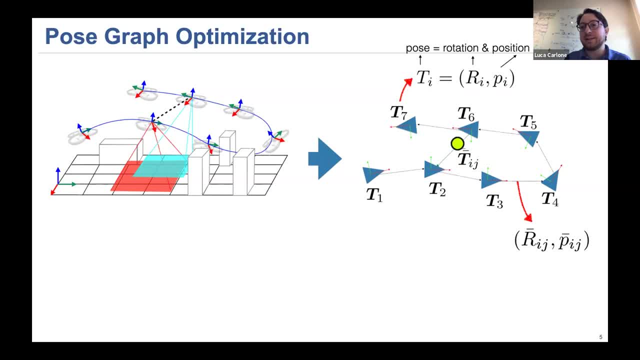 And what we are given to solve these poses are relative measurements attached to the ages of this graph. So we are given this Tij bar, which is a measurement of the relative pose between node i and j, in this case between node 6 and node 2.. 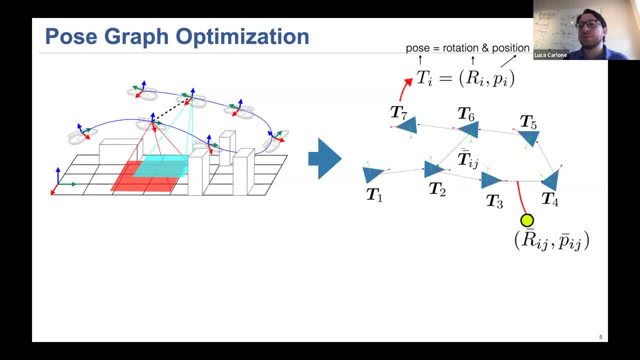 And these relative poses attached to each age are again relative poses. So there is a rotation component, Rij, and a position component, Tij. So geometrically, for example, for this age the measurement is a measurement of the pose of this guy, T4, with respect to the pose of T3. 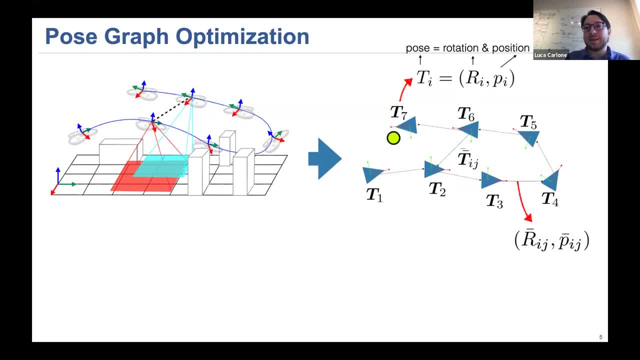 So this is what is called a pose graph, And there is actually a fairly established way to compute the poses attached to the nodes of this graph, which is indeed called pose graph. optimization, and not surprisingly for this tutorial is an optimization problem. So just to reassure you that you know. 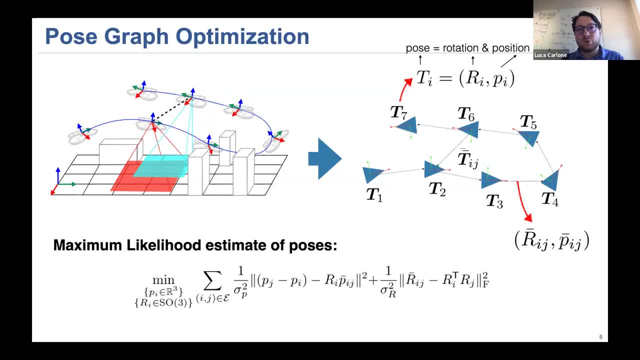 this is a fairly popular tool. this is what you will find at some point in the backend of orb-SLAM. This is what you will find in the backend of direct methods for SLAM, like optimizing the entire pose graph after you do loop closures. 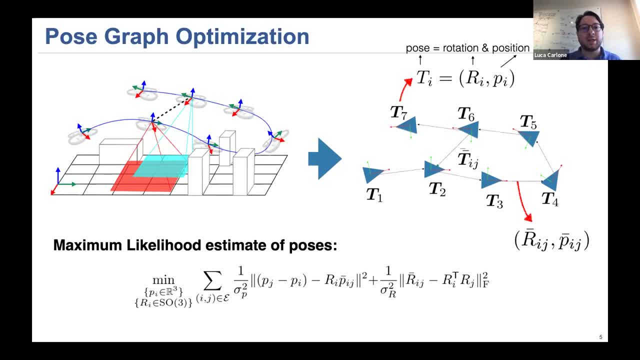 And this is implemented in very popular libraries, including G2O, GTSAM and so on. So what is this optimization problem? This optimization problem is a bit looks, a little bit complicated, so I will tell you all the details about it. 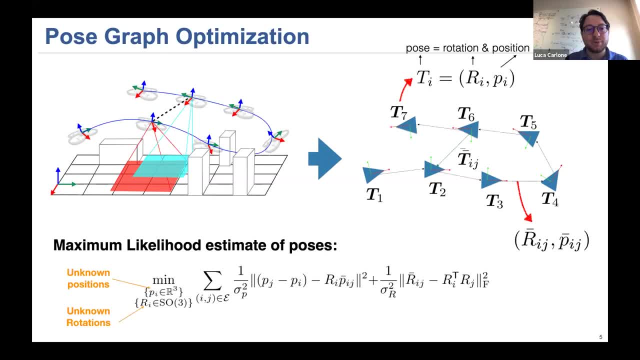 But essentially what you are trying to do in this optimization problem is to try to figure out the unknown position and the unknown rotations of the robot, And remember that we have many of those, So we have one for each node in the graph. So we are sampling these poses along the trajectory. 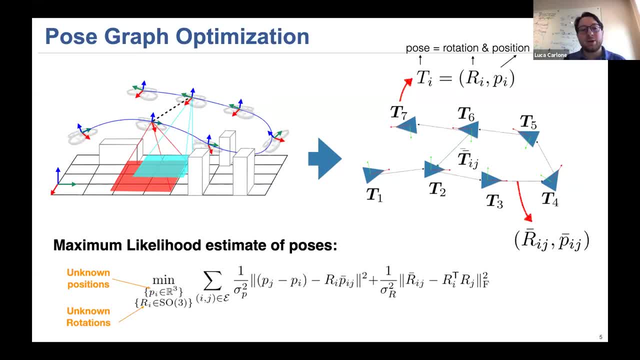 of the robot And we are computing this position and rotation in a way that minimizes this cost. And the cost function at the high level is just penalizing the mismatch within the pose estimates of the corresponding measurements. So this is particularly easy to see. 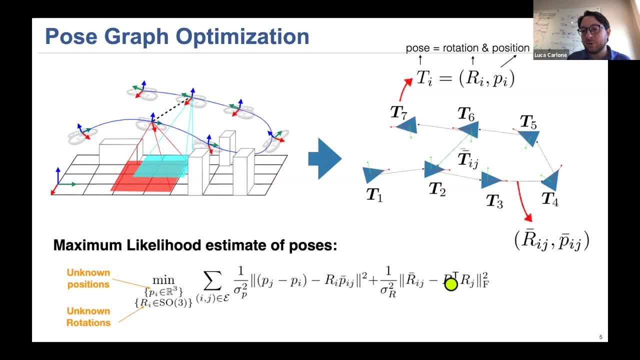 in the second term here. So you can see that you are trying to find the rotation at node i and j such that the relative rotation between i and j is as close as possible to the measurement r, i, j, bar And there is some norm. 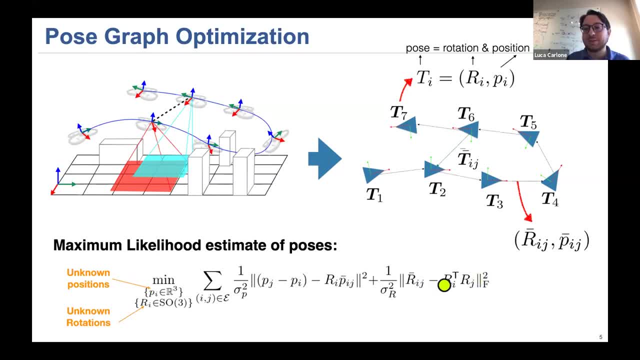 which is the Frobenius norm, which is essentially, like you know, just measuring the distance between these two rotations, And there is potentially, if you want, you can set this to one, but in general there is a weighting term. 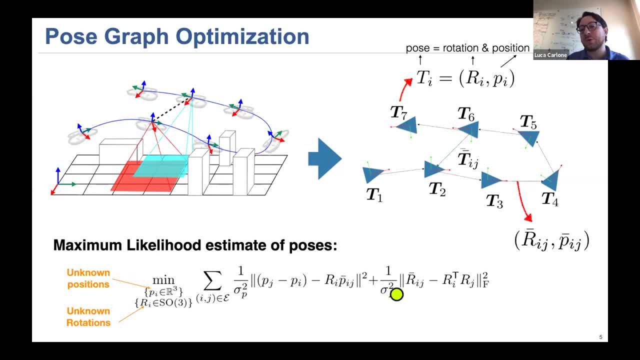 It's just a known weight which is measuring how certain you are about this measurement. So the sigma will be large if your measurement has a lot of noise. The sigma will be small if your measurement is very accurate And the first part is doing kind of the same. 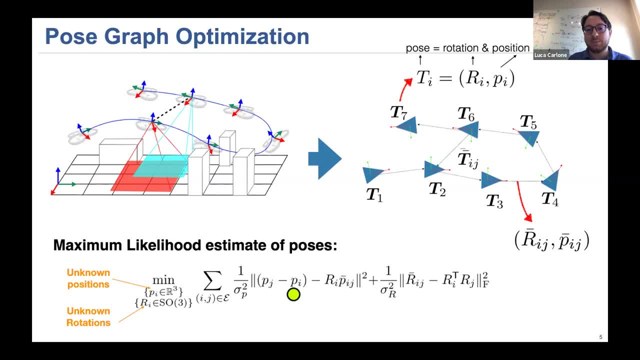 for the position part. You are trying to figure out positions p i and p j such that you match as well as possible the measure relative position p i j. Since the relative position p i j is in a local reference frame, you have to rotate it by r? i. 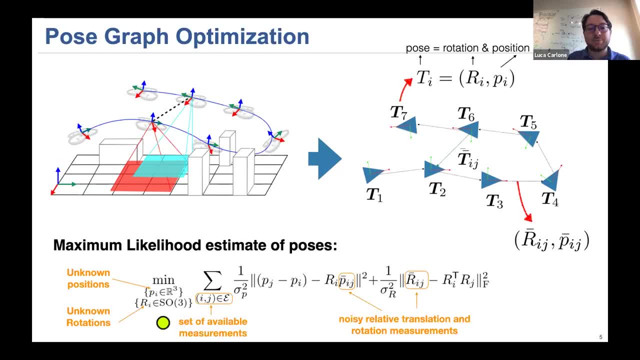 And you have a bunch of measurements, one for each edge in the graph. So you have potentially a large set of measurements. And again, the quantities with the bar are the measurements attached to the edges in this graph. So I started when I was even a student. 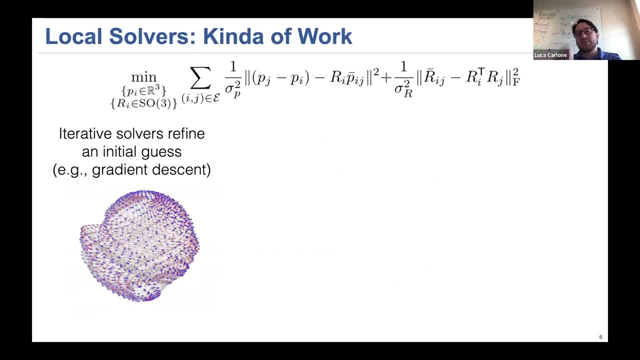 I started looking at these problems and I was kind of frustrated because the state of the art was about using local solvers And the basic idea of local solvers is that they kind of worked in the sense that you know they got, you were able to get like decent performance. 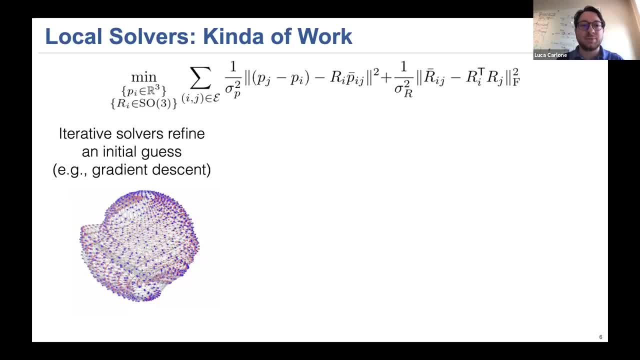 but not the robustness that you really wanted from this kind of systems. Local solver is about as Anders was saying. it was about starting from an initial guess and going downhill. You can think about an iterative solver being some sort of gradient descent. 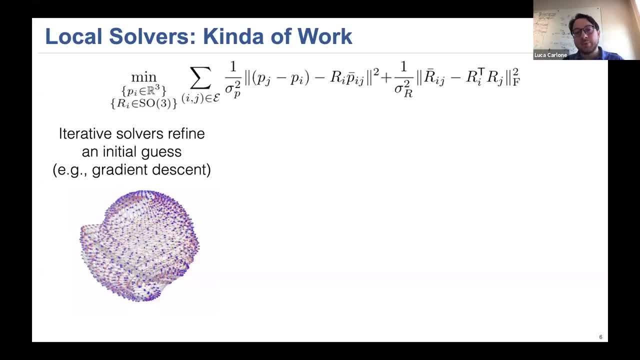 which is starting from an initial guess and trying to go downhill in the cost function. The video here is an example of a gradient descent applied to a postgraph optimization problem in which the poses are sampled along a sphere. You can see that we start from an initial guess. 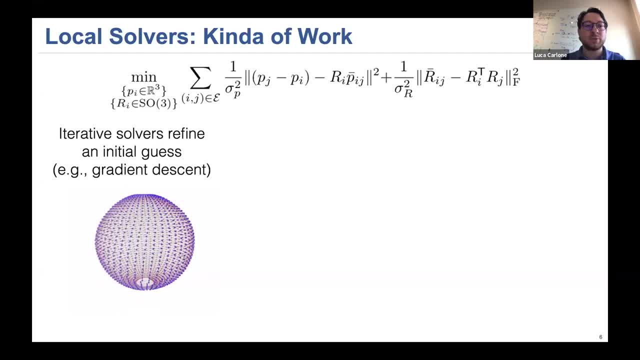 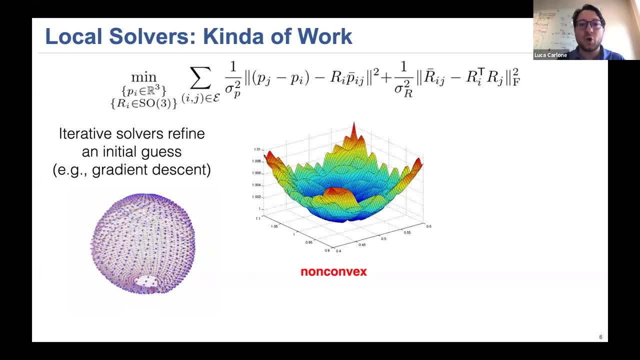 Hopefully we converge. we converge to a good solution. In this case, we converge to a nice solution. The issue with the postgraph optimization is that, again, this is a non-convex problem. So if you initialize this local solver close to the global minimum. 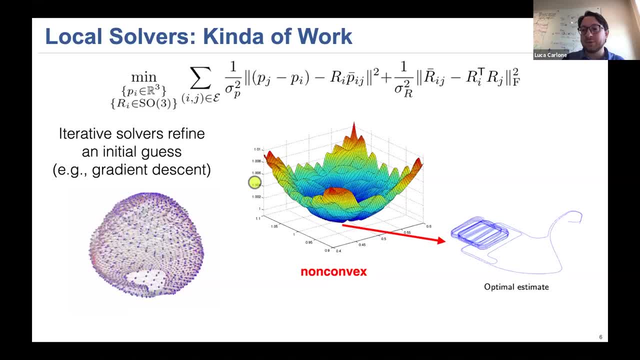 you get a very nice estimate. In this case you get a nice reconstruction of the trajectory of a robot moving in a parking lot. But if you initialize your local methods with a bad initial guess, you get a suboptimal estimate which typically corresponds. 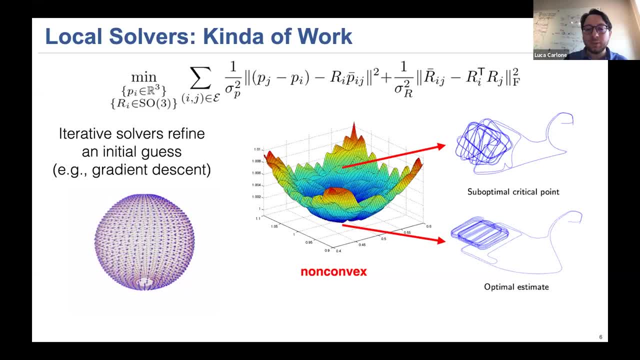 to a very wrong trajectory. reconstruction- So, in other words, the issues that iterative solvers are brittle, might convert to bad solution if the initial guess is not accurate. One thing that is worth mentioning is that in many of the problems that we are going to discuss, 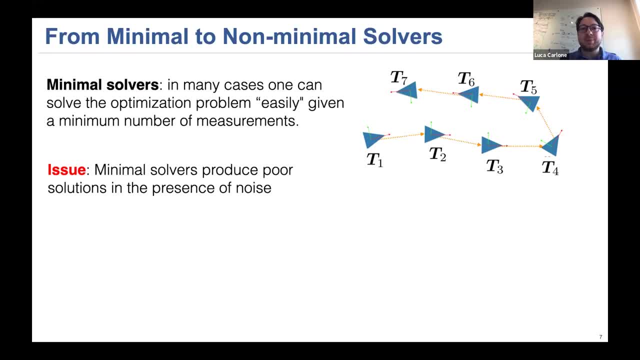 including SLAM, it's possible to design a minimal solver. So a minimal solver is a solver which is taking just a subset of the measurements and is trying to estimate the quantities you care about, in this case the poses, starting just from this subset of measurements. 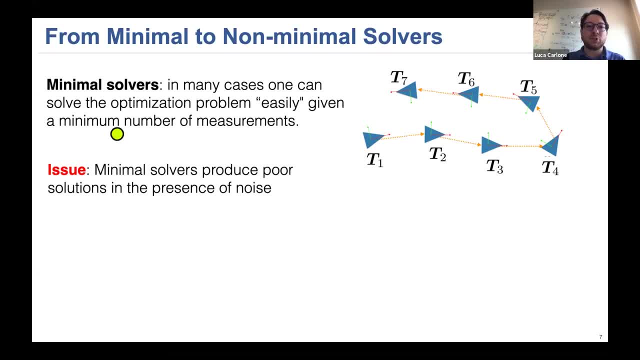 So here I'm saying that in many cases, one can solve the optimization problem easily given a minimum number of measurements, And that is definitely true for SLAM. So if, instead of considering all the edges in the graph, I just consider a path, 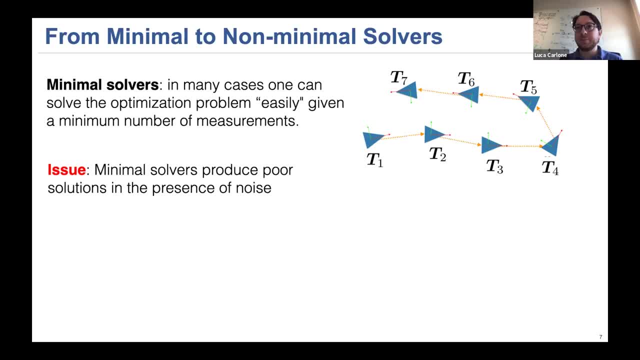 as in this case, or I consider a spanning tree. it's trivial to consider, So I can compute the poses, I can just chain the measurements and I can obtain an estimate of the poses. But the issue with this approach, which is actually indeed very popular, 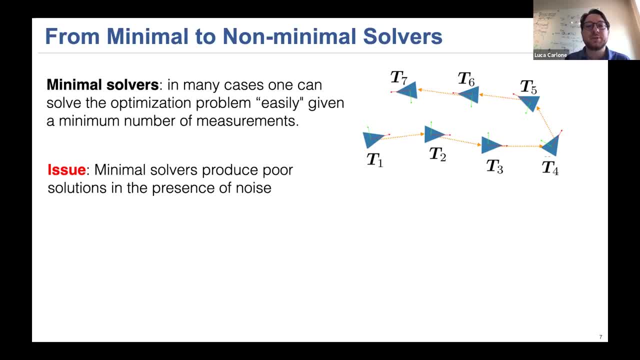 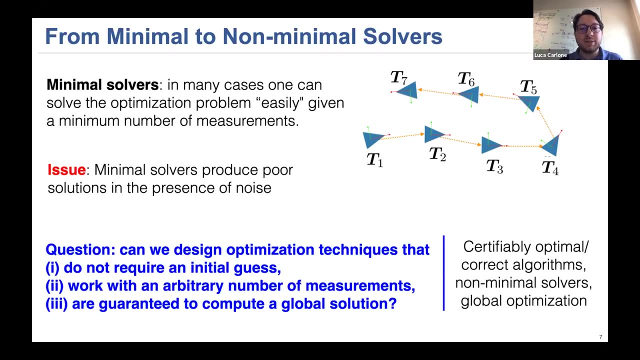 in computer vision is that these kind of minimal solvers produce poor solutions in the presence of noise, because indeed they are neglecting most of the measurements. So the topic of this tutorial really is about addressing a fundamental question, which is: can we design optimization techniques? 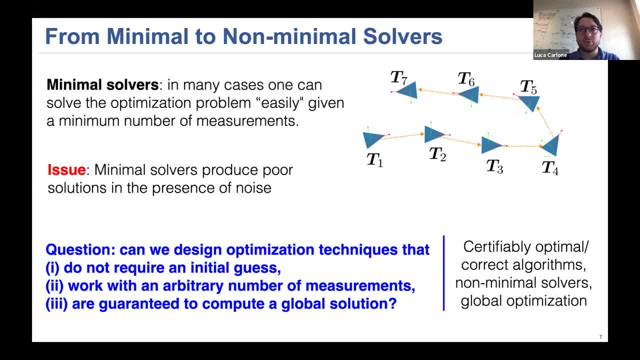 that, first of all, do not require initial guess, which is a source of brittleness. Second, that work with an arbitrary number of measurements. We don't want to use a subset of the measurements, We want to use all of them. 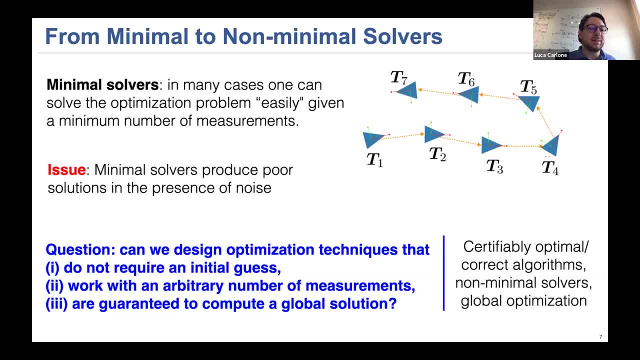 And third, we want to design a technique that is guaranteed to compute a global solution. So the answer to this, of course, is yes, we can do this, And the result is what we call what have been called, in general, certifiable algorithms. 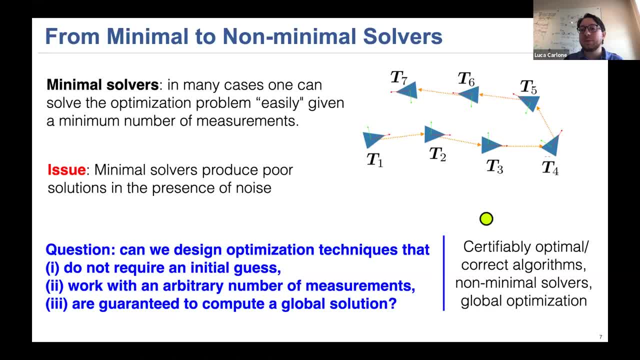 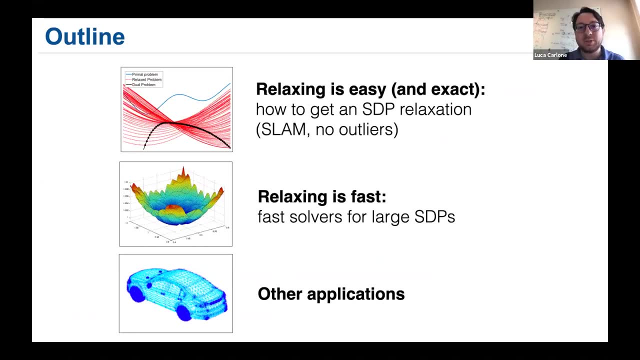 certifiably optimal, certifiably correct algorithms in computer vision that are also called non-minimal solvers, And the basic idea is essentially algorithms that are performing global optimization. So I want to give you an example of a certifiable algorithm in this presentation. 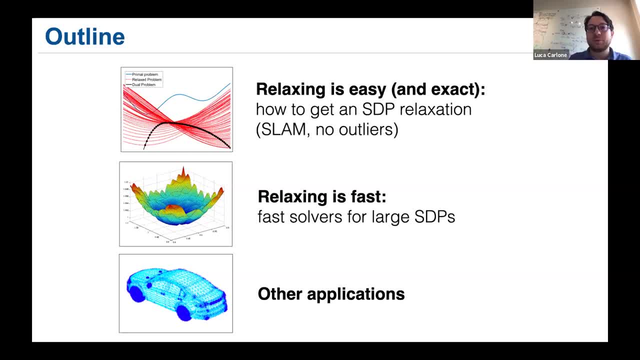 And I will spend some time- actually most of the presentation- on the first part, which is about telling you that getting a relaxation in many problems is actually easy, And I will show how to get an SDP relaxation, a semi-definite relaxation for SLAM. 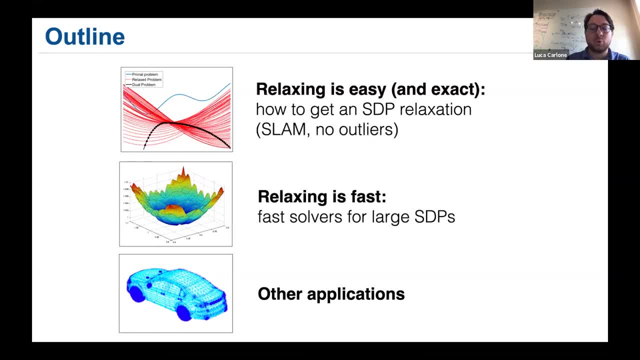 for the case without outliers And following talks. I'm going to focus on the case without outliers. I'm going to touch on the fact that, if you get lucky, relaxing, solving a relaxation can be indeed fast to solve. Okay, And I will have two or three slides. 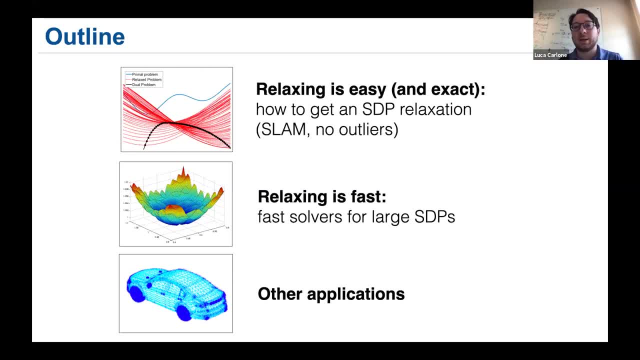 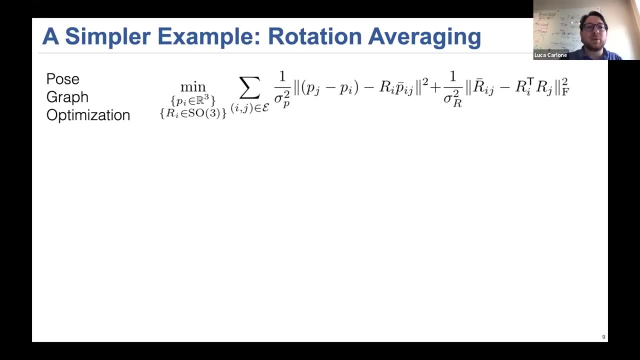 with the extra application which you can replicate the same derivation to get relaxation for other problems. So I started relaxation with. relaxing is easy, Okay, So I'm going to start looking at post-graph optimization, but actually we started a problem which is slightly easier. 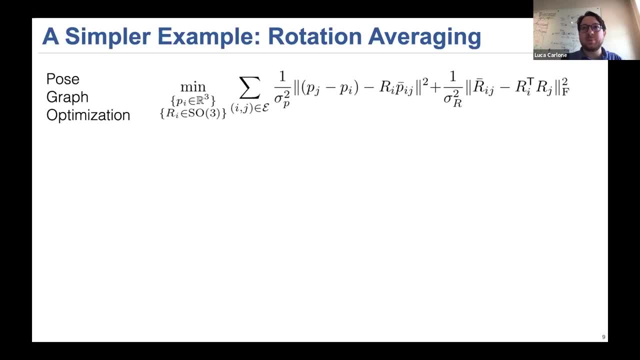 than post-graph optimization. I will show you that by simplifying the problem a little bit. I will go back to post-graph optimization Later on. I will show you that you don't miss anything. Okay, So we started a simple problem which I will show. eventually is the same. 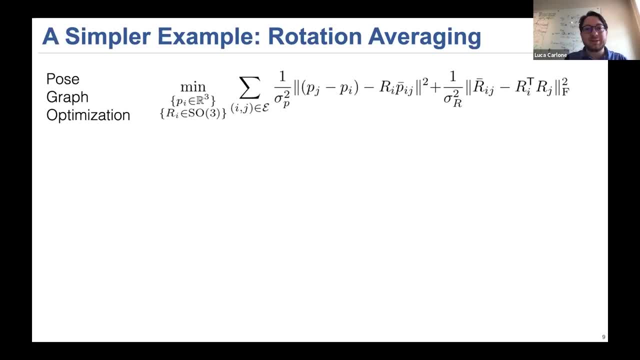 as solving post-graph optimization. So what I want to do is that, instead of solving these- which is a little bit scary if you look at it- I want to solve just the second part of it. So I want to solve just the rotation part. 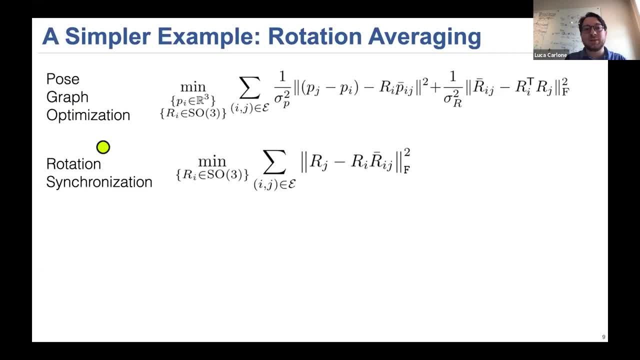 So I'm moving from post-graph optimization to something that is called rotation synchronization. So these two problems are the same, except I gave up on the first part and I gave up on solving for the positions PI. So I'm just solving for the rotations. 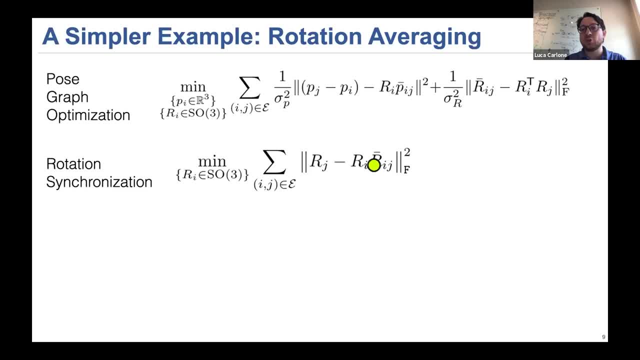 in a way that is minimizing the mismatch with respect to the rotation measurements. Rij bar- And again I will go back to the fact that rotation synchronization is generally enough later on will allow us to solve even post-graph optimization. So this is kind of nice and simple right. 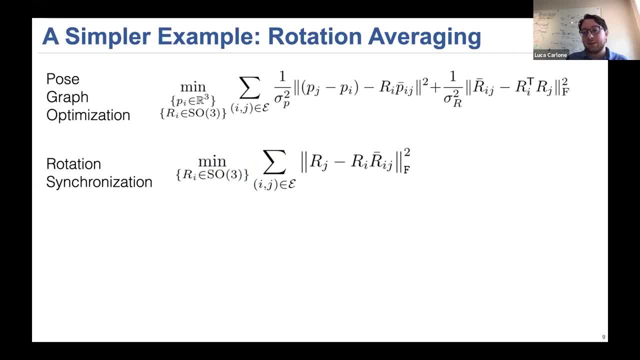 There is a quadratic cost function. There is some constraint here. We can manipulate these a little bit to make it even more elegant. So we can realize that I can rewrite this term Rj minus Ri, Rij bar as the product of two matrices. 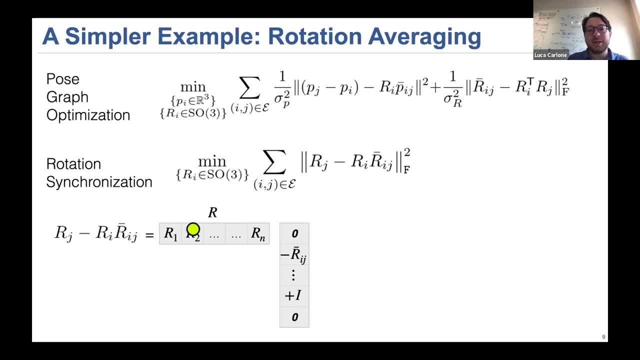 So one which is the R, in which I'm stacking all the unknown rotations I have in my problem. So this is 3 by 3n And I just multiply with a known matrix which is just including the measurements and some identity. 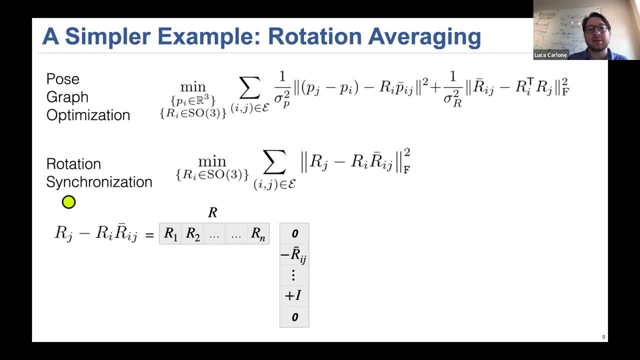 And just by multiplying these two you can see that you can get exactly this term. So if we can write each one of these terms as a product of a rotation by a constant matrix, it shouldn't be surprising that if you massage a mat a little bit. 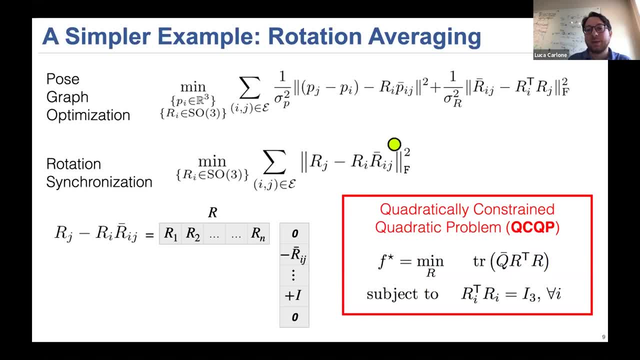 we can reformulate exactly this optimization problem as a problem with a quadratic objective. Okay, so everything is function of R, which is this stacking of rotational matrices. We can reformulate rotation synchronization as a problem with a quadratic objective in quadratic equality constraints. 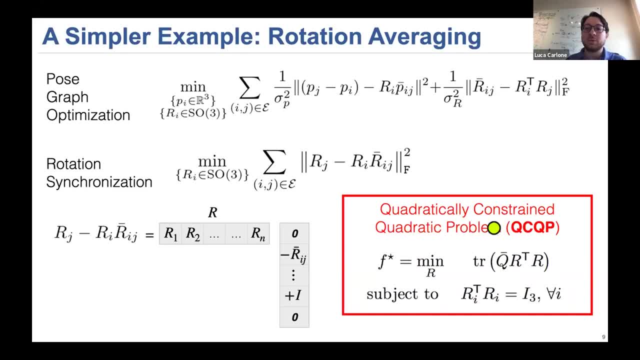 which is what Enders called the QCQP, a quadratically constrained, quadratic program. So again, the objective here is just applying this trick to each term in the sum and you get the quadratic term. And there is also a constraint. And on the constraint, 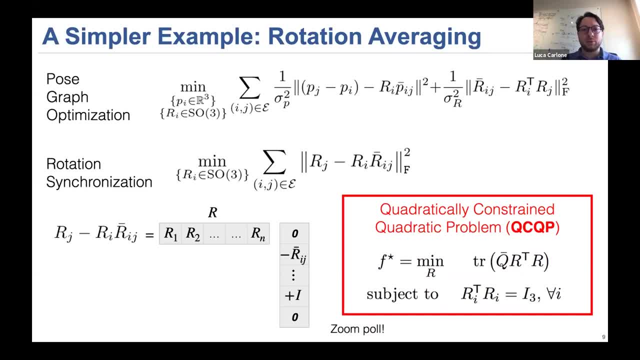 to make sure that you guys are still there. I want to just try real quick if I can poll you guys about. you know what you think about essentially where the constraints are coming from, So at this point you should see a poll in front of you. 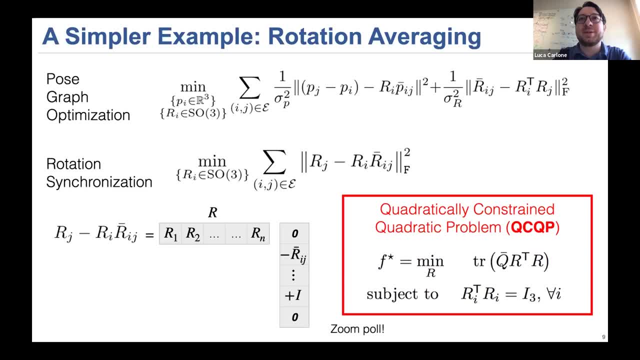 And I'm going to call on Anders Heng to confirm that they're seeing the poll And I will ask you guys to take a look at the poll and try to reply. The poll is essentially asking: where do the constraints in this optimization problem come from? 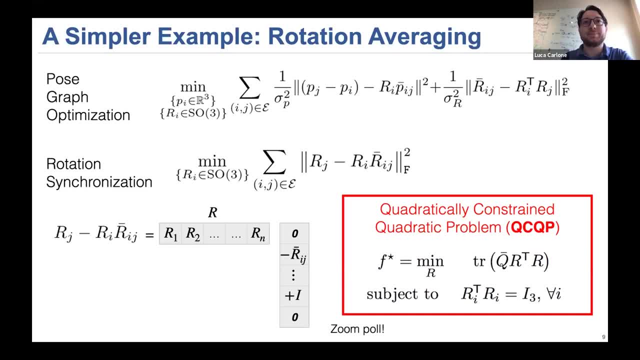 And I will give you a few seconds to answer that. We have a few votes coming in, All right, You guys are still there. That's good to see, All right, So let's give maybe 10 more seconds, Okay, And again. 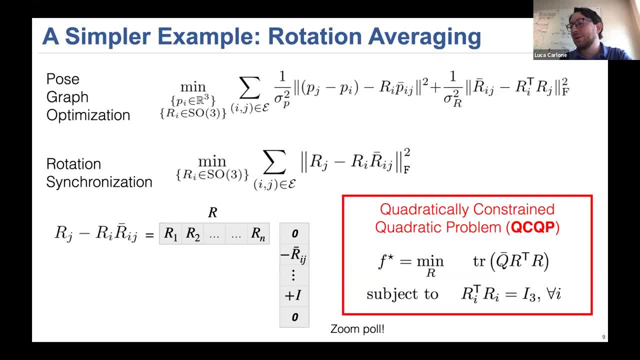 if you're not sure, just answer. not sure is still a good bit of information. Excuse me, How do we access the poll? You should see it just on your screen And I see responses. So many of you are seeing the poll. 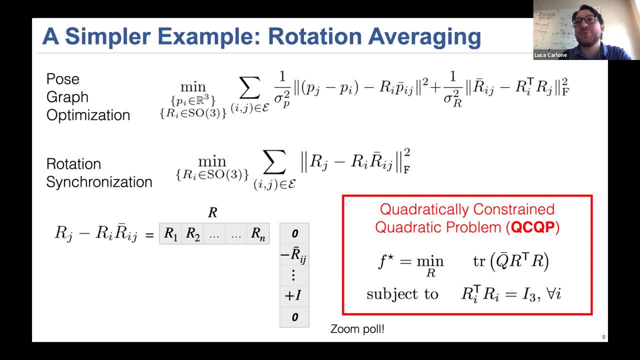 Unfortunately, if you don't see it, it's probably glitching Zoom, So don't worry about it at this point. I think the problem is if they're using the embedded Zoom client, then they won't see the poll. Okay, So I guess that the people I see here 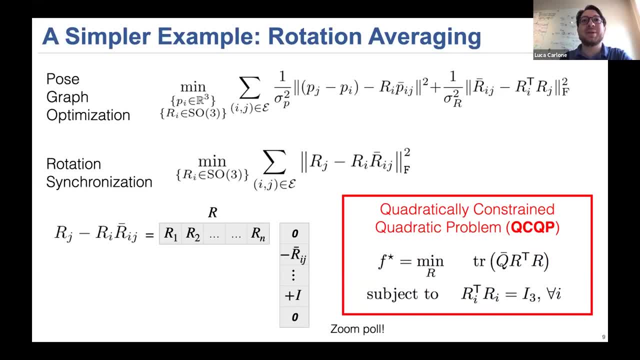 are just opening Zoom on their side. Okay, let me end it. I think it's still a good exercise. I can read you the answer. The question is: where do the constraint array, transpose array equal to the identity come from? And sorry, 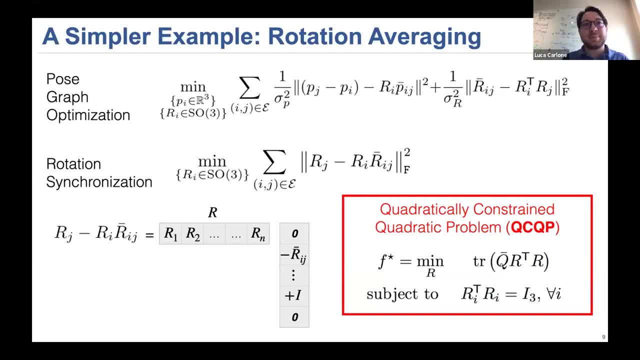 And there are different questions here, but essentially the basic answer that most of the people replying got correctly is that essentially here we're starting with a problem which seems unconstrained, but actually there is a constraint hidden here, So we are not looking. 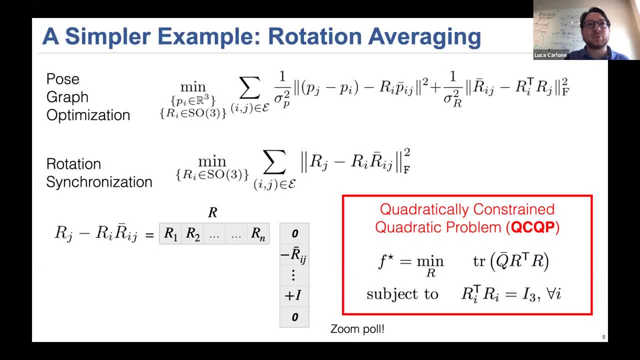 for any metrics array. Let me stop sharing the poll, All right, Okay, So back to the slides. Okay, So the basic idea is that in this optimization problem we do have a constraint, which is the rotation matrix. is a member of SO3,. 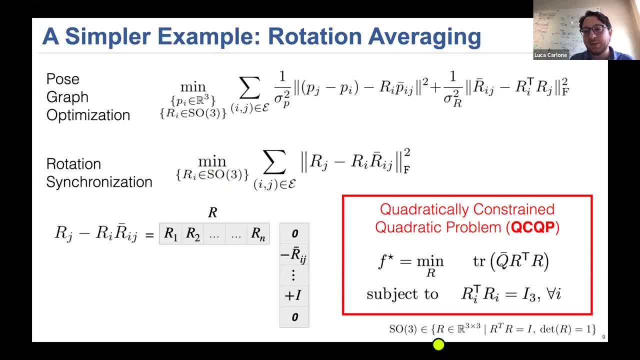 which is the set of 3D rotations, And the set SO3 is defined as the matrices which are three by three, which are orthogonal, So satisfy r, transpose r equal to the identity and have determinant plus one. So this is exactly where. 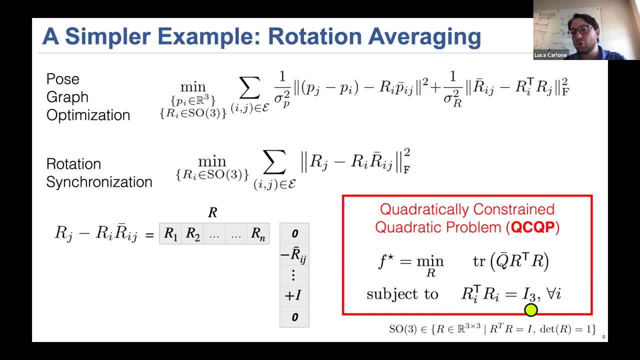 the constraint here comes from. I'm just enforcing each rotation to be orthogonal, which is each rotation should be, like you know, a rotation, And something that is important, obviously, is that I'm dropping the determinant constraint. There is a way to model. 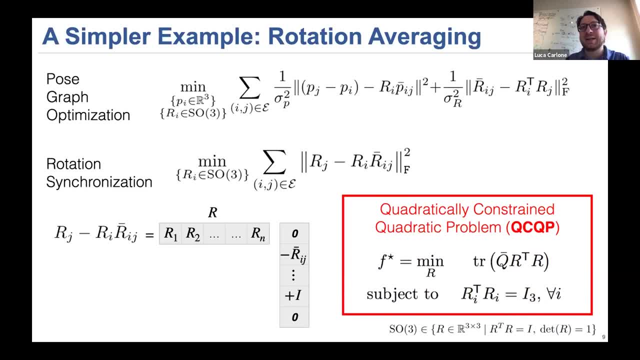 the determinant constraint within the relaxation Doesn't help, Like you know. it doesn't change much in the relaxation and it's just a little bit more complicated. So we're going to forget about it and actually don't lose anything in performance. 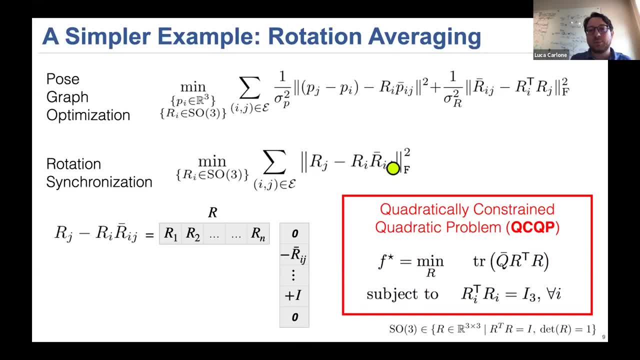 So in this slide what I'm saying is that we're going to consider rotation synchronization as a proxy for SLAM. Rotation synchronization can be written as a very nice and simple problem in which you have a quadratic constraint, The cube bar. here is a known matrix. 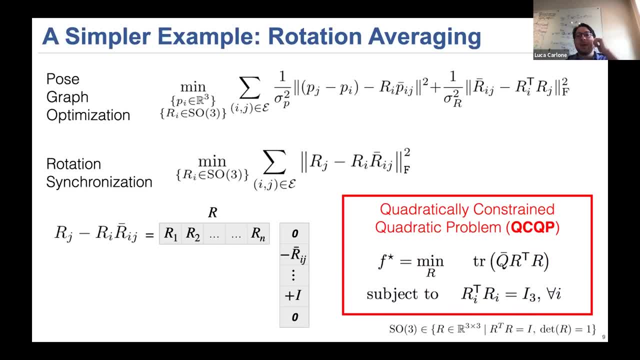 And you have these quadratic equality constraints And understanding already mentioned that this is a non-convex problem. Okay, So the quadratic cost is fine, This is convex, But the constraints are non-convex, because quadratic equality constraints are non-convex. 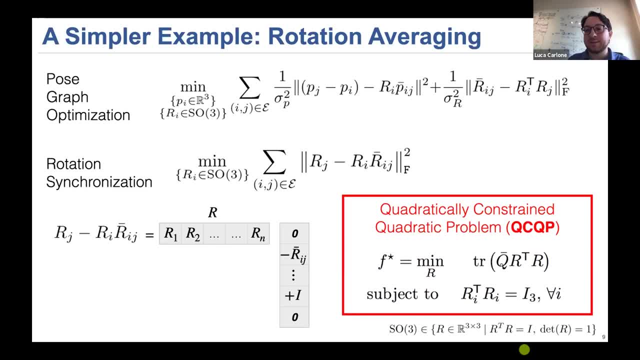 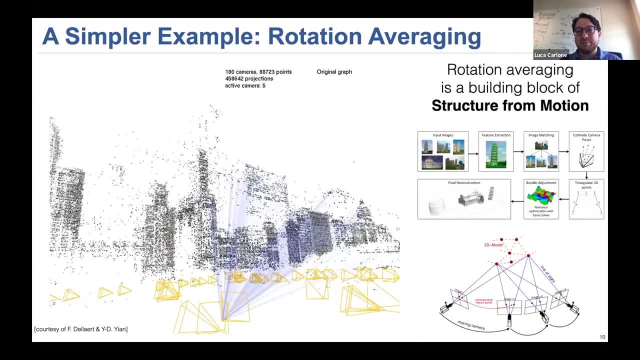 So a lot will be of this presentation about how to relax this problem. formulation: Quick slide to show that rotation, So rotation synchronization, is actually not the toy example. Indeed, rotation synchronization, which is also called rotation averaging, is a building block of structure from motion. 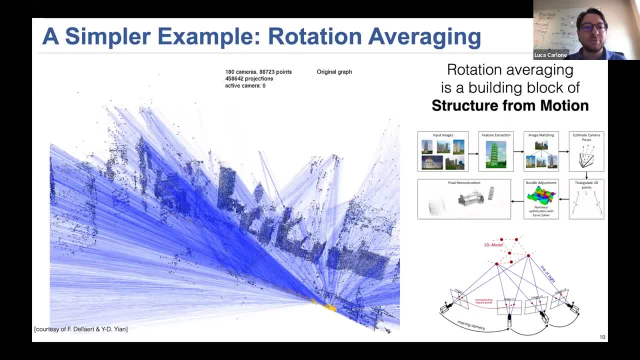 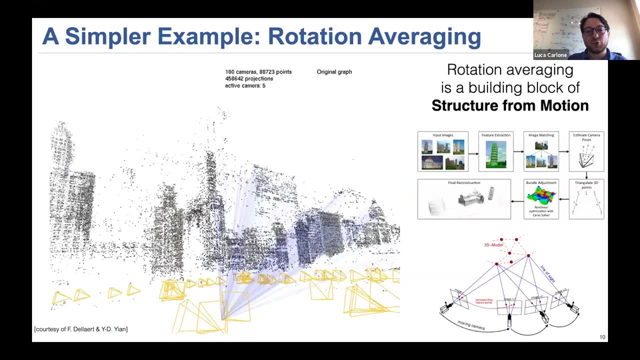 in computer vision. It is actually a very important problem. There will be papers in computer vision looking at rotation synchronization And this is a paper in robotics doing essentially structure from motion and estimating in the process, estimating the rotation of the cameras through rotation synchronization. 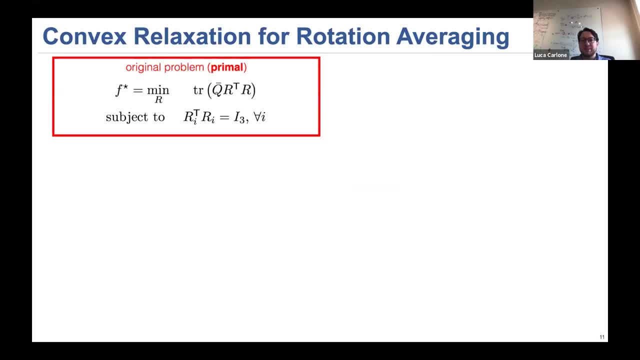 Okay, So let's get on how to do the convex relaxation for rotation synchronization. Again, it's called also rotation averaging And you're going to see that in these slides. actually in two steps I'm going to get the convex relaxation. 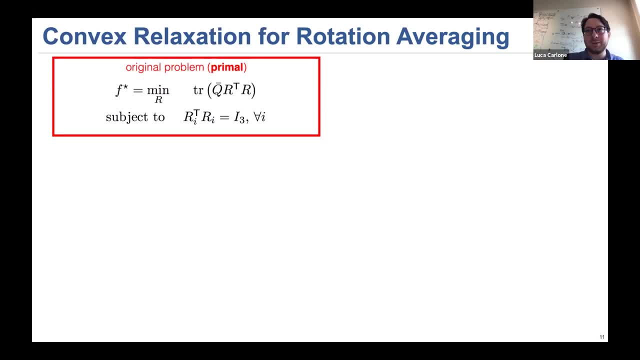 which is much, much easier than using Lagrangian duality. And then I will show that using Lagrangian duality pretty much is the same. Okay, So we start with a heuristic way to design the relaxation, And then we're going. 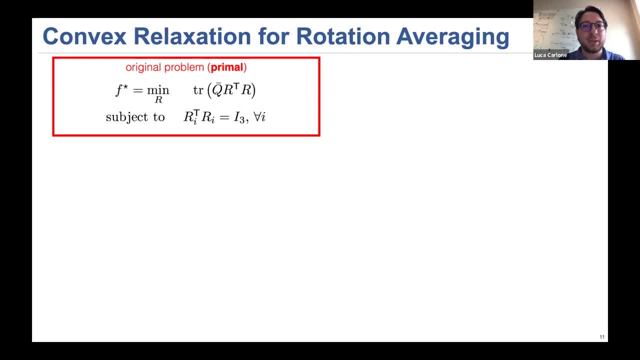 to do the formal way using Lagrangian duality. So this is the original problem that we want to solve. Again, this is called the primal problem And we said that this is non-convex So it's hard to solve. 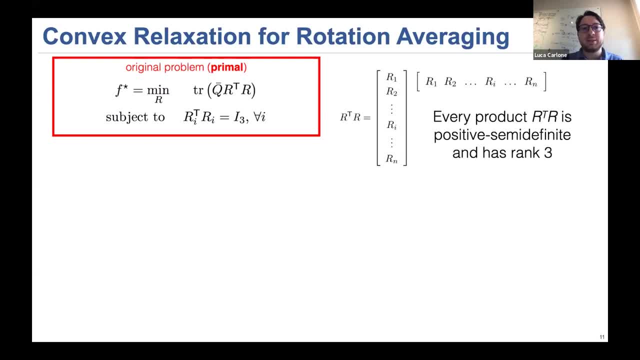 The basic insight of this problem is that this problem, if you stare at it, you know the r, which is the variable, shows up only in the form r transpose r. And if you look at the shape of these matrices, r transpose r. 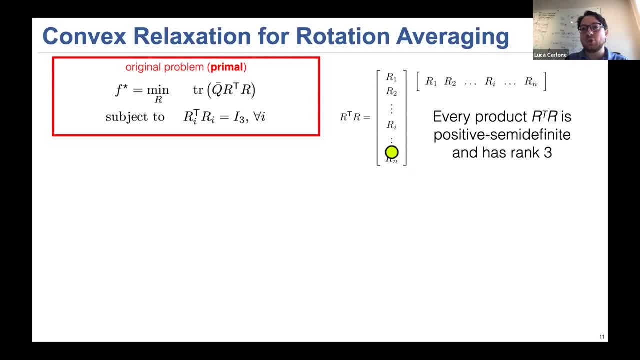 you know, will have this shape in which the rotation matrix is multiplied by itself. I think these- there are a bunch of transposes missing Here, but I think that's fine- And the basic observation is that r, transpose r is a square matrix. 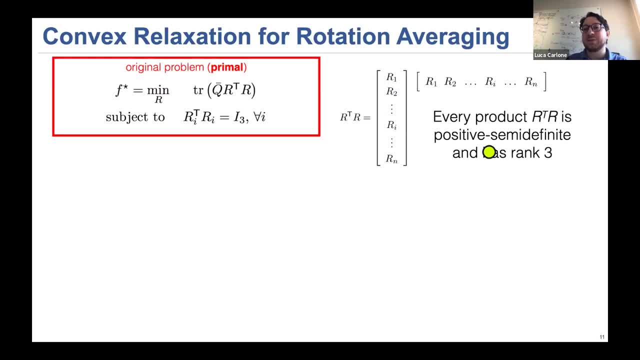 Okay, After you do this multiplication, you get a square matrix. Moreover, being a multiplication of a matrix by itself will be positive, Semi-definite will have all the eigenvalues larger or equal than zero, And also we'll have rank three, just because. 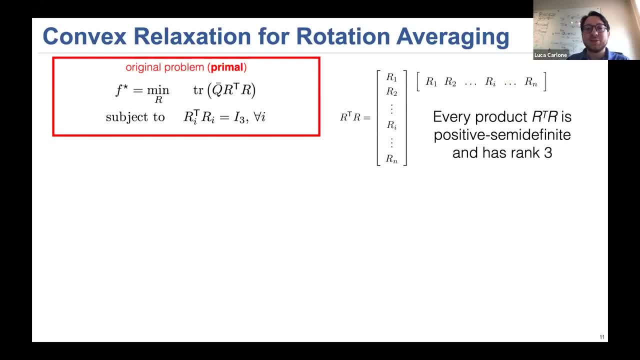 it's the product of three by three n matrices. So the basic idea, very easy way to get the convex, is to see why don't we replace r, transpose r, with a square matrix. So let's call this square matrix z. So if we replace 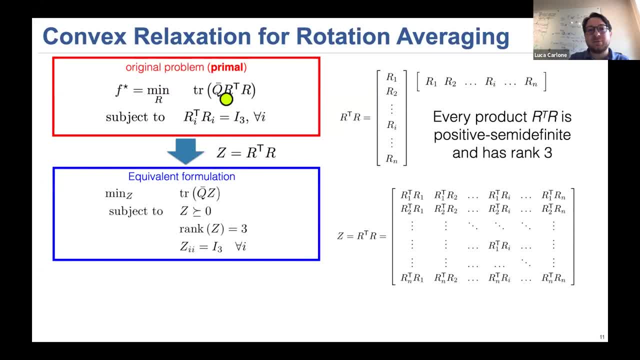 r transpose r. with this square matrix, the objective becomes, like you know, essentially a linear objective in z. At the same time, we have to enforce the fact that z is equal to this, which we said is the same as enforcing that z is positive. 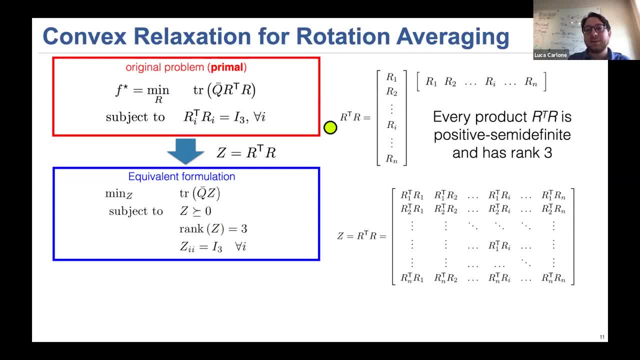 semi-definite and the rank of z is equal to three. And if you stare enough at the structure here, you'll realize that r transpose r are essentially on the diagonal of the z. So to enforce the same constraint here, r transpose r, equal to the identity. 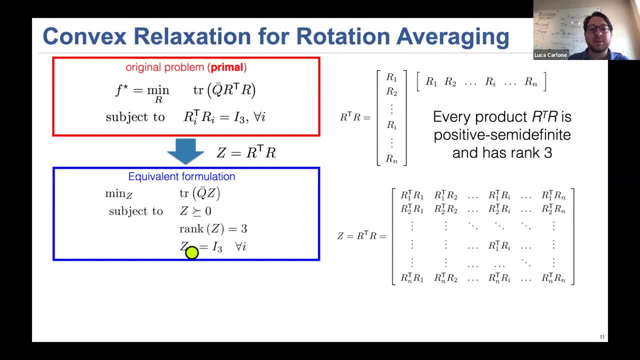 you just have to force that the diagonals of the z matrix is equal to the identity matrix. So you see that here we're just changing variables, right, You're moving from r, transpose r to a z formulation. but these two we said 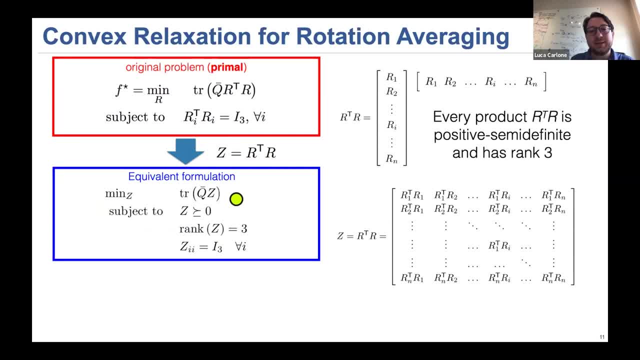 they are exactly the same right. And the nice thing here is that we isolated the non-convex of the problem because we got an objective function which is linear. that's definitely convex. This is a semi-definite constraint which is convex. 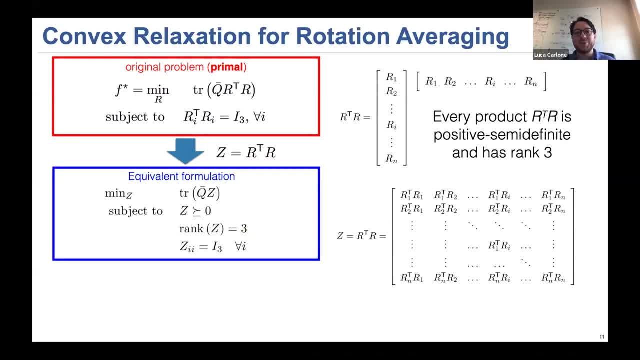 The rank constraint is the only thing here that is non-convex. okay. So a heuristic way here to get the convex relaxation is to say: okay, let's take this equivalent formulation: let's drop the rank constraint and the resulting problem is convex. 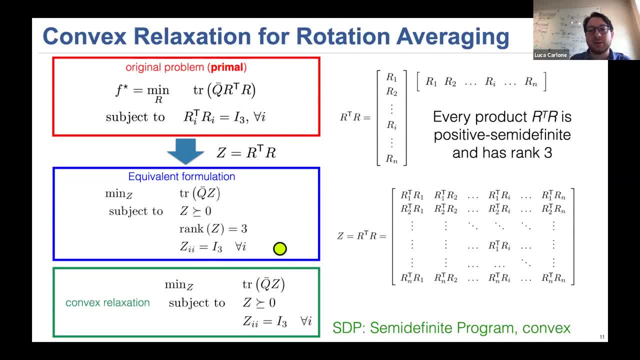 the constraints are the same, but we dropped the rank constraint, which was non-convex. So the resulting problem is a convex relaxation and this is a specific convex problem which is called the semi-definite program because it has constrained, like you know. 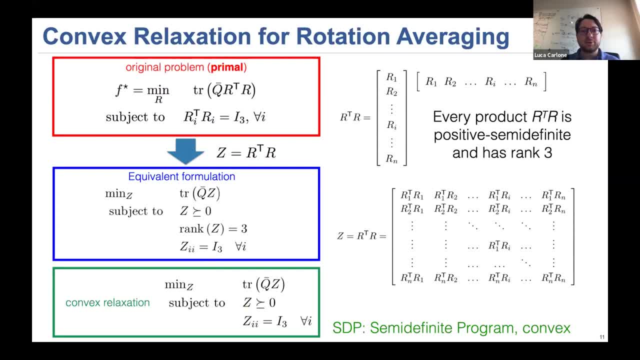 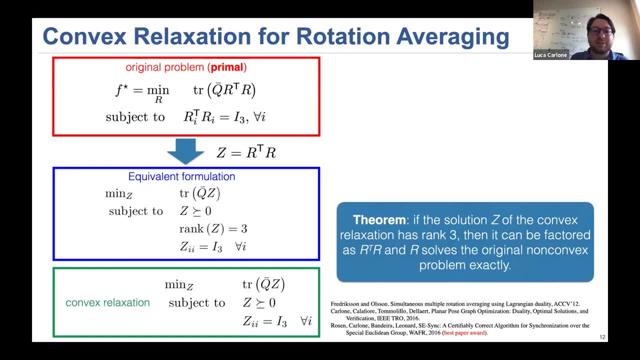 matrices being positive semi-definite. The nice thing out of this convex SDP relaxation is that it's easy to get a posteriorly check after you solve the convex relaxation. you can check whether you have the right solution or not, So it's very easy. 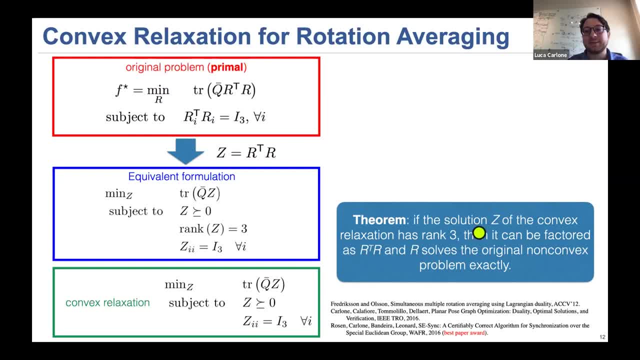 to get the theorem seeing. if the solution Z of the convex relaxation has rank three, then it can be factored into R. transpose R and I'll solve the original non-convex problem. exactly okay, So you can solve the heuristic relaxation. check the rank of Z. 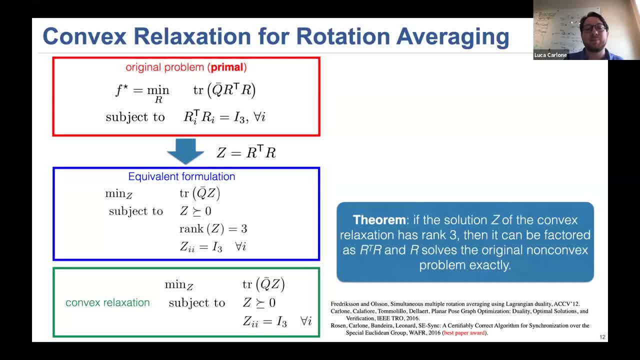 if you get lucky and you get the rank three solution, you essentially were able to solve exactly the same problem. And the nice thing. I will go. I'm going to stress that in the next few slides I'm going to often rank three solutions. 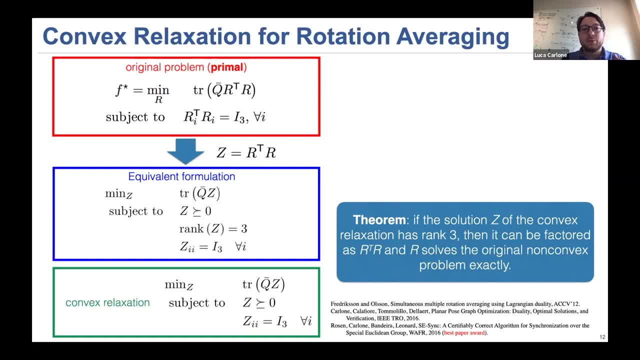 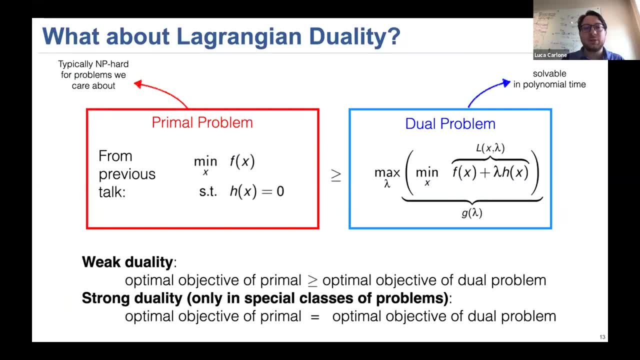 out of these. so the relaxation is exact. So this I said is a kind of a heuristic way to get a convex relaxation. What about you know? how can we use instead the theory from Anders about using Lagrangian duality? So 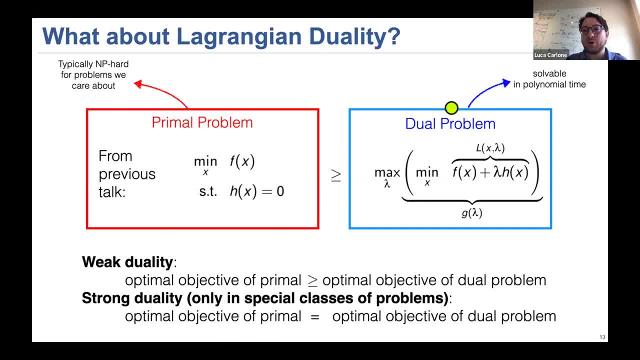 Anders said that for any primal problem we can build the dual problem, which is somehow, like you know, tricky. it looks complicated, While the primal problem is MPR, typically for is going to be solvable in polynomial time. And Anders also mentioned that. 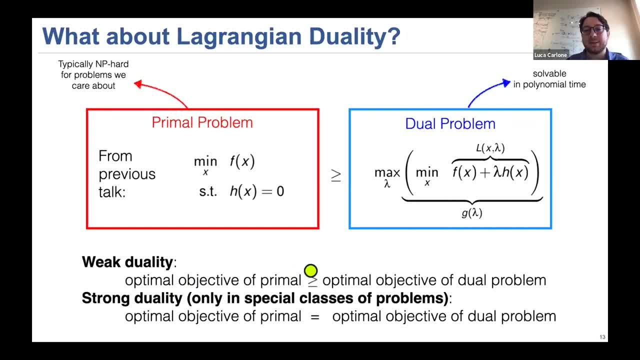 under weak duality, the objective of the primal is greater than the objective of the dual. If you get lucky, we have strong duality and in that case the objective of the primal and the objective of the dual are matching. So if you try to, 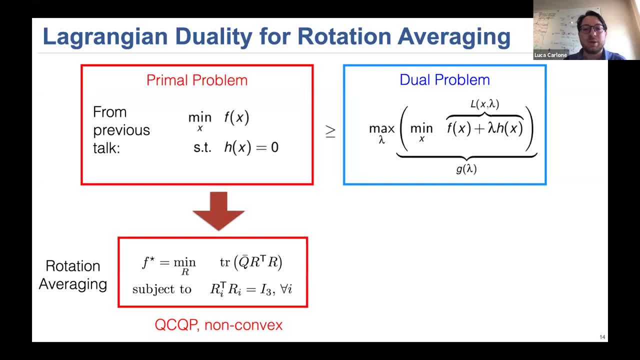 apply this exercise to rotation averaging, we get that the primal problem is the one that I was showing in the previous slides, is a QCQP which is non-convex, And if you do the math you can get also the dual problem, which is this one. 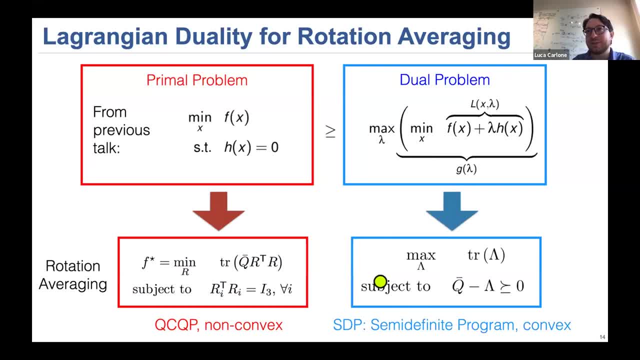 So in the previous version of this tutorial I was doing the derivation of this expression. Actually it takes 10 minutes. It's like straightforward, just math. It's just. it's just essentially formulating this cost function and showing that. 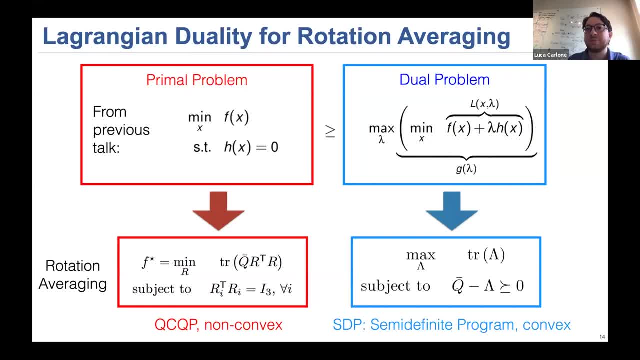 the minimization, the inner minimization, can be solved in closed form. So in this specific problem is very, very easy to get a dual problem, And the dual problem is the addition of the dual variable lambda, which is again another matrix subject to a constraint. 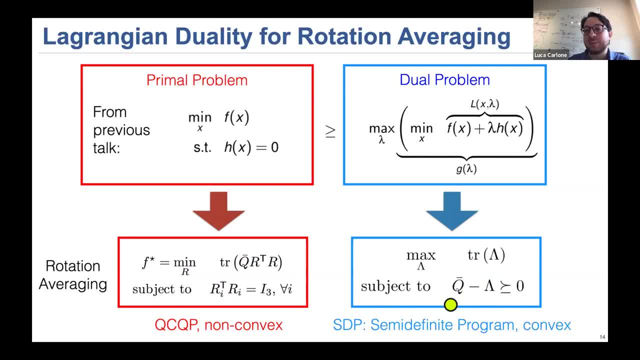 that this lambda somehow, with respect to the data matrix Q bar, should be positive semi-definite. So so far I showed you two different ways to get relaxations, essentially Just a heuristic way to get a convex relaxation and Lagrangian duality. 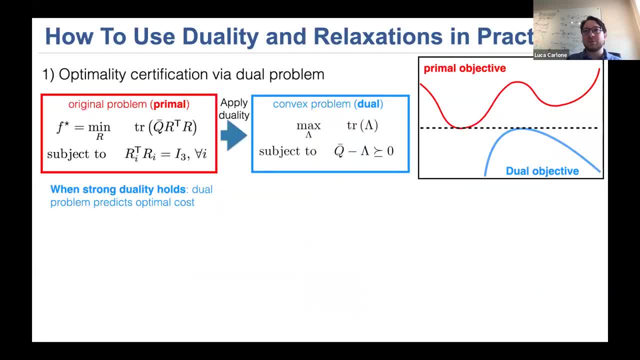 And in the next slide I want to discuss how to use these two things and how they relate to each other, which goes back also to one of the questions we got in the chat during the previous talk. So the first way in which you can get 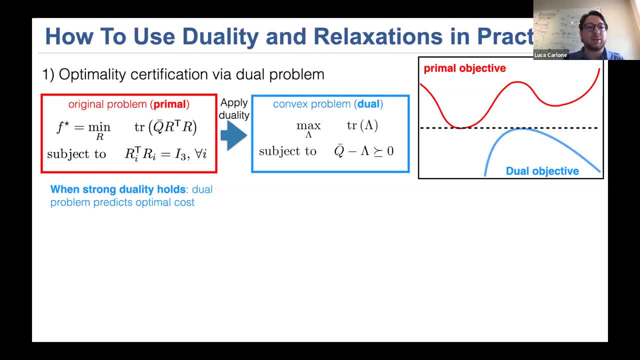 you can use this idea of duality and relaxations, for example, in rotation averaging is for optimality certification using the dual problem. I think this was already hinted to by Anders, So let's say that I have my original problem I try to use 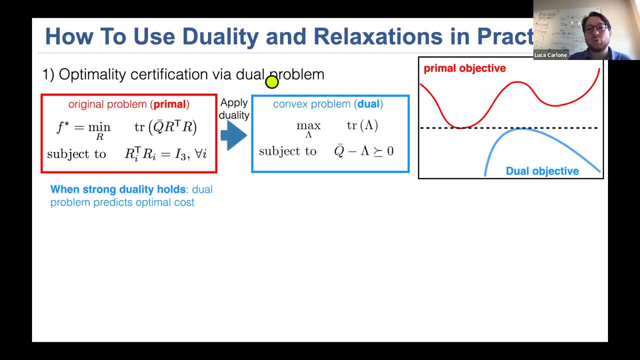 any existing tool to get the solution to this problem. Then I compute what I can solve in polynomial time, and the basic idea is that when strong duality holds, the dual problem is able to predict the optimal cost of the primal. exactly Okay, So 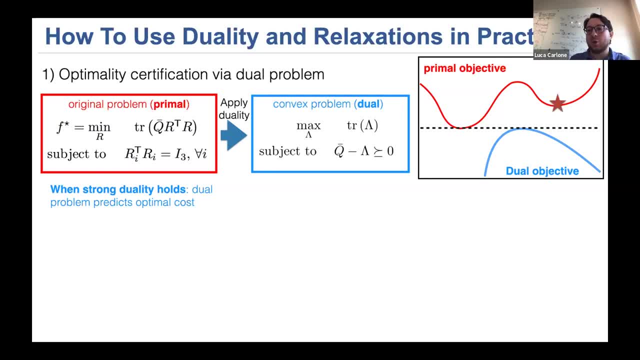 what I can do here is that I call a local solver. The local solver is giving me a local solution to the primal. I can solve the dual to get this optimal objective and using this optimal objective I can say: okay, this local solver converts to a wrong solution. 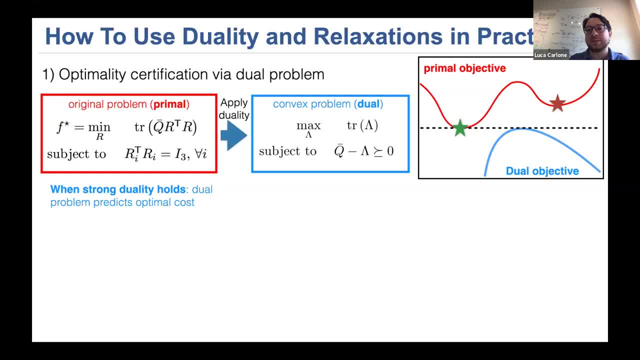 suboptimal and instead, if I call again local solver and it contains the optimal solution, I can essentially verify the optimality of the solution returned by the, by the local solver. Okay, This is what is called optimality certification, or is also called, sometimes, verification. 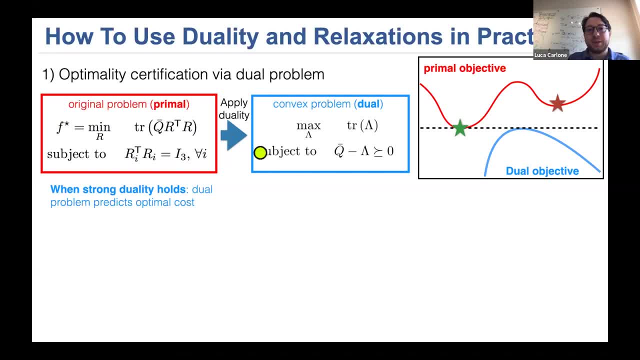 So this is the way we can use the dual problem It turns out. something that is pretty interesting is that if you have the primal problem and you apply duality, of course you get if you apply duality to the dual problem. in other words, you get. 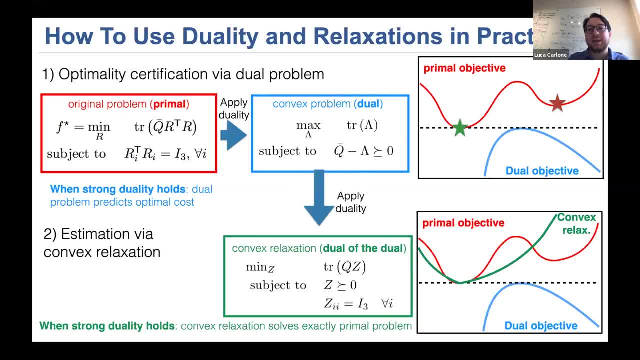 the dual of the dual, you get another problem, which is a convex relaxation. Okay, And if you work out the math, it turns out that the dual of the dual problem is exactly the convex relaxation that, heuristically, we derived in the previous slide. Okay, 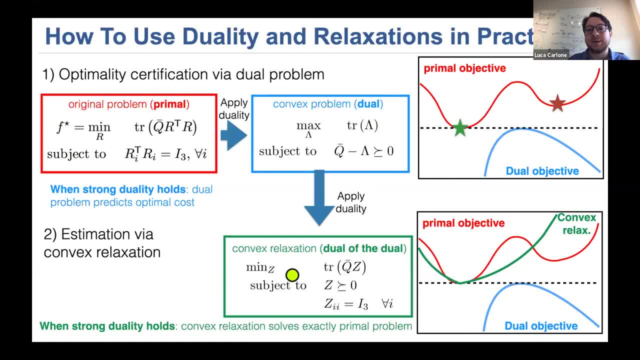 So, in other words, the relaxation that you get through Lagrangian duality and the relaxation, the math at the dual of each other. and since they're both convex, they will give the same optimal solution, they will attain the same optimal cost. So to the convex relaxation. 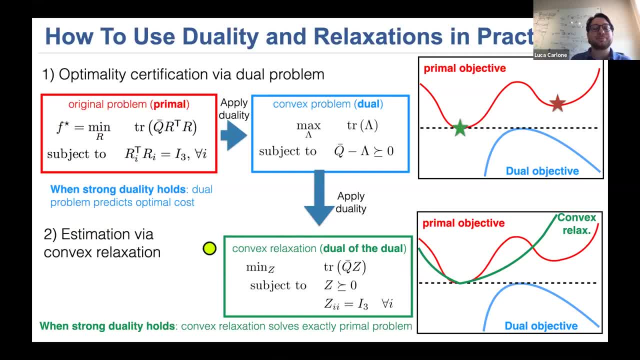 I can have a second use of of this convex relaxation. I can essentially solve the convex relaxation and I can try to estimate my variables directly from the solution of the convex relaxation. And again, when strong duality holds, the convex relaxation solves the primal problem exactly. 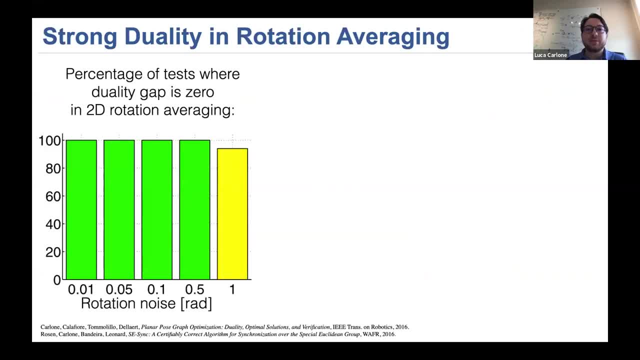 So the reason why we care so much about this relaxation in SLAM is that it turns out that strong duality holds in the problems you care about for rotation averaging, and we are going to see that the same message holds for post-graph optimization. So 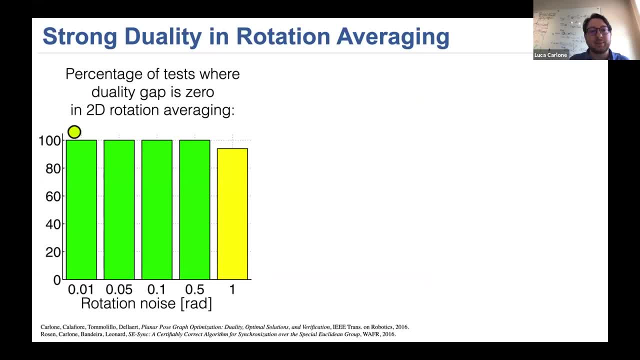 back in 2015-2016, we were, for example, looking at the percentage of tests in which the duality gap is zero, which means that strong duality holds in 2D rotation averaging. And here we're plotting the percentage of strong duality holds. 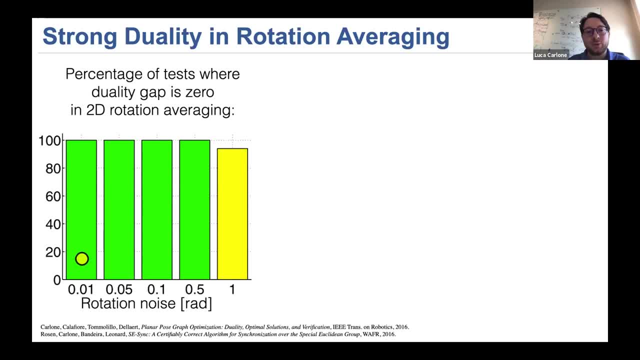 for increasing the rotation noise and you can see that strong duality holds up till the rotation noise is equal to one radian standard deviation, which is a noise that you will never find in practice. So essentially, in practice, strong duality holds for all the problems. 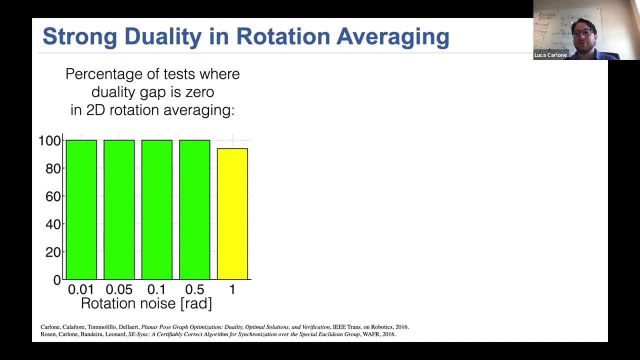 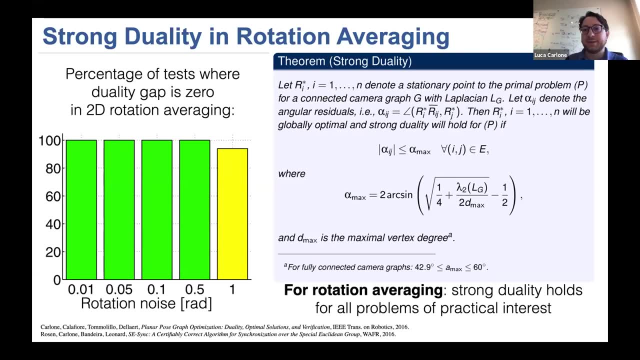 you care about in terms of rotation averaging. This was our original empirical observation. Anders and TJ came a couple of years later, CVPR, saying that essentially we can indeed compute a bound on the maximum noise below which strong duality must hold. Okay, 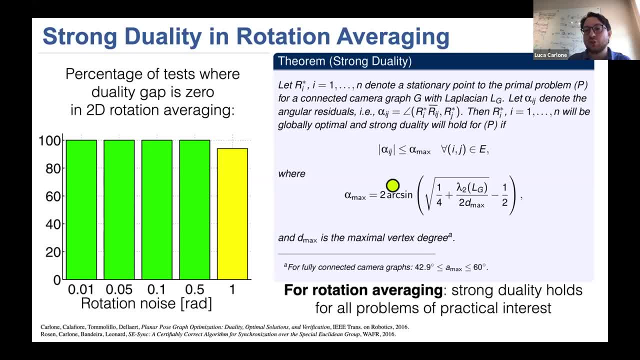 I will not read the entire theorem, but the theorem is saying that if the rotation error on the measurements is below this threshold, then strong duality holds and the threshold essentially depends on the structure of the graph. Okay, the good news is that for fully connected graphs, 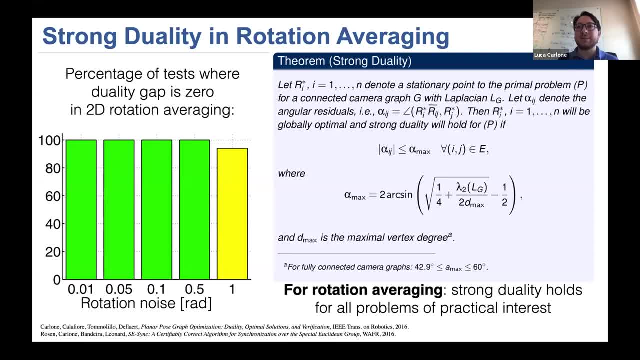 you can tolerate up to 40 to 60 degrees error and you can still have strong duality, which means that which makes this convex relaxation a very powerful tool. So rotation averaging can be solved through convex relaxation. It turns out that if you go back, 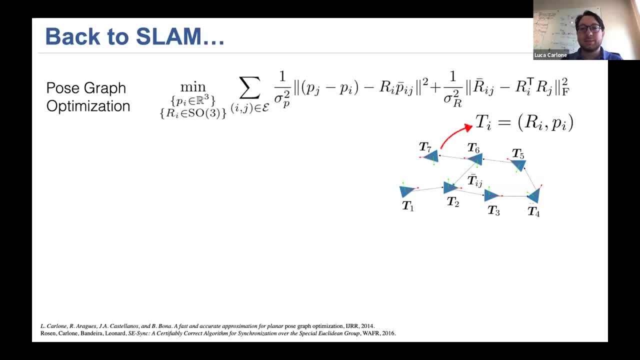 to SLAM. we can do pretty much the same, and this is the expression of post-graph optimization I was starting from. Again, there is the position part and the rotation part. Already, back in 2014, we noticed that the position here appears quadratical. 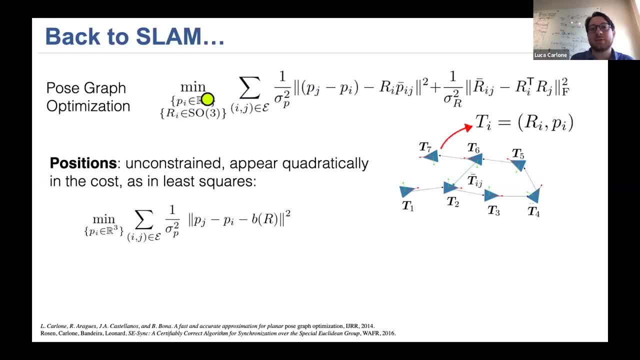 in the cost function and is not constrained. Positions are any vectors in R3. So essentially, what happens is that, for the sake of the position, this is a least square cost which is easy to solve in closed form. So what you can do 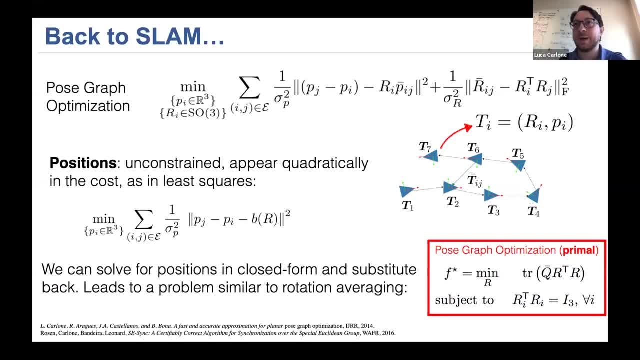 is to, you can solve for the position in closed form and substitute this position back, leading to a problem which is only dependent on the rotation and indeed, if you do the math exactly with the same structure of the rotation, averaging problem that we saw in the previous slides. 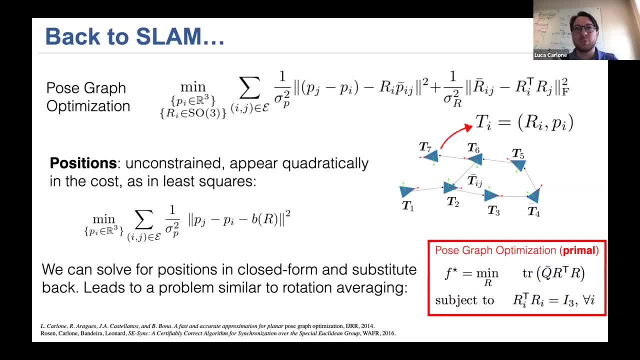 with. the only difference is that the cube bar here will have a different structure, because we'll also include information about the position measurements. So what I'm saying here is that, with this formulation, exactly the same convex relaxation that I was showing in the previous slides. 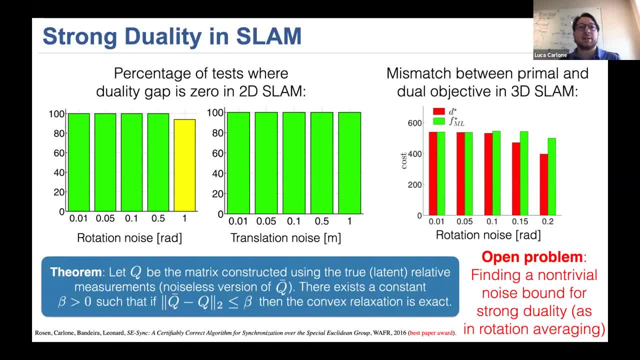 will apply also to SLAM and post-graph optimization and the good news is that strong duality will also apply to SLAM. Again, you can try to increase the rotation noise and the translation noise. on the SLAM measurements You can check the percentage. 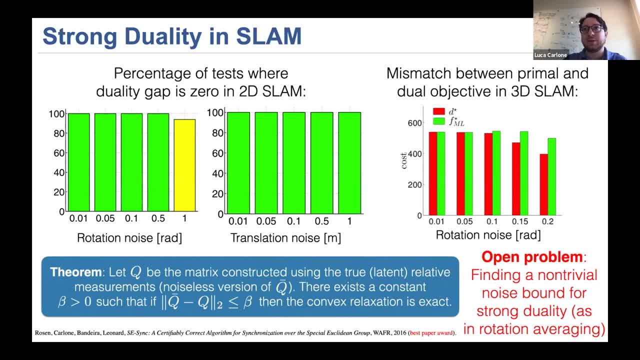 of cases in which strong duality holds and it turns out that for extreme noise you can still get strong duality, and this is particularly true for 2D SLAM. If you move to 3D SLAM, strong duality breaks a little bit. 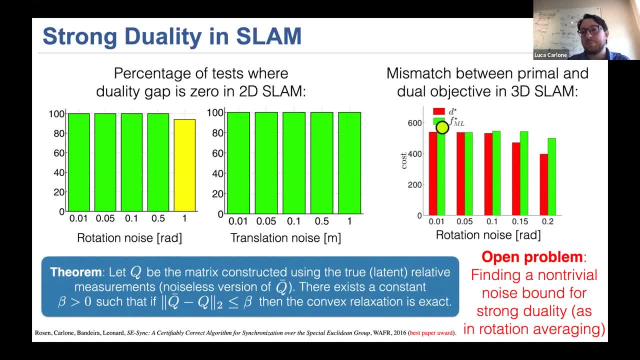 before. So you can see here that I'm plotting the primal optimal objective and the dual for increasing the level of noise and essentially strong duality breaking at 0.1 to 0.15 radians. standard deviation on the, on the, on the rotation measurements. 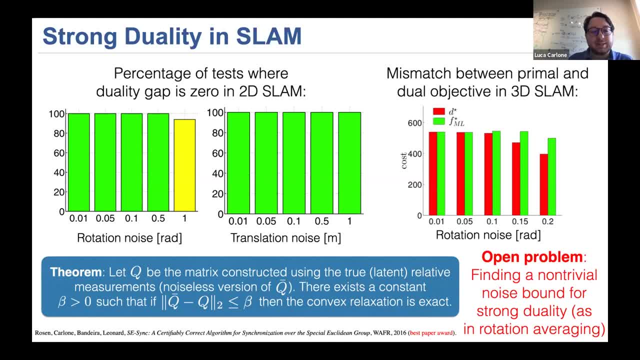 Here's a big open problem which was partially addressed by the work with David Rosen back in 2016.. The problem is about finding an untrivial noise bound for strong duality. So we said that Anders and PJ for rotation averaging they were. 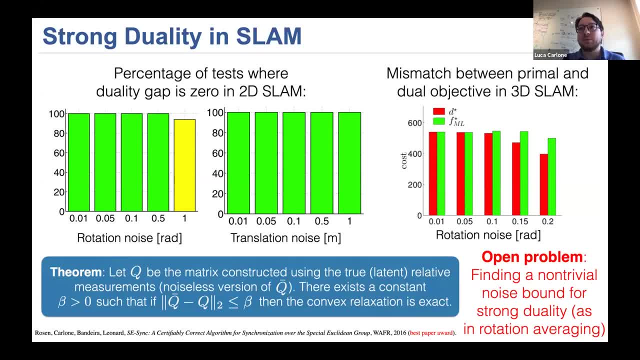 able to establish this theoretical bound below which strong duality must hold. The same result is not available for post-graph optimization. We cannot quantify what is the maximum noise under which there is strong duality. We have some initial result again, like you know from the work. 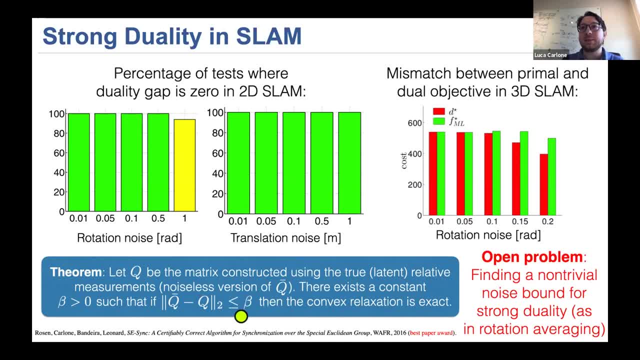 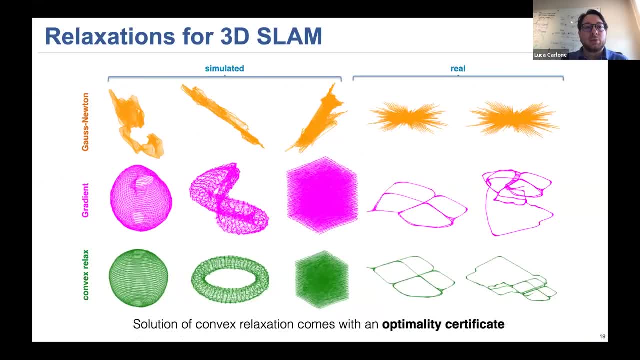 on scsync, but which is saying that essentially strong duality will hold below a beta. but the expression of beta is not something that we were able to give. so you already noticed that actually convex relaxation will make a difference. so if in SLAM you run a local solver, 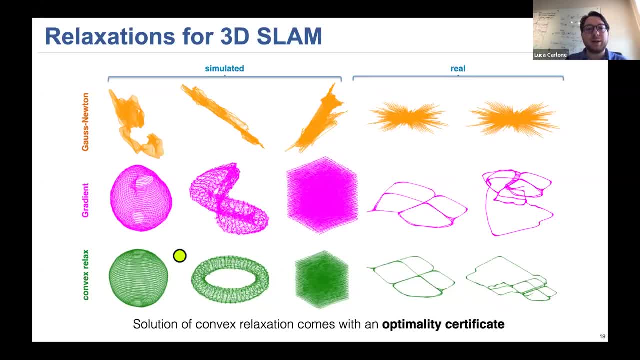 like Gus Newton and Gradient, for different data sets you can get local minima. the convex relaxation will return you a visually correct solution and will also give you an optimality certificate again when the solution of this problem is rank 3.. Okay, so in the second part, 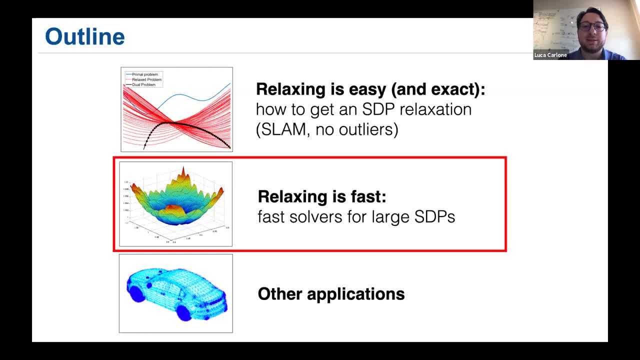 of this talk, I want to spend three slides commenting on the fact that for specific problems, in particular for SLAM problems, doing this relaxation can be very fast, and I'm I want to spend like a few minutes on that. the typical concern is that that you can hear. 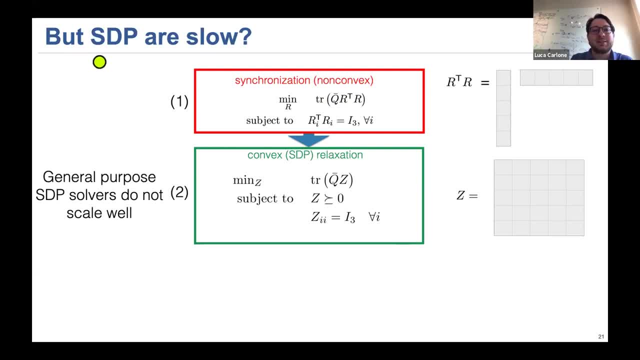 after you work a little bit on convex relaxation is that. the comment is that semi-definite programs are slow to solve, so they are polynomial time, but they are not as scalable to solve as what you can do, for example, in local solvers. but the truth is that. 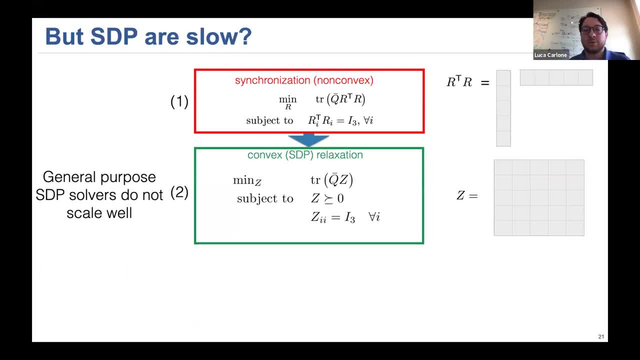 for specific problems. you can indeed engineer an optimization for these, for these semi-definite relaxations. So what I said in the first part of the talk is that we transformed, let's say, the rotation synchronization problem into a convex, semi-definite relaxation. and if you look, 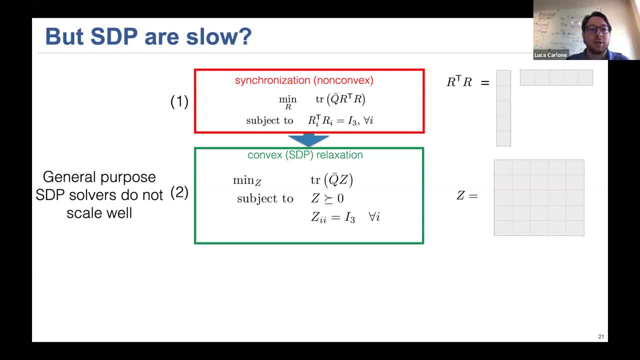 back into the literature on convex optimization. it turns out that Bure and Monteiro, back in 2003, said that a good way to solve this kind of optimization problems is to replace z with a product x, transpose x and try to solve locally this problem instead. 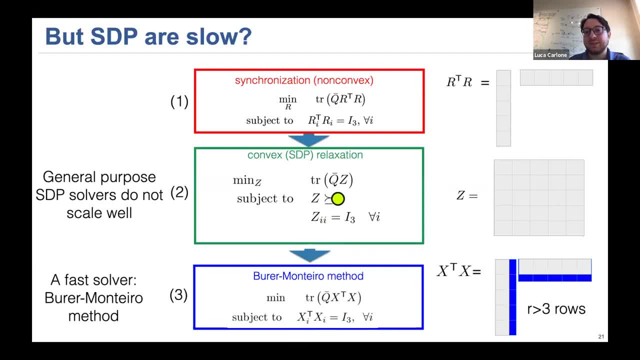 Okay, so after you solve, you replace z with x, transpose x. the positive semi-definite constraint becomes redundant and you remove it, and these constraints can be written as x- transpose x, and for those of you who have seen this for the first time, this would sound a little bit crazy. 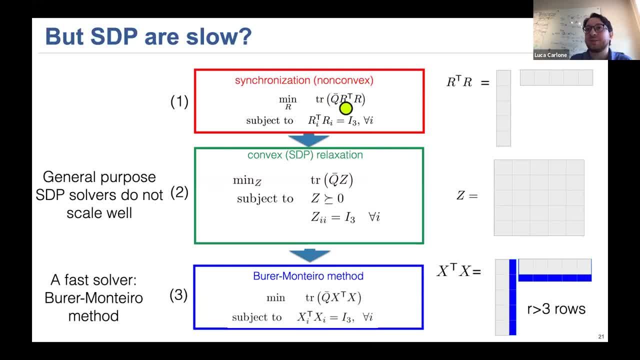 but the problem structure, which is identical to the first one, right, but here the trick is that the x is a little bit larger. so instead of having, like you know, three rows, we'll have many more rows. we'll have, like you know, five, six rows, and the insight. 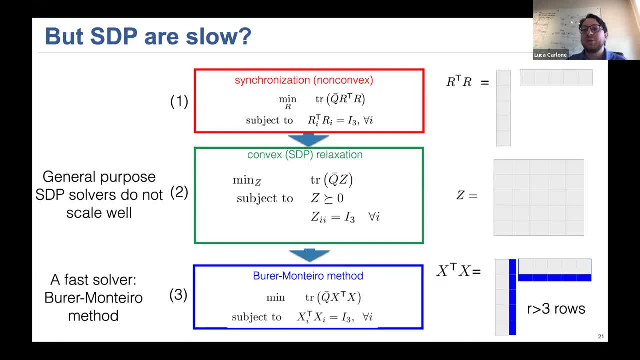 here is that, if this number of rows is large enough, you can prove that the local solver applied to this problem will give you the optimal solution to the SDP relaxation, which is something that we'll analyze in the next slide. so the Buhler-Montero method. 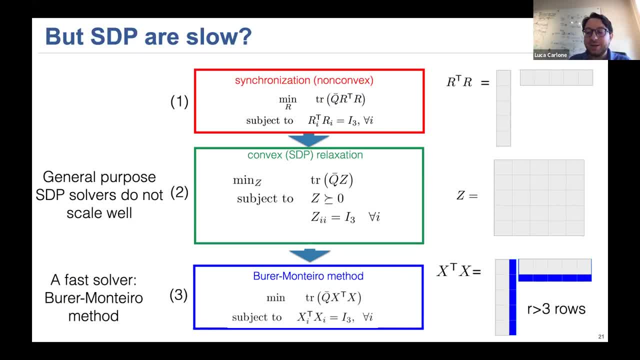 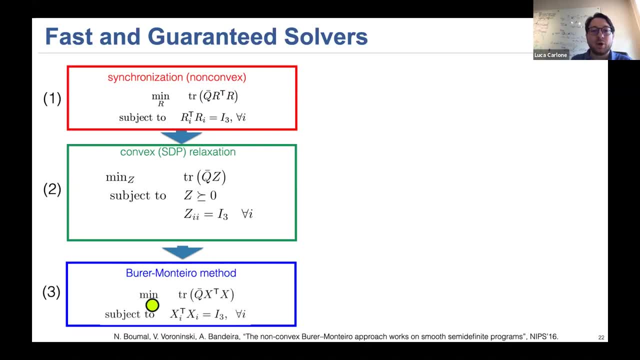 has been known since 2003, but only recently people started to understand that there is- there are, like you know, theoretical guarantees that you can establish when solving the Buhler-Montero method and, in particular, Bumal in 2016 got a very nice result. 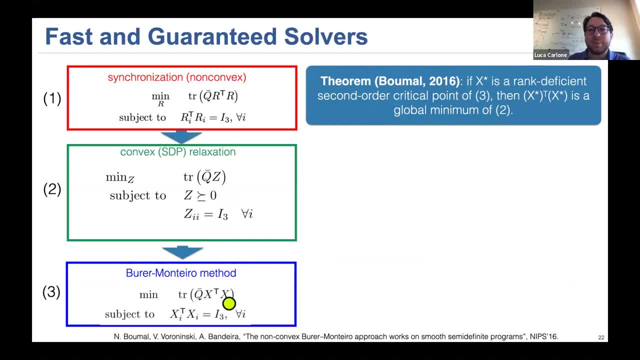 seeing that essentially, if you solve the Buhler-Montero method, you get an x star. this x star is rank deficient and is a second order critical point of this problem. second order critical point is a condition which is very easy to check. then x transpose. 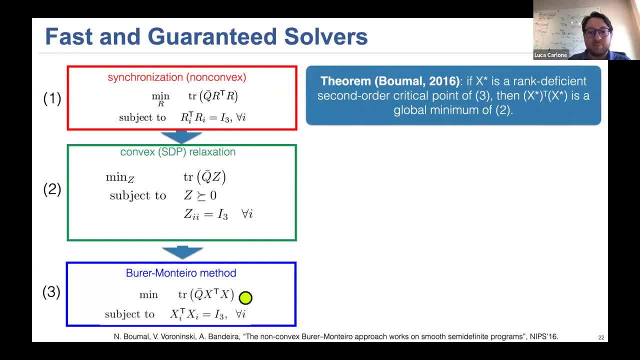 x is a global minimum of two. okay, so a local solver applied to this problem can find a global solution to this one. and Bumal also said that if the number of rows in this matrix x- if the number of rows are- is large enough, any second order. 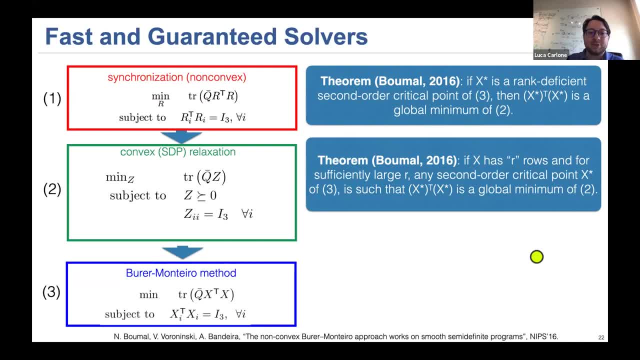 critical point will be a. so if you make x large enough, you can try to solve with a local solver these Buhler-Montero methods and you will always get a solution to the SDP relaxation. so this insight sparked a number of contribution and the important- 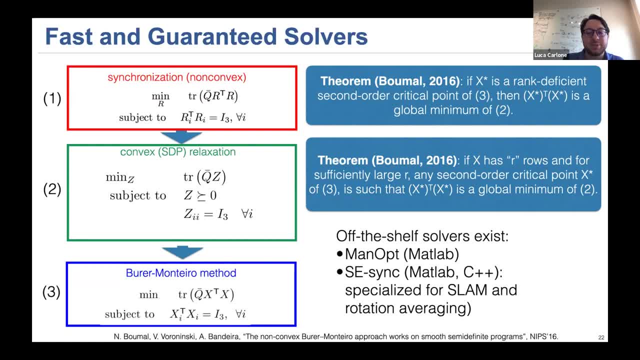 bit here is that there exist solvers. you know, Manopt is a general solver for this kind of problems in MATLAB and this work has been pioneered in robotics by, in particular by David Rosen, who has been working with SYNC, which is in MATLAB, and C++ is open source. 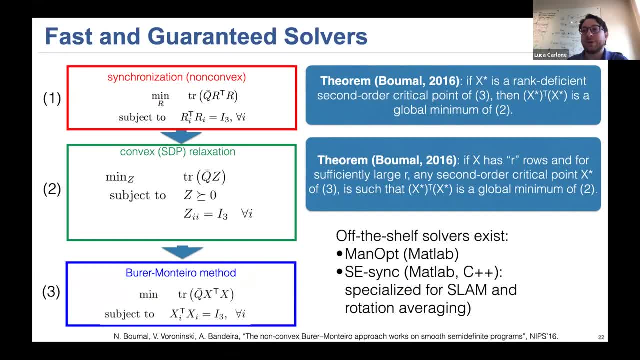 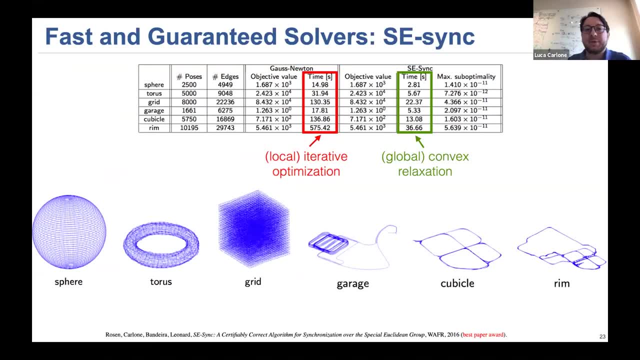 which is a specialized solver for SLAM and rotation averaging based on the Buhler-Montero methods. so how fast is this Buhler-Montero method? well, indeed, it's pretty impressive if you consider, like SLAM data sets here on the rows. 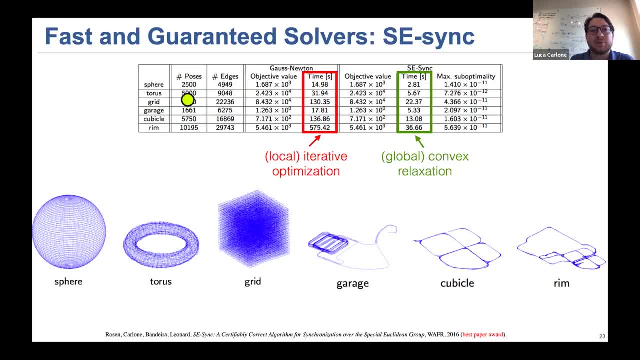 you can see a bunch of SLAM data sets and very large problems, like you know, thousands of poses, ten thousands of poses, thirty thousand edges, and you can see that the cost in terms of time for a local solver, let's say the Gauss-Newton solver, and you compare that. 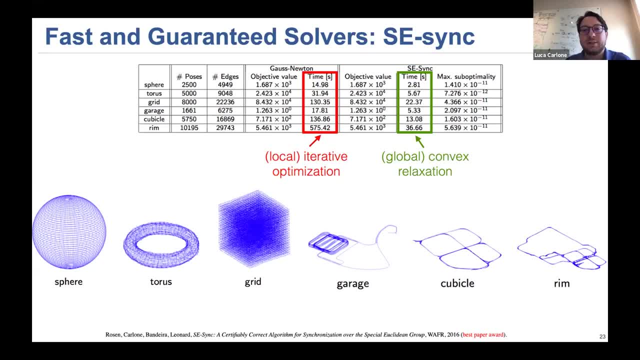 with the SCSYNC, which is based on this idea of Buhler-Montero, you can see that a good implementation in SCSYNC can be even faster than a local solver. and here not only SCSYNC is faster, you can see, there is. 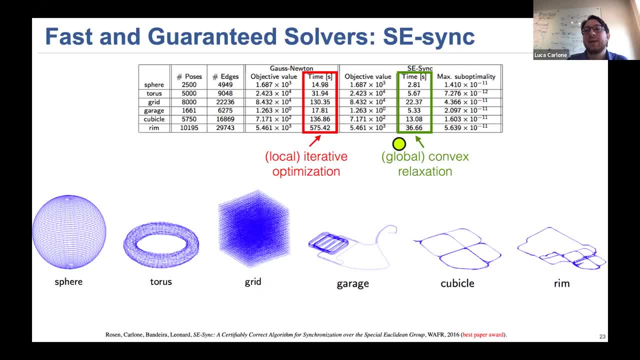 roughly like an order of magnitude difference in terms of timing for some of the data sets. not only that, but SCSYNC is a global solver, so we'll get to the optimal solution here. all right. so I'm running a little bit out of time, so we'll close. 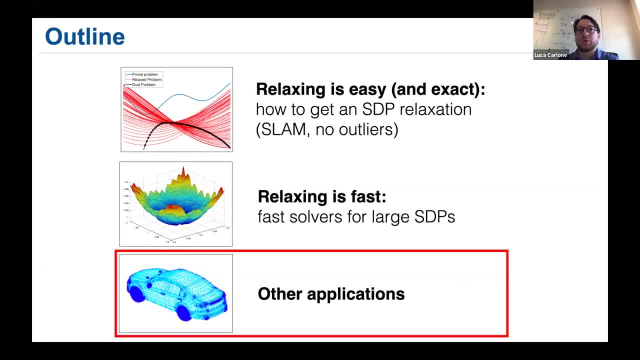 with other applications. here I really want to mention a few key ideas. I think I have two or three slides left. the basic idea is that S4SLAM was like a success story. we're able- like you know, the community was able- to design convex relaxation which are empirically tight. 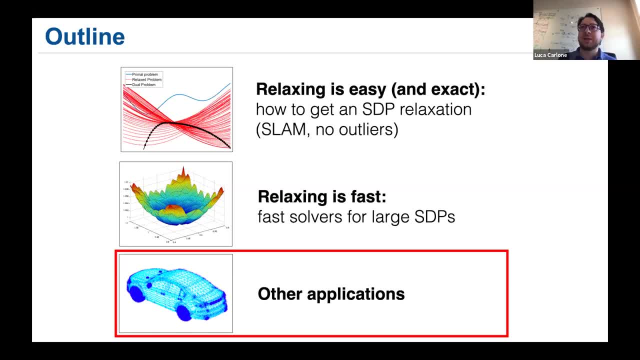 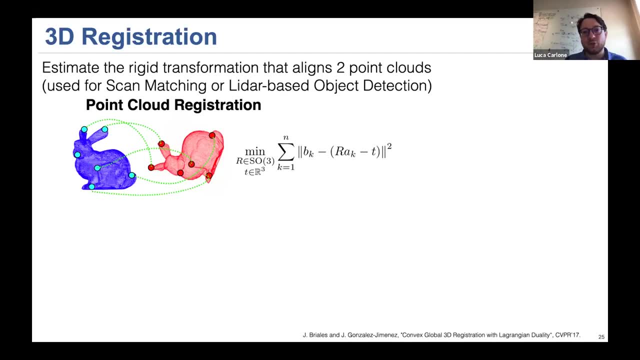 and to develop even fast solvers. we're seeing the same trend in other applications. so for 3D registration, Anders mentioned his slide that 3D registration is about aligning point clouds, which is a following showing up for scan matching in robotics or for LiDAR detection. 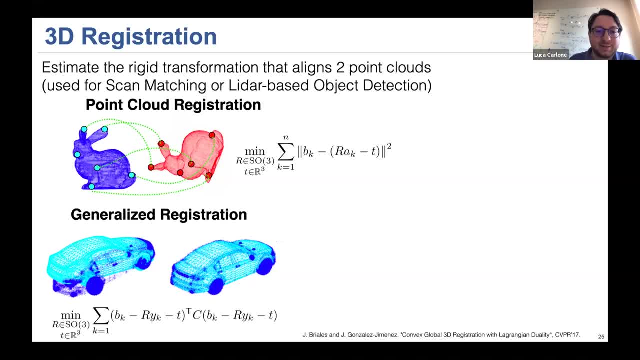 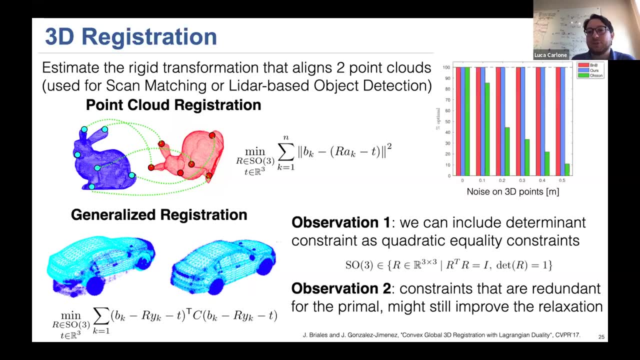 in LiDAR based object detection, and I think Anders already mentioned that there exists a tight relaxation for this problem, and what I want to stress here is that well, first of all, I'm showing here again: the percentage of optimal tests for increasing noise is always tight. 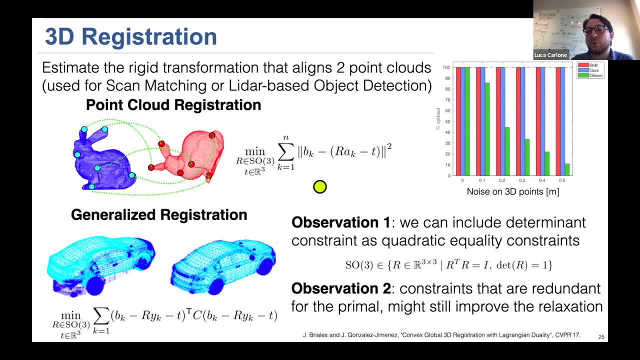 always successful, but I want to use this slide to observe a couple of things. okay, so the first observation is that I already mentioned that it is possible to include the determinant constraint, which is arises from the rotation matrices, as quadratic equality constraints, and I mentioned that that didn't matter. 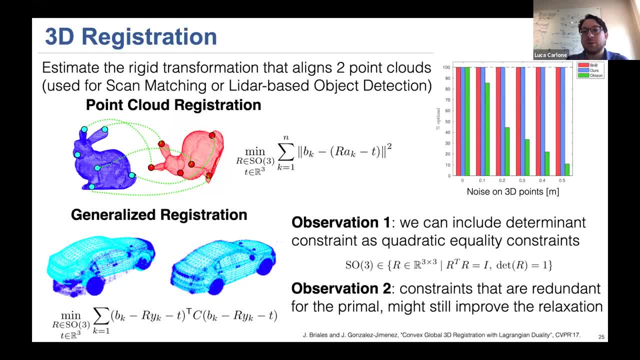 in SLAM. but it turns out that for this problem of generalized registration, including that, it makes a difference and in particular there is a general observation that if you have constraints that may be redundant for the primal problem, you may still end up with a better relaxation, okay. so 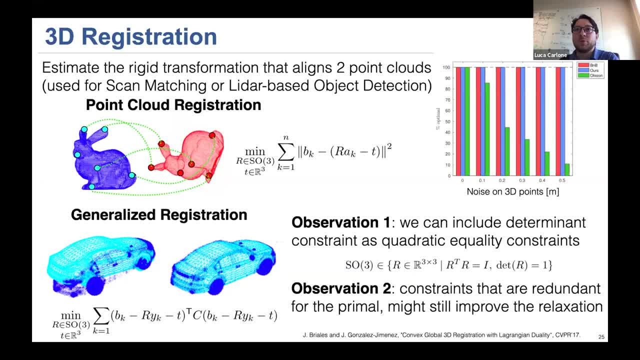 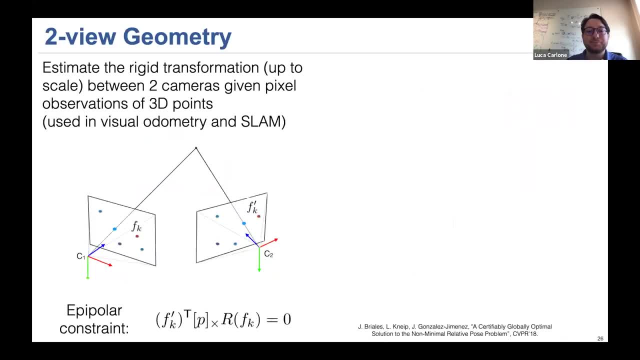 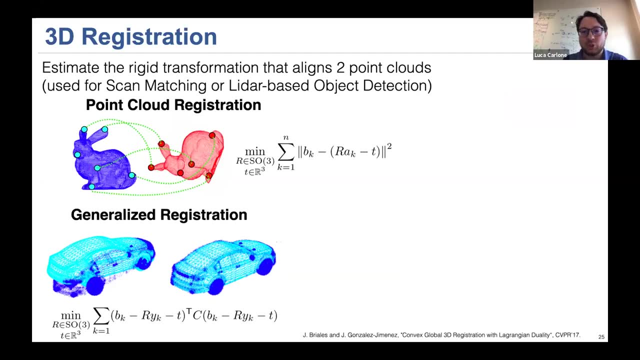 if you have more and more constraints to the primal problem, you can help improve the quality of the relaxation, which is some key idea that shows up in this work on registration and also in the next slide. by the way, this is work from Bialis on tight relaxations. 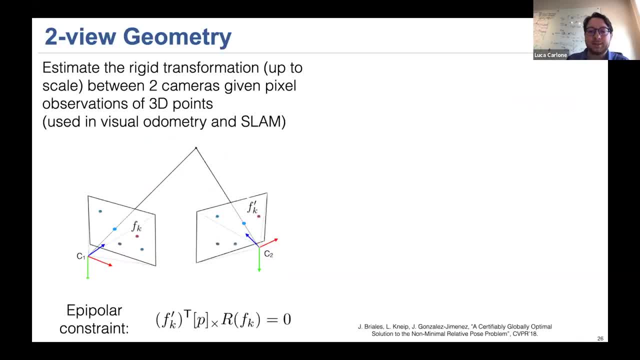 without outliers. this one is another example from Bialis. CVPR 2018 is about two-view geometry, which is about estimating the motion of the camera within two timestamps. so the camera is observing a bunch of points projected on the camera itself and the problem: don't pay too much. 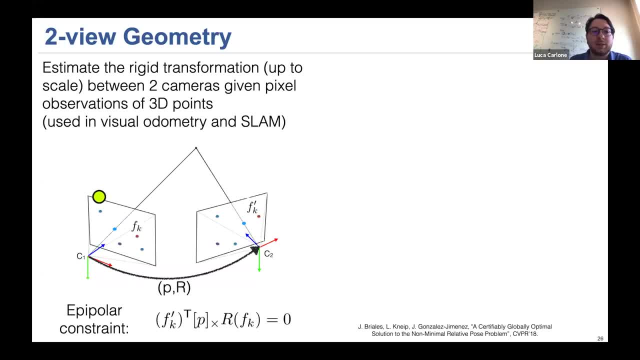 attention to the math, but the problem is about using these pixel measurements to figure out the position of the robot up to scale, and Bialis again show that it's possible to get a tight SDP relaxation where the suboptimal, the optimality gap, is zero. 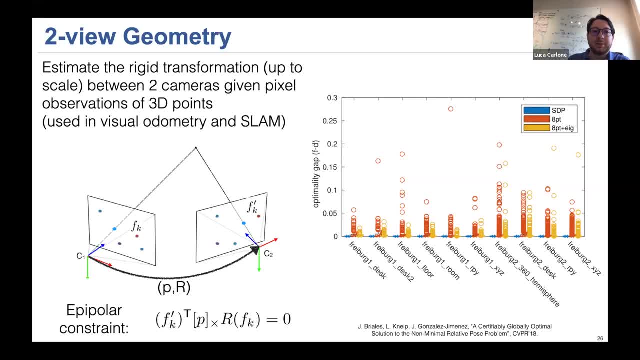 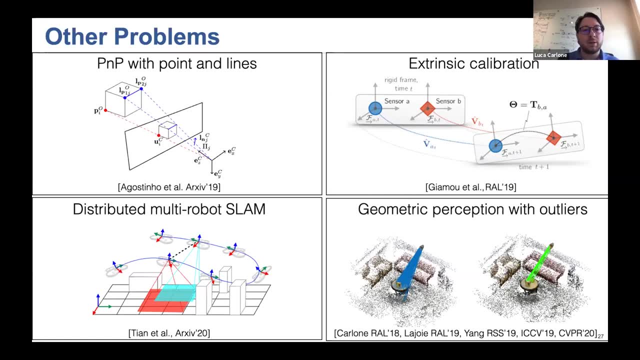 which in other words, means a strong duality holds. these are just two examples, but the truth is that in the last, I would say, two to three years, we've seen many, many examples of cases in which we have geometric perception, in particular geometric perception without outliers to 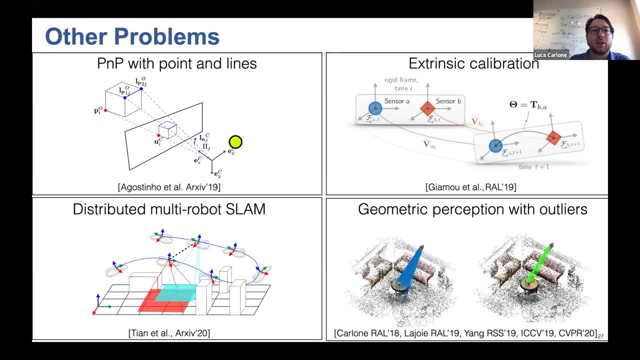 typical SDP relaxations and we have strong duality. one example is object detection in images using lines and points, which is called the PMP, with points and lines problem. again, this is like an archive 2019 group from Jonathan Kelly at the University of Toronto. 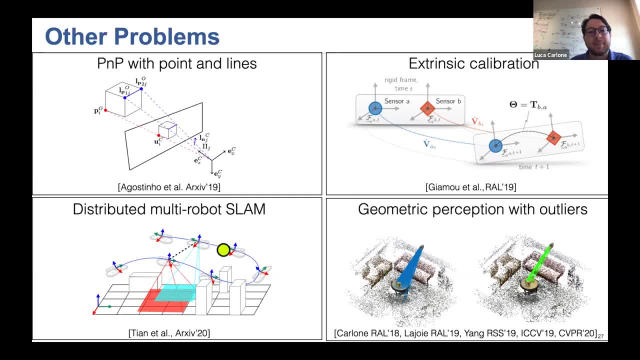 have been showing tight relaxation for extrinsic sensor calibration, which is an important problem in robotics and we are working on use of these. convex relaxation for SLAM, for distributed multi-robot SLAM and, more recently, there is an increasing emphasis on geometric perception without layers. I will not talk. 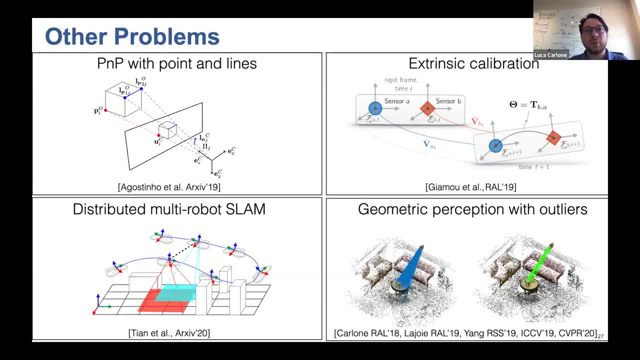 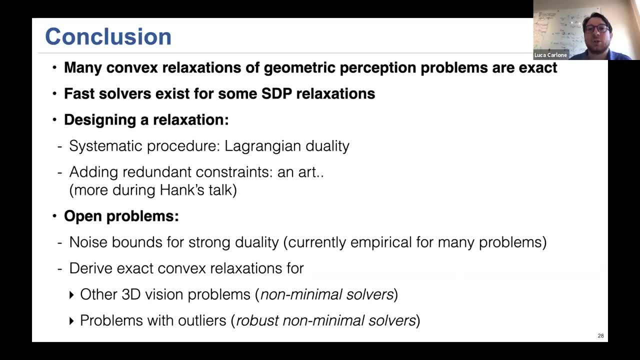 too much about these because essentially the topic of the next two talks. so we conclude here and I will say that for the bottom line of this talk is that for many convex relaxation, many convex relaxation of geometric perception can get even fast solvers for these relaxations. 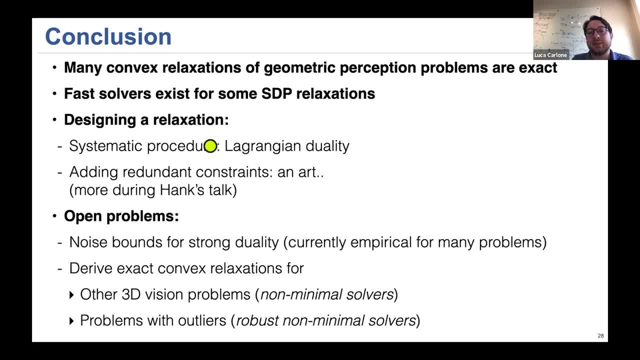 and designing the relaxation is actually a systematic. there is a systematic procedure which is Lagrangian duality, although sometimes you have to heat. you know to manipulate the mat and other redundant constraints to improve the quality of the relaxation is a little bit of an art, although Hank 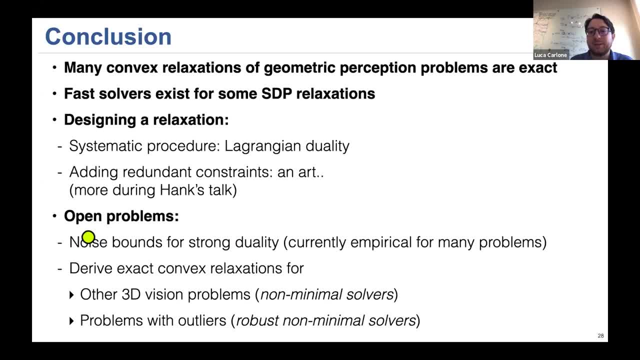 in his talk is going to provide a little bit of a more systematic way to do that. but this is an open problem for many, many problems, except for rotation averaging, deriving exact convex relaxation. for other three division problems is largely open. there are still many problems to go. 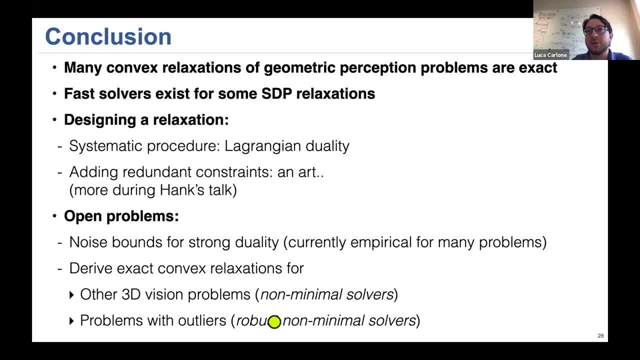 and problems without layers. again, most of the work on problems without layers is over the last two years, so there is definitely more and more work to do there. so I'm largely out of time here, so I will finish here the questions, otherwise probably we'll have to move. 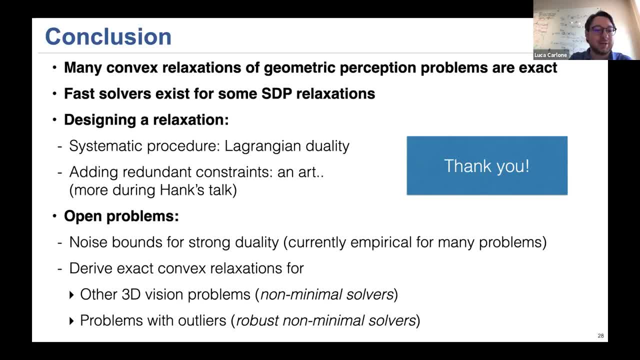 to the, to the. we'll take a short break and then move to the next presentation. I can ask a question if there's? yeah, I see many, many questions. I don't even know where to start here. so, yeah, go ahead, please. yeah. so yeah, I posted one question. 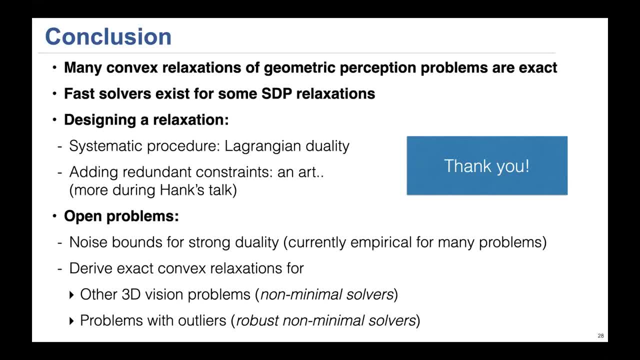 on the chat. it's pertaining to most of the results that you showed. they seem to be for a batch mode slam solution where you have all of the data beforehand. do you have any insights into how this can be, you know, made adapted for an online or an incremental? 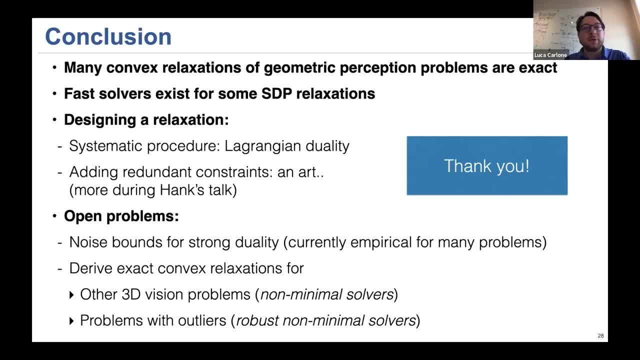 solution. yeah, I think there's a question, a lot actually, and I think that there is a trivial question. there is a trivial answer and there is a deep answer. so the trivial answer is that you can do two things right, so you can solve at time t right. 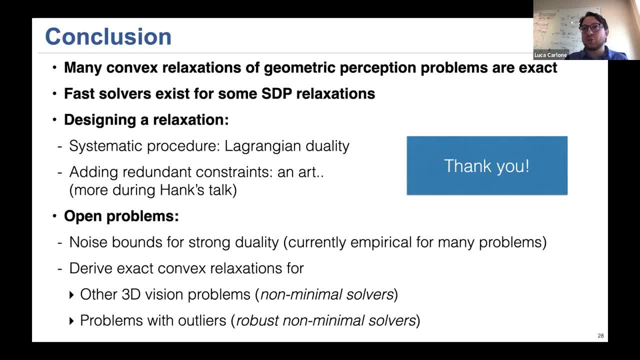 you can compute an estimate and you can use that estimate to warm start mechanism. another potential solution is to realize that in slam and in postgraph optimization you don't need to optimize it each time, actually if you do not have loop closure. the optimal solution for slam: 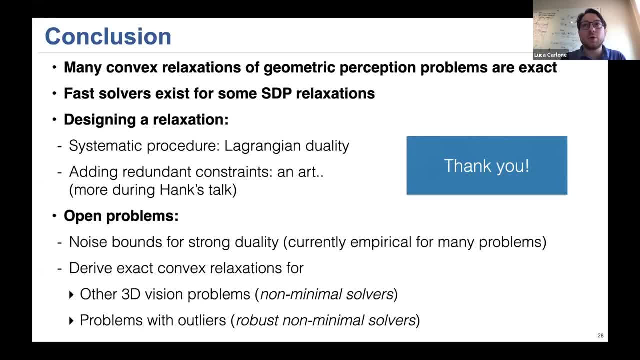 is just to concatenate the odometry right. so ideally, more than being just batch, this is a solution resolver that you need to invoke only when you have loop closure. yet another answer is that you use a local solver most of the time. use gtsam and these existing 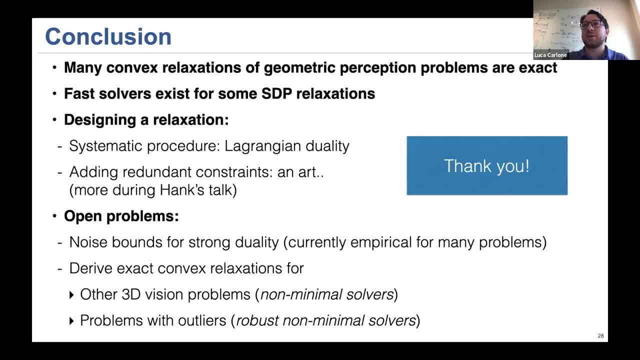 local solvers. i use this theory in the background to sanity check that the solution from the local solver is optimal, which is this idea of optimality certification. so these are the three immediate ways in which i would i would deal with incremental operation, online operation in slam. 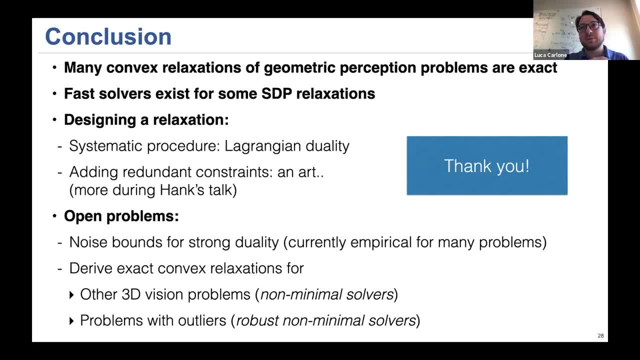 manipulating the math in a way that is typically done in incremental slam to make this truly incremental. there is a deeper answer there and there is investigation to do so. that's open problem. i would say so just to summarize. there are three ways to do that. if you want to get 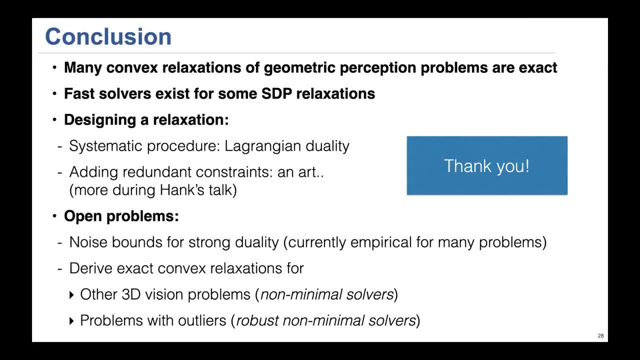 really the maximum speed up and work out the math to get the maximum speed up. it's an open problem. yes, thanks. so there is a question about. there is a question about the determinant constraint that i dropped from the derivation, so i will try to address a bunch of questions. 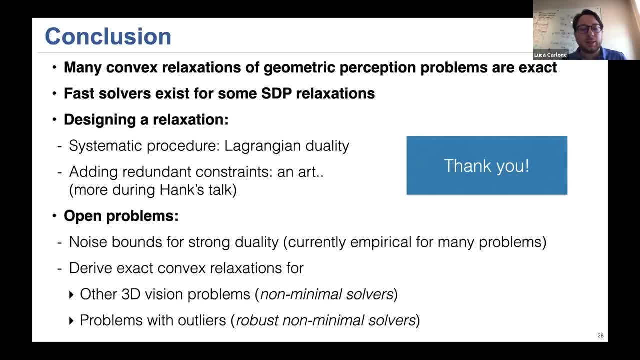 at the same time on this determinant constraint. the basic idea is that if you drop the determinant constraint, you can get both rotations and reflections right. so reflections are typically not, it's not a physical motion of the robot. so you don't want that. you want proper rotations. 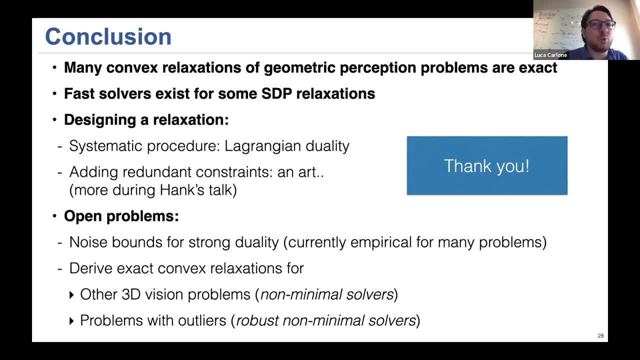 so what is possible to demonstrate- and i think david has a proof for that in the assessing paper- is that under some, if the noise is not crazy, like you know, under all reasonable noise assumption for the rotation measurements, the solution of sc sync will be either all rotations, 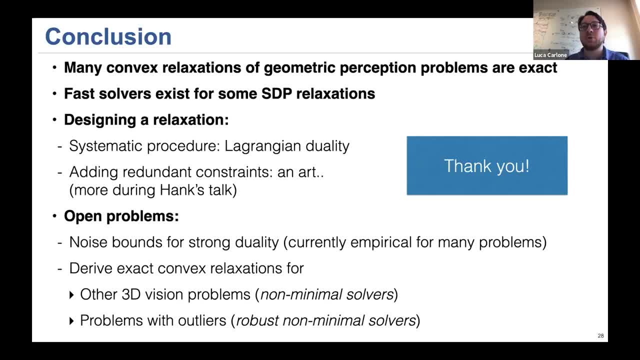 or all reflections, and in the case in which they are all reflections, you can flip the sign. let's say, you can flip the sign of these reflections and you can get the corresponding rotation. okay, so in other words, you can apostrophize the rotation and you can get. 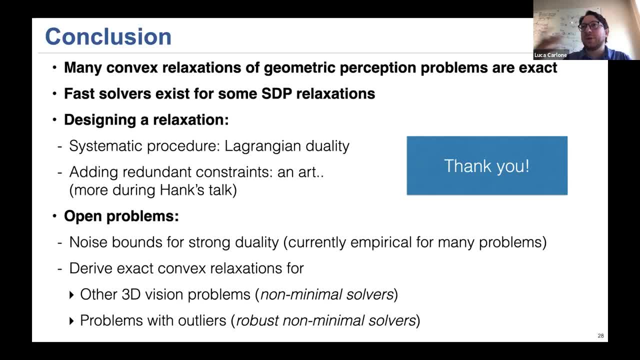 the corresponding rotation. okay, so in other words, you can state that that constraint is redundant for the slam problem. it's not true, for example. i mentioned that for registration, for example, is not true um other problems which are open in three division. so that's another question can you give? 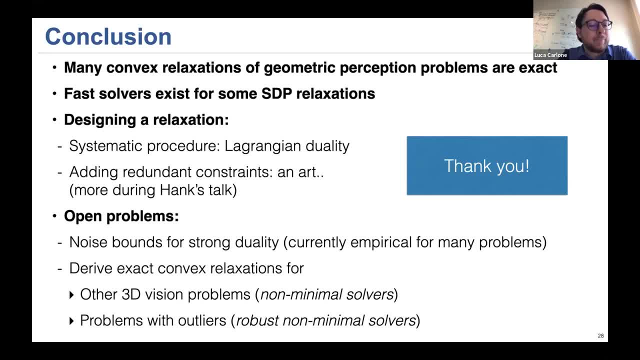 some examples of other open three division problems. um so um. i mentioned one area which for which you will learn much more in the last presentation, but the truth is that, while this work i'm presenting here, scc and all these relaxations have been like you know. 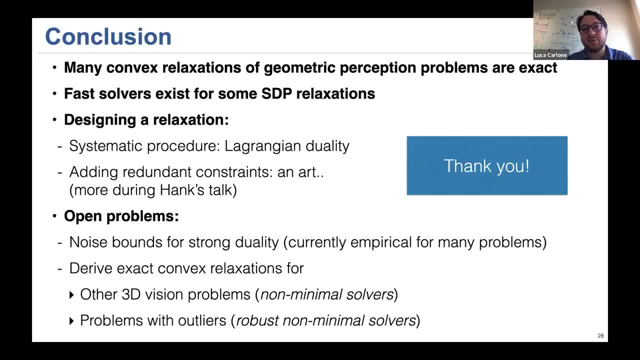 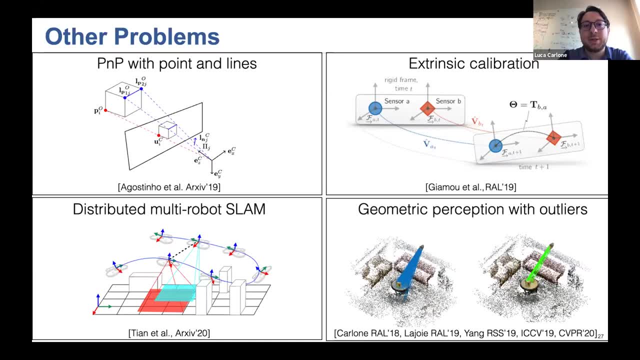 the first to show the power of this relaxation for robot perception, the presentation i just gave and all the the relaxation that i've been showing the previous slide. but the truth is that in practice you always have outliers. so i think that right now, one of the most 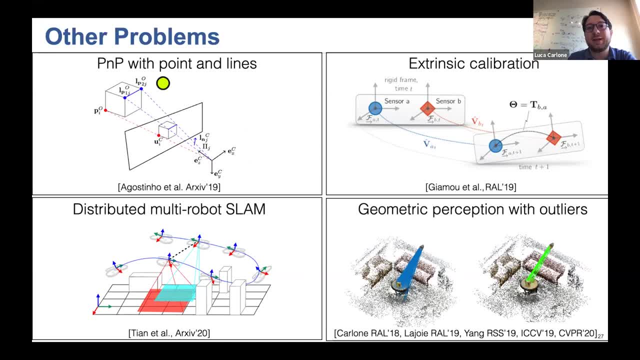 promising research areas is uh, to repeat the success of, like you know, these problems, uh, point and line, pmp extrinsic calibration, distributed multi-robot slam in the presence of outliers. okay, so we started to do a lot of these uh simulations, for example, something that uh. 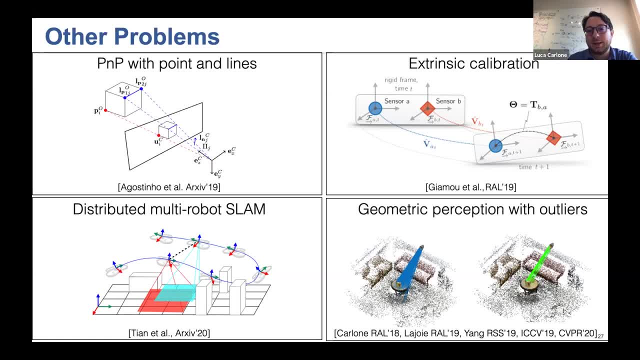 uh, i can be very upfront saying that we do not have a satisfactory solution is slam without pliers. so you will see that i'm putting a reference here to uh la croix, erav 2019, where the initial relaxation for slam without pliers is not performing. 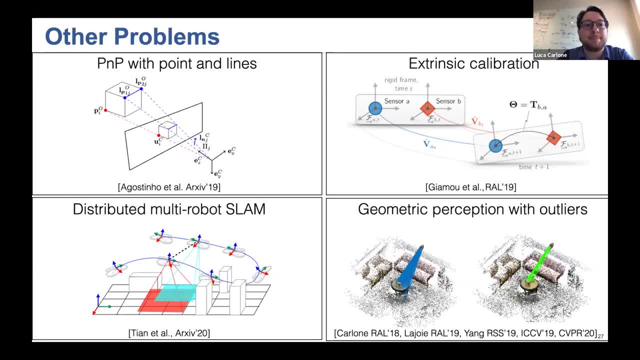 as is not as robust as you want, for example. so if you think about other vision problems, um, i don't know, i feel that somehow, like you know, you can um this, this stuff of convex relaxation can essentially redesign the way we understand vision, the way we understand. 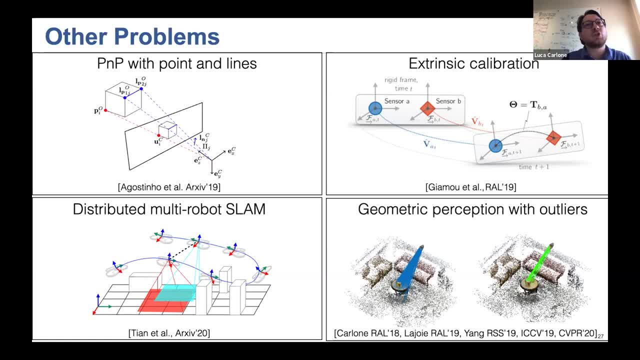 optimization for vision. so i suspect that if you go back to very traditional problems in vision and geometric vision, you can see that there are a lot of problems, um, and you can see that there are a lot of problems, um, but if you think about slam, there are. 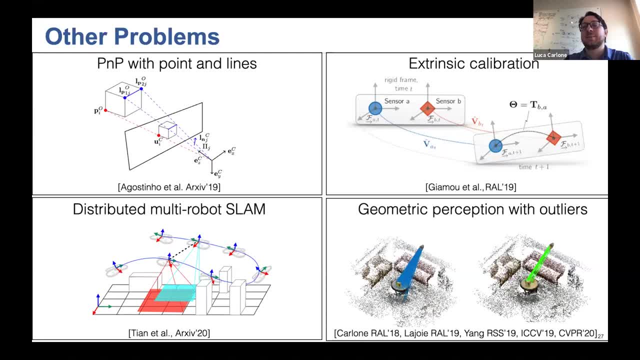 many, many more different formulation. there is visual navigation, there is visual slam. all of these will have a slightly uh uh similar, uh more uh um, uh uh uh. i don't. i think that's what. what uh um here. yeah, um, i think that's uh a i think. 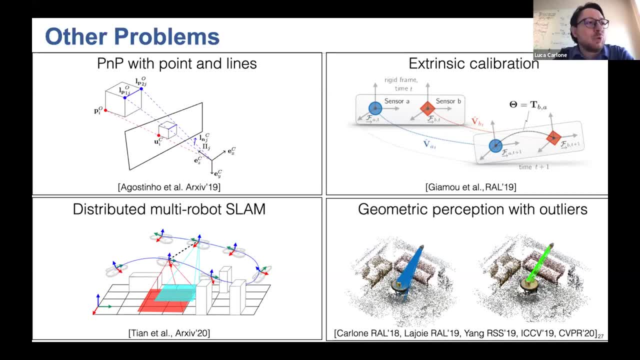 that's a- uh, I have to admit that- bundle adjustment. I tried looking at the math, I think back in 2016 or 2017, and for a reason or another I decided to focus on the outlier case. I don't think that there is. 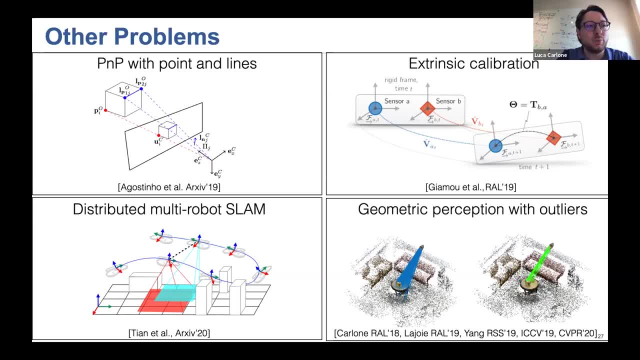 there is. I think the math is very more complicated because if you do projective geometry, there will be, like you know, fraction and division by, by variables, and so will be like rational polynomials, and so on will be a little bit more complicated. 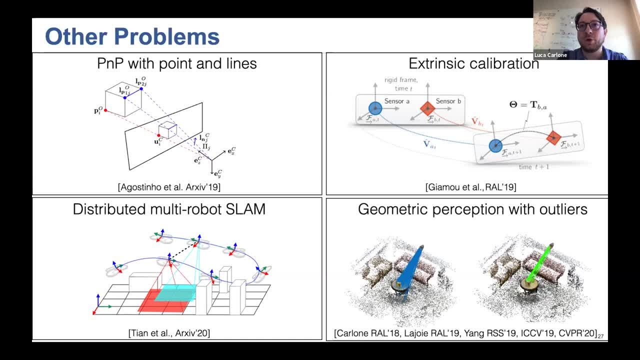 And at that time, like you know, I decided to look more into problems with outliers. My suggestion is to look into this. So I think that right now, for example, what we learned as a community over the last three or four years, I think that these problems are attackable, Okay. 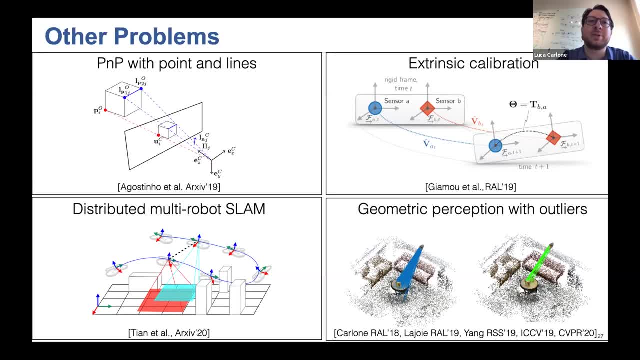 so bundle adjustment is attackable. visual interaction automatically is attackable And I think, if you're interested in that direction, David, listening to the talk from Hank should be particularly useful in understanding, like you know, how tools which are a little bit more advanced than Lagrangian duality can help design these. 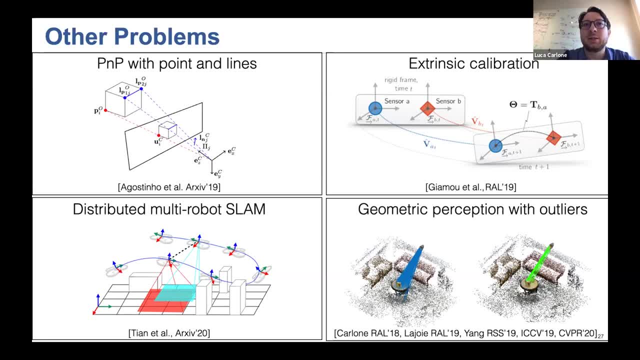 these convex relaxations. The warning you know that I give you is that remember the point from Anders about you know problem construction. So problem construction is fundamental. Not only you have to be clever in designing the convex relaxation, you have to be. 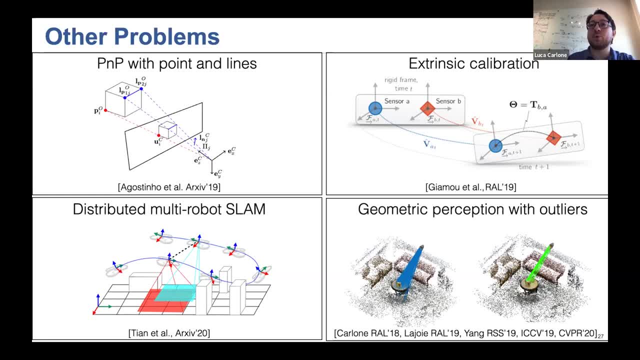 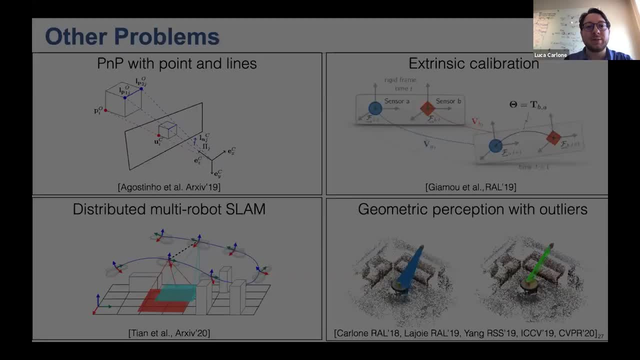 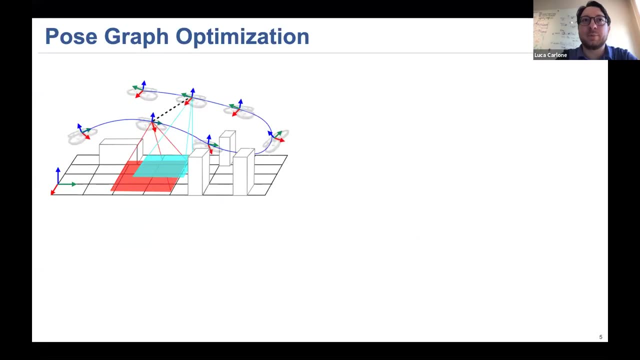 clever about picking the problem in the first place, picking the formulation in the first place. So something that I didn't mention in this talk- and I was mentioning, for example, back in 2016,- is that now we are calling these the standard formulation for postgraph optimization. 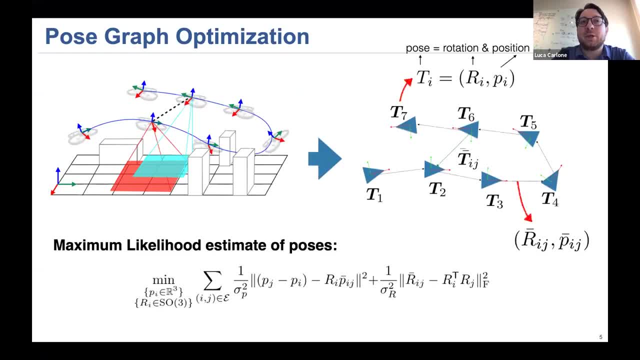 this one in the slide, But actually before. like you know, we proposed this idea of convex relaxation. was very common to use a different error for the angular, for the rotation cost- okay, So this is called the cordal distance Many people before 2016 were using. 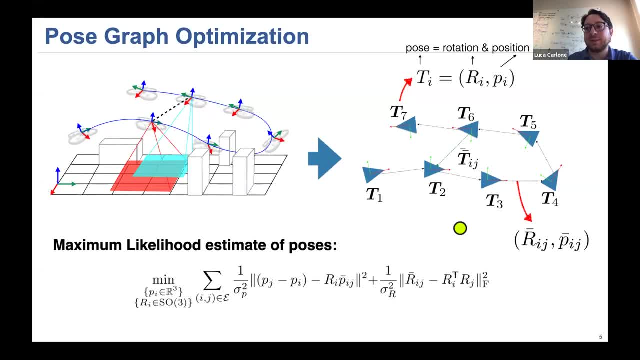 the angular distance, which is a little bit of a different mathematical expression. It turns out that you know, with that formulation was kind of very tricky to design a convex relaxation. So my invitation is to be clever about picking the cost, function and understanding. 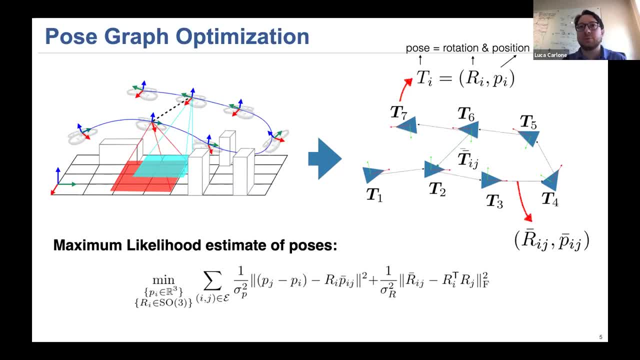 typically, when you pick a better cost function, there is a motivation for that. So, for example, we justify that for a specific choice of noise on the rotation, that's the right cost function. So try to understand what is the most convenient formulation and try to understand how to ground that in terms of assumption on the noise of the measurements. 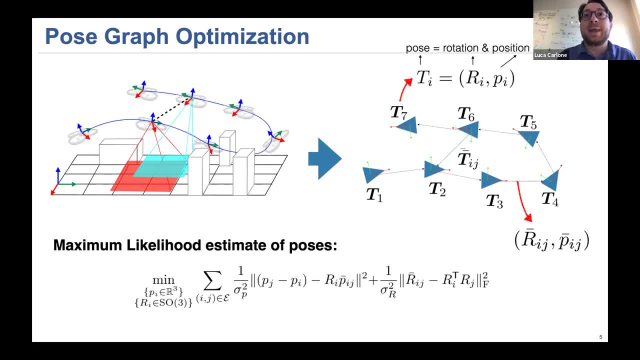 So, guys, I'm running super late here and I think there are more questions, but I will try to address these directly in the chat. At this point I think it's pretty much needed to have a five-minute break. Maybe let's start actually in seven minutes at 11.. 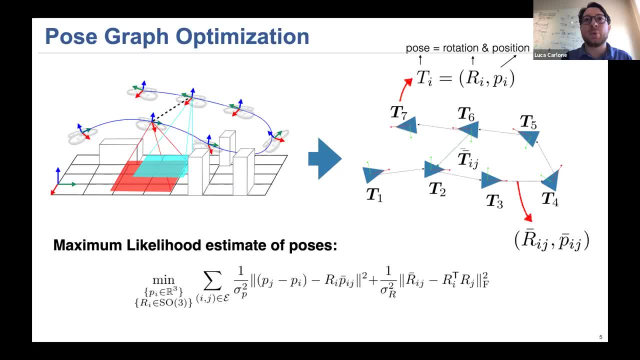 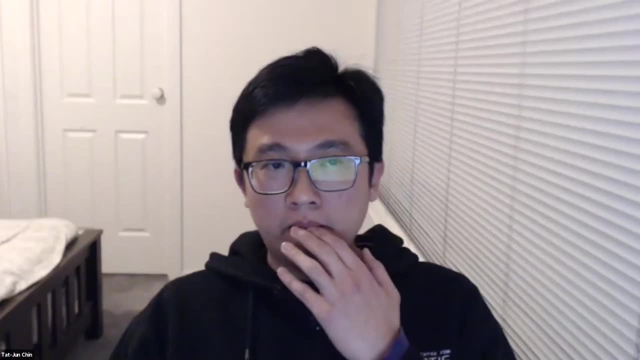 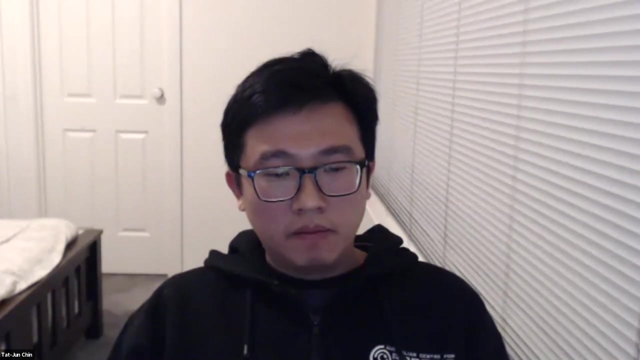 55 with TJ's talk. We are running late. I apologize when it will be long, TJ. in the meanwhile you're going to have a little bit of time to answer some of the questions that we've been asking you, So if you have any questions, please feel free to ask them in the Q&A box. 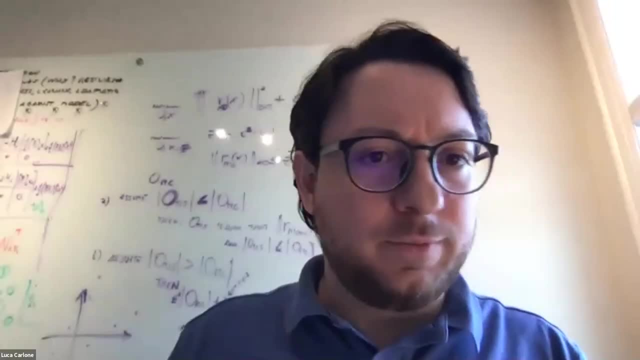 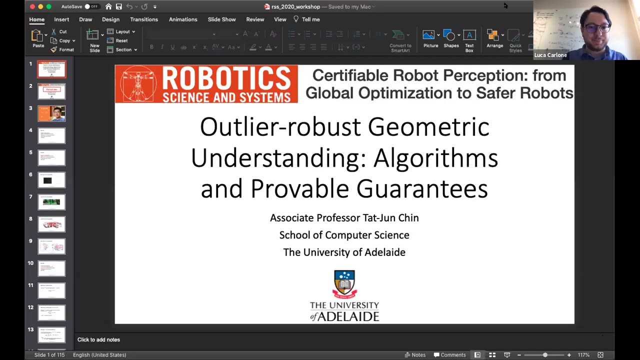 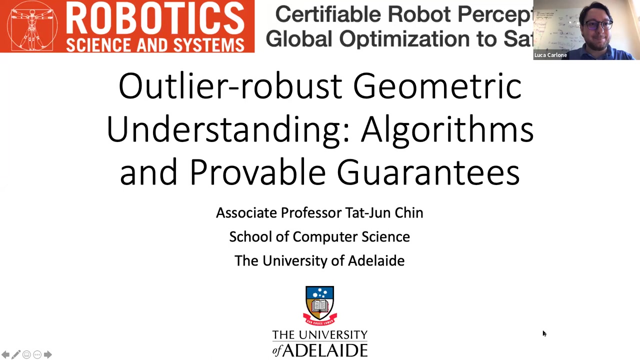 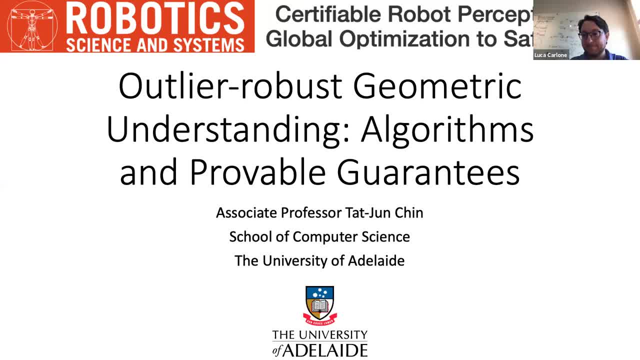 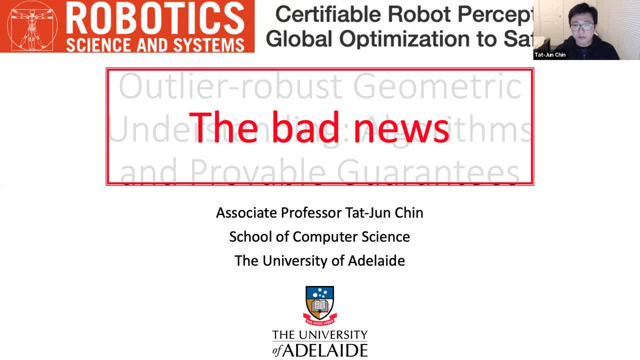 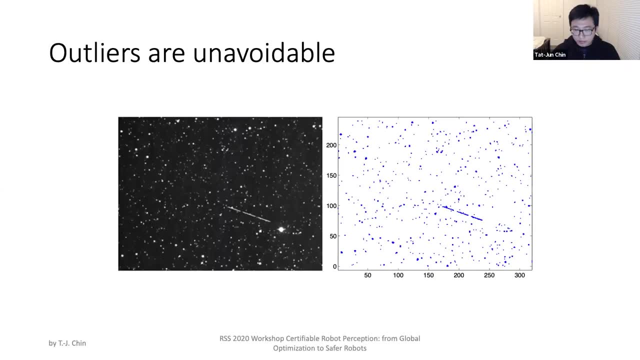 Thanks everyone for being here. The title of my segment is Outlier, Remastering, Metrics, understanding, or, as they call it, the bad news. so this is myself. everyone calls me tj. i'm from adelaide uni, so, um, you know it. it's, it's uh, not surprising, and it has been mentioned a few times. 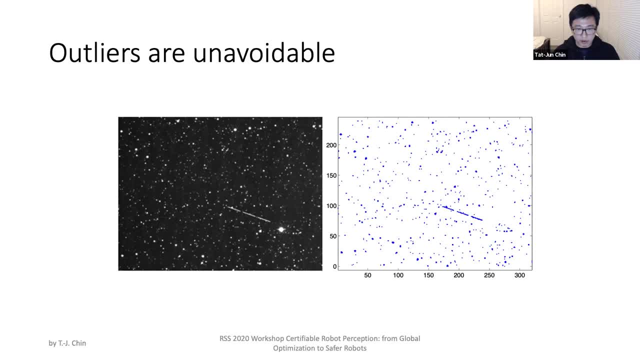 before that outliers invariably exist. this is a problem from a space problem where we're trying to detect orbiting satellites and they tend to streak, as they- because they're orbiting really fast- tend to streak when they- when they um appear in front of the camera. so the task here is to find 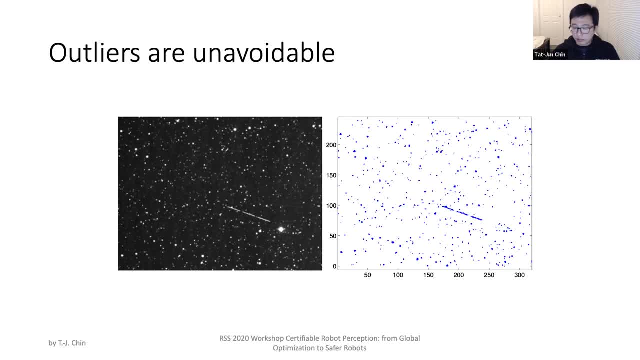 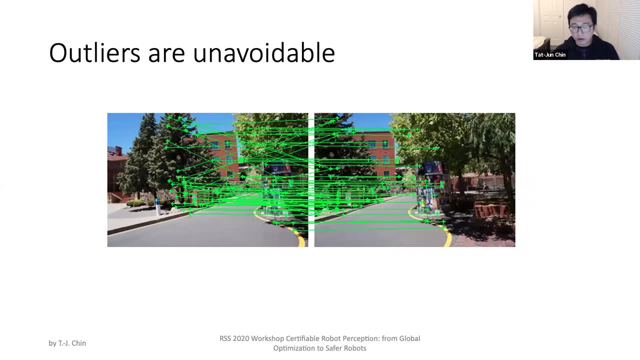 a line, uh, uh, corresponding to the streak amidst a you know a bunch of clutter and you know very standard problem in computer vision in two view geometry. given a set of correspondences, feature correspondences computed using a black box method like sift or surf, try to estimate the uh. 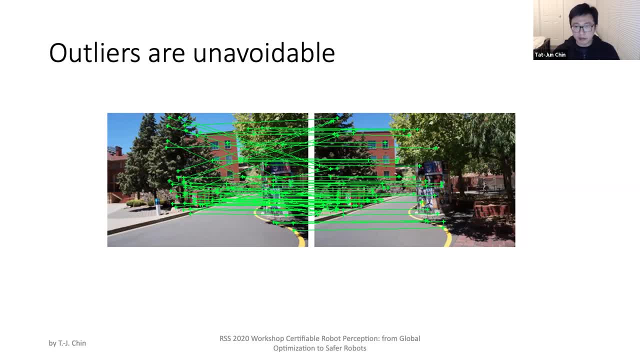 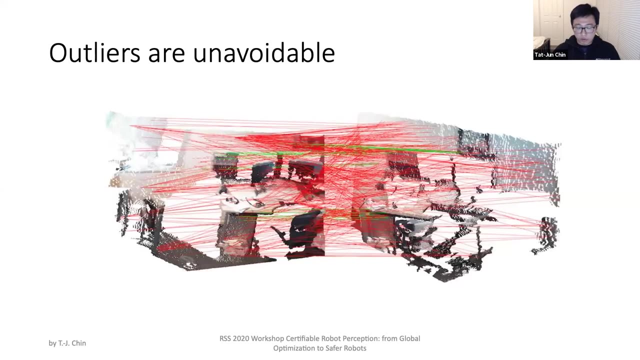 transformation, the geometric model that that you know aligns them or, uh, you know, underpins this set of correspondences. some of the correspondences will be wrong because the black box method is not perfect, thereby uh giving rise to outliers. um luca mentioned uh scan matching. 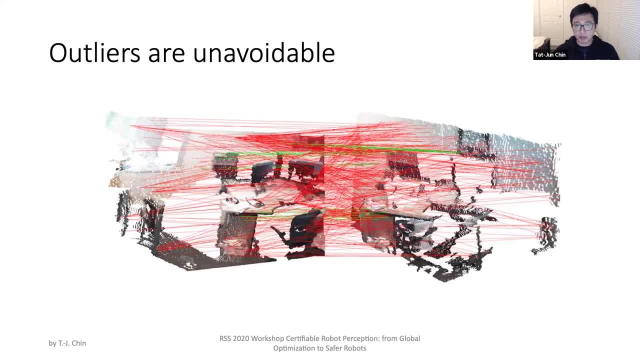 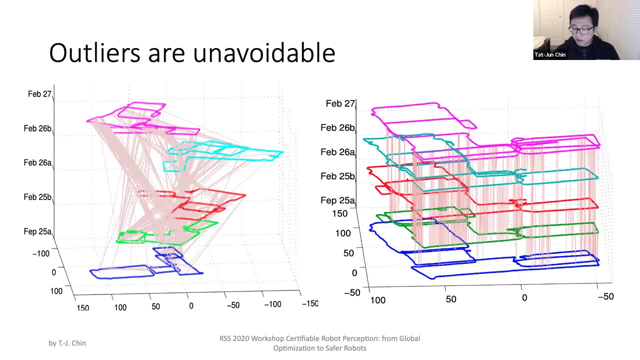 before in robotics, often we want to match 3d point clouds and again a black box feature. matching algorithm will give you wrong correspondences, which again gives rise to outliers. um in, in postgres optimization, um, we have uh incorrect constraints arising from long wrong loop closure detection, for example, so they give rise to. 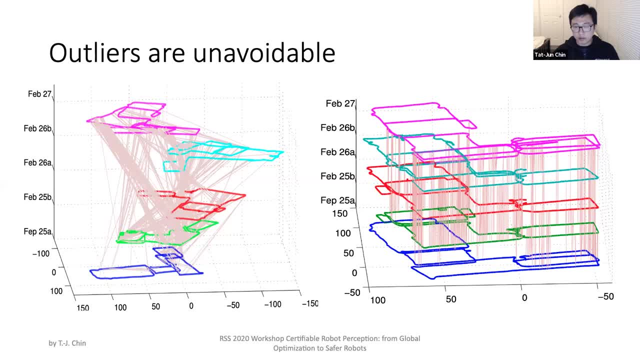 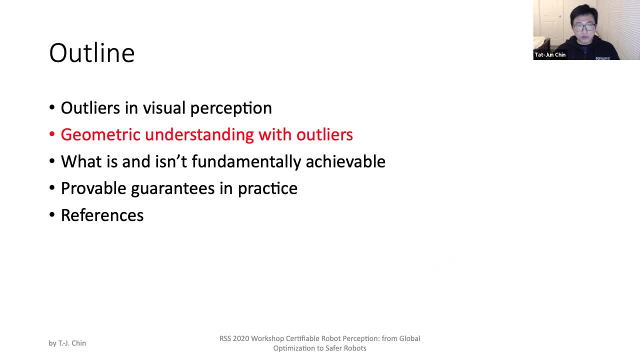 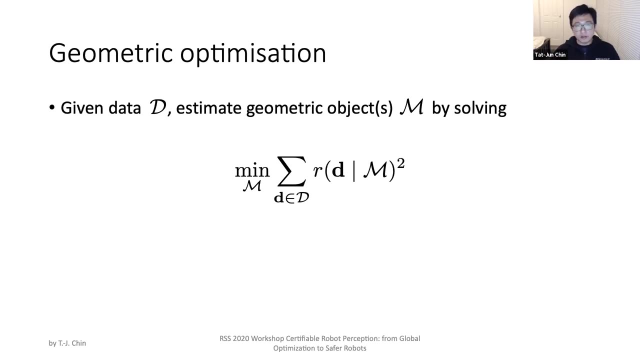 incorrect constraints, um, which again gives us the outliers in the in the formulation. okay, so a very quick intro to um. why we have outliers. now, how does that change geometric understanding on geometric optimization when we have outlines, um without outliers? normally we want to find an estimate of a model m, given a set of data, d, and we want to 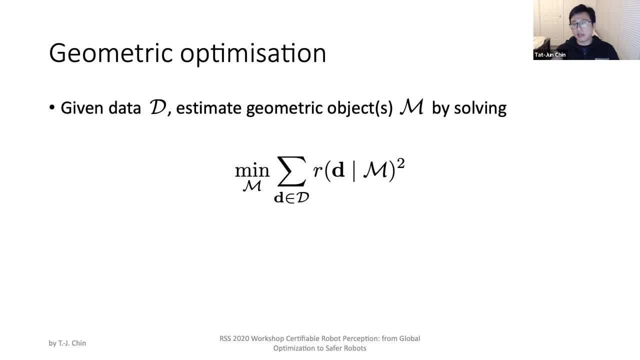 minimize the sum of some error of each data point for a candidate model: m- okay, if we square it, then this tends to be a least squares type of formulation. and r- r i forgot to mention- is residual or the error. if we have outliers, we want to avoid um, avoid the outliers from biasing the result of the estimate. 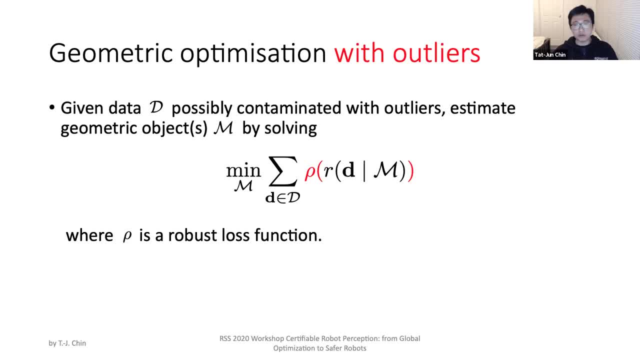 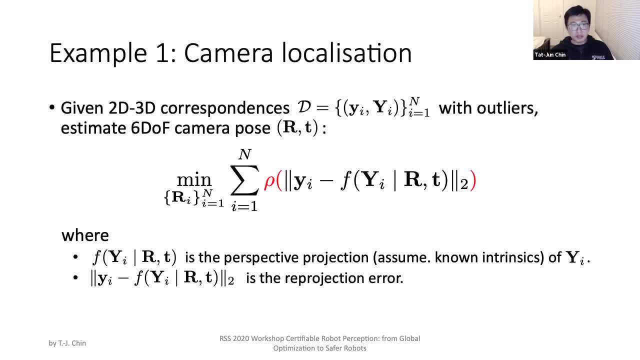 so typically we want to pass the residual or the error through some kind of a robust loss function. so example one: camera localization. given 2d, 3d correspondences with outliers, we want to find the 60 uf camera pose, rotation and translation. oh okay, i'm missing. i'm missing the rotation. and translate, translate. i'm missing the translation. 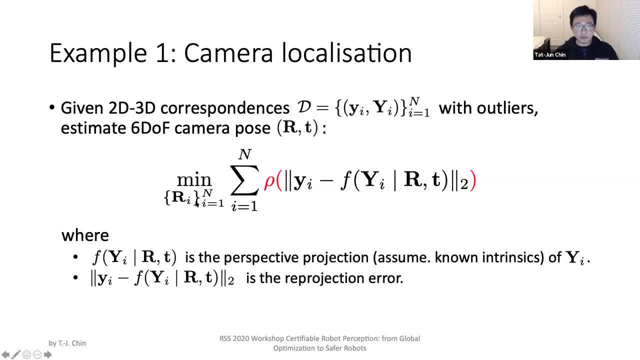 in the, in the um domain here. but you know, just imagine that there's a t there, um, so we'll minimize, for example, um, the reproject, the reprojection error, and then, if there are outliers, we want to pass the reprojection error through a robust loss function in rotation averaging. we're 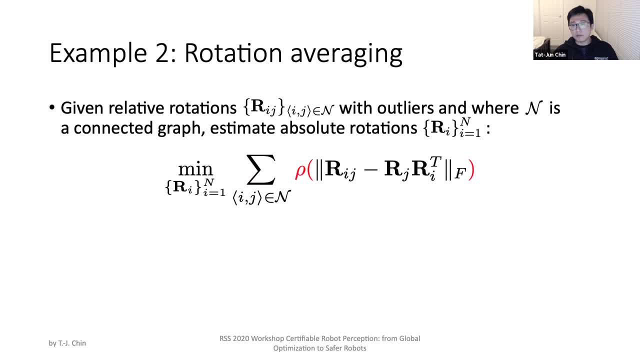 given a set of relative rotations, one estimate set of absolute rotations, using the chordal distance again. but if there are outliers, we don't want to minimize the sum of all the chordal distances, we want to minimize the sum of them, uh, being passed through a robust loss function. 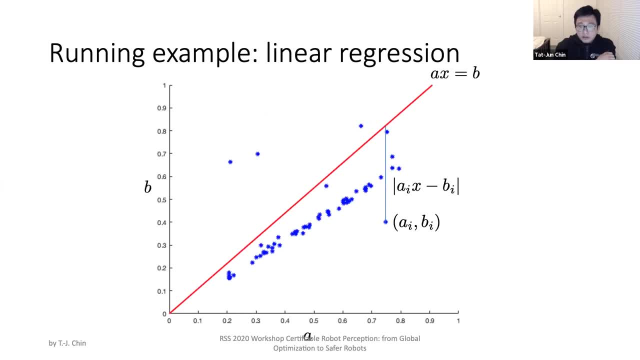 okay, so this will be a standard um, a running example in in this segment of the talk at least it's. it's easy, it's simple. i can, i can draw diagrams easily and and the results can also be more easily motivated. so i want to estimate a simple line x, um. and this is not even a line. 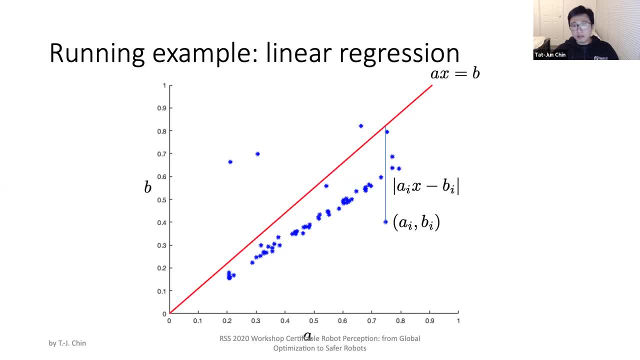 with an offset. it's the line that passes through the origin. so really it's just a direction. a x equals to b that one estimate given a set. but it's not even a line with an offset, it's a line that passes through the origin. so really it's just a direction. a x equals to b that one estimate given a. 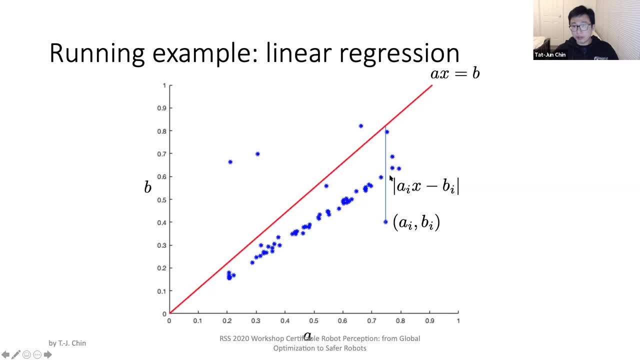 bunch of points a, i, b, i and the residual would be given by this vertical distance here between the point and the line estimate x. okay, so ideally i want to find that line x star. okay, so in a robust formulation because, as in the previous example, in the previous diagram i have outliers. 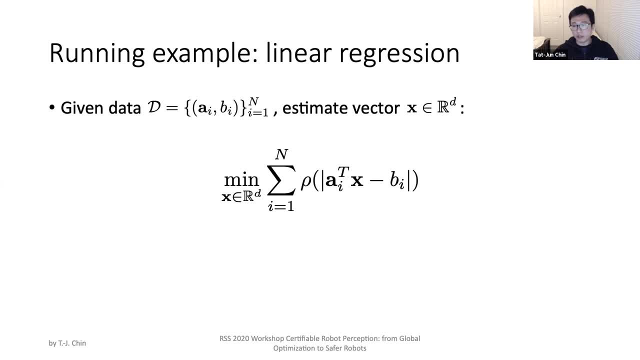 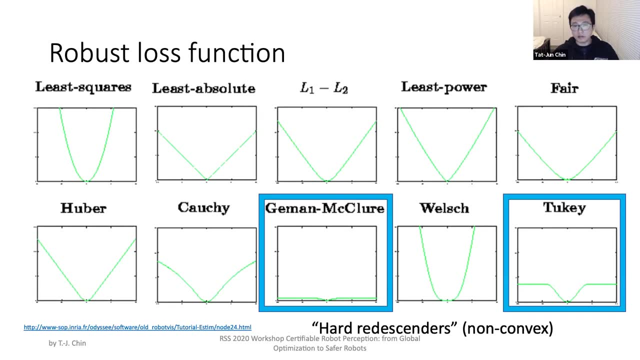 i want to pass the this vertical error through a robust loss function row and here's a a few robust loss functions that have been, you know, proposed in in statistic, in the statistical literature. all right, um, the ones that i i highlight in that blue circles are called the: 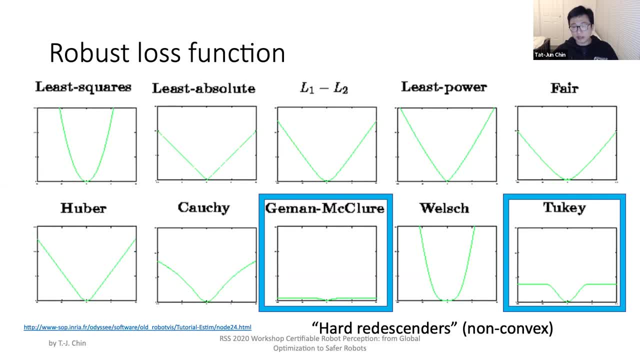 hard redescenders because, as you see, as the error goes away, further away, from zero, up to a point, um, the the loss function row starts to, uh, stay constant, they don't increase anymore, okay, um, hence they're called hard redescenders, the hard redescending robust. 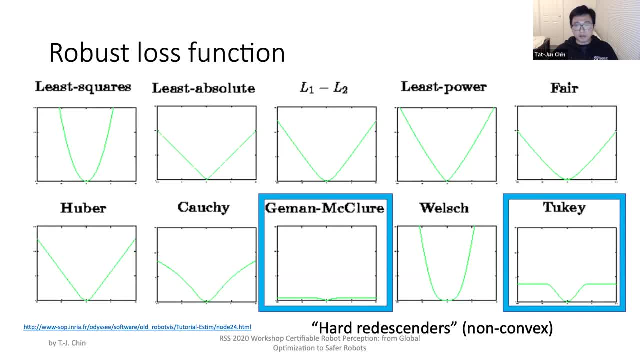 loss functions are non-convex and that's necessary because, uh, we want to absolutely limit, we do not want the outliers to limit in, we do not want the outliers in any way to bias result of the estimate. so if it's a normal l2 function, a row, the robust loss function is normal. 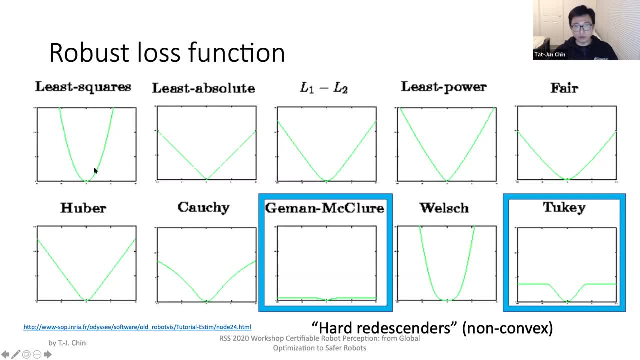 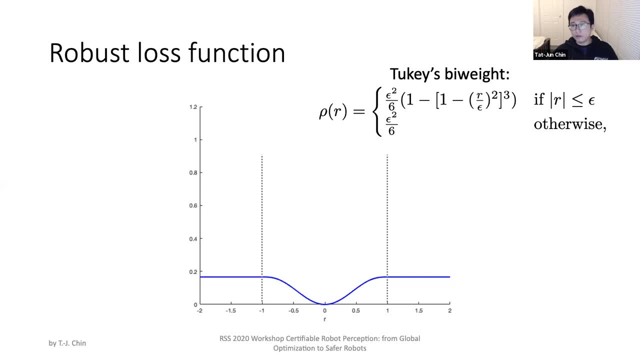 l2 function. then we revert to the normal least squares, which, as we know, is not robust. okay, so here's a hard redescender. it's called two keys by weight, which, yeah, it's, it's the the last one here. um, that's the method maker formula for it. um, it's kind of like you can, you can, imagine it. 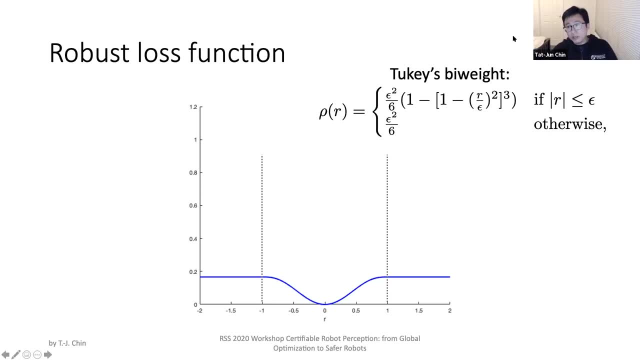 and some kind of a truncated l2, but it's not. not really if you can see the definition here. but you can imagine what it's doing here. it's. it's allowing the inline points to, to to influence the estimate, but the outlying points after a certain threshold stops uh. 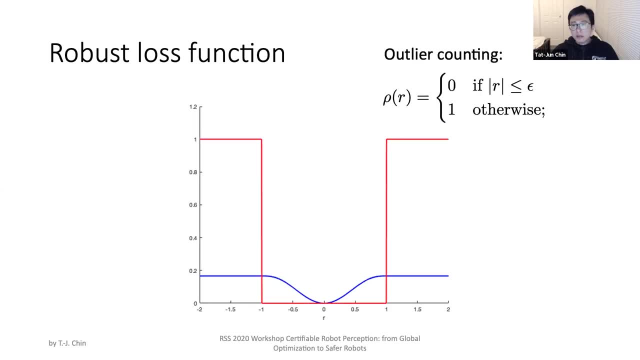 influencing the, the estimate in in computer vision and in in robotic vision. we we often use this kind of robust loss function. um, it's simply counting the number of outliers, okay. so instead of paying attention to how much the error is, we just want to count how many points are within error with. 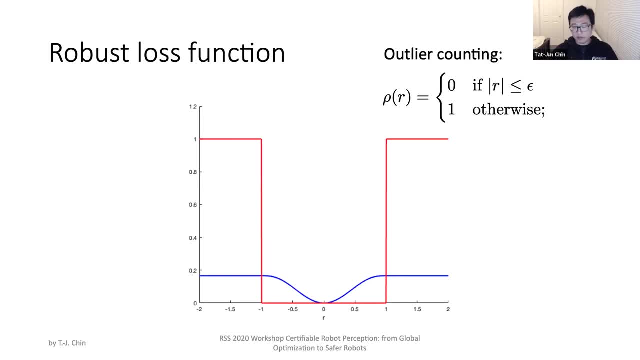 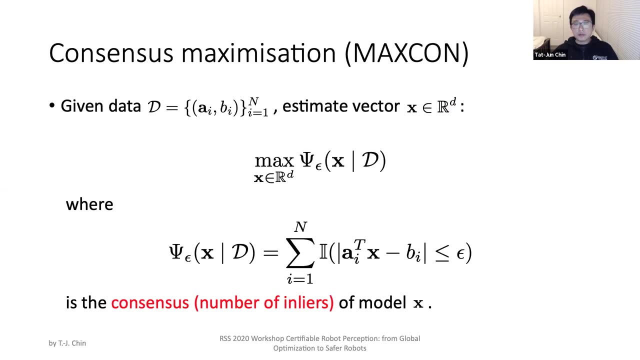 error within the threshold. how many, sorry, how many points are outside of the uh threshold? one in this case. and this gives rise to what we call the consensus maximization formulation, which is often used in computer vision and robotic vision. um, so we're going to count, given a bunch of 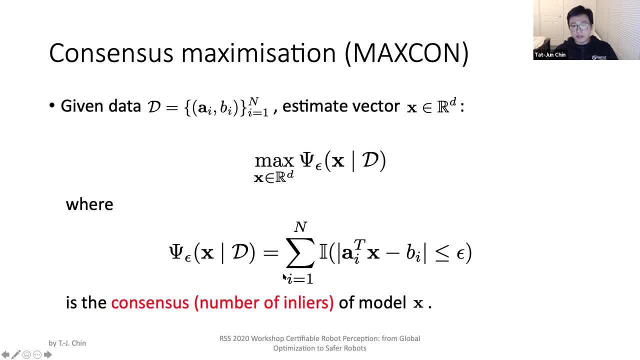 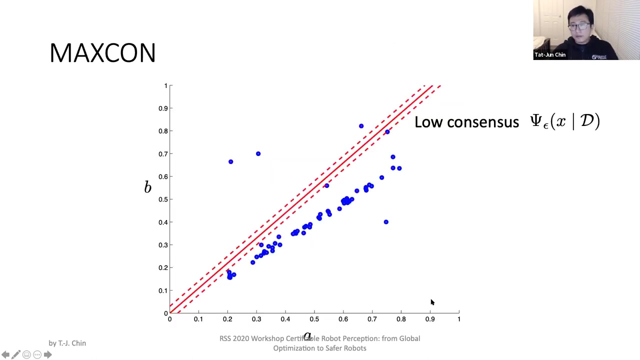 points, estimate a model x, but estimate x such that the number of inliers are maximized. okay, so we find number of points such that its error with respect to the candidate x is within a threshold epsilon, and this indicator function simply counts them, and that kind of inlier is called the consensus of a candidate model x. okay, so, um, back to our 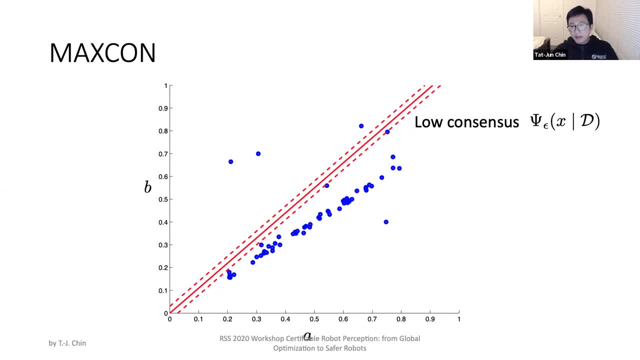 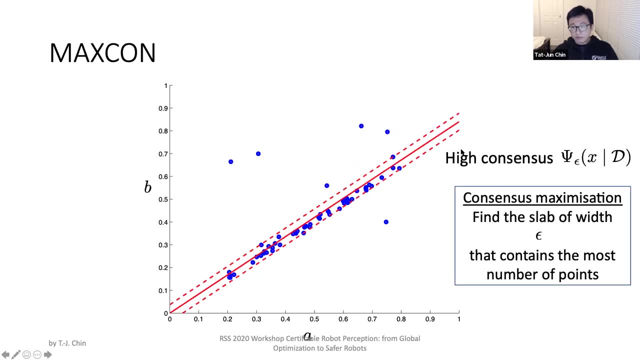 running problem. uh, if, given candidate x, this has a low, low consensus because it doesn't have a lot of inliers in it and therefore it's not a good fit. what we want to find is this line where it has the most number of outlines. so, essentially, find a slab epsilon or fixed with epsilon that contains the 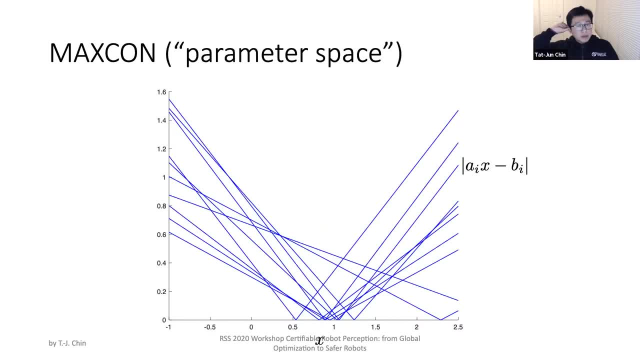 most number of points within the slab. okay, so another point of view of the same problem is: we look at it in the so-called the parameter space, right? so in the x-axis here, in the horizontal axis, here, that's the, the parameter value x that we want to find. every data point, a, i, b, i, you can plot it in this parameter space. so every line here is: 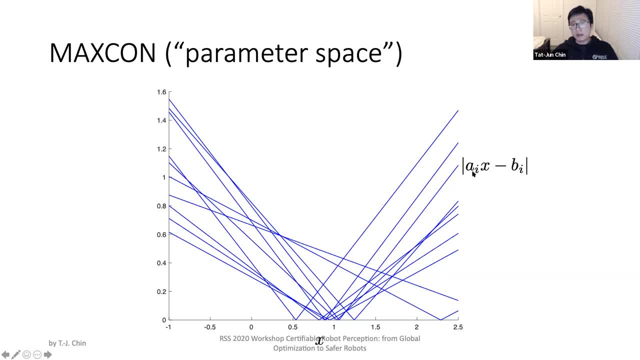 the residual of a particular point given any candidate x. okay. so you know, if we have a bunch of points, then we have a bunch of v curves that look like this. so the consensus maximization or the maxcon problem is i we're only willing to tolerate. 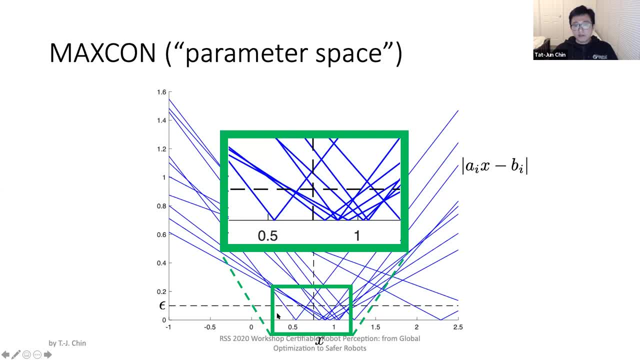 an error of epsilon, that's the so-called inlier threshold. find me the x such that as many of the points line lies, as many of the v curves lie below the line epsilon as possible. okay, so, for example, if my x is here, then i count that there are exactly three points or three v curves that lie below. 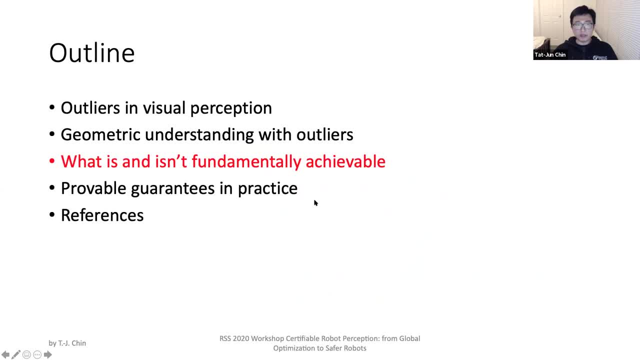 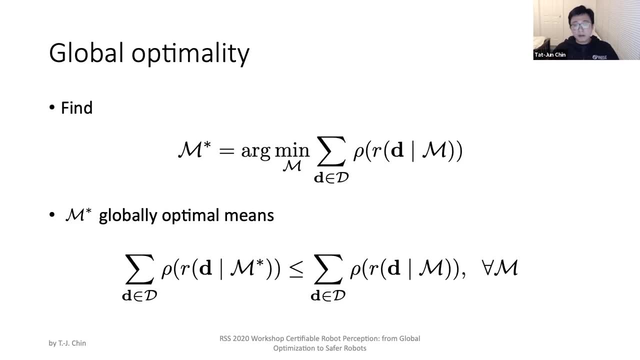 epsilon in this x, and therefore the number of inliers is three in that example. all right, so quick definition of a particular robust formulation. what does it mean when we say we want global optimality? that means that we want to find the model m star or the model parameter m star, such that 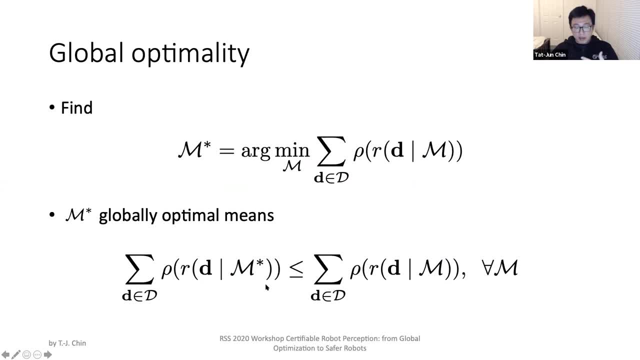 no other model is is. is has a. has a lower objective value, okay, has a lower robust objective value, all right. and that's what we mean by a global optical solution, and immediately, because we see that rho, for example, the heart redescenders, or that inline outlier counting objective function. 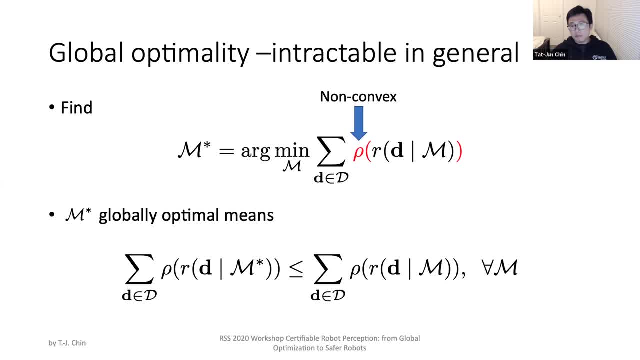 that i showed earlier, because they are non-convex. immediately, we know that this problem is intractable in general. right, and really there is nothing much to say beyond this point. remember, in anders's segment there are two, two ingredients to make a problem tractable. first, the objective function has to be. 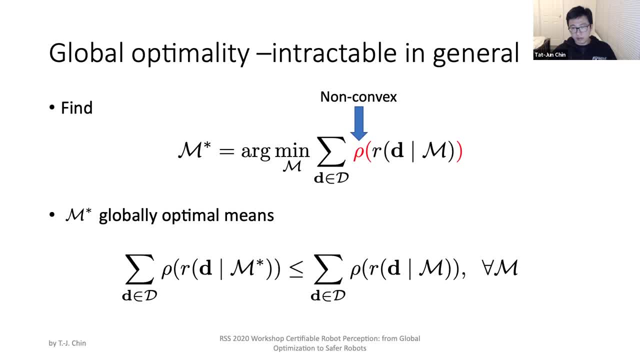 convex. second, the optimization domain has to be convex. okay, in the previous talk by anders and luca on relaxation, it was mostly about making the optimization domain convex. the objective function to begin with was convex, so there wasn't much of an issue. but when we have outliers and we want to ignore, 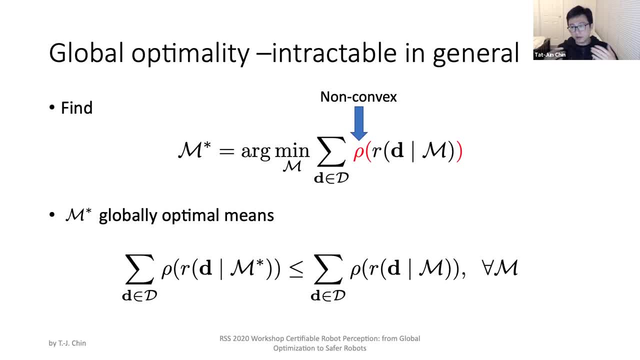 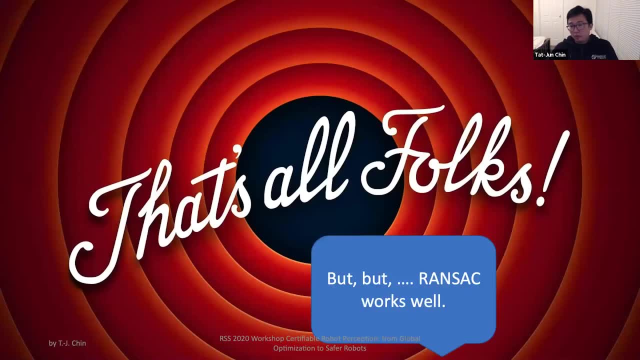 outliers, we will use hard redescenders. there are non-convex and that basically means you know it's empty heart. to begin with, some of you would say: you know, but ransack works well. what are you talking about? yes, ransack works well usually. what is ransack? let's recap a bit in the running problem. 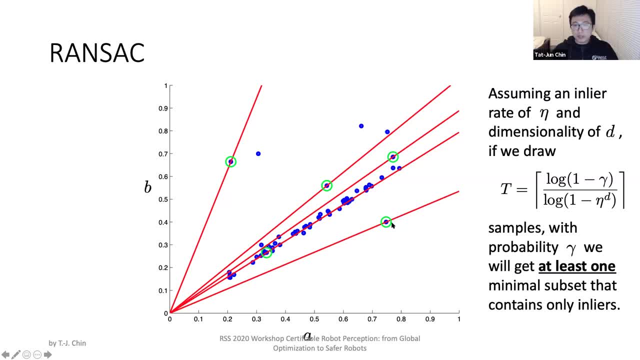 here. so it works like this. so it's, you know, with the extent that it's a penso, that you can use linear tops or linear sets of ones. you can use linear tops, you can use random sets of ones, so you actually have like a whole set of random sets of different weight sets, a set of random. 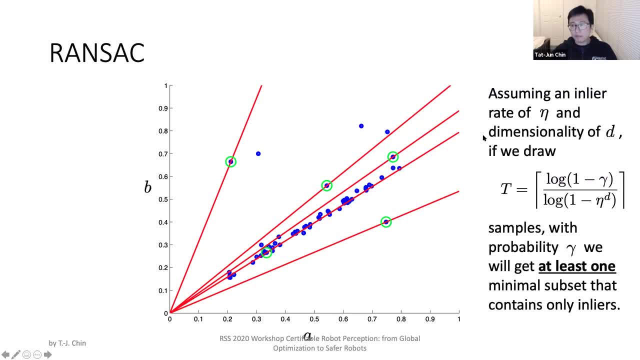 sets of random sets of random sets. so there are some ways that you can do it and it may depend on the type of output you're using. so you can use linear top, but also you can try to use linear multiple sets of random sets and you can try to do it with a. 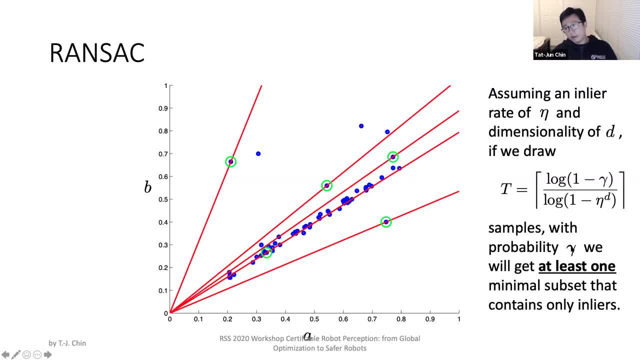 random number. you can, because when you drawส and a it's going to decrease your probability in pso of you think the variance of the number of random sets you're going to need to do is to draw a higher range of. with probability gamma you get at least one minimal subset that contains only inliers. 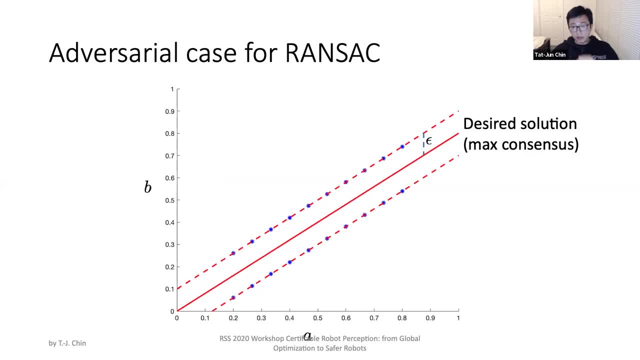 Okay. so what is the problem with that? Well, here's an adversarial case for RANSAC. Maybe adversarial is the wrong word to use for it, but you know it's popular these days with deep learning. Adversarial case for RANSAC because why? Why is it an adversarial case? 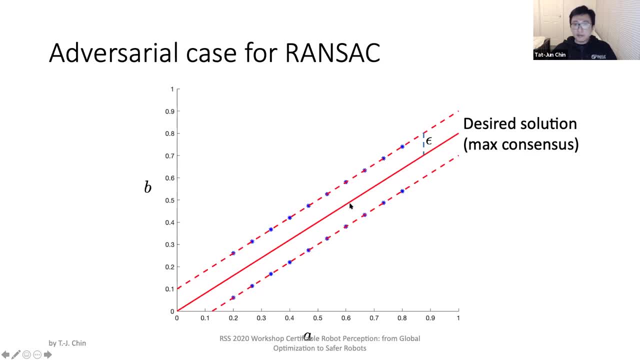 Well, you can see that this is an estimate, you know, with the inline threshold epsilon, that captures all the points in the consensus. sorry, in the epsilon band, but that estimate does not pass through any of the points. These are two estimates, or two minimal subsets that a RANSAC algorithm would sample. 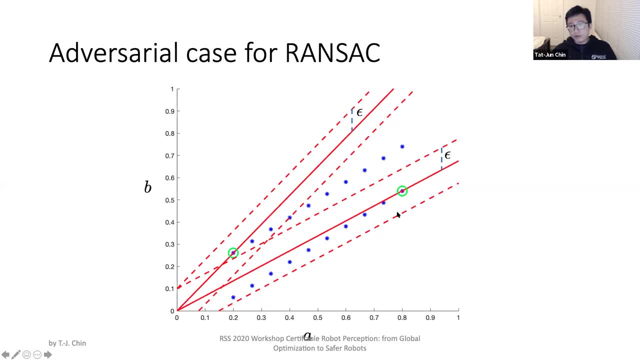 but you know, none of them give you these two, don't give you a good estimate for that line we want. and if you can try, you can try all the other points, other minimal subsets, minimum estimates. none of them will give you good estimates. 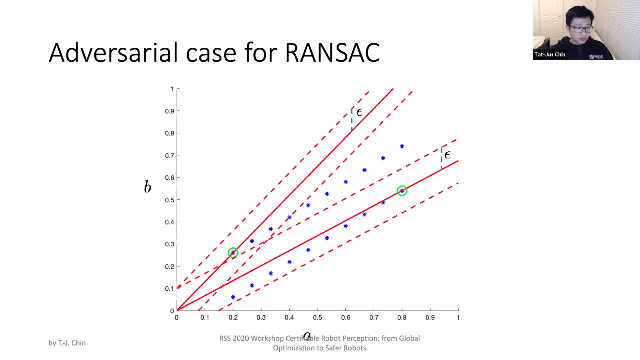 Okay. so yes, RANSAC works well in general, but this talk is about certifiable global optimality for safer robotics. What we worry about is not when RANSAC works well. what we worry about is when it doesn't work well. you don't know why. 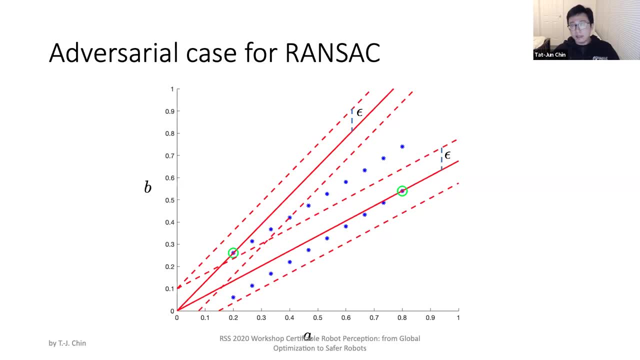 you don't know if it's because you've been unlucky or because there are no good solutions to be found. Personally to me- and I think with my co-organizers as well- for this workshop, that's not a satisfactory solution. When it doesn't work, you don't know why. 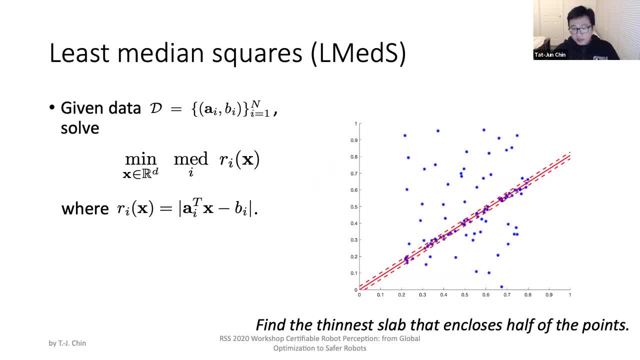 Okay, so okay, fine, we said it's already non-convex, it's empty heart. what is bad? what is more to be said about this? What is it? Well, I mean, if you dig deeper into it, there are actually interesting results we can make as well. 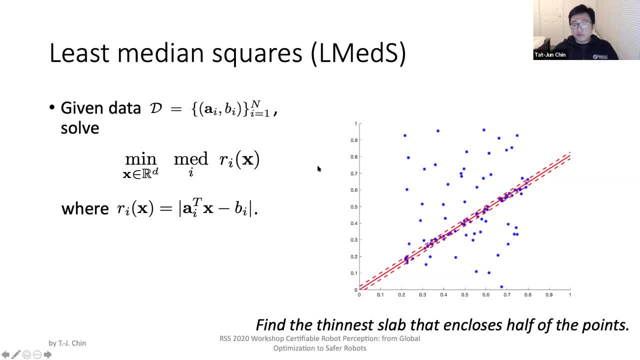 So, before we get there, let's look at a problem that's related to RANSAC. eventually will be related to the consensus maximization problem. these median squares Given the same number of same setup, instead of minimizing the count of outliers, we minimize the median of the residuals. Okay. So geometrically or intuitively, it should be well-safed, but in general it is well. it is not known available. Okay, so we still have our results. we have the PQR. let's look at the current data. 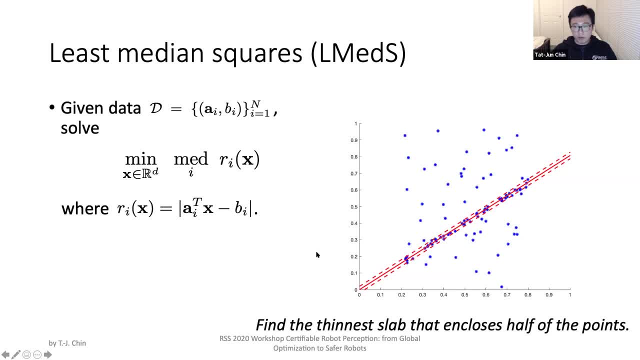 Okay, so here's the time limit. we have the peak time limit and here's the medium time limit and here's the zero time limit. it's find the thinnest slab that encloses half of the points. We can generalize that a bit and says: 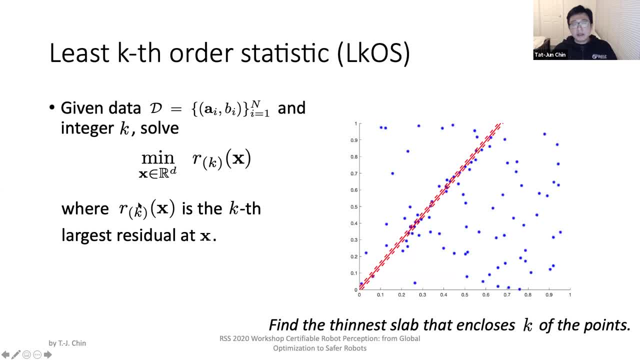 in the problem called least kth order statistic. LKOS find the thinnest slab that encloses k of the points, So R in brackets. k here means the kth largest residual given candidate X. okay, So in the previous slide 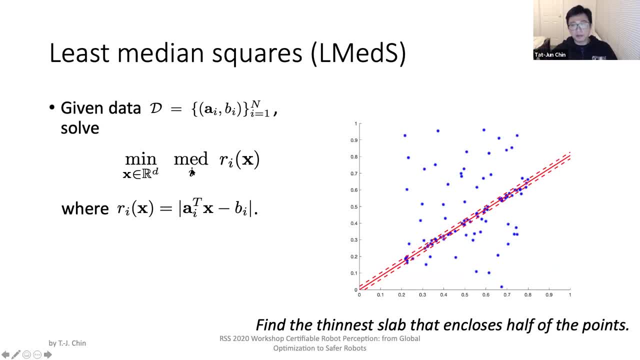 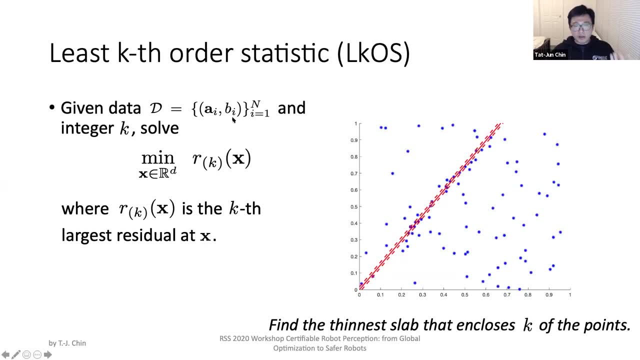 we just take k as half of n. all right, This is generalizing it, saying k can be any number between one and n. So, given any candidate X, we sort all the residuals. we find the one that's the kth largest okay. 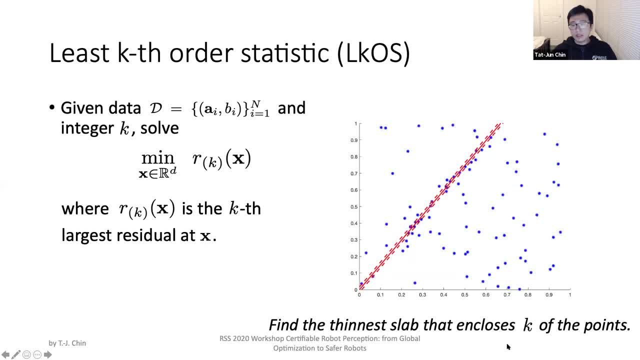 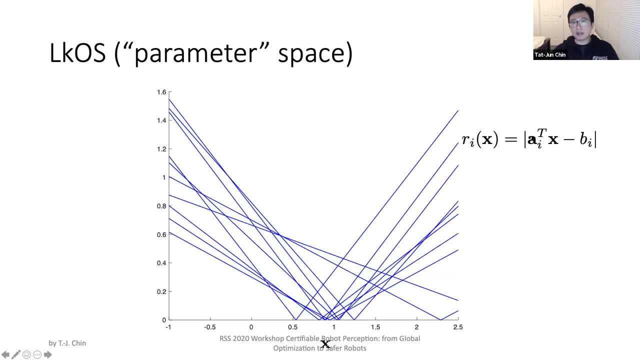 And we wanna find the X that minimizes k, largest residual Geometrically. this is finding the thinnest slab that encloses k of the points. Cool. so how does it look like in parameter space? this LKOS Again. remember that we said earlier. 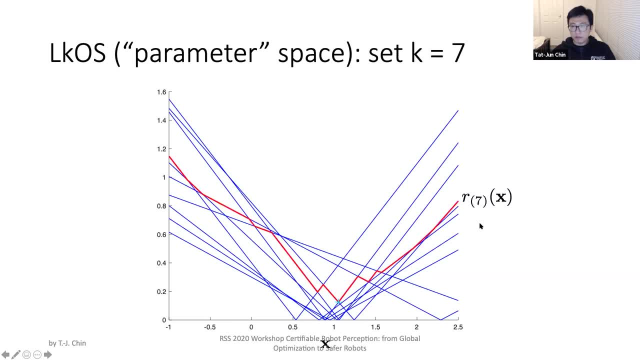 each data point gives rise to a V curve. At any X, we can sort the residuals and we find, let's say, the seventh largest one right. So for this X here, remember, X is a point on the horizontal line, horizontal Exes. 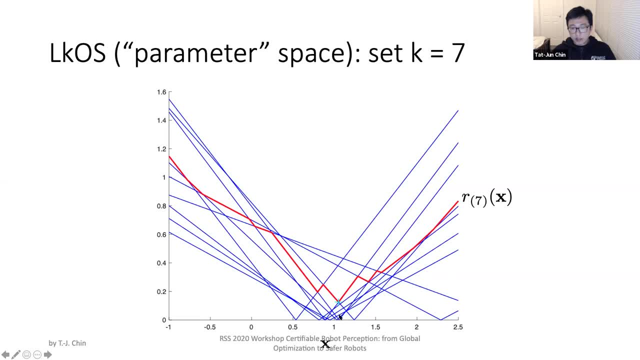 For this particular X. here we count which is a kth largest residual and it's given given by that root point there or cyan point there. okay, If we check all possible Xs and find the K-largest residual, they make up that red line there, okay. 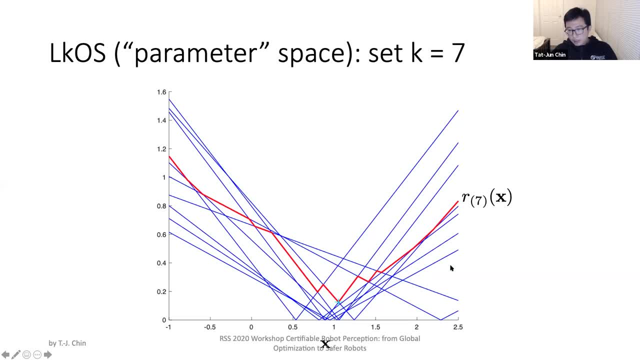 So you know, take any X, count all your way up until the seventh. it's where that red line is all right. So that's the objective function R in bracket seven. Okay, so what are we trying to do here? 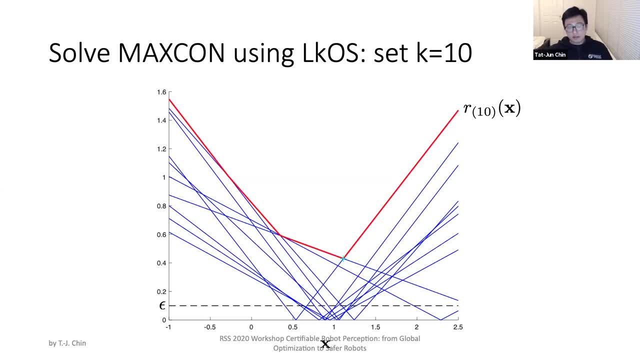 So let's say, we know how to solve LKOS. okay, Let's say, if I give you any K, you can always find that cyan point. okay, You can always find the minimum point on that line there, the red line. 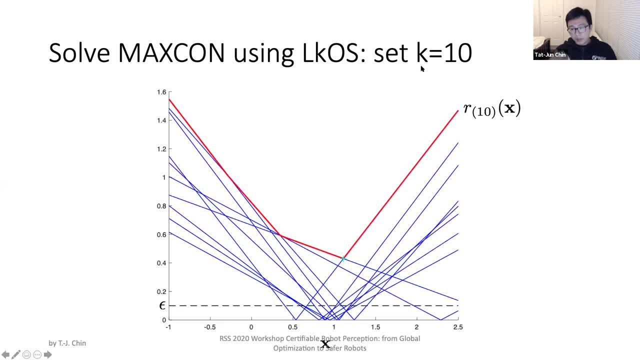 If I change different K, you can still do it, Assume that we have a black box algorithm that allows us to do that efficiently. And for K: K equals to 10, that's where the cyan point is. For K equals to nine. that's where the cyan point is. 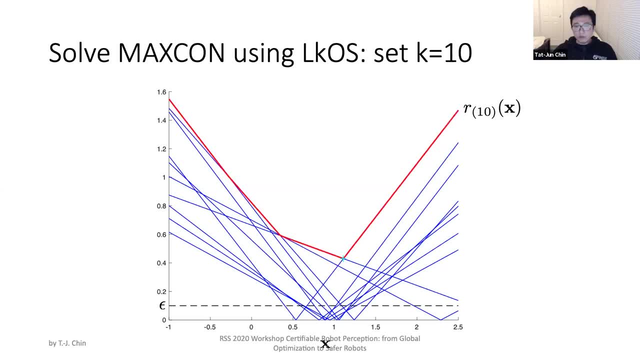 All right, so let's say we can do that Now. if we can always do that, then we can use the black box that solves LKOS to solve actually our target problem, which is a consensus maximization problem. okay, So how do we solve it? 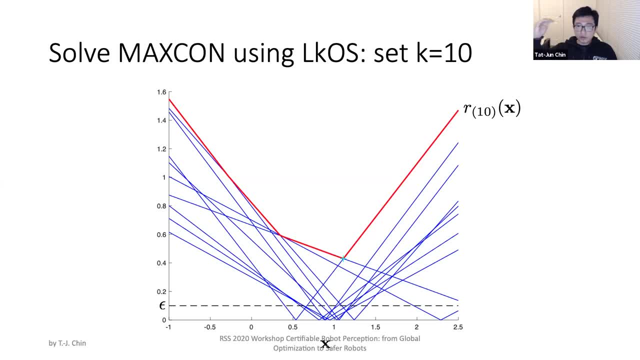 Well, we just iterate through K from K equals to N, 10 in this case- and keep reducing Every time we find a solution of LKOS for that particular K. if that solution is below epsilon, then we stop okay. 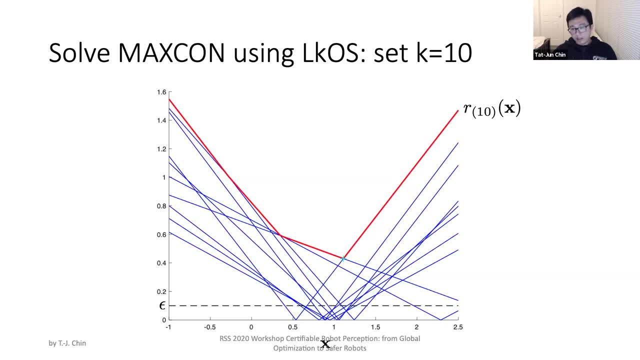 So this is what we do Again: K equals to 10, find that cyan point. Is it below epsilon? No. K equals to nine. is it below epsilon? No. Is it below epsilon? K equals to eight: No. 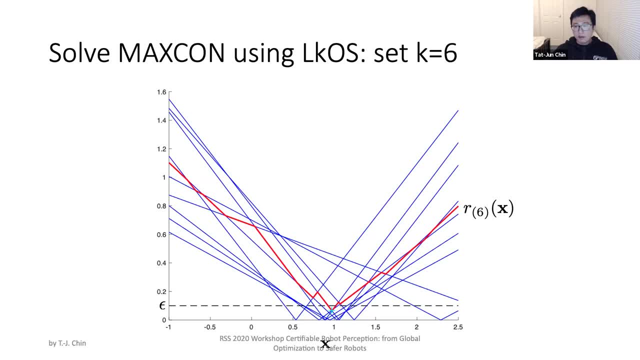 We keep going until it's below epsilon, Then that also actually says: hey, this is the point X where the most number of lines lie below epsilon at that point okay. So for this particular problem we know that we can solve the maximum consensus solution. 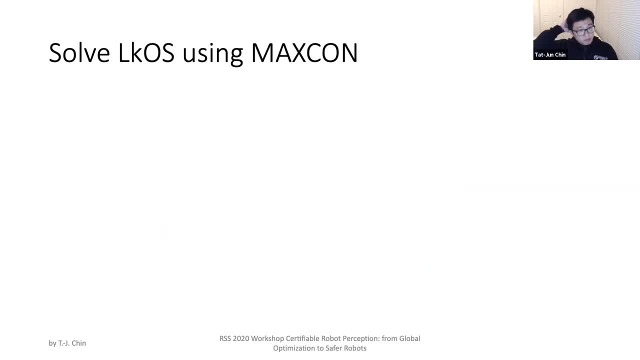 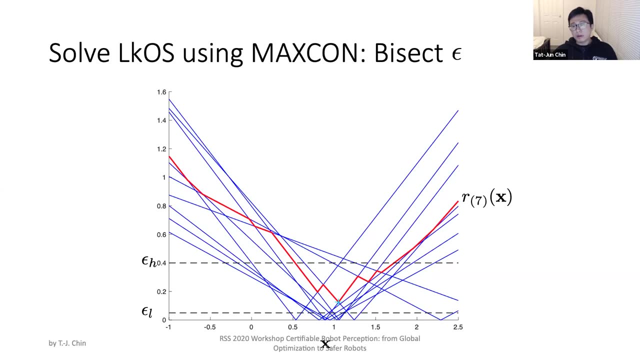 with six inliers. All right, so let's flip the problem over. Can I solve LKOS using Maxcon, Assuming we know we have a black box routine that can solve Maxcon? for whatever epsilon we provide it, it can always find the line. 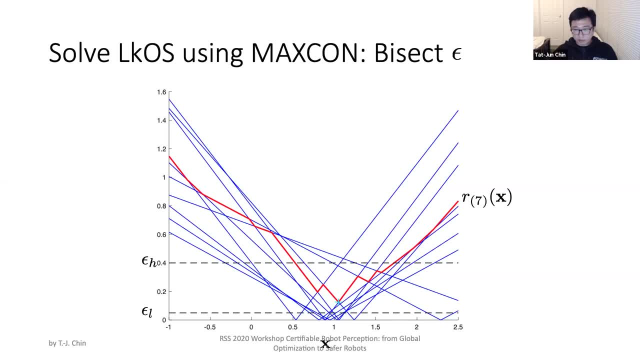 that contains the most number of points in that epsilon slab. So I could try different epsilons. In fact I could do bisection: start with a big range for epsilon and keep halving the interval Every time I have a specific epsilon range. 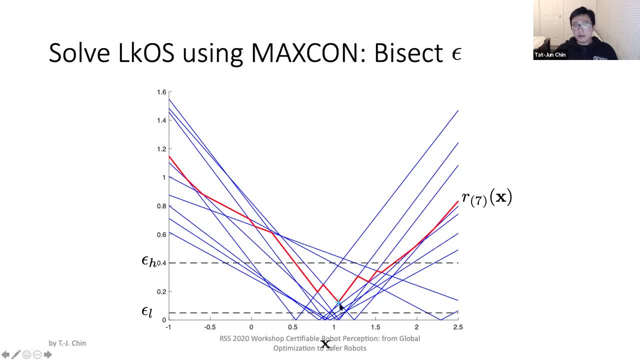 I check in the middle, can I find a X that contains the most number of inliers. And what is that number? Okay, so I keep going until that number is the number I want for the LKOS, let's say seven. 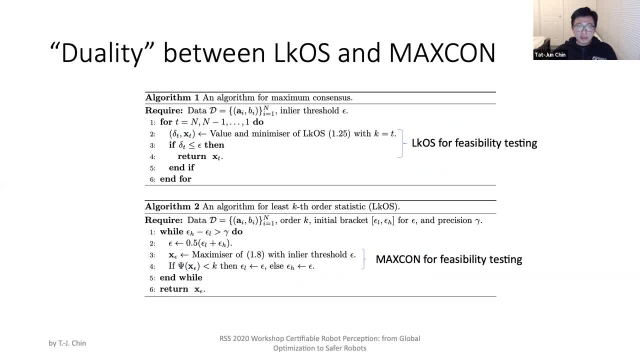 then I would have found the solution. So what this is saying is that if we know how to solve one, we know how to solve the other. If we know how to solve LKOS and Maxcon, if we know how to solve LKOS, we know how to solve Maxcon. 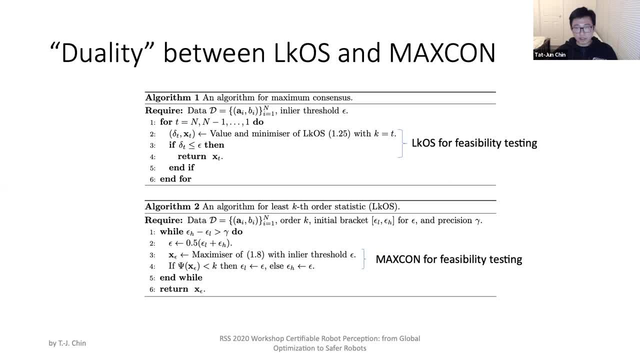 If we know how to solve Maxcon, we know how to solve LKOS, So the problems are kind of dual- dual in a different sense. that was mentioned in the two previous talks- And since we don't have efficient algorithms- polynomial time algorithms- for either of them, 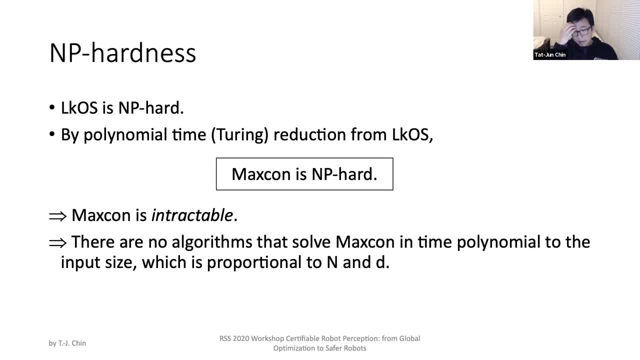 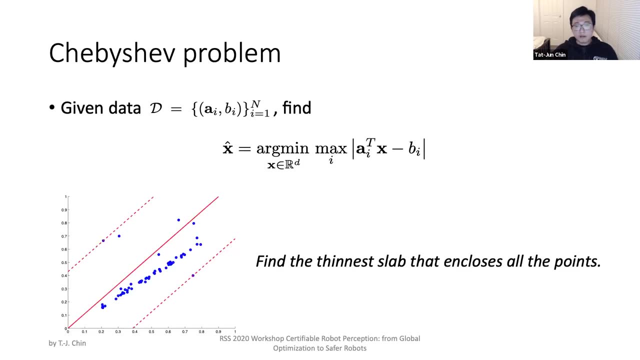 that means that both of them must be difficult, So that's a hand wavy, quick way of saying. this is an NP-hard problem, which is not surprising. to begin with, as we said, the cost function is non-non-convex. 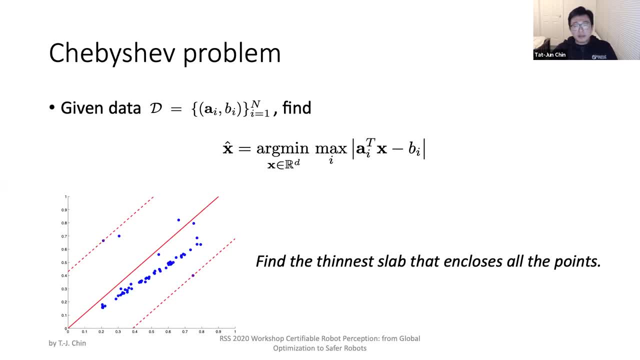 So we can push this further and say, hey, let's say I solve a different problem. First, I'm minimizing the max norm. This is a different name for it, the Chebyshev problem. Find the thinnest slab that encloses all the points. 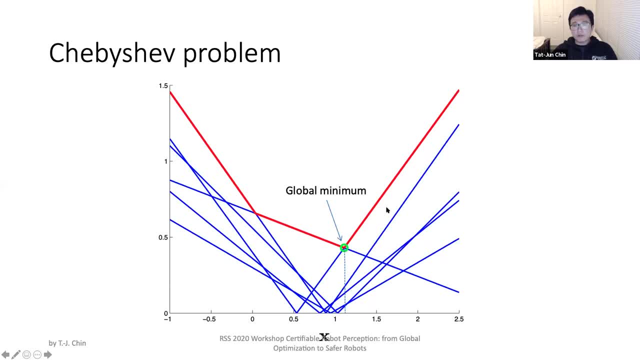 So Anders kind of mentioned this. So this problem is always solvable, because now the V curve is equivalent to setting K equals to N for LKOS, And I can always find the global minimum because that top line there is always convex, So I can solve it using a convex routine. 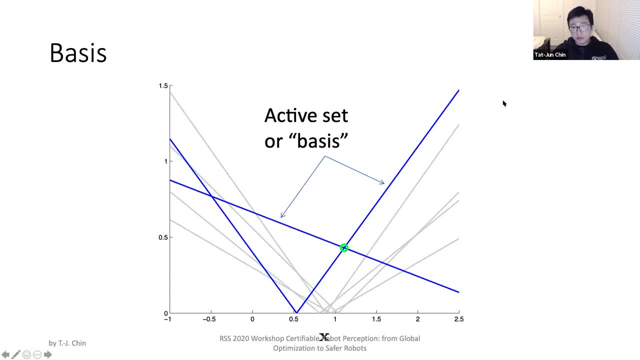 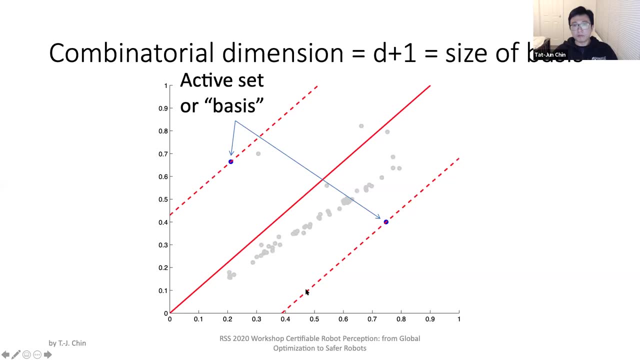 And in fact you can observe other things, interesting things about the solution as well. It's always supported by two V curves here in this one dimensional problem. So these two V curves correspond to two active points, or what we call the basis of the problem. 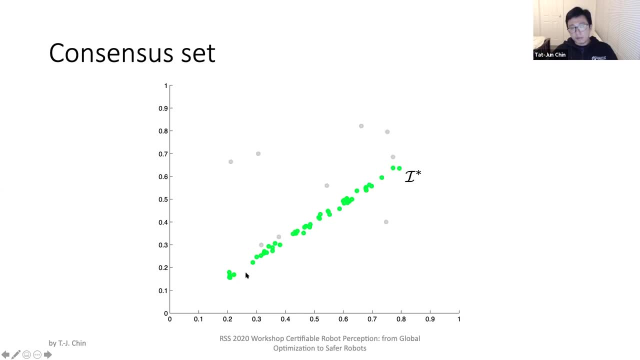 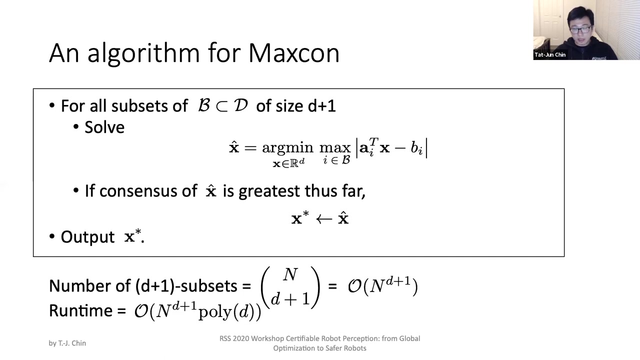 And, in fact, this inliers set that we're looking for. you can also find the basis for it, So this always exists, which provides us a solution for MaxCon that looks like this: We just simply sample all these active sets. And for linear residuals like this: 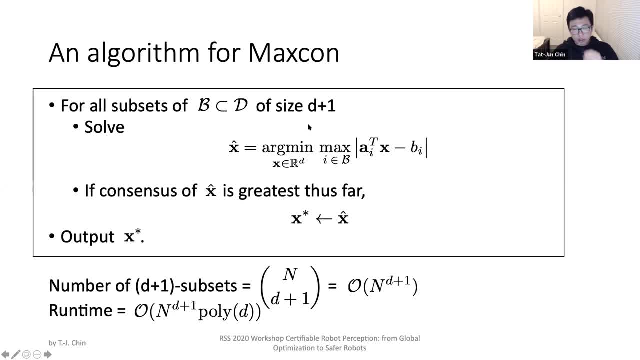 you can show that the active set is always size d plus 1.. You generally enumerate all of them And we have an n to the d plus 1 solution. There's a polygons, So you can see that Poly d there, because every time we sample a d plus 1 subset. 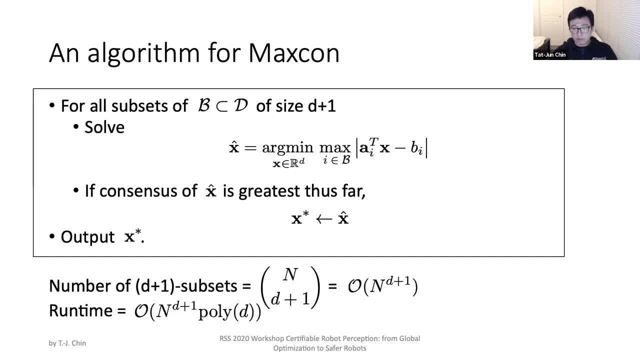 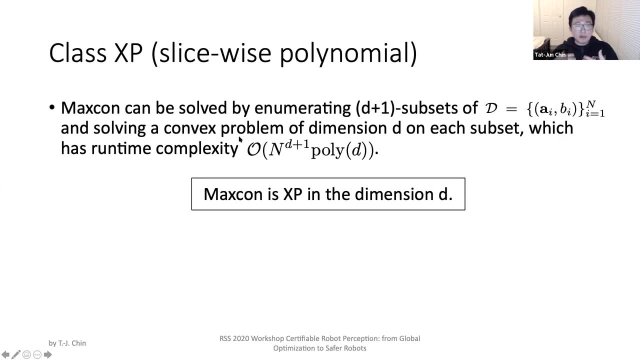 we need to solve the Chebyshev problem. So this means that we can solve MaxCon in time. This means that MaxCon is in class XP or slicewise. polynomial Meaning that if you fix the dimension the problem actually becomes polynomial time solvable. 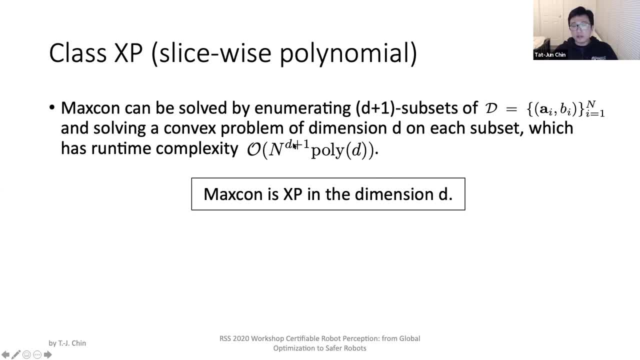 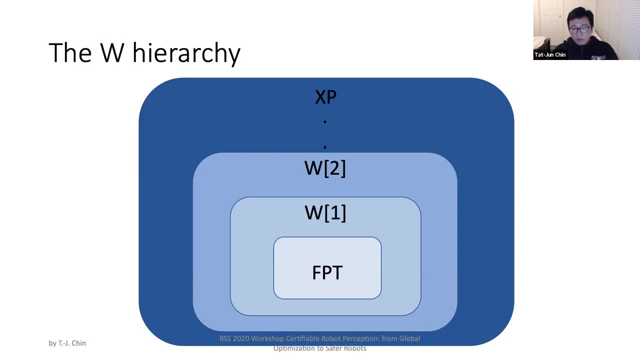 But it doesn't mean that it's easy to solve, because d is actually part of your Part of the variable part of the input size. So it's still exponential. But now we're exploiting the structure of the problem. What we're trying to do here is to push further than that. 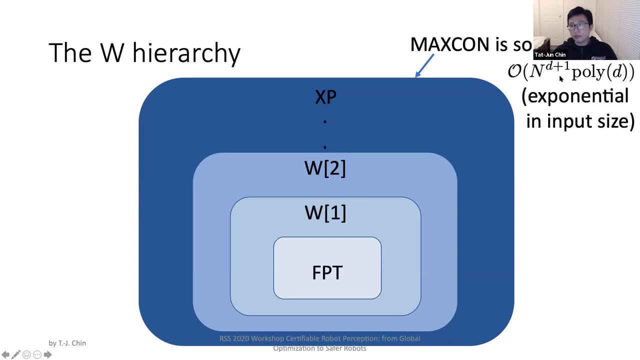 Can we do better than exponent in d If it's already in class slicewise polynomial? we wanna ask the question: can we remove the dimension from the exponent, put it in front in an arbitrary function f okay, So if that's possible, 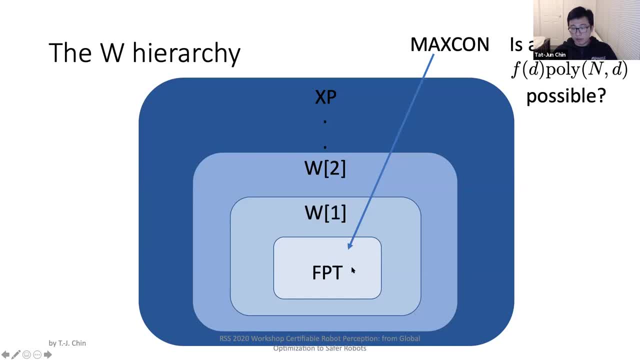 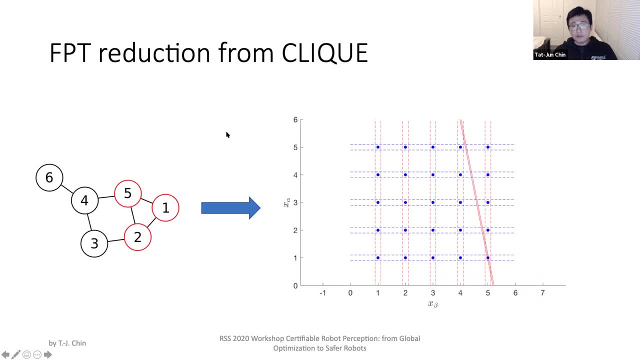 we would say that Maxcon is in a class- fixed, branded, tractable- So unfortunately I'm not gonna go through the detail here. it's quite involved. You can show that via an FPT reduction from the click problem to the consensus maximization problem. 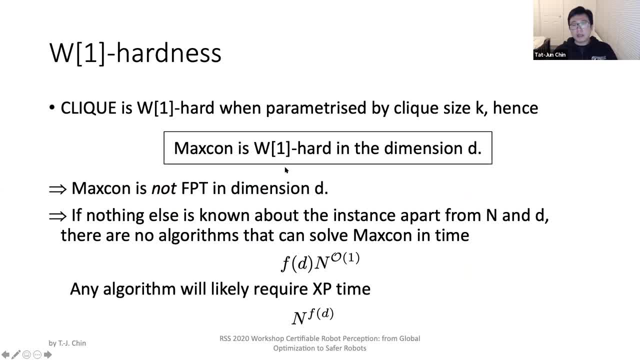 that it's just not possible. And we say that Maxcon is W1 hot in the dimension D, which means that any global solution, even if D is a parameter that you can fix, D must be in the exponent of the runtime of the algorithm. 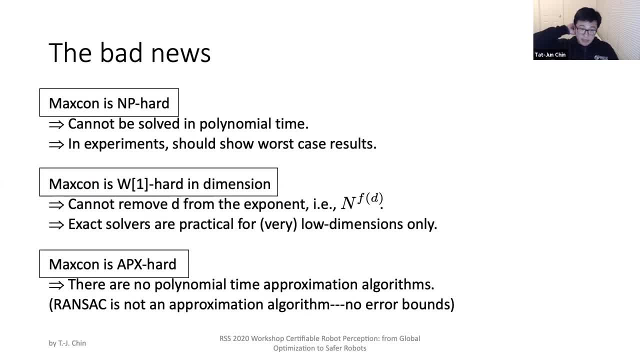 Yeah, this is the W1 hotness result. So this is the start of the bad news. Okay, this is the start of the bad news. we have more bad news For this particular formulation of geometric understanding with outliers consensus maximization. it's NP-hard. 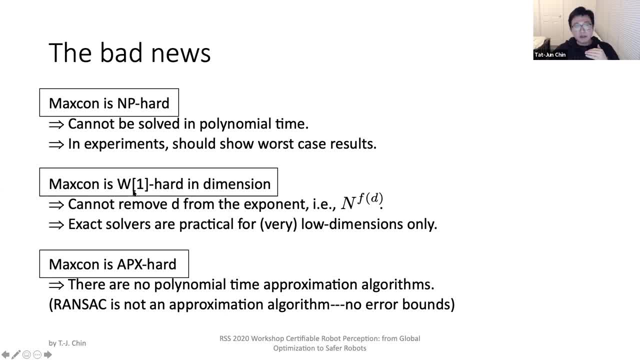 It cannot be solved in polynomial time And it's W1 hot in the dimension. even if you're allowed to use knowledge of the dimension D, D has to be in the exponent of N And this derivation I'm not showing in this talk. 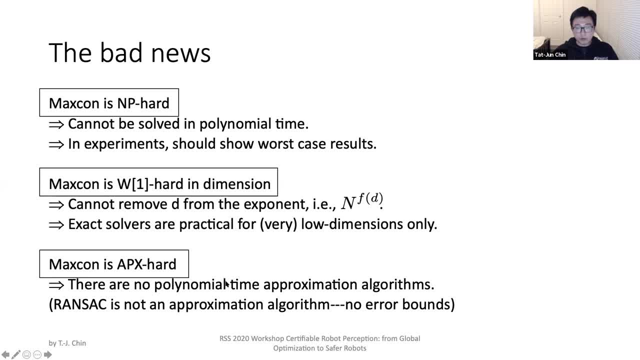 because there's not a lot of time. But you can also show that there are no polynomial time approximation algorithms. Okay, you can't have an algorithm that runs in polynomial time where you can be sure from the onset you know there are sufficiency conditions. 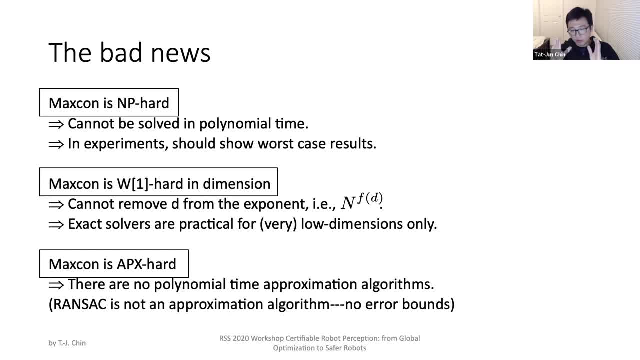 that tell you that your result won't be, you know, a bounded error away from the optimal solution. So RANSAC is not an approximation algorithm, by the way, because there are no error bounds, As we said mentioned earlier, when it gives you. 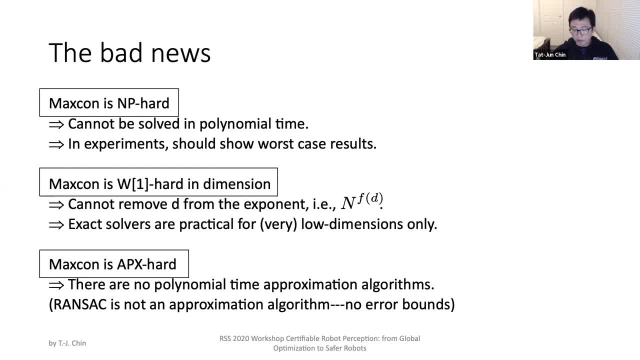 a bad result. you do not know why. You do not know if it's because you were unlucky, you sample the wrong in those subsets, or you know there are no good solutions to be found And our collaborators have discovered similar results as well. 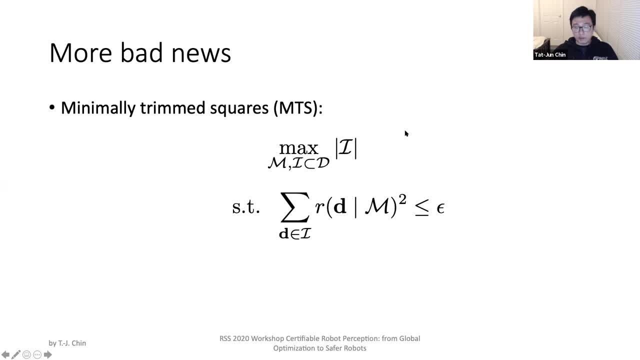 for the minimally trimmed squares. formulation of geometric understanding with outliers, for example. instead of just maximizing the number of inliers or minimizing the number of outliers we want to, so here it is minimizing the number of outliers. We also check that the inliers 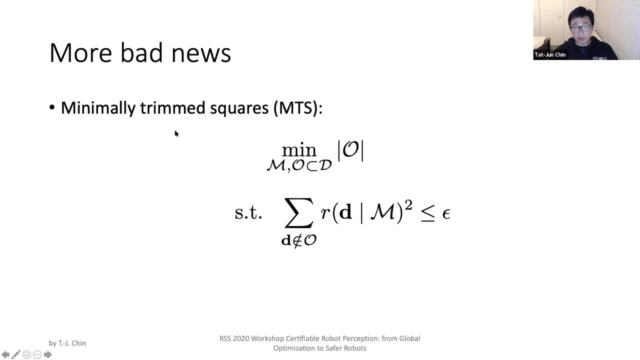 the sum of squared of them are less than equals the epsilon. So this is the minimally trimmed squares formulation for robust geometric understanding without one, And it's also you can show that there are no Watson polynomial time algorithms that can find the solution we want, that is, within a factor Lambda from the optimal. 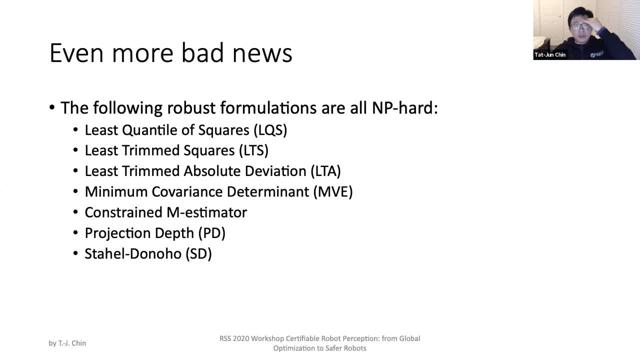 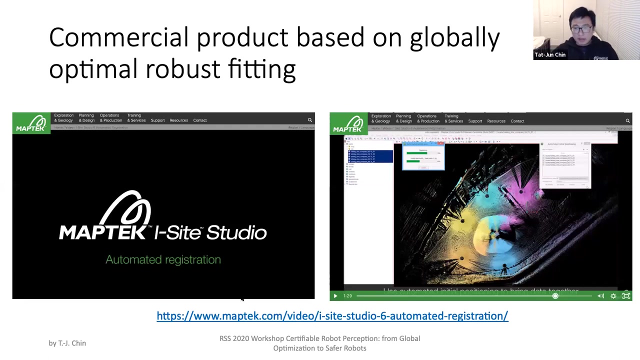 solution And these are all robust formulations that have been proposed in the statistical community and it's provable. these are all NP-hard. So yeah, bad news, right? So yeah, here's some good news and I want to show a. let's see if I. 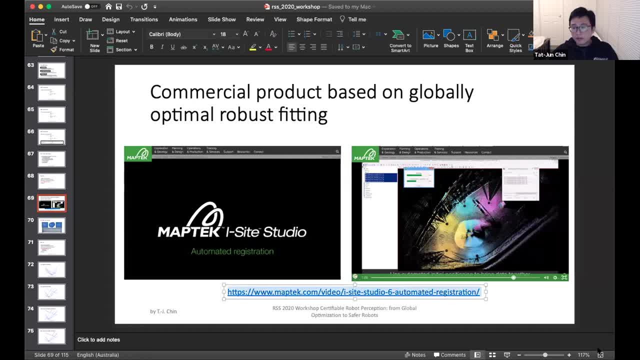 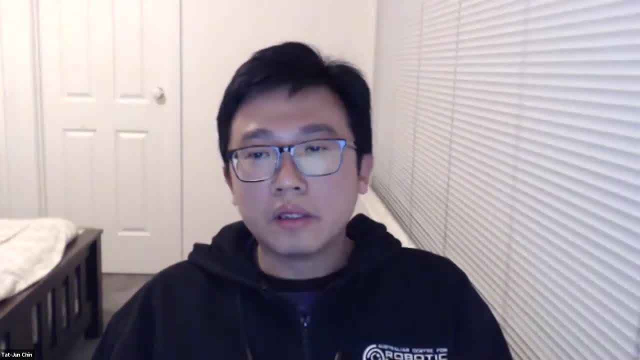 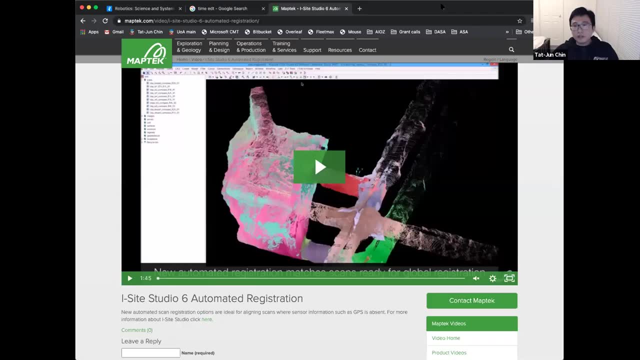 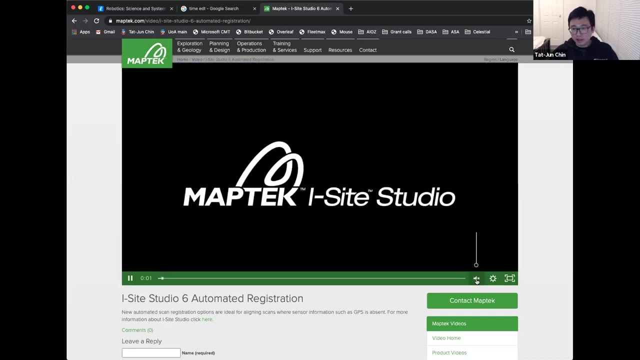 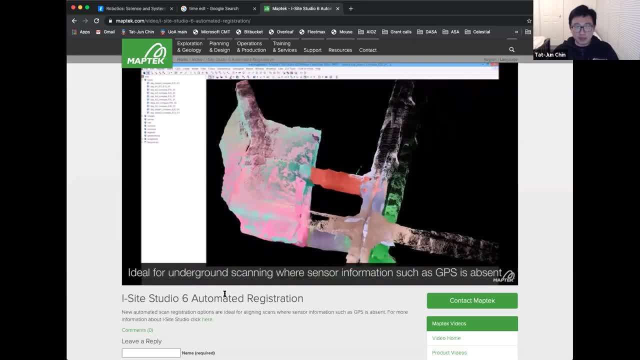 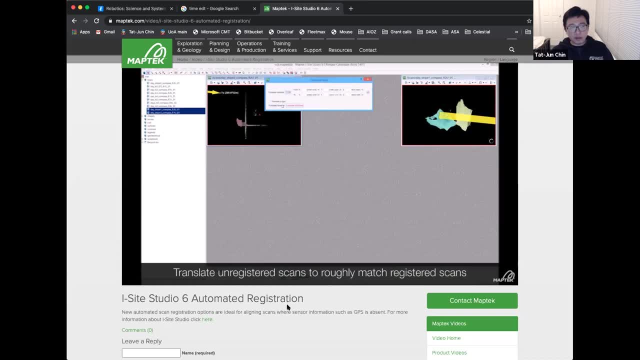 scan matching. But you know, it's basically point: cloud registration, right, And this is- this is a soft point- cloud processing software suite by a company called MapTec that's headquartered in Adelaide. here They deal a lot with the mining industry, As you. 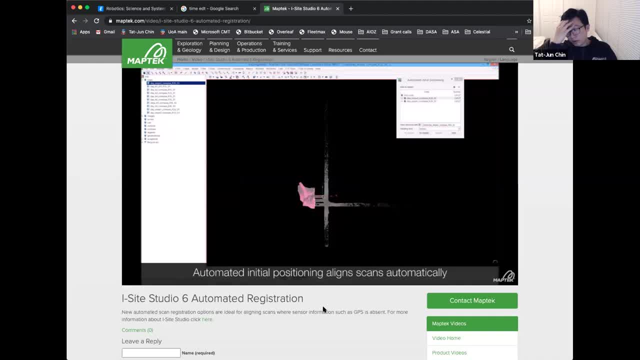 can see here. what you're seeing here is a global algorithm, point cloud registration algorithm running, you know, really, really efficiently. So we in, we have a- you know, essentially an overwhelming amount of software, right, And we have a whole bunch of software. 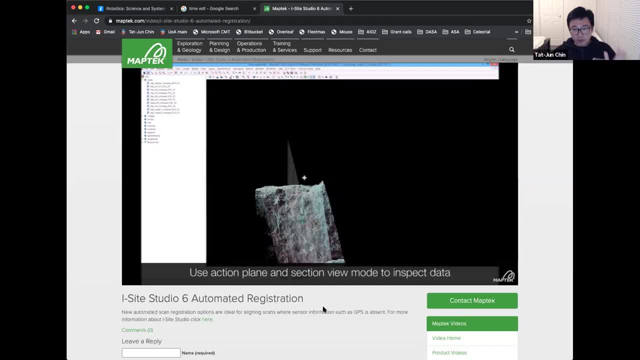 in our company. that's all legal right And we can. it's a comprehensive digital software right. the in the research community care a lot about. you know, polynomial time solvable, global optimality and all that. but on the other hand, let's not forget as well: 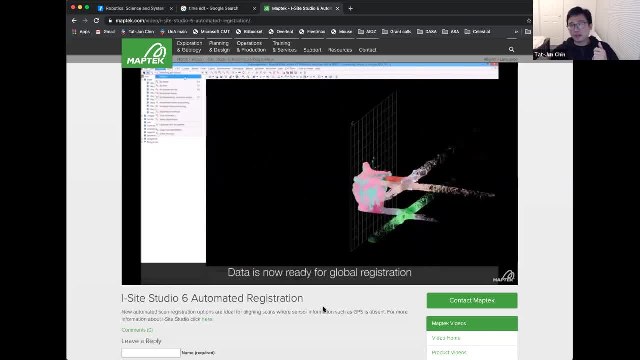 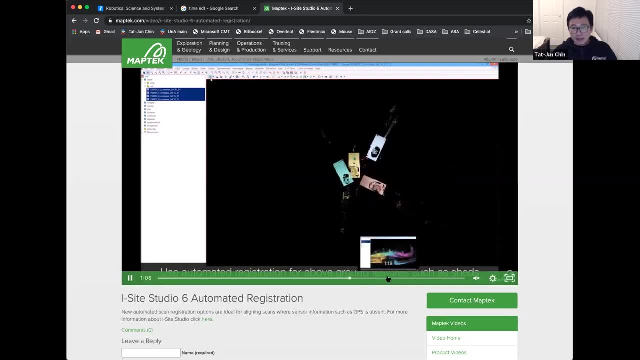 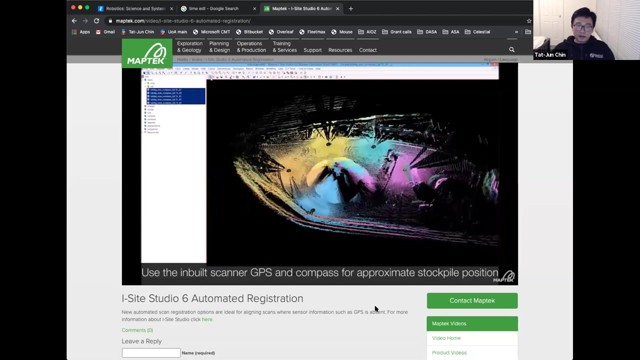 that if you have fantastic software engineering, sometimes algorithms that are not provably efficient can run really, really fast in practice. and yeah, we're about to see another example of global, globally optimal registration happening. and here they're: they're aligning LIDAR scans from an open pit. 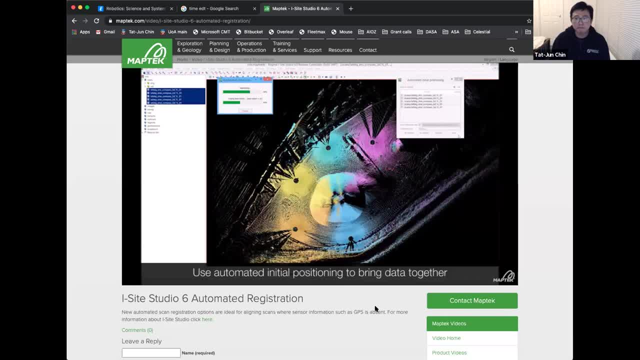 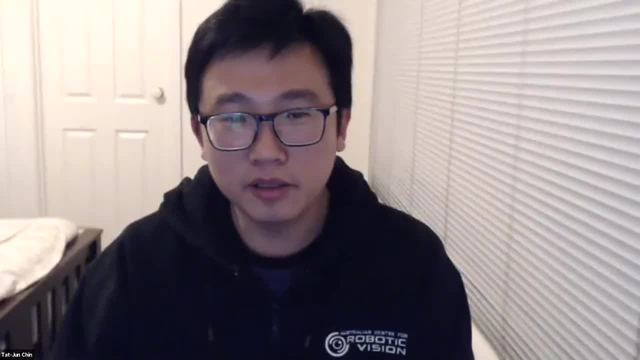 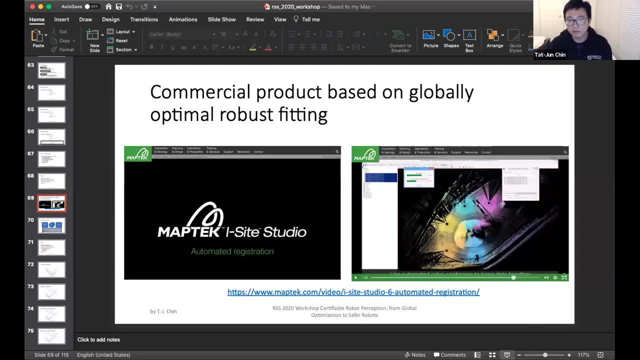 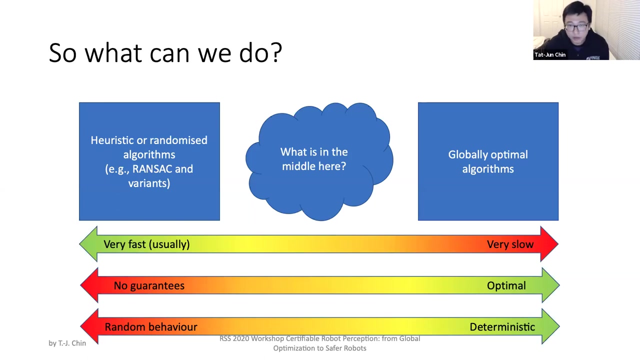 mine, as you can see, cool so it's. it's not all bad news, sick as six dof at least we can still solve quite efficiently if it engineered well, okay, so theoretically though, what? what can we do? I think Hank will, in his talk, will, mention more recent results that are more optimistic, but before that, 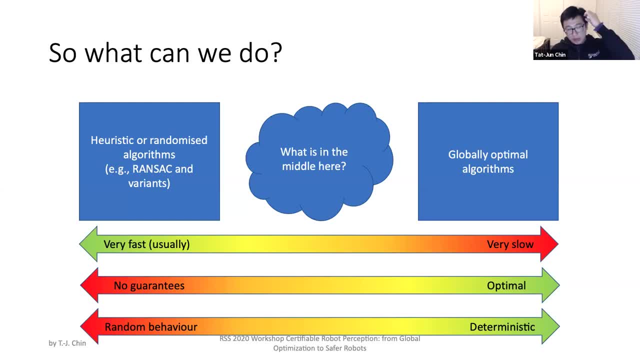 let's see what the theory allows and does not allow us to do right. so, in regards to geometric understand without liars, we have two extremes. on the left, we have heuristics or randomized algorithms such as rent, second variance. on the light right, we have globally optimal. 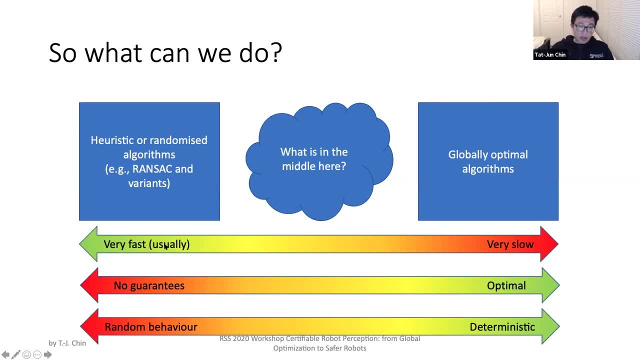 the theory says: sorry, in practice we know that the left, left extreme is very fast. usually the right extreme is very slow. but the theory says that if you want fast, you can't have guarantees, okay, and and if you want globally optimal, it has to be very slow. okay, that's what the theory says. there's nothing we can do. 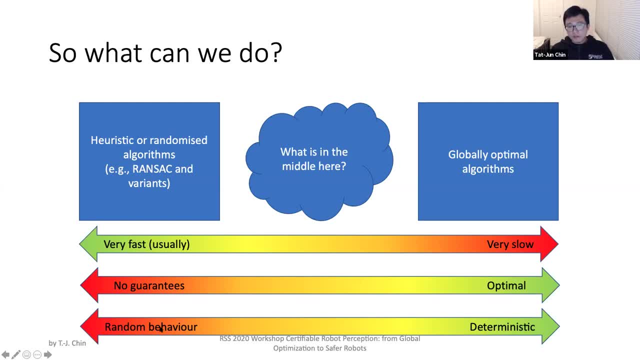 about this. the other thing we can fix is, of course, for for a lot of robustness algorithms. a lot of them use sampling, and this might be an aspect that we can improve by making them deterministic. so what is in the middle? here you know, algorithms we all want fast, because our self-driving car needs to operate. 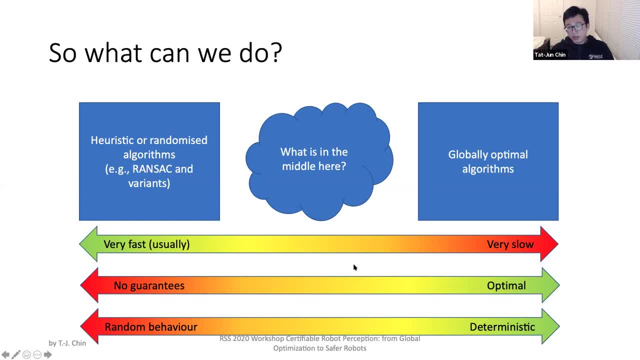 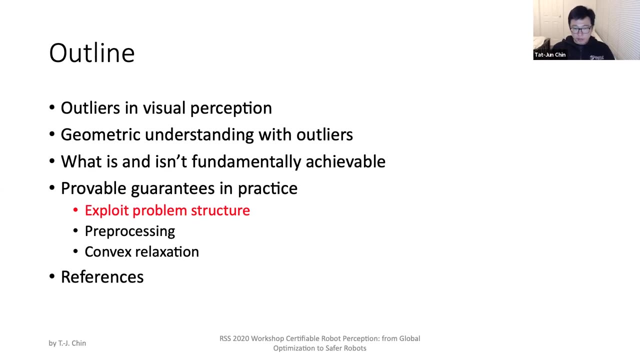 efficiently. the theory says we can't have, we can't have guarantees- not global optimality guarantees, at least- but at least we can make it deterministic, and that's what we're trying to do. okay, so what else? what can we do in regards to that previous plan here? making it deterministic and also, hopefully, speed. 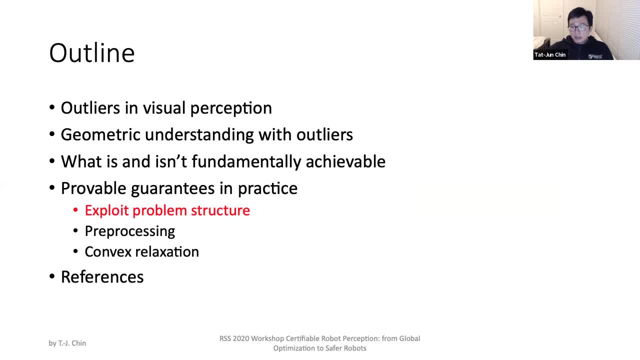 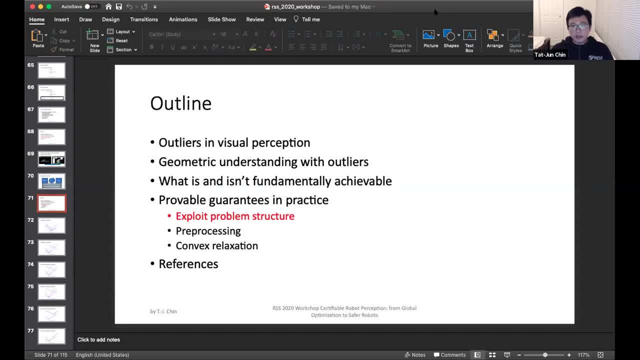 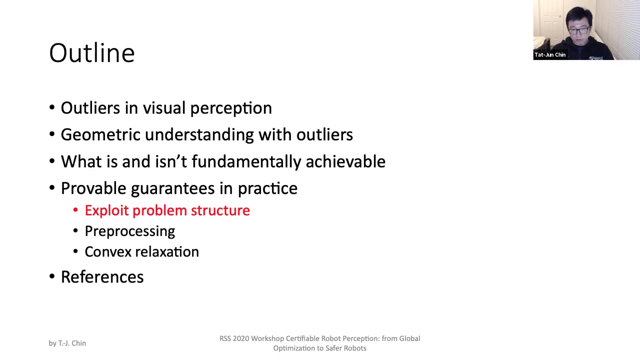 up as much as possible. three main strategies here. let me check my time. I think I have five minutes left if I, if I use my 35 minute limit and based on my starting point. so I'm gonna just roughly sketch these, these solutions. the first solution is to exploit the problem. 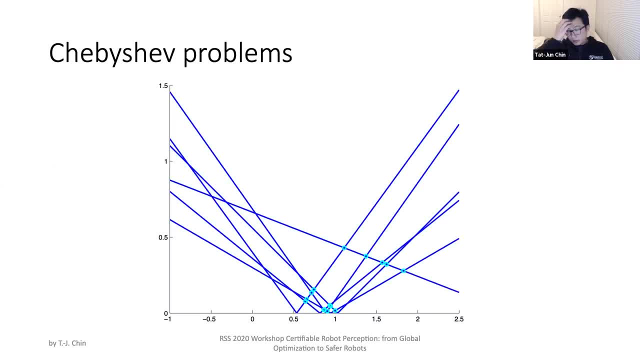 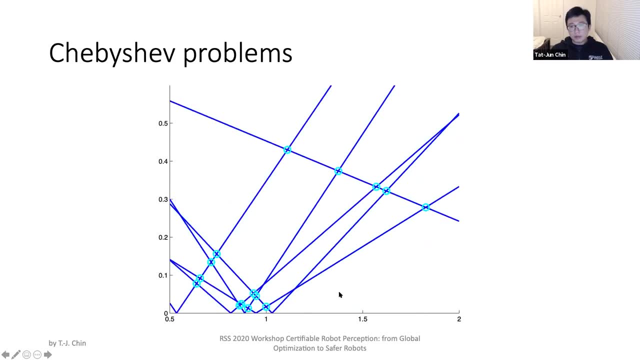 structure and this is ongoing work that we're still doing. so, coming back to the V curves again and and looking at these cyan points, zooming in a little bit more now, if we solve the, the L infinity or the max norm problem, it's easy, we know. 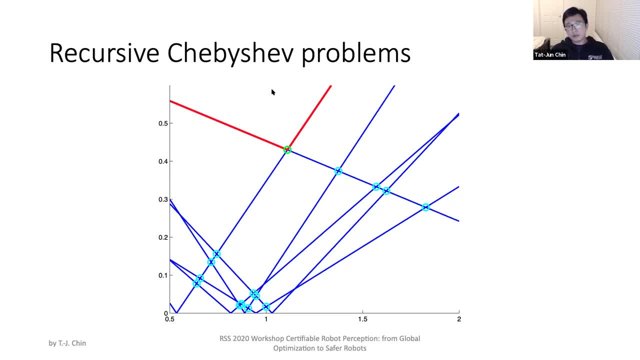 that we can. we can solve it globally optimally, because in in this example or our curves are linear anyway. but you can generalize it further and show that this works even when it's pseudo convex. so we can find that solution, find that green point quite easily, but if we remove it, 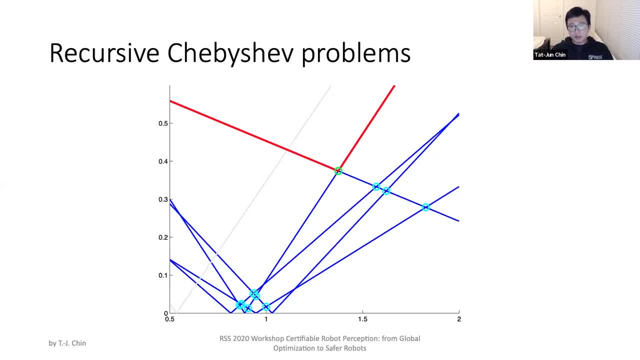 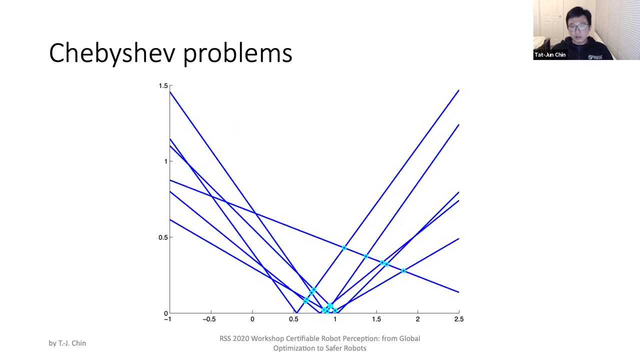 one of them at least. then we can solve it again as well, recursively solve it again by removing one point and keep going, okay, so this is not trying to do anything, but to illustrate that actually, these cyan points here, you can reach any of them from the top by 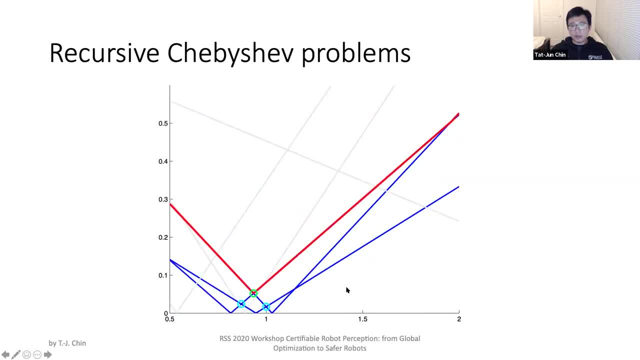 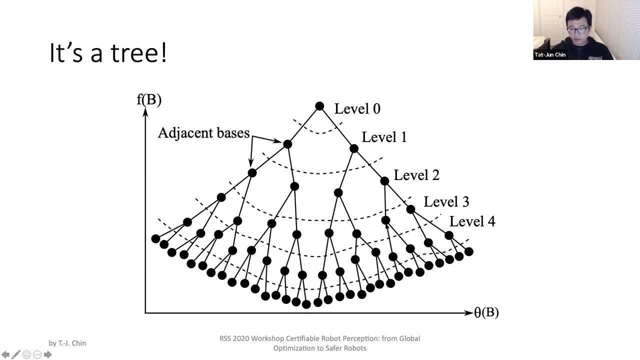 following a sequence of removals. so all these cyan points lie actually on a tree and each level of a tree corresponds to a number of points you have removed. you can regard these points at the outliers that you have removed. so, by exploiting structure, this is what we mean. if you just run a standard RANSAC on the. 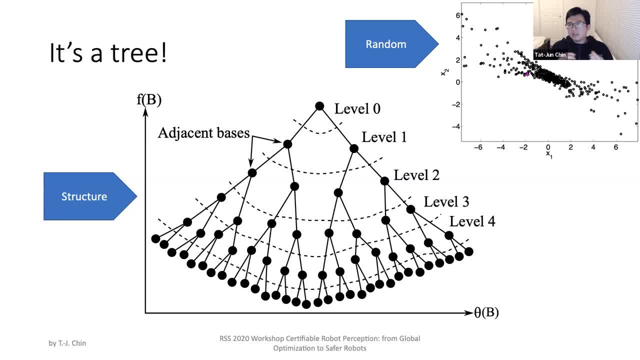 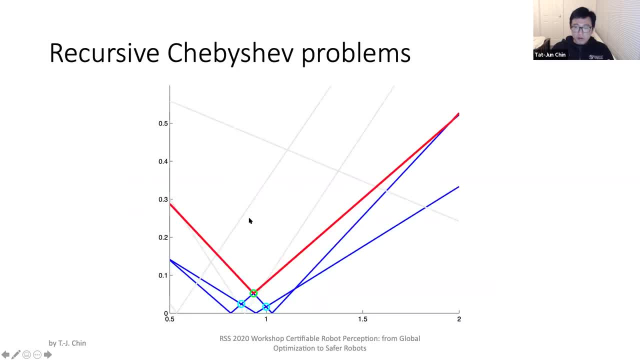 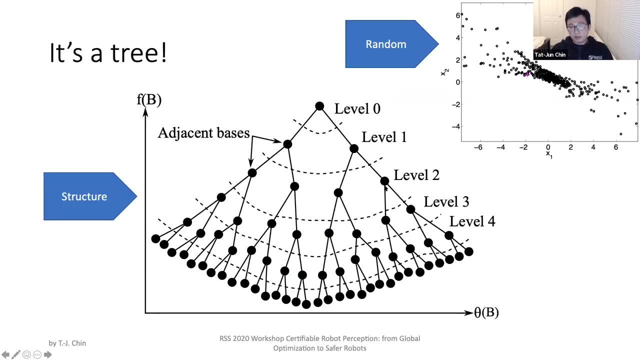 bunch of points there. you would think that all these estimates, these minimal estimates, actually lie lie randomly in the parameter space. but if you look at the how these V curves are organized, you realize that there's further structure in the data, in particular tree structure. okay, the the points are organized in. 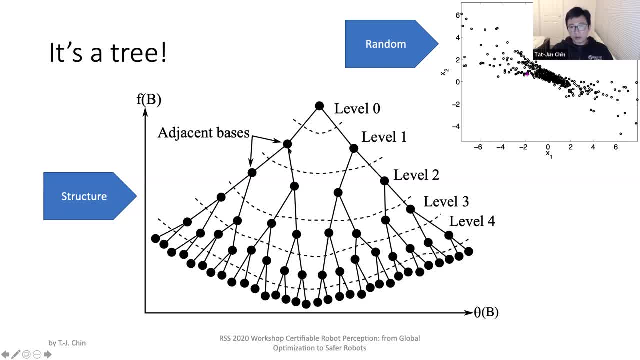 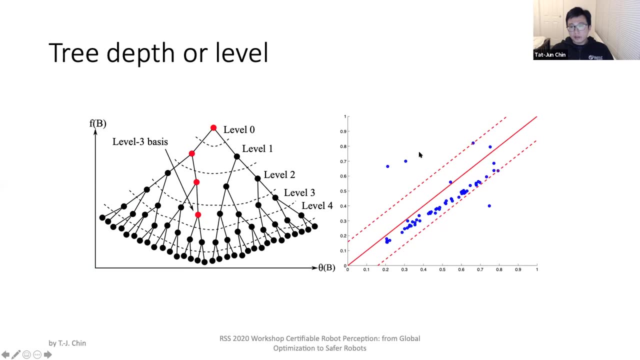 layers. actually, I should be more careful. it's not. these are not the data points, but each of these is a active point of an active set, a basis. so the depth of the tree tells you the number of points that's being excluded. okay, so this red point here, for example, corresponds to: 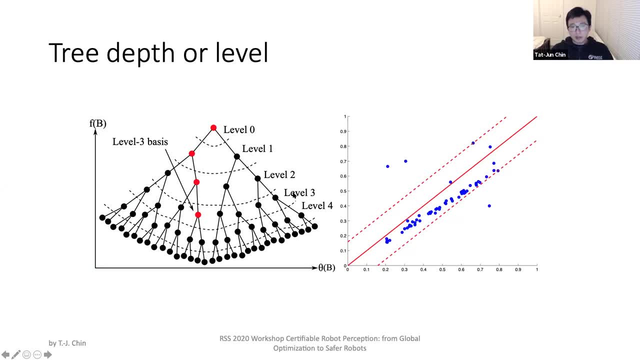 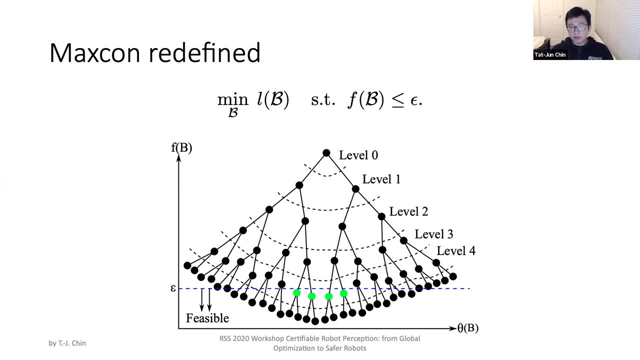 that and that point as the active set and because it's at level three, it's excluding exactly three points. so with this knowledge we can solve the consensus maximization by searching the tree. so this provides us a structure to work with with all right, So we can restate the problem as finding the active set B that has the lowest. 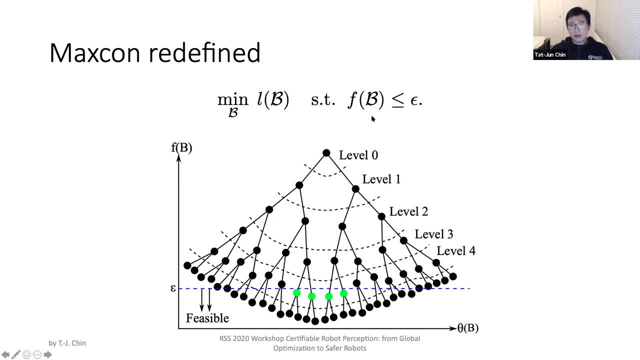 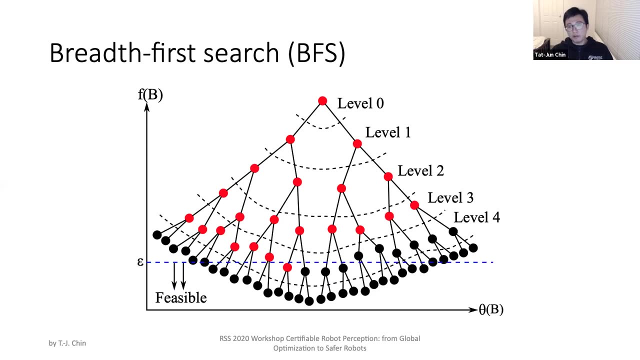 possible level, as close as possible to the root, and whose height, which is the size of that slab, is below epsilon, which is what we call feasible. okay, So we can search it level by level. This is one algorithm and that will be the breadth-first search. We. 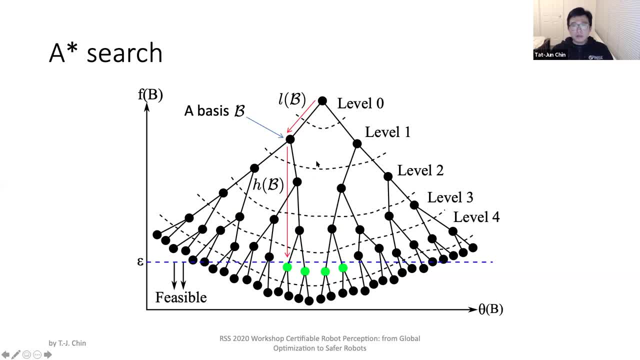 can search it using A-star search with a heuristic. and this is when we get back to the branch-and-bound idea that Anders mentioned at the start. If you think about it, searching the tree, isolating and pruning the branches is actually similar. It's actually the exactly same idea as branch-and-bound. 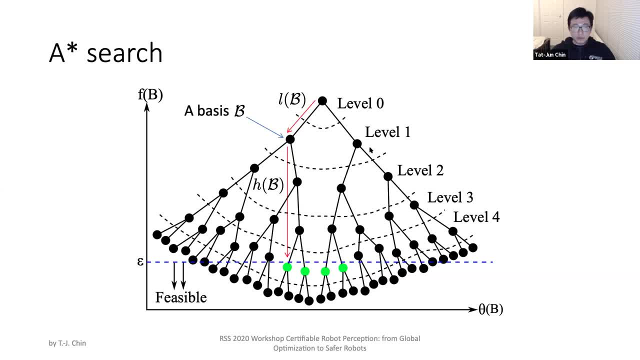 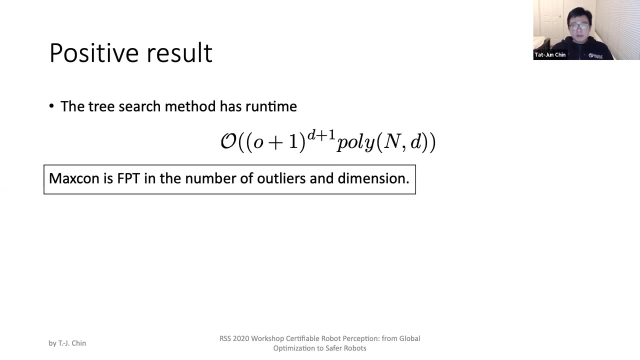 Instead of pruning using a bounding function, you prune it using a heuristic which is really, you know, can be solved, can be computed using a convex relaxation of you know, a subset of the points. all right, So it's the same idea expressed using different knowledge. 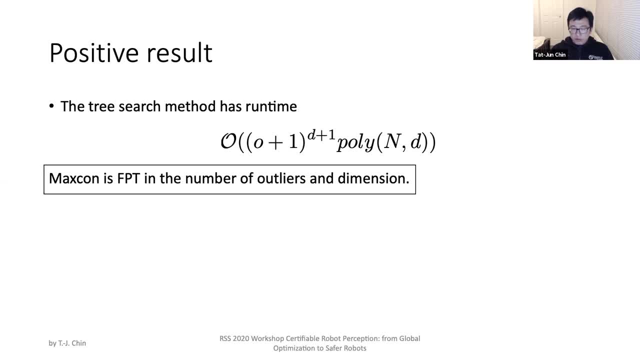 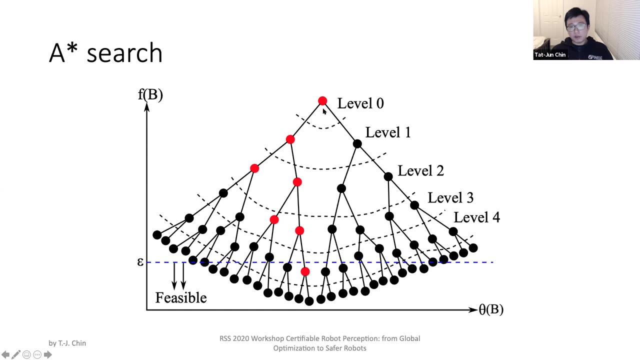 But what we can do here, though, this type of this way of doing branch-and-bound allows us to bound the runtime. okay, We can show that because we don't need to search beyond level O- O is the number of outliers we have, and because we know that the branch-and-factor 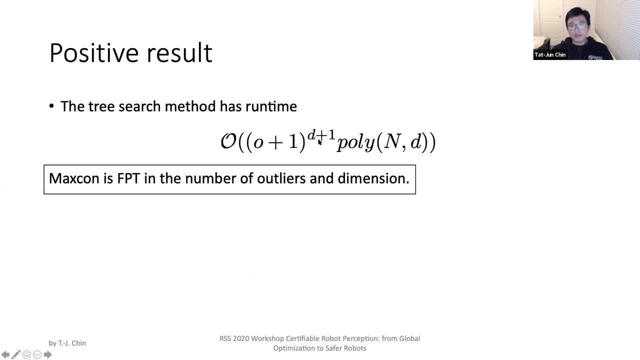 because each basis has D, D plus one points. the branch-and-factor is therefore is D plus one. It allows us to bound the runtime such that you know it's only exponential in the dimension D, and also the number of outliers O. okay, So this would be one solution. The 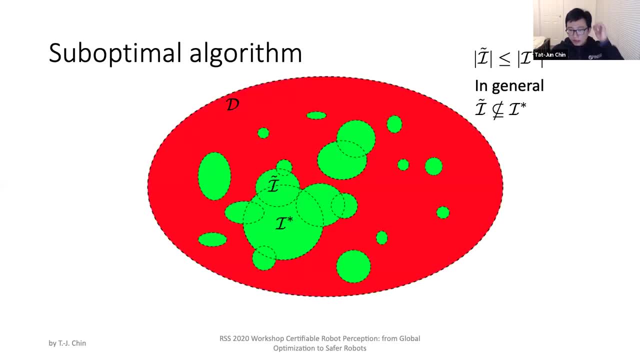 other solution is pre-processing. I need to speed up here. We're trying to find a subset of the points that contains inliers only, and we know, you know, that's very difficult to find. This big set here is difficult to assign. D is the whole data set of points that we have. We have, you know. 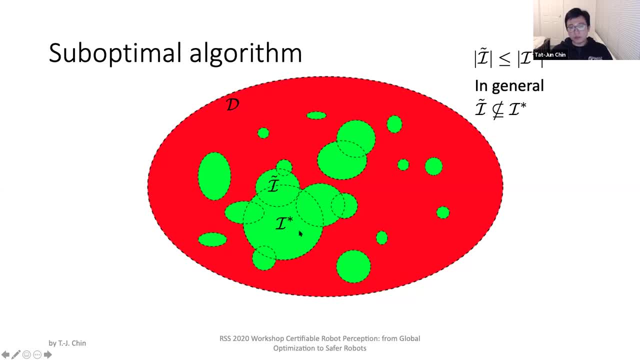 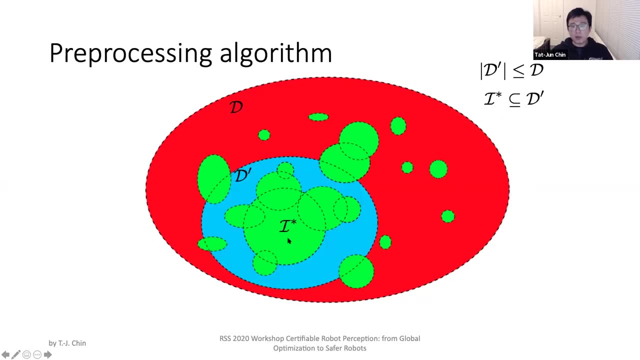 we're finding pockets. If we have a heuristic algorithm or suboptimal algorithm, we're finding pockets of these inlier sets We can never find. we can never guarantee finding the big one. But what if we change the problem? Instead of trying to find, I star. what if? 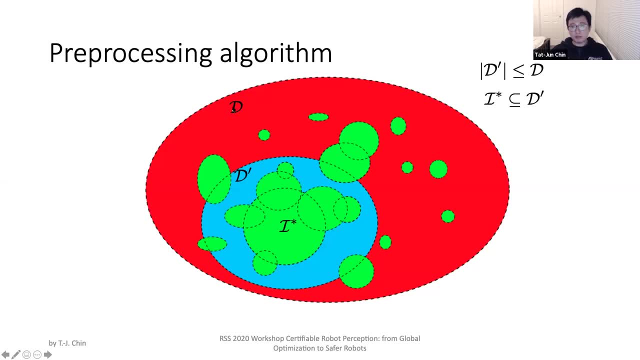 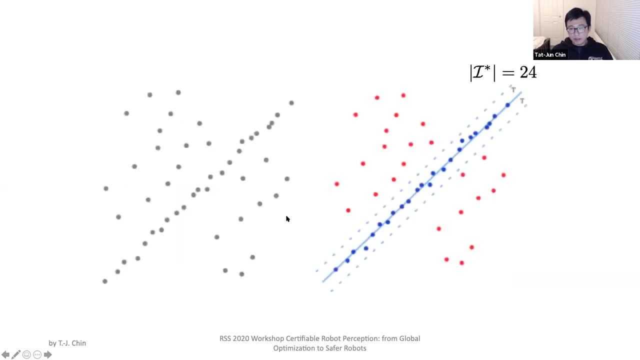 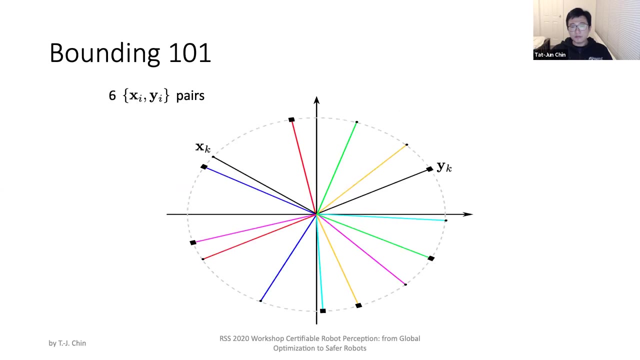 we find D prime, Where D prime is a subset of D but D prime guarantees to contain I star, And this is what we call the pre-processing problem. I don't think I have time to go through this. I'm going to show you the outcome of it. Sorry about that. So in the point cloud. 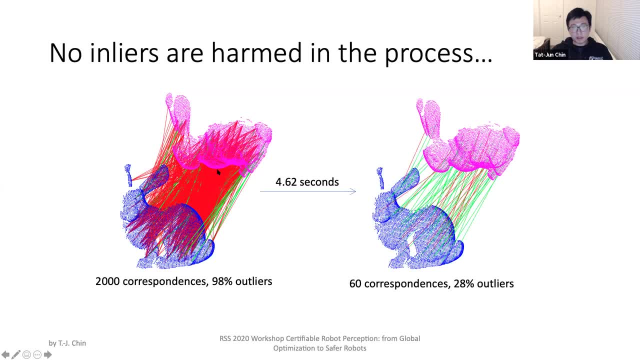 problem again. we have a bunch of correspondences competing using a black box. Instead of trying to find those green lines that I star the inlier set from the get-go, what if we just remove as many of the red points as possible in a manner that guarantees that none of the 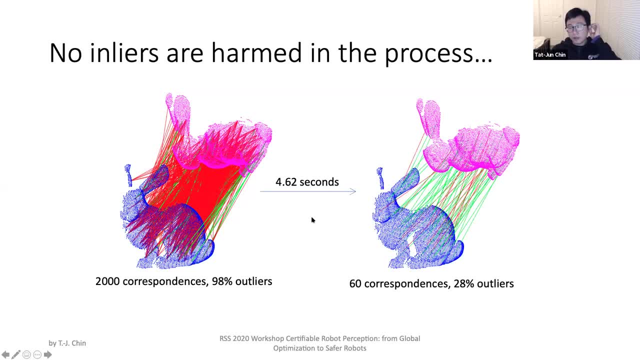 green lines are removed. Okay, So this will be the what we call the pre-processing step. It's actually can be achieved really quickly, like in 4.7.. So we can see that we have a set of points and then we remove almost all of the correspondences. 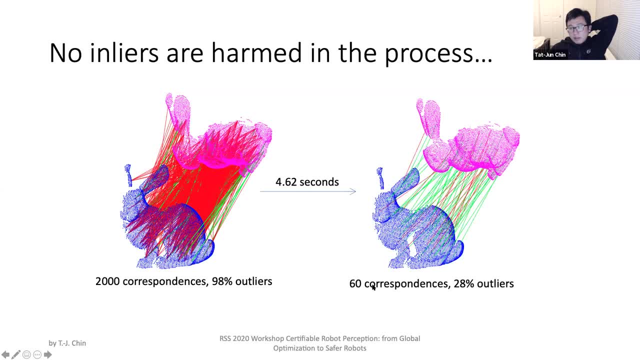 And then we're left with 60 in a manner that guarantees none of the inliers are removed. Okay, And if we subject this, this set of remaining points, to further optimization, then you know it's, it's much faster because there are fewer, much fewer points to deal with. 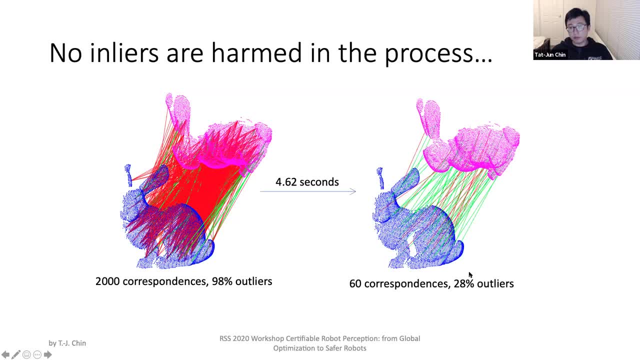 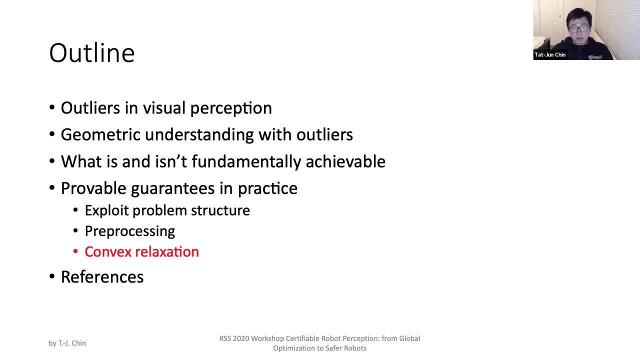 much fewer correspondences to deal with And the outlier rate is also significantly reduced. So sorry, I didn't have- I don't have time to go through this And convex relaxation. I'm just going to briefly go through this because I know Hank. 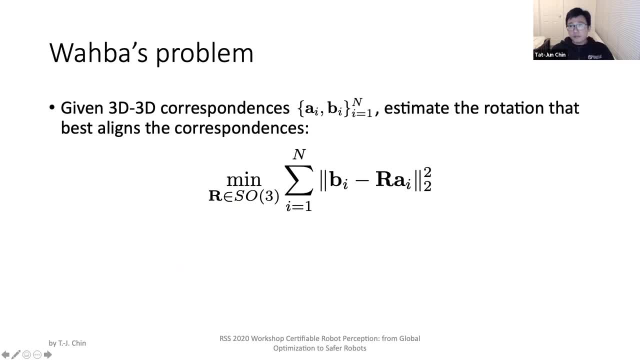 will be covering this as well. One of the previous work that Hank and Luke have done is on 3D-3D corresponding estimating rotation from 3D-3D correspondences, or so-called Wabaugh's problem. Given a bunch of these correspondences, find the rotation R that minimizes square. 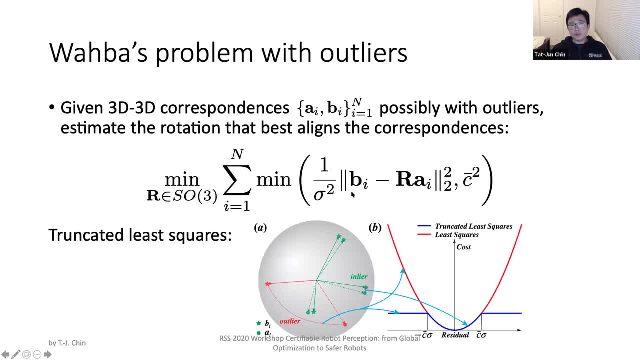 sum of square of the errors. If you have outliers, you need to consider a robust norm. In this case we can consider the truncated least squares norm And you know we're trying to find the minimum between the error itself as well as some threshold C, C which. 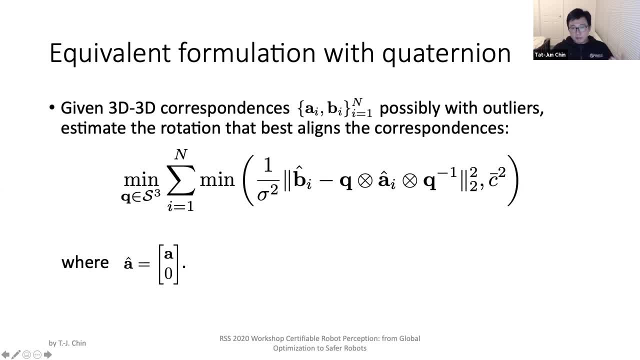 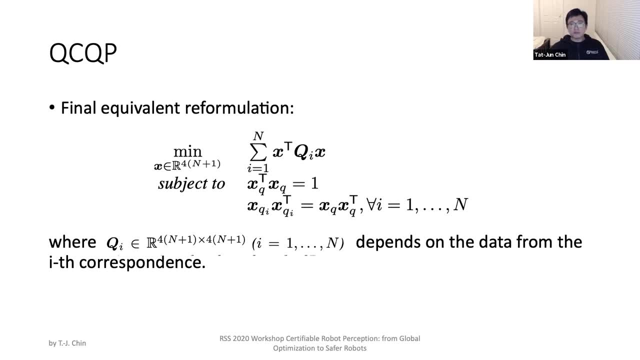 is square And not going to go through the detail, but, as before, we're trying to get it to a QCQP formulation, which is then relaxed And similar to the techniques that covered by Luca before: instead of finding R, we find Z, the matrix. 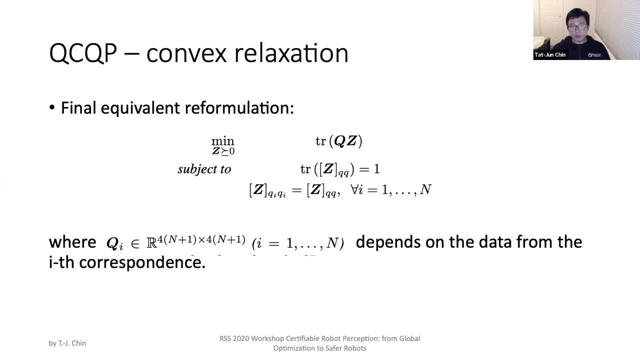 that multiplies, you know, the R's together And we've removed the rank constraint. hence we get the convex relaxation And it's provable that it's always tight and noiseless in RYA-free case. If you add further constraints, as Hank will show later, it will often lead to certify. 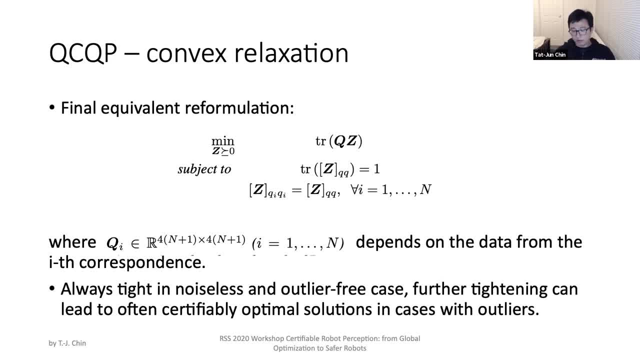 the optimal solutions in QCQP. So this case we're going to see the underlying case. So this is the case with outliers. So these are the three main things we can do under the fundamental hardness result. okay, So I want to spend one minute to talk about that. last point here. I mentioned at 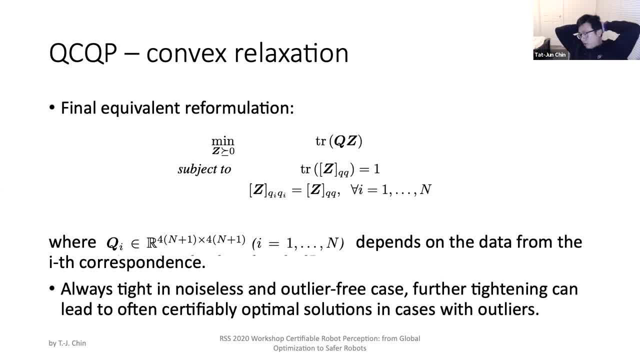 the start of the, a large part of the talk is on showing what's not possible, And what we found was that, with outliers and you use a robust norm, the theory is that you can, you know, see the difference between the three. 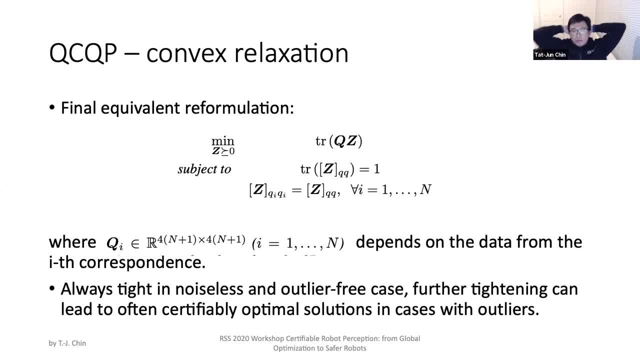 Right, And the theory is that the problem is this: you know, if you call it a constant forbids you to do anything. But then how is it consistent with that last point? here, You know, we can still get certified of the optimal. 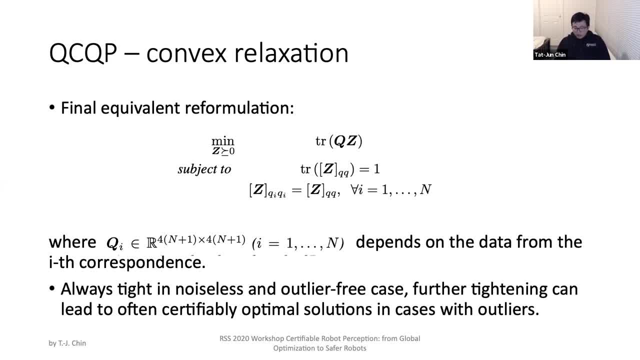 solutions. The key concept here is sufficiency. right, As Anders mentioned, there are two ways to achieve global optimality. One is to show that there are conditions where it's always possible, and one is to verify after you get the result that is global optimal. What the hardness result. 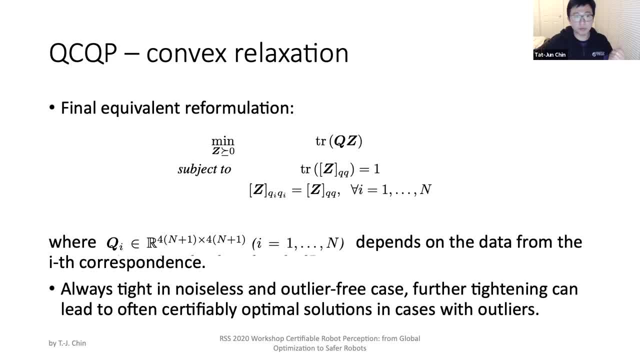 forbids is the first type, the sufficiency: coming up with an algorithm at the onset that says this algorithm runs in polynomial time. it will guarantee you an error within this much. So that's what the theory forbids. So it's not inconsistent with the result here, And here's a list: 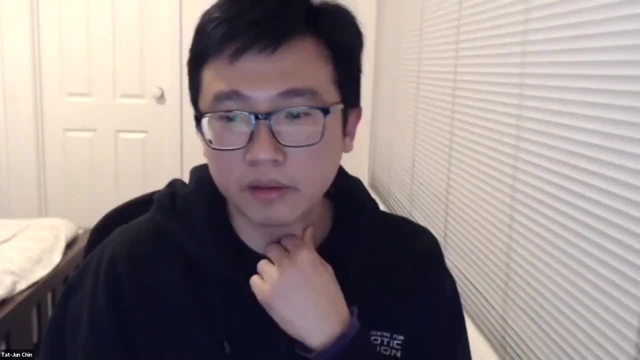 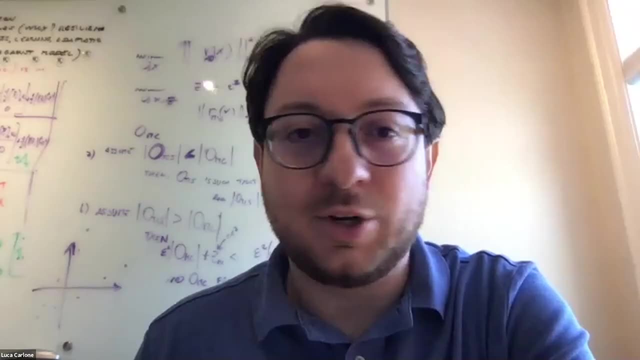 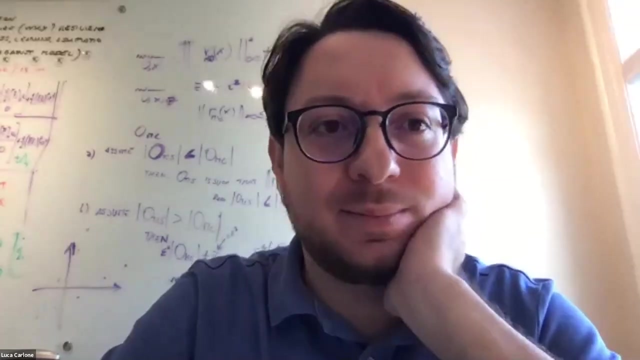 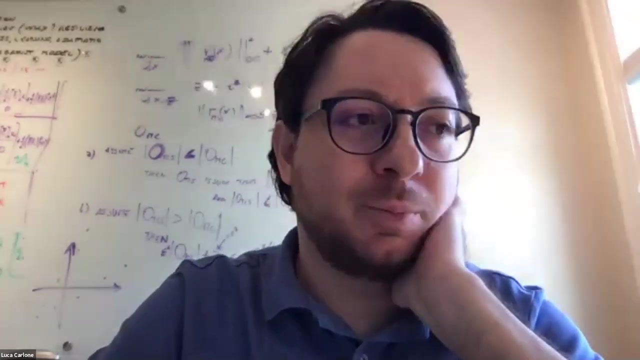 of references. Thanks, I love the plots. I think the plots are super insightful, like you know, looking at low dimensional problems and try to really look at the search problem, which is solved, like you know, for these outlay rejection problems. I think it's super. 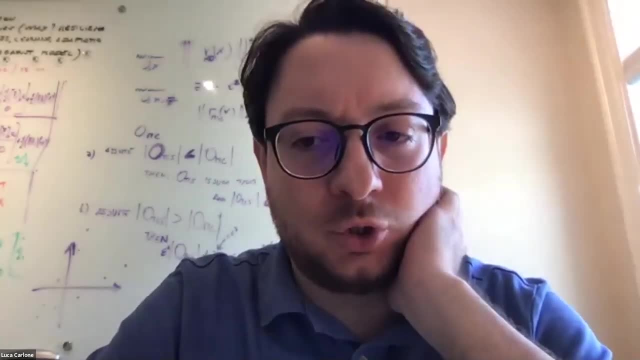 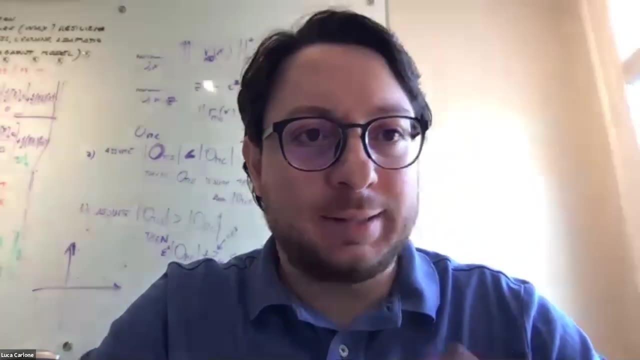 insightful. I have a question which goes back to what's possible and what's not possible. The question is the following: In fact, the results clearly are showing that, in the worst case, there is not much you can do in polynomial time, right. So there are these very unlucky 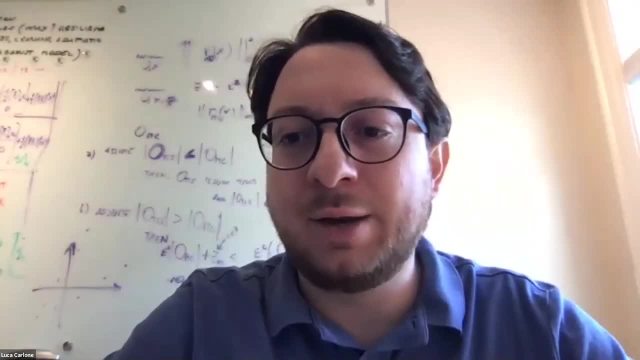 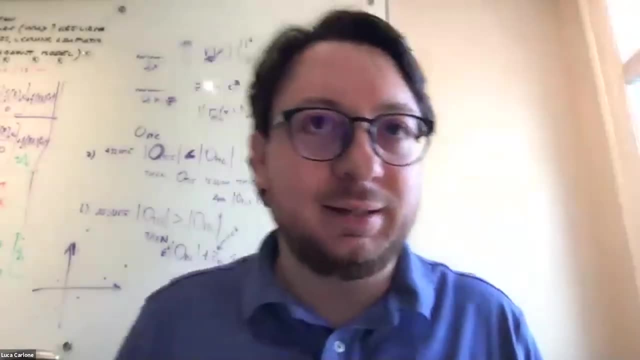 instances in which there is nothing you can do. Are you aware of any result which is looking more at the average case? Maybe we would be happy seeing that if this worst case instance is up and with probability zero, maybe that's not too bad, right. So are you aware of any? 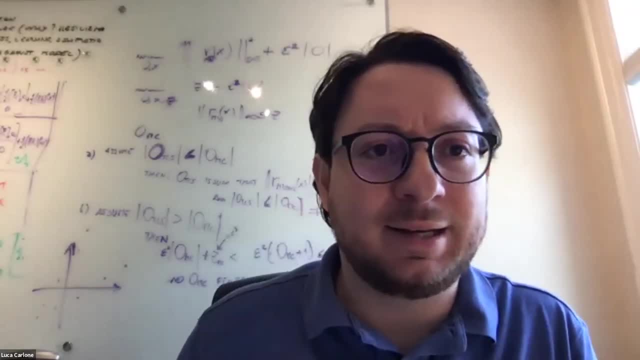 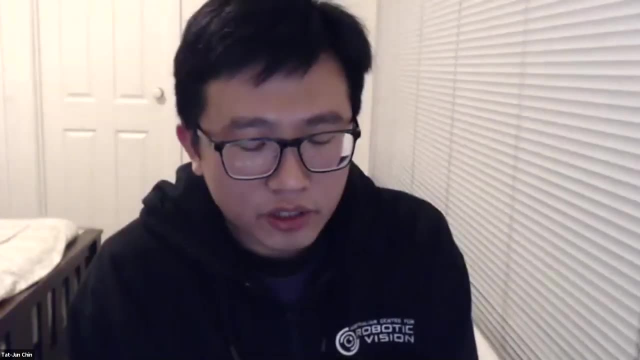 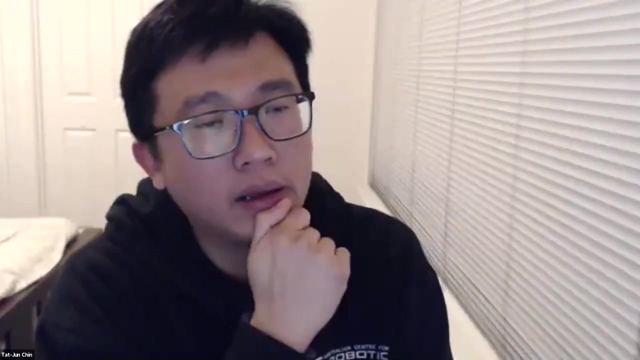 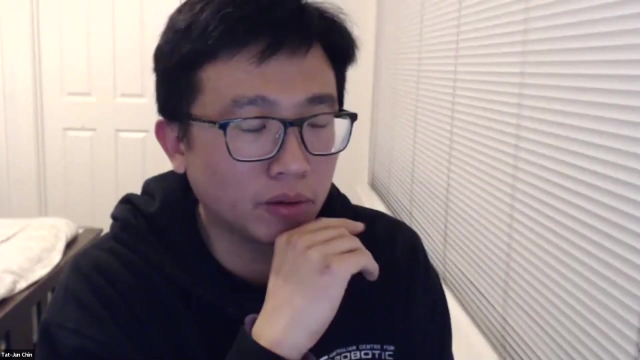 result, seeing that in that sense, Like maybe average complexity or like you know anything else along that line. Average complexity, no, I'm not aware of. We did run some empirical result to find out. you know, yeah, the hardness theory says it's never, it's not possible to bound The worst. 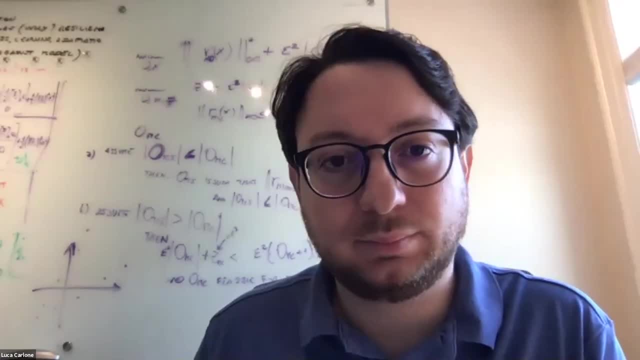 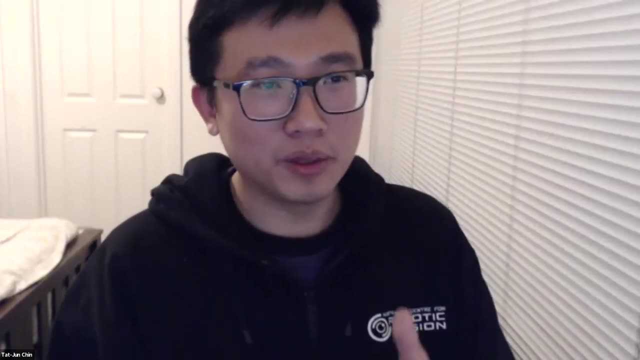 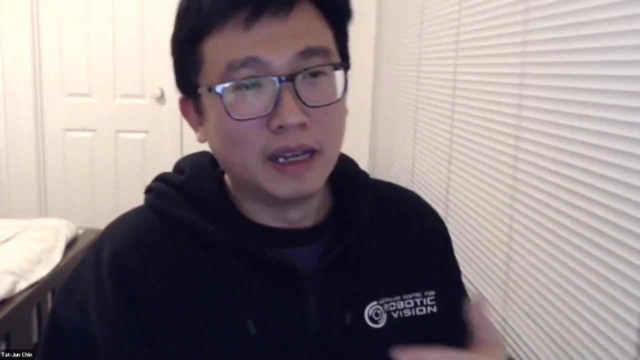 case bound is bad, But are there instances where? how often do these hard instances occur? We ran on the KT dataset and we discovered that you know just estimating, for you know successive frames estimating the polar geometry. most of the cases are hard, unfortunately. 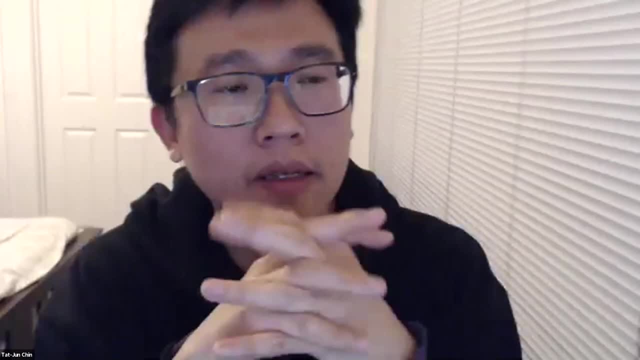 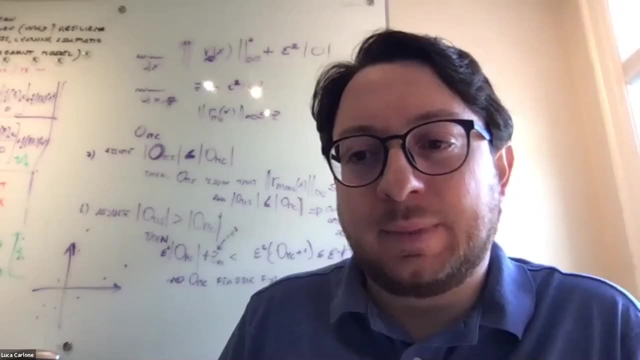 Empirically, Empirically, yeah, So that kind of reduce our motivation to go further down that track. That's my probably. that's consistent with the experience that we have on our side, Like you know, at least if you look at. 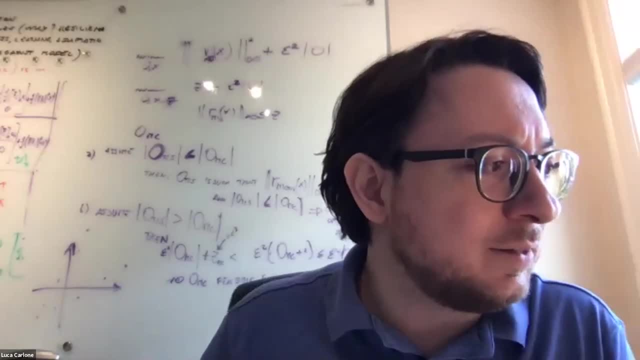 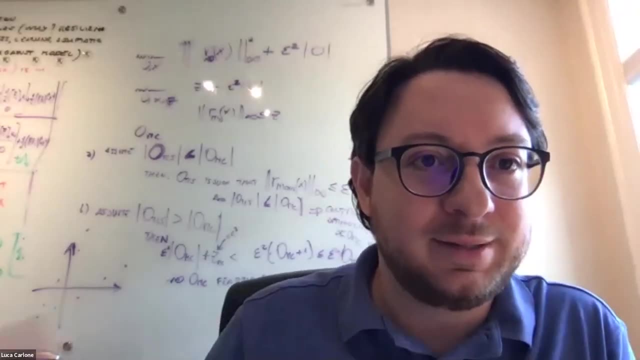 Ransack and so on. that's consistent. When asked the question I was thinking also about. I don't know if you're familiar with these results from simplex method used for linear programming. Simplex method is exponential time in the worst case. but there are these nice. 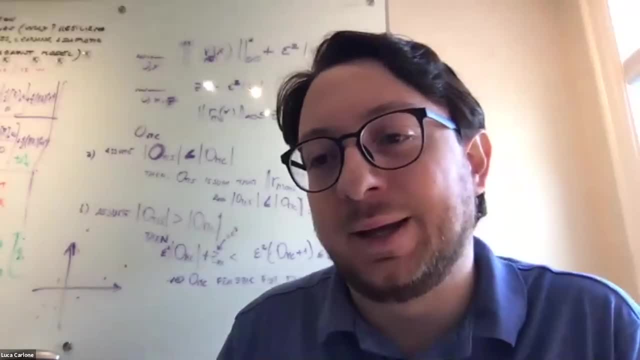 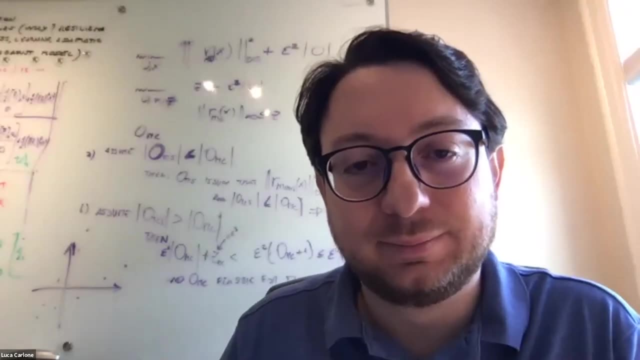 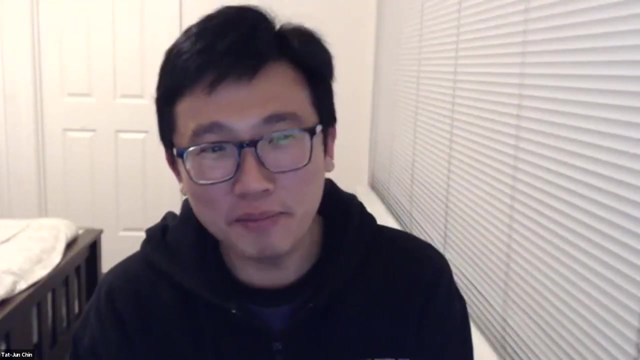 average complexity results in which everything becomes easier. Smooth analysis, That's right, That's right. So smooth analysis is another path we considered before, but yeah, it's not easy to get into, at least for for for me. So it might be possible. but even without smooth analysis there's already. 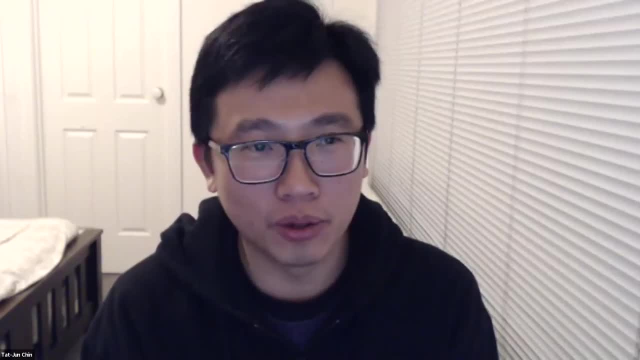 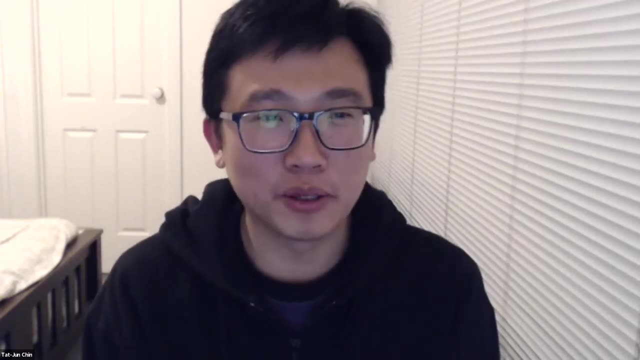 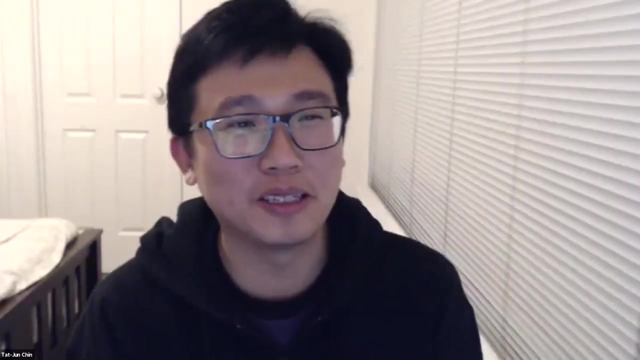 strong empirical result. that simplex is usually polynomial time right. The smooth analysis kind of confirms that empirical result. What we're facing here is different, though, Most of the time the empirical results. so that it's not, it's not easy, It's fast. 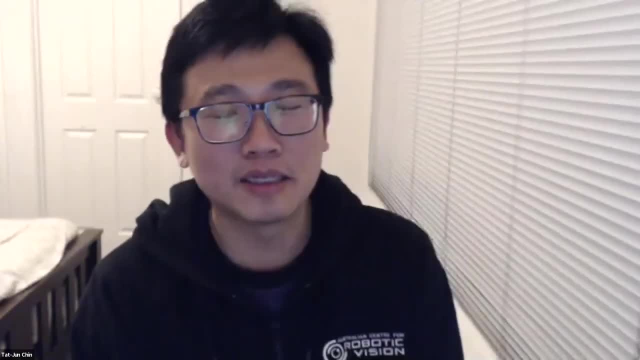 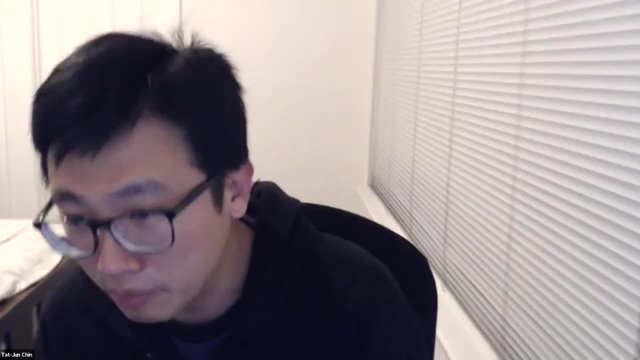 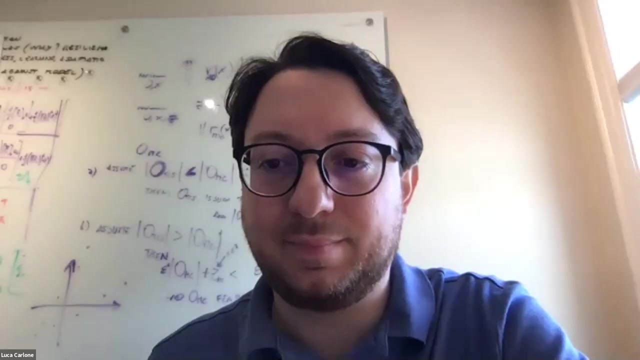 Yeah, So we we did. we did toy with smooth analysis. So I mean, Shubh in the chat window mentioned something which is very reasonable and promising. He said I was wondering what would happen if probabilistic guarantees are sought instead of exact solution. Yes, that is an avenue. 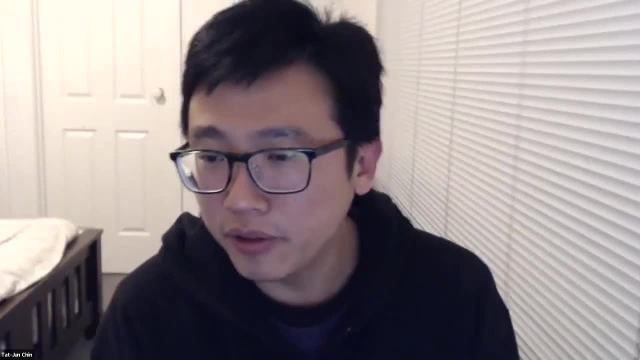 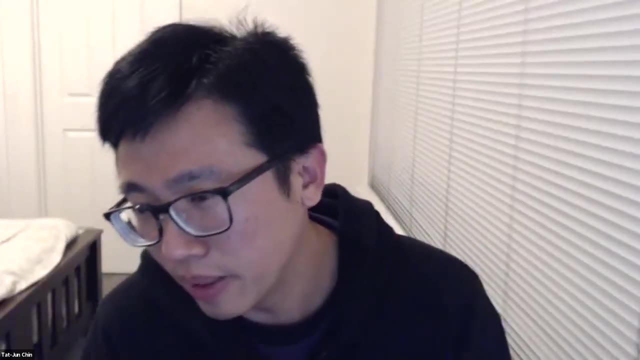 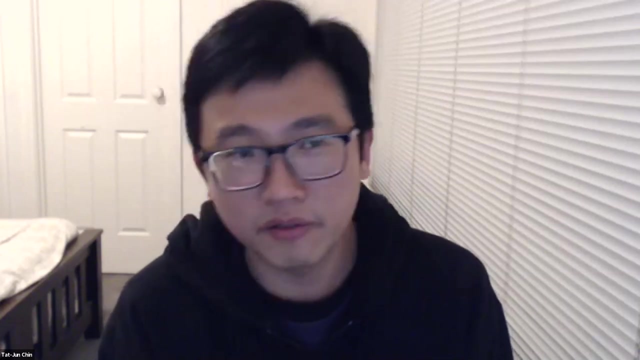 That is an avenue And, Shubh, if you, if you check an archive paper we published, we submitted or uploaded a couple of weeks back, we we were aiming for a quantum solution to this problem And in in finding for that quantum, 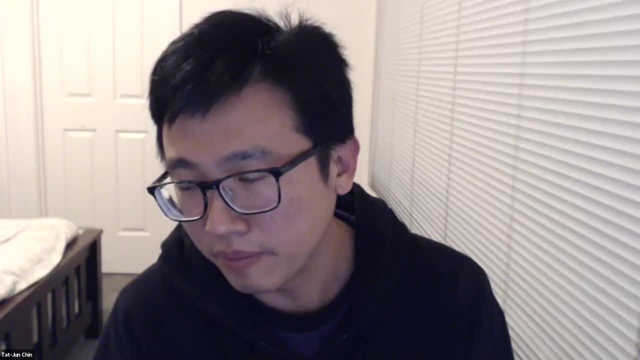 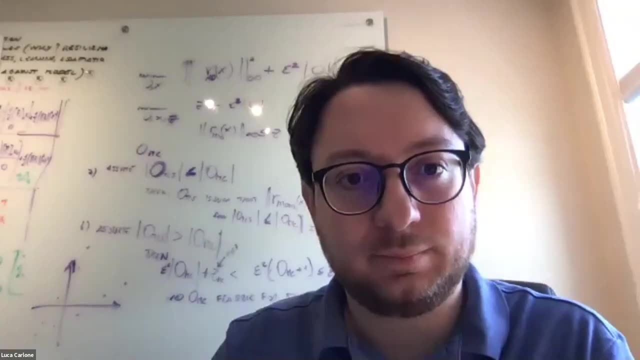 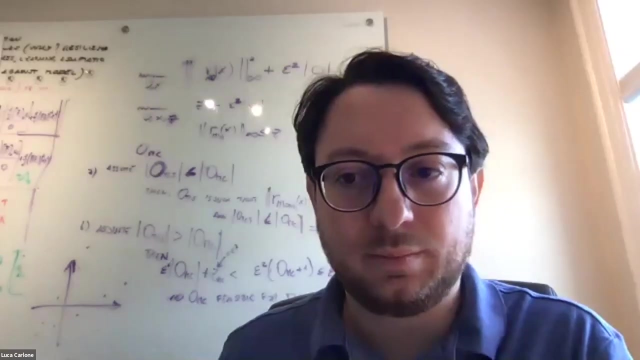 solution. we found a classical algorithm that provides probabilistic guarantees, not not in the exact consensus maximization or any of the robust norm that we were talking about. I was talking about in my talk. different formulations for robust, fitting and classical algorithms can. 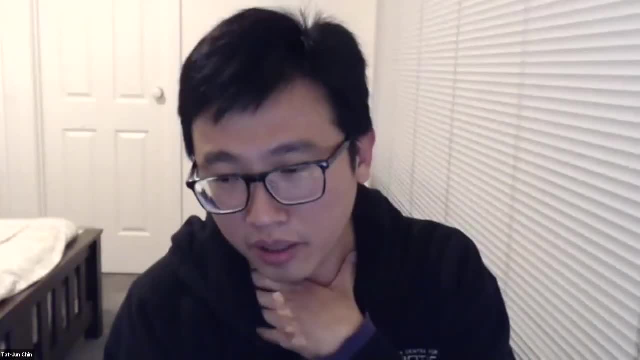 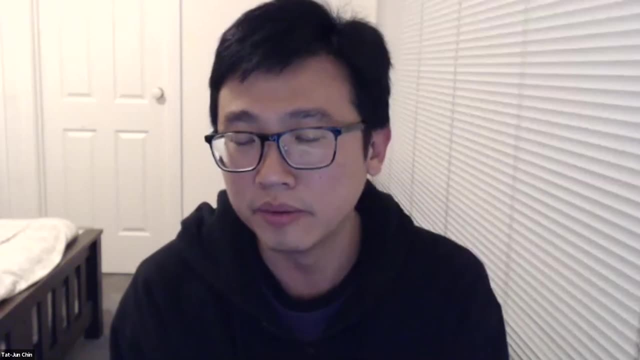 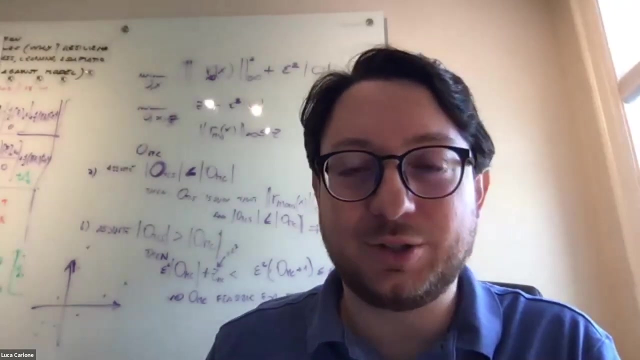 provide probabilistic guarantees, and and quantum algorithms can, in fact, speed it up. So, which is why I'd say it's, it's promising, promising avenue, Very cool. So, TJ, thank you so much, And at this point we'll pass the word to Hank for the 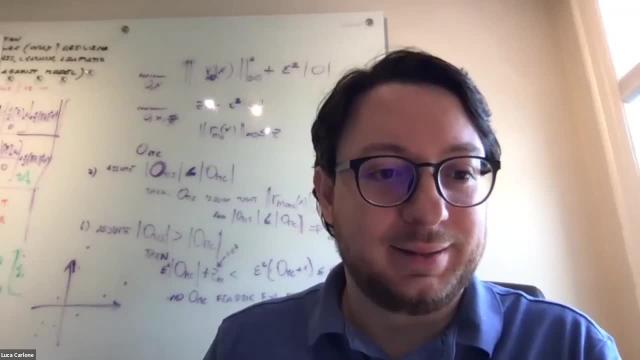 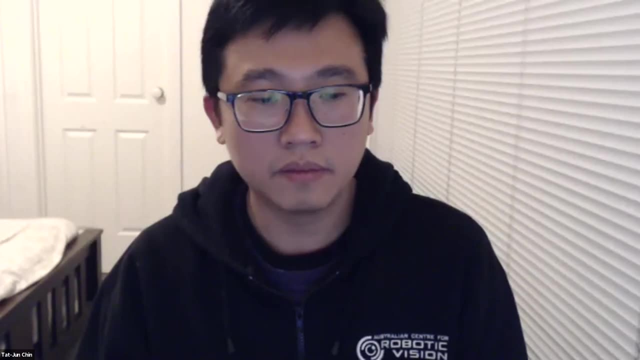 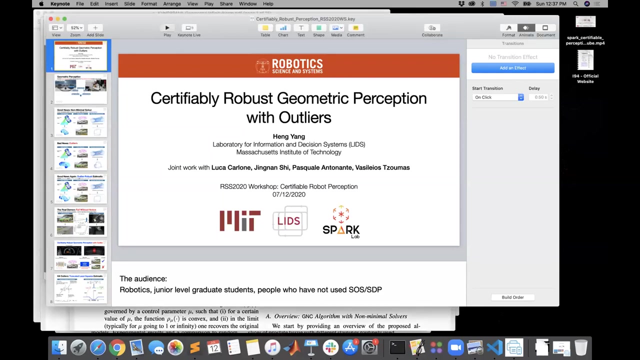 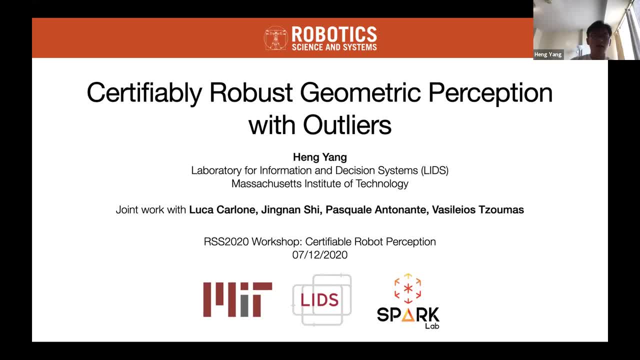 Okay, Okay, Yeah. So in this last talk I'm going to particularly talk about basically the third point of TJ's strategies in dealing with a robust estimation with outlier, which is convex relaxation, And I'm going to talk about certifiably robust geometric 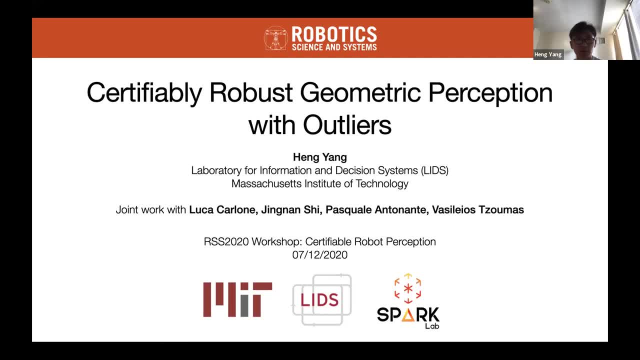 perception with outliers Basically. so you know, we already know that. you know the theory prohibits us from doing anything that has guarantees a priori. But then we're trying to answer the question that, after solving them problem, can we certify or 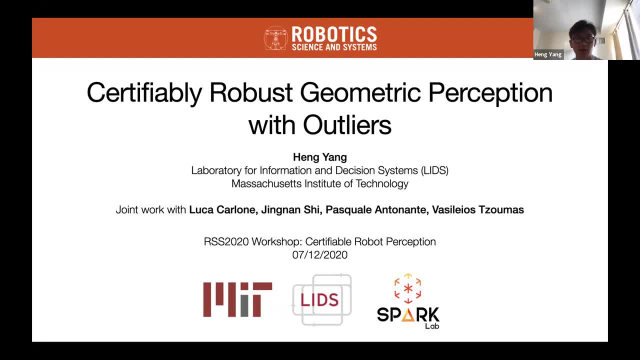 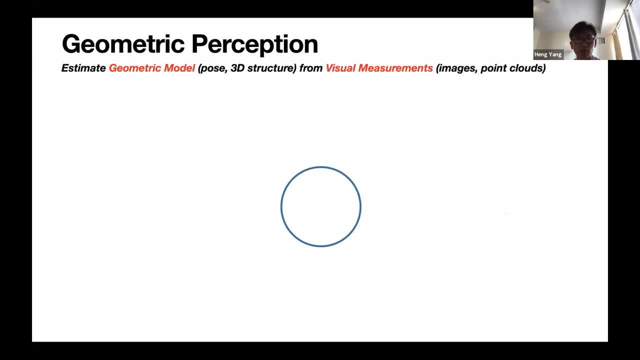 verify if the solution is actually globally optimal. So basically we want to get a posteriori guarantees from it. So before I talk about the technical details, I still want to kind of motivate the geometric perception and also geometric perception with outliers- Geometric perception. 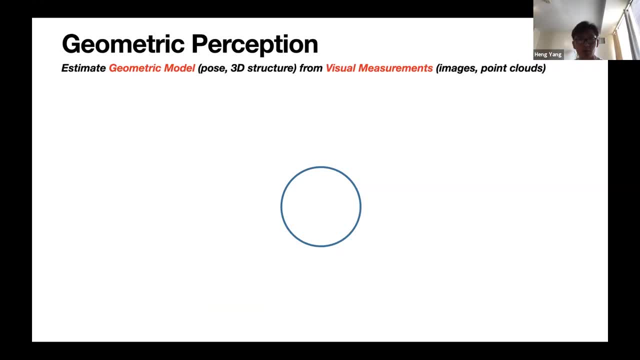 is essentially the task of estimating geometric models from all sorts of visual measurements. The model we're trying to estimate can be poses, can be 3d structures, And then the visual measurements can be images or point clouds, as we have already seen in a previous lecture, previous talks and 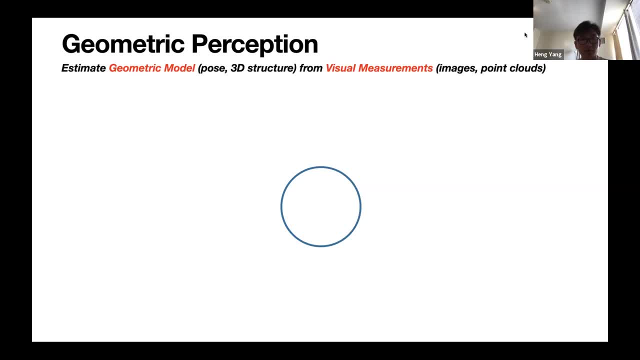 geometric perception spans a whole spectrum of problems. For example, it can be post estimation, it can be a localization and mapping, it can be object detection and 3d reconstruction. And then in robotics we have geometric perception actually underpinning a bunch of applications for 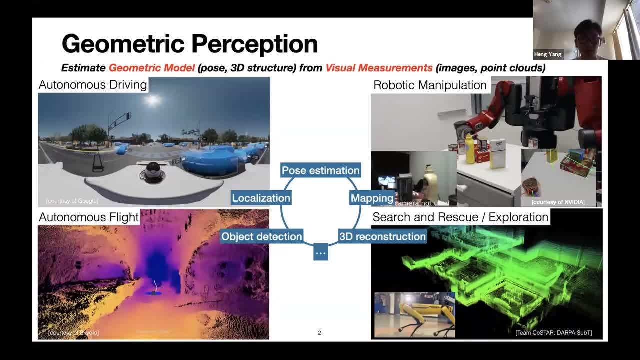 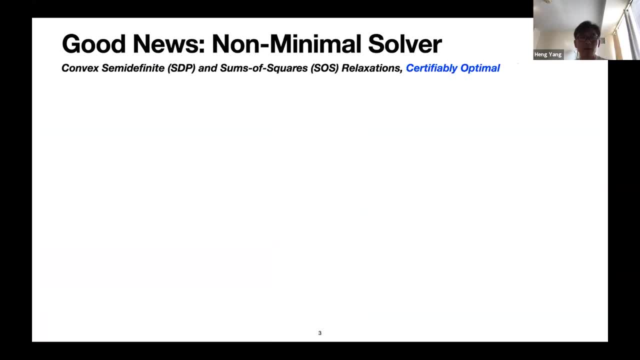 example, autonomous driving, manipulation, autonomous flight and also autonomous search and rescue, a slam, these, these type of applications. And then, as Luca talked about, over the past few decades the community has made a tremendous progress in terms of solving geometric perception with optimality. 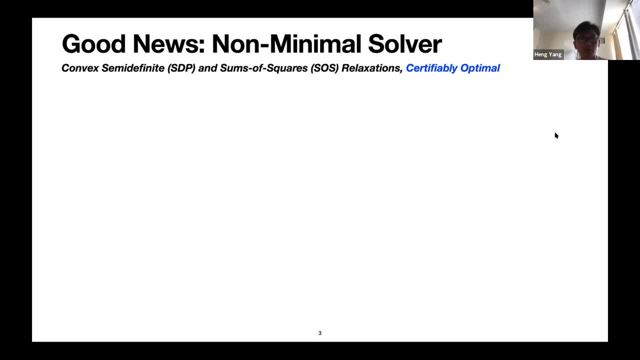 guarantees. in particular, an increasing number of so called non minimal solvers are being discovered, Typically based on convex, semi definite and some more squares relaxations, And the unique feature of these non minimal solvers is that they not only provide an estimate to an to a. 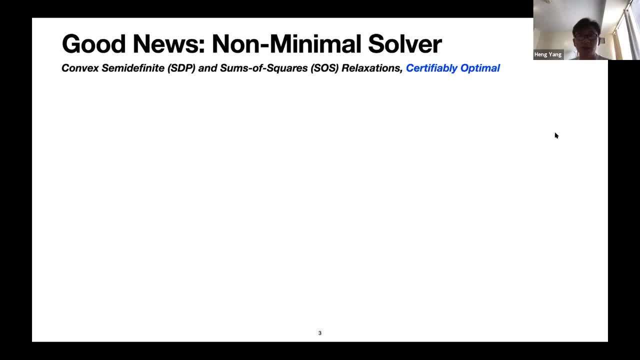 geometric perception problem, but also they provide these optimality guarantees after computing an estimate. So, for example, we've seen examples like mesh restoration, in the case where we have a clean 3d mesh and then we have a noisy point: cloud observation of the mesh And then given all correct 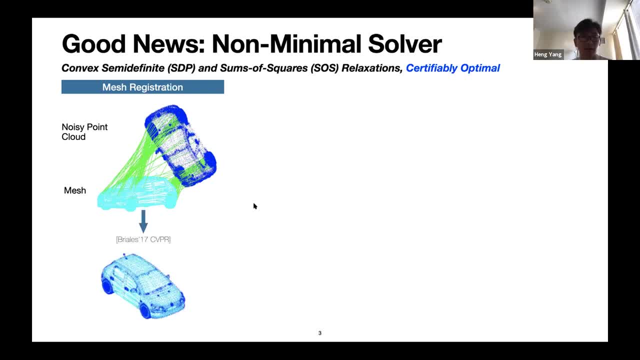 correspondences from the mesh to the point cloud. we have the globally optimal solver, proposed by Borealis a few years ago, that can compute the globally optimal alignment from the mesh to the, to the, to the noisy point clouds, And then we have a shape alignment which is basically we're still given a. 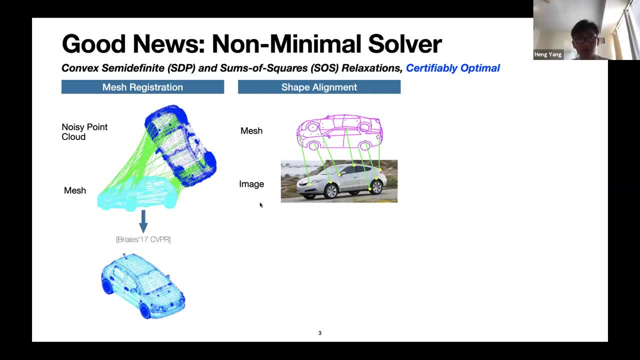 mesh, but now the observation is in 2d, which is just a 2d image of the 3d mesh, And then we're trying to figure out the optimal camera pose of the when observing the 2d image. And then 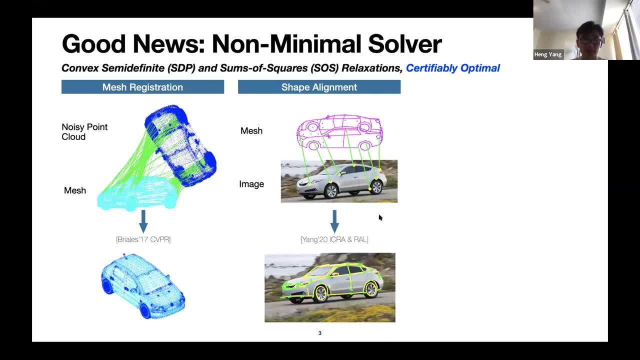 in this year's equal, we proposed a sum of squares based relaxations solver that can actually compute the globally optimal camera pose And eventually, in postgraph optimization- which- which is the example that Luca helped us walk through in great detail- that the famous se sync solver can actually compute the global. 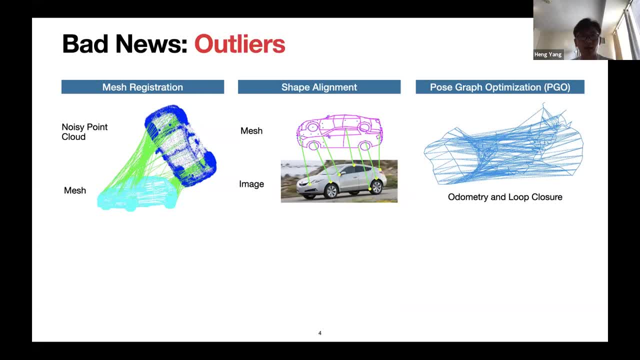 optimum pose graph. But then also, as Luca and TJ hinted, the bad news is, you know, in practice we always have outliers. and then these non-minimal solvers. since they are designed using usually a least squares estimation framework, they're actually not robust to be to two. 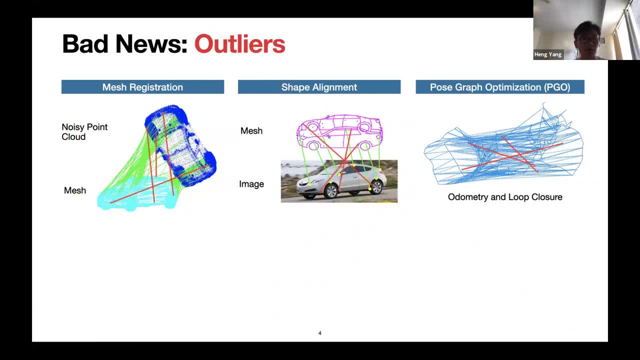 outliers. For example, if we just spoil a couple of incorrect correspondences in these data association, then these non minimal solvers will actually squat, struggle a lot in computing the, an estimate that's actually close to the ground truth, As shown by these images. the estimations provided by the 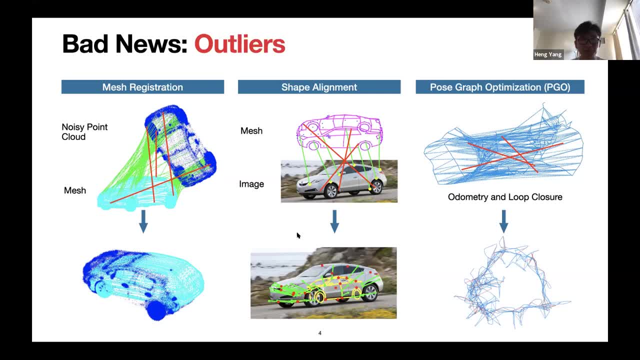 nominal solvers, actually far away from the ground truth. But then what comes to? what comes to rescue is that in in computer vision and robotics, we have a tool set of all our robust estimation that can actually handle these outliers with great empirical performance. For example, from the very classical 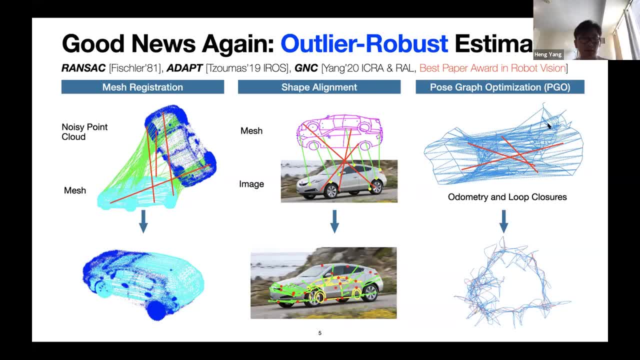 ransack that TJ talked about is actually very fast And usually it gives you an estimate that's actually very accurate. And then more recently in the in spark lab we proposed the adapt and GNC, where adapts stands for adaptive trimming and GNC stands for 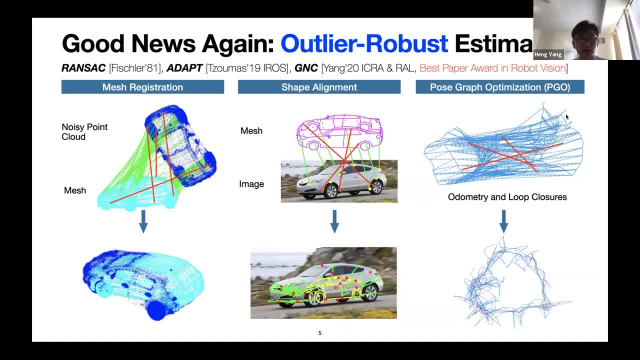 graduated non complexity that can actually also as X, as a general framework to robustify all these nominal solvers. So to give you an example, if we actually use GNC together with the nominal solvers that I've, that I've talked about in the 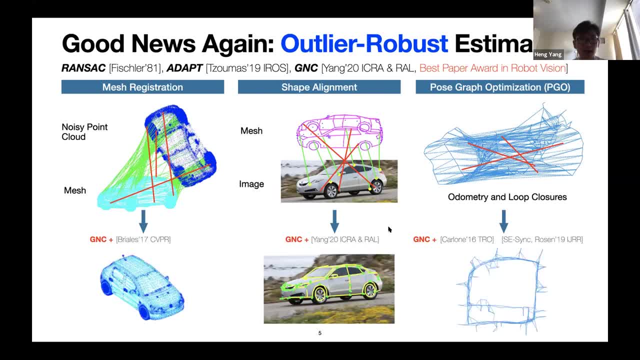 previous slides, then you know the estimates that we can get is actually very close to the, to the, to the ground truth estimation. So you know, in summary, you know we can actually regain robustness using these general purpose outlier, robust estimation frameworks. But actually you 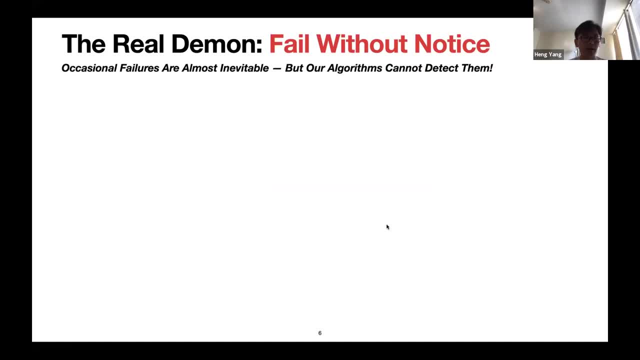 know, in this talk or in this workshop, what we really care about is optimality guarantees, or, you know, basically we want to ask the question: has the solver given me the globally optimal solution? So and then? so basically, we're trying to. 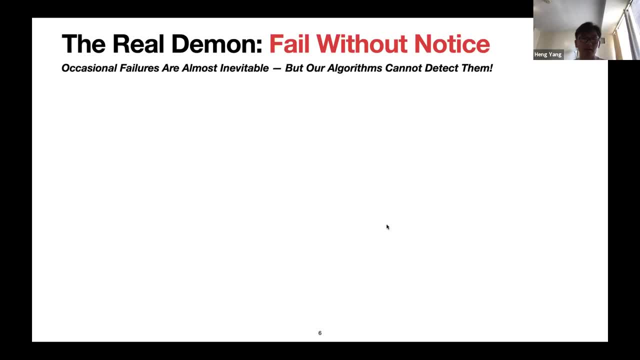 tackle or, you know, deal with the real demon, which is that we want to provide some sort of performance guarantees to these robots. So I'm going to show you some examples of some of the algorithms that we use to try to help you understand the 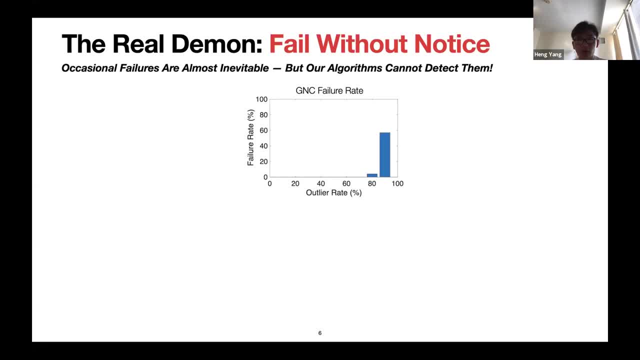 foundation frameworks. And then if you look, then if you look at these ransack or GNC, then you see that these algorithms, typically they perform really well when the ally rate is below, for example, 80%, And then they start failing when, when, 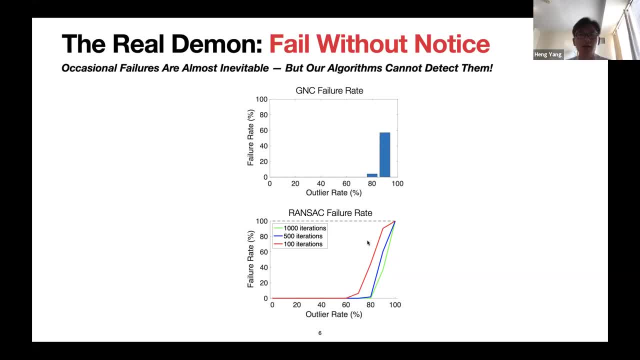 you have more than 80% outliers. Similarly with ransack, it also performs quite well when the ally rate is below 60%, And then And then in these. so then one might ask the question that do these local minima, or do these? 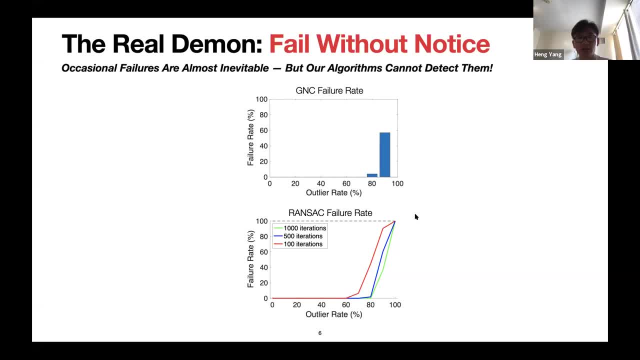 failures are really. do we really care about these failures in practice? So the answer is usually twofold, right? So on one hand, if we are applying these algorithms to entertainment applications such as AR and VR, then probably you don't really care about these. 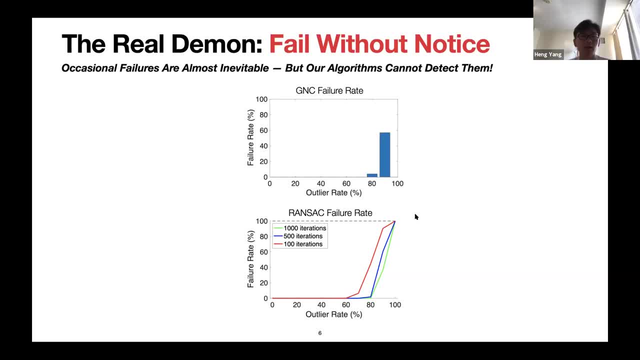 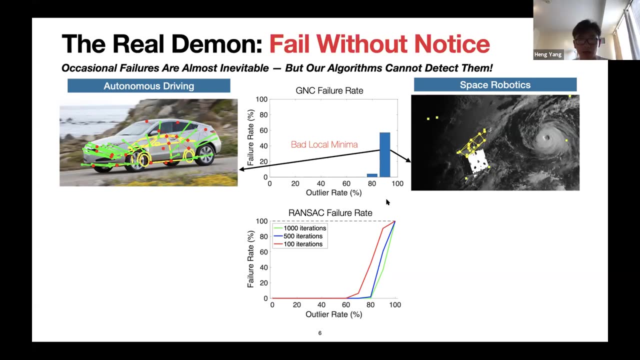 random failures, because they don't necessarily give you any results that are actually very catastrophic. But then if you are trying to apply these algorithms to safety curricular applications such as autonomous driving or space robotics, then these bad local minima are actually going to translate to catastrophic damages to either human life or the machines that 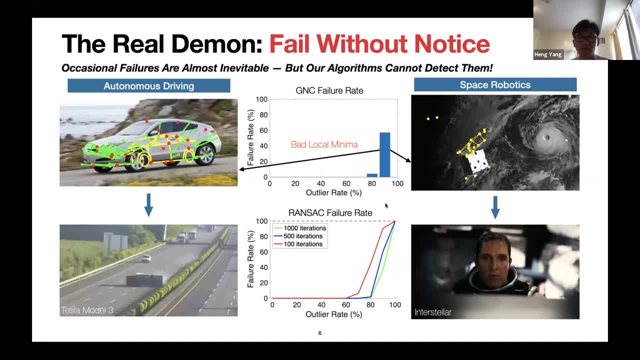 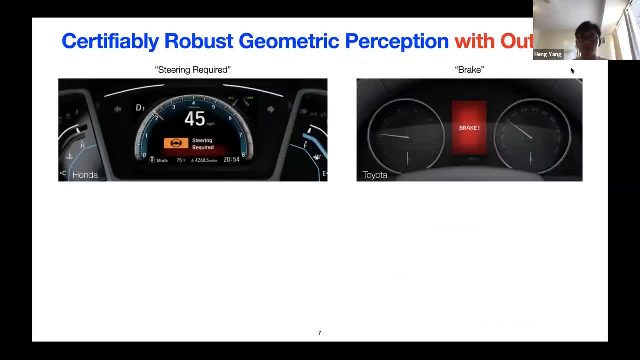 could possibly be really expensive, or we just cannot afford These failures. So, then, what we propose in this workshop is to use certifiably robust geometric perception without wires. So, in a nutshell, I think these algorithms probably have already existed in the current driving or driver driving assistance systems. For example, if you drive 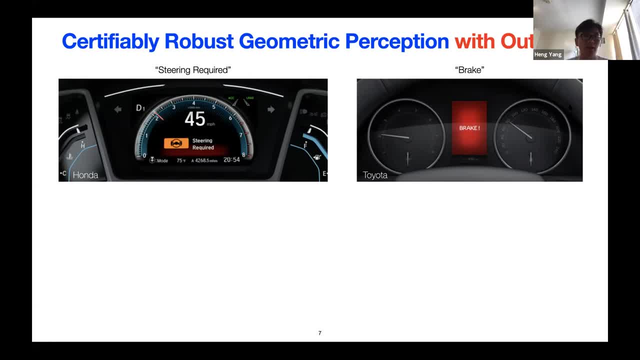 something like Honda or Toyota. they have these safety packages that if they're going to steer the wheel for you in the highway, in most cases they can- they can do it correctly, but then when they are not confident of their actions, they will actually signal these uh uh red signals. alerts to. 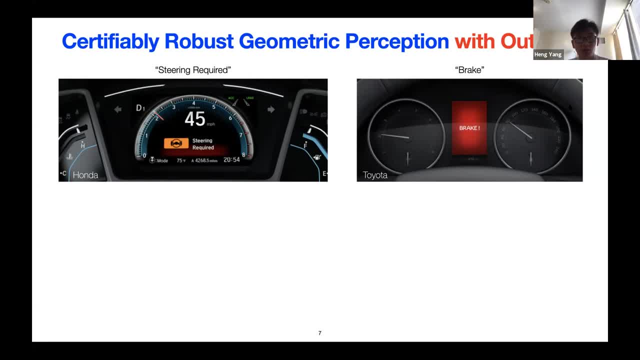 you such that you know you want to take the. the person might need to take the wheel back or simply to break the car when, when the condition is too dangerous. so, and then to provide uh, to put these certifiable, robust, geometric perception in the context of modern perception, uh, pipelines, uh in. 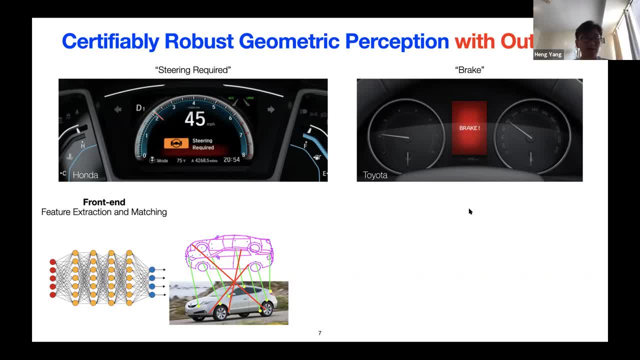 modern perception pipeline. we usually have a front end that does feature extraction and matching in. in these days usually it's a neural network based uh pipeline and then they're going to output these, these puritive correspondences between uh visual measurements, for example from the 3d mesh to the 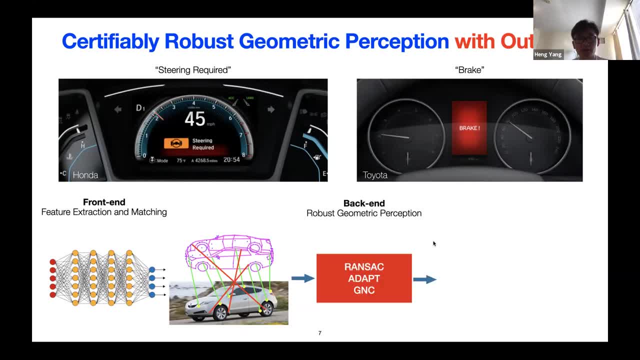 2d image and then in the back end we're performing some sort of robust geometric perception. uh, these days it's mostly ransack. adapt or gnc is very kind of very efficient, but uh, but algorithms that do not provide any guarantees. so they're going to give us some sort of estimates. these estimates are: 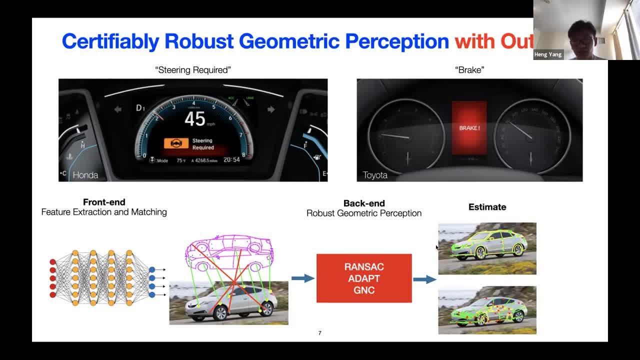 most likely going to be correct, but in some rare cases it does fail, as i, as i showed in the previous plots about the failure rates. but then these, uh, as i also motivated you know, these random, these rare, rare cases of failures will actually hurt you when you try to apply these algorithms to safety critical applications. so what? certifiably robust? 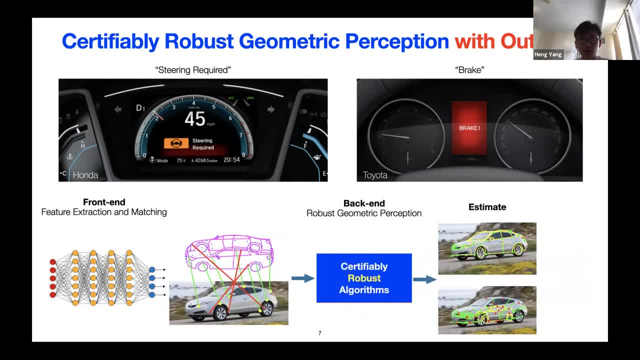 geometric perception does is that it's going to replace these ransack, adapt or gnc with some algorithm, algorithms that can actually certify these estimates. so, basically, it will not only compute an estimate, but it also gives you a certificate of when the estimate is correct and when the estimate is not correct. and i also want to just want to stress that, also stress the 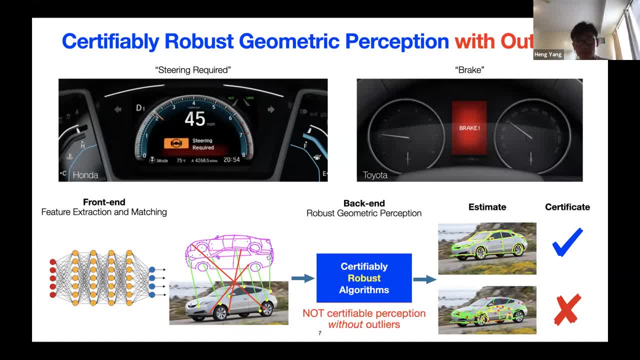 fact that these are�� by uh luca and tj. so these these certify robust algorithms are actually uh significantly different from these certifiable perception. without without outliers, as i'll as i will show uh this difference into, uh assume they actually differ in two main aspects. so the first: 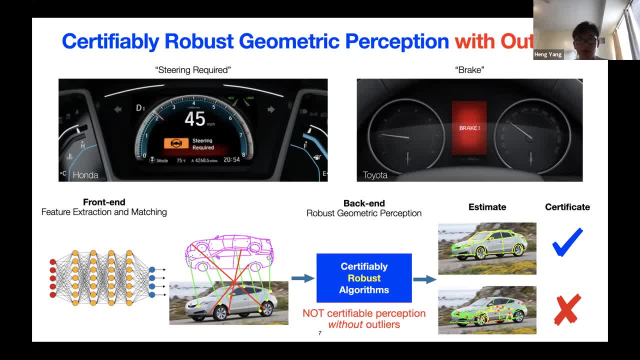 main aspect is that in certified robust algorithms we uh explicitly consider outliers, and then we use a robust cost function, that that is known to be robust to outliers, and then the second. the second difference is that when you're trying to relax these, these problems, it becomes significantly more challenging and then it requires some more tool sets, tools. 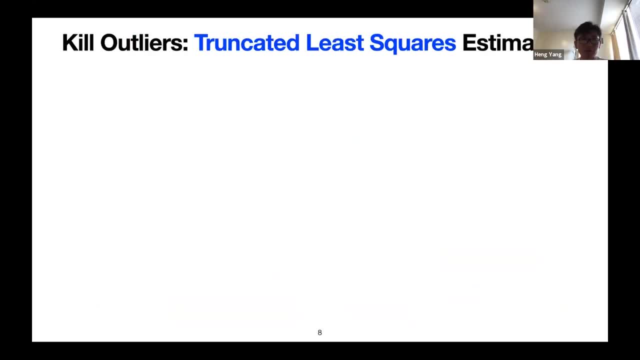 from optimization and apply mass. so the first difference, as I as I hinted, you know the- we're going to use a robust cost function that's called truncated least squares. and then this, this robust cost function is going to help us kill the outliers so as, as TJ already introduced geometric perception as we 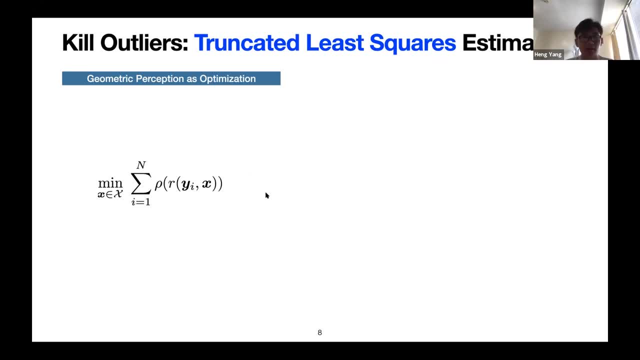 can treat geometric perception as a general form of optimization, and then in this optimization we're trying to estimate the geometric model to know it as X, and then we are given visual measurements to know it as Y, and then we have a residual function. for example, it can be the Euclidean distance in 3d. 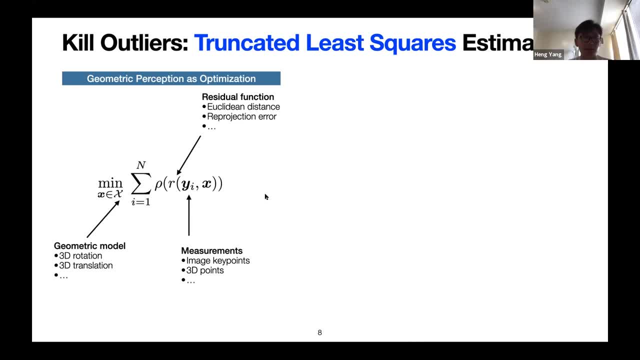 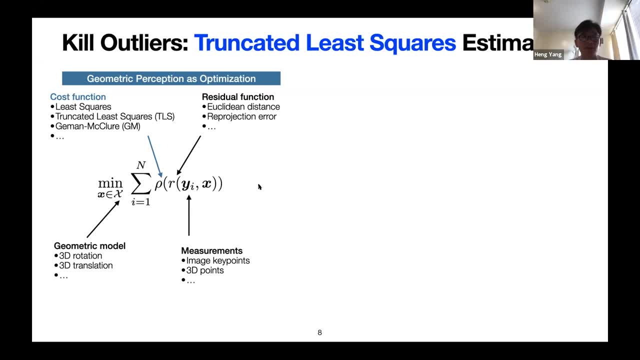 non-robust case is least squares. and then in the robust case, TJ has a part of all sorts of robust estimation cost functions. so to give, just give you a very simple example, to to actually to insert instant, to give you an example of this optimization problem in 3d restoration, when you have all correct. 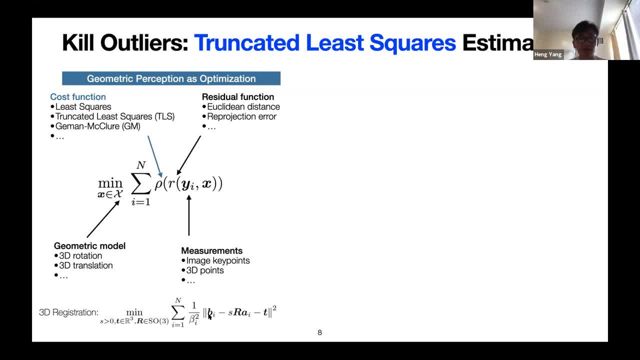 correspondences. we're trying to estimate the scale translation rotation given visual measurements bi and a. we're not dealing with data by natural 백신 x, so this is nothing more than we're dealing with data by natural fx-trainers. it equals a Bayesian truth. this available now and capabilities for 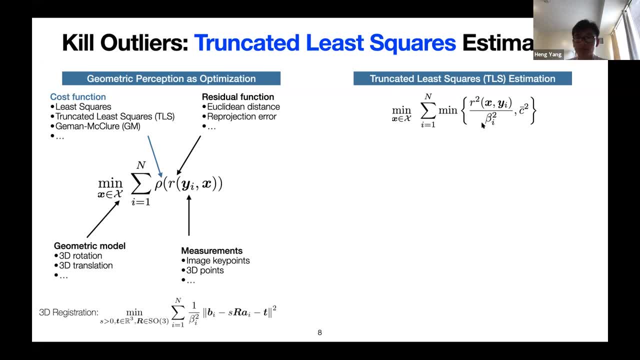 threshold C bar square. And then if you look at this inner minimization more closely, then you will realize that when the residual is actually small, which usually means that the corresponding measurement yi is an inner layer, then the minimization will prefer the residual function, which is 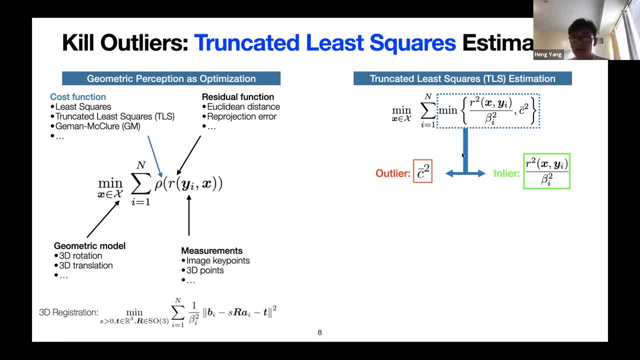 R square, But on the other hand, when the residual is actually larger than C bar square, which is the constant threshold that we've set, then this outlier will not be penalized, so it will become a constant. that will not affect the solution of the optimization. 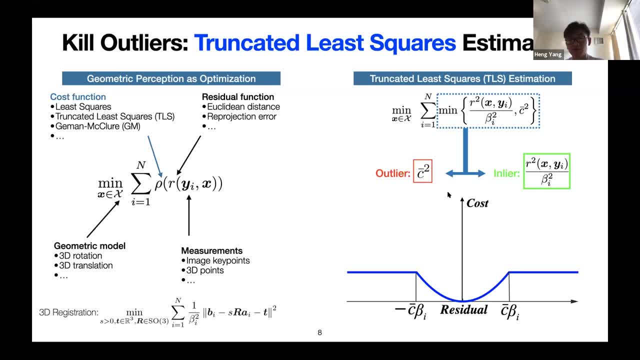 Pictorially, the TLS estimation cost function is a truncated least squares, and then the inliers will be mapped to the least squares part, and then the outliers will be mapped to the horizontal constant part. And then you know these. since outliers are mapped to the quadratic part, it's going to be preserved and then the outliers will be killed. 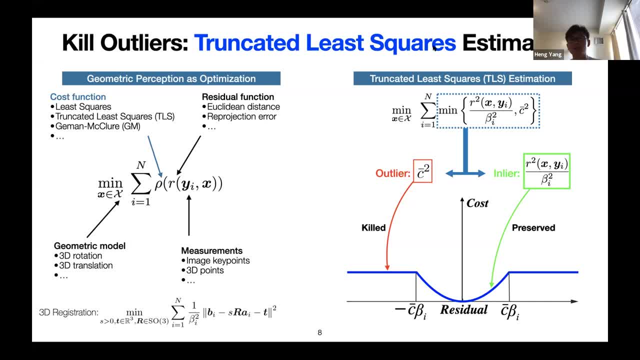 And, as TJ showed, this TLS estimation is theoretically hard to deal with, as can be seen from the non-convex shape of this cost function, And also it's also non-smooth because you have these, you know- sharp edges as 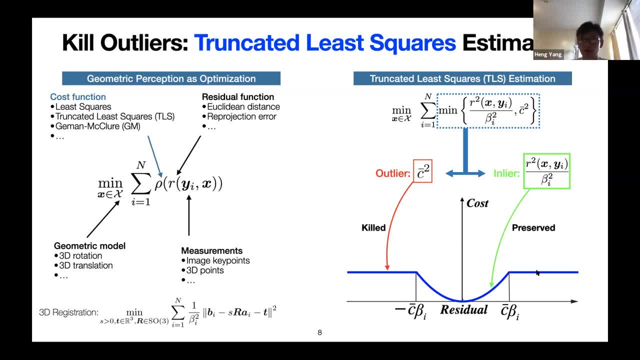 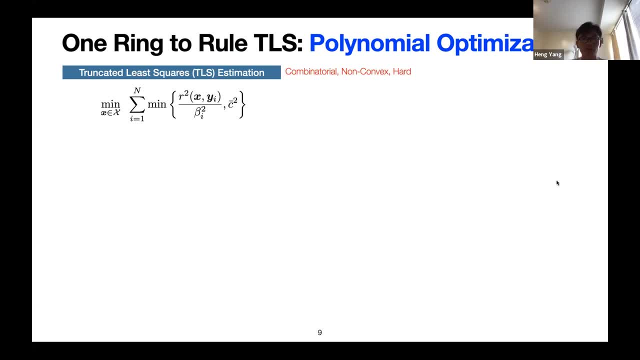 transitions from the quadratic part to the constant part. And then, in the next slide, I'm going to show the ring that can rule TLS, which is the ring of polynomials, And then we're going to use polynomial optimization tools to rewrite this TLS optimization problem. 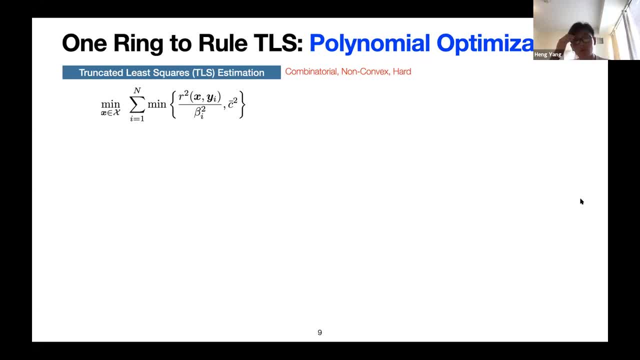 And then you know, this TLS estimation framework, as written here, is combinatorial, it's non-convex and it's hard. And then we're going to use, we're going to take a closer look at this inner minimization And we realize that this inner 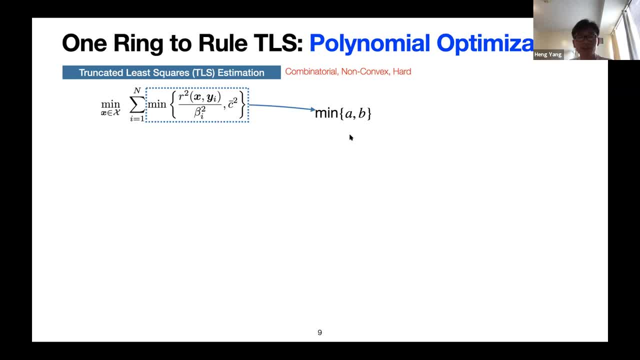 minimization is nothing but a minimization of two scalars, a and b. So the a is just a residual divided by beta i square, and then the b is just c bar square. And then one realized that this minimization of you know. 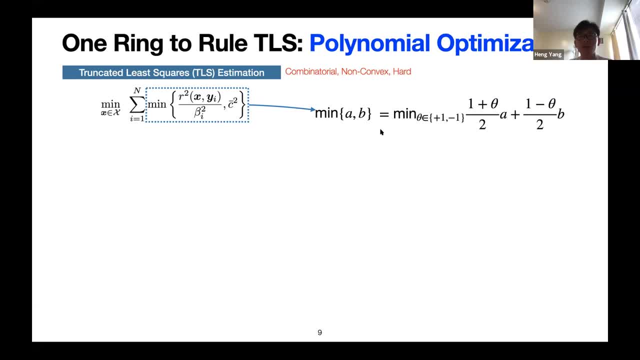 simple minimization of two scalars can be written as a minimization over a binary variable, theta. So if you check this left hand, right hand side, when a is actually smaller than b, this minimization will choose theta to be equal to plus one, and then 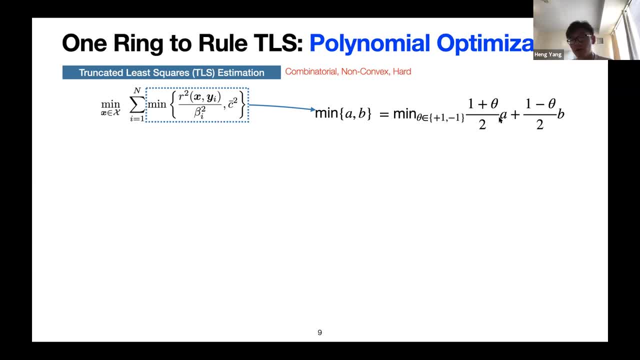 this objective function will recover a And, on the other hand, if a is actually larger, is actually larger than b, then the minimization will choose b by setting theta to be minus one. By using this trick, we're going to rewrite this inner minimization as now a function of. 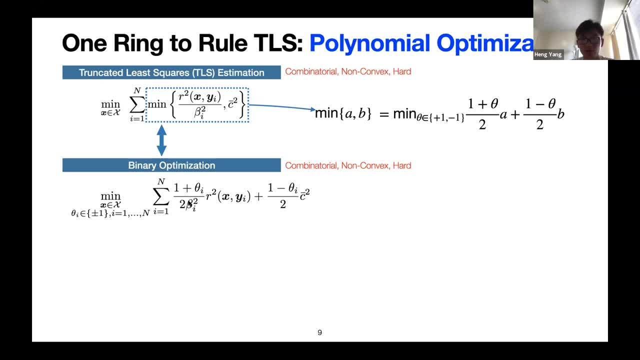 the x and y as well as the thetas that we have introduced. So note that we have introduced one theta for each measurement, yi. So now the optimization becomes binary optimization, which we know that is still combinatorial, non-convex and hard. 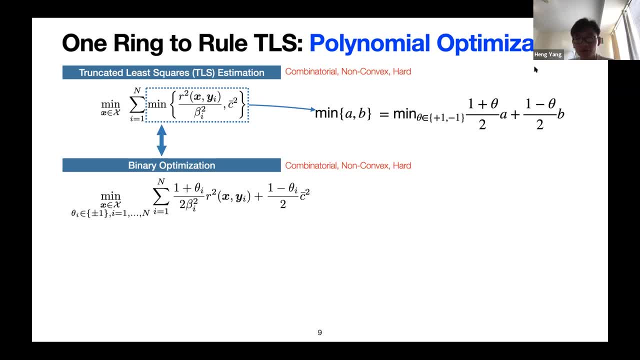 But then this comes to the nice feature of TLS, TLS framework, which is actually, you know, these thetas are actually, although they're binary, but they can actually be written in a continuous fashion, So which I will show here, that you know. 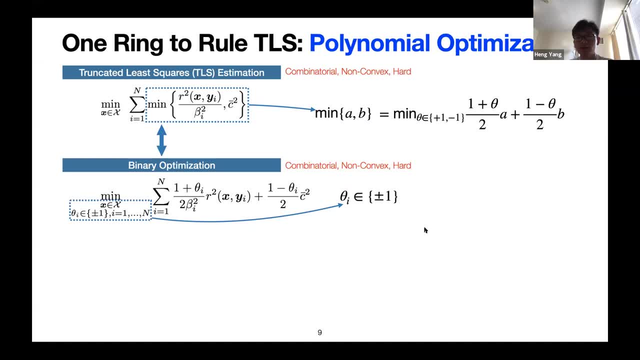 by enforcing theta to be either plus one or minus one. it's equivalent to saying that theta i square is equal to one. So on the left hand side you know this is a combinatorial problem. But on the right hand side you actually go back to the continuous optimization land. 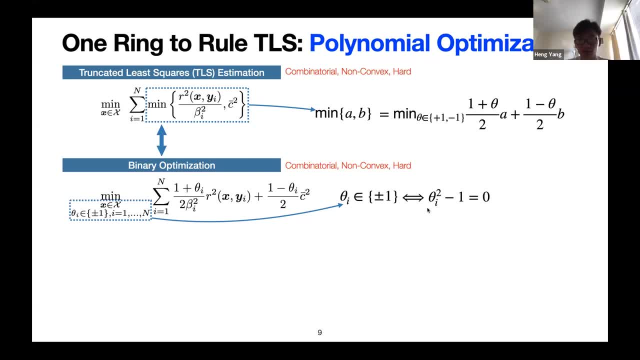 So this is the first nice thing about this TLS estimation framework. And then one also realized that for common geometric perception problems the x is usually the rotation matrices or translation vectors, And they usually live in a space x, calligraphic x- that can actually be described using a bunch of 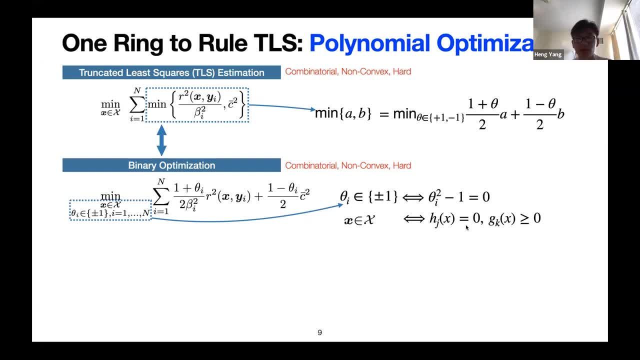 Poinomial constraints. For example, the Luca has shown that the r is, you know, in the orthogonal group of orthogonal group O. three can be written as r times r, transpose equal to one. And then if you look at the look at that constraint element, wise, it's actually just a. 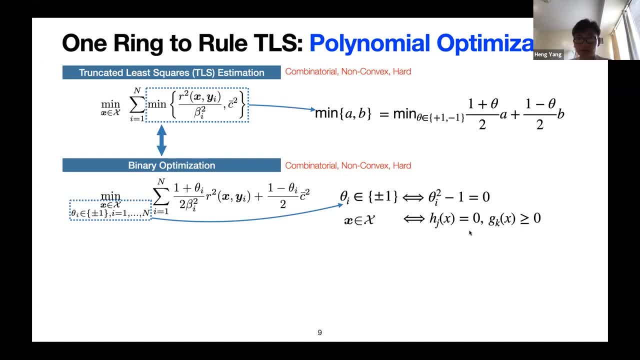 system of polynomial equations, equalities or inequalities, And then by stacking the x, which is the model that we're trying to estimate, together with the binary variable thetas, which actually will tell you if, if some measurement is actually inline or outline. 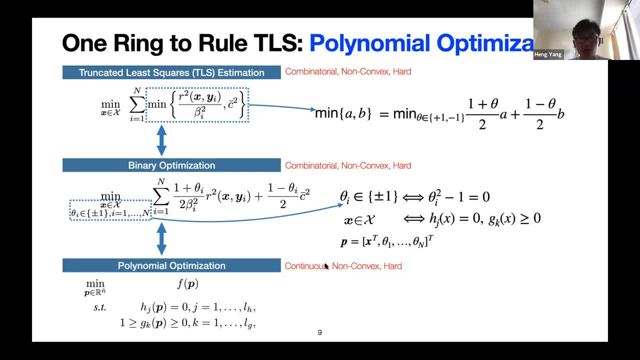 we're going to rewrite this optimization as a continuous polynomial optimization on the on this new variables p. So now this is a standard form polynomial optimization. So you might wonder, so you know this, since we have these double ended arrows here. 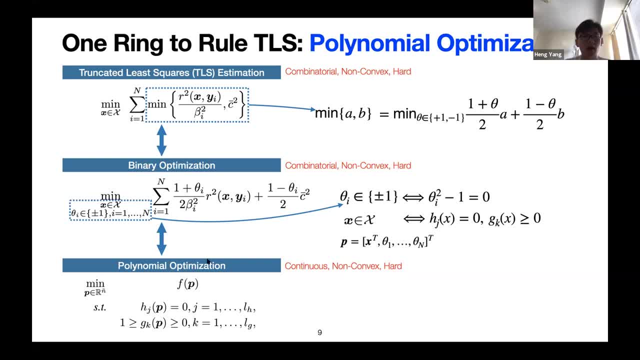 so the polynomial optimization is actually equivalently hard as the TLS estimation. It's. although it's continuous, it's still non-convex and hard to solve. But then, as hinted by Anders and also Luca, the formulation really matters. So now that we have written the TLS estimation in this polynomial optimization framework, we can do something. 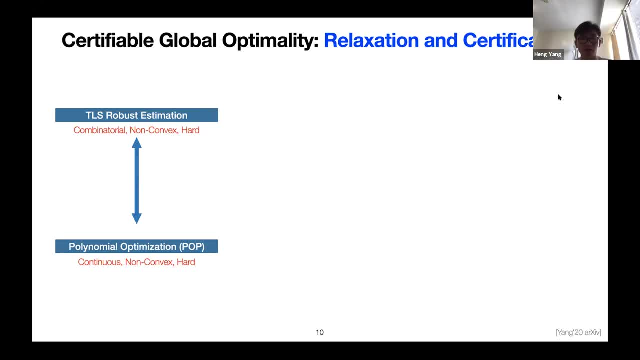 that's very kind of standard in the optimization literature, which is actually to relax and do certification, So to to build up, to establish these certified robust solvers, I'm going to propose or claim that there are actually exactly two ways of designing certifiably robust geometric perceptions. 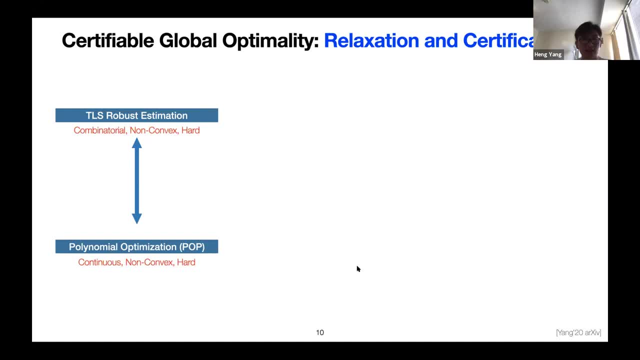 So one way of of designing or relax this problem is actually to directly try to directly tackle the polynomial optimization problem. So what we're going to, what we're going to do, is to relax this non-convex problem to a convex one. 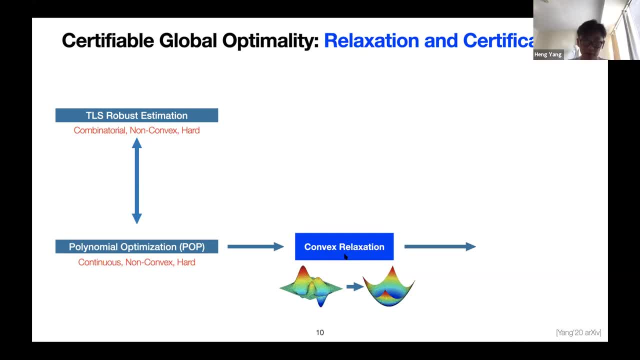 which we call convex relaxation- already talked a lot in the previous talks And then by you. by solving this convex relaxation, which is usually, we'll admit, will becoming a semi-definite programming- you can obtain an estimate but at the same time you can get a certificate, or when the 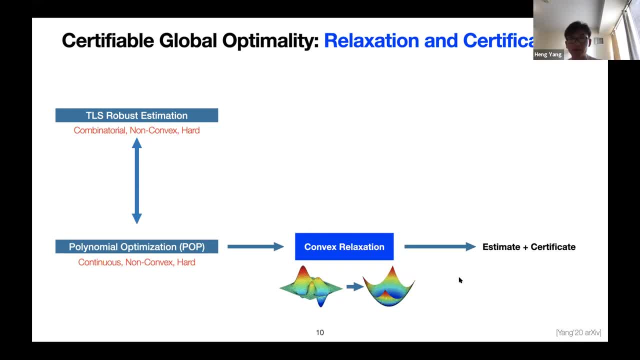 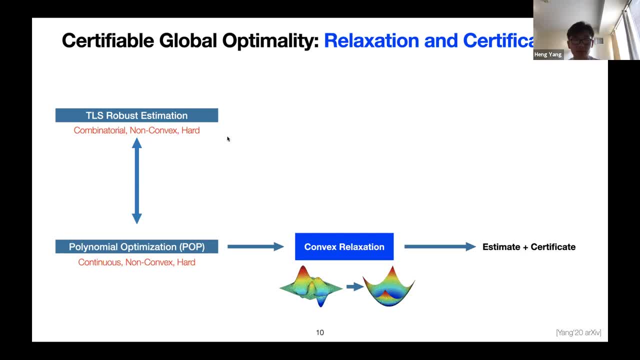 method of designing certifiable algorithms, which is which is actually. we will directly solve the TLS- robust estimation using fast heuristics such as RANSAC, ADAPT and GNC, which will give us an estimate. and then, but now we're not going to stop here, because we care about global optimality. 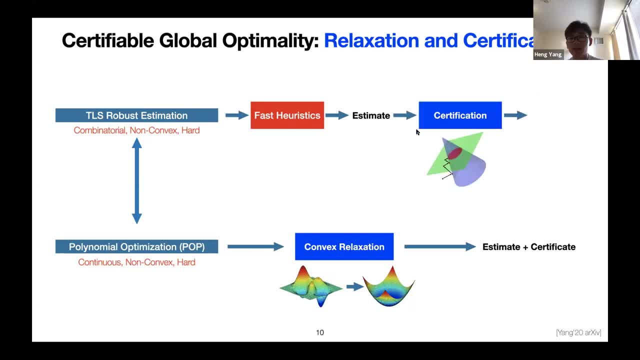 And then what we're going to do is we're going to take these estimates and then we're going to perform certification or verification that will give us a return, a certificate for this estimate, And then- so this is the general, the high level view. 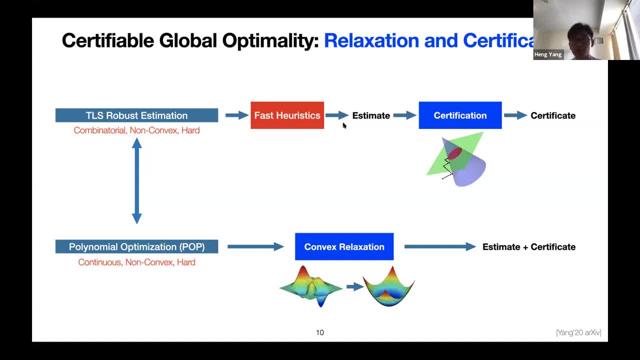 the high level view of doing, of signing certifiable algorithms. more specifically, what are we going to do, or what are we? what tools are we going to use to design a convex, relaxation and certification of of any estimate? So I will introduce, not me, 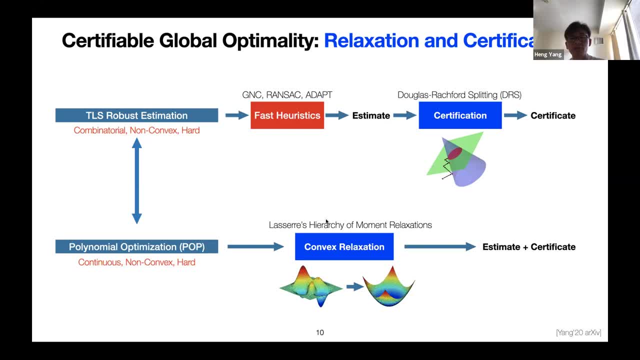 So it already exists in the application literature for convex relaxation. We can use Lasserre's hierarchy of momentary relaxations, which is which has has great similarity with SDP relaxation or or relaxation of QCQPs, but it's a more powerful hammer that can deal with more general polynomial optimization problems. 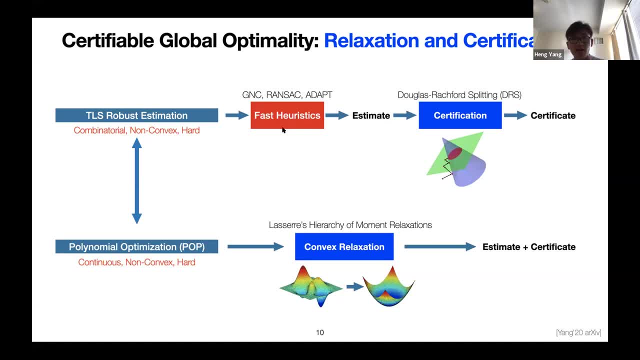 And then for the fast heuristics, which is, we already have them. We have. we have a GNC, RANSAC and ADAPT- all these fast heuristics. that performs really well in practice. but then for the certification we're going to use a different. 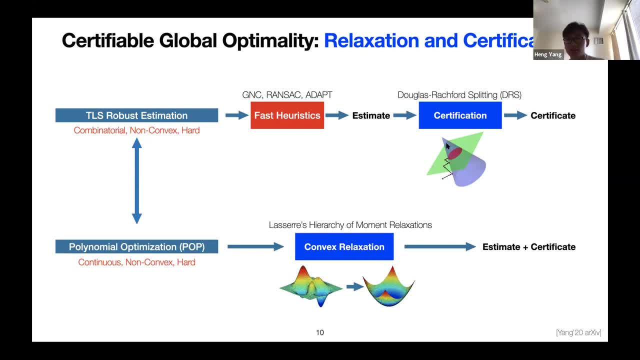 different optimization technique called darkness rational splitting, which is different, which which is, which is different than directly solving. solving that, an SDP And then this DRS, will actually offer some scalability benefits to two to our problems and which I will show in the next few next few slides. 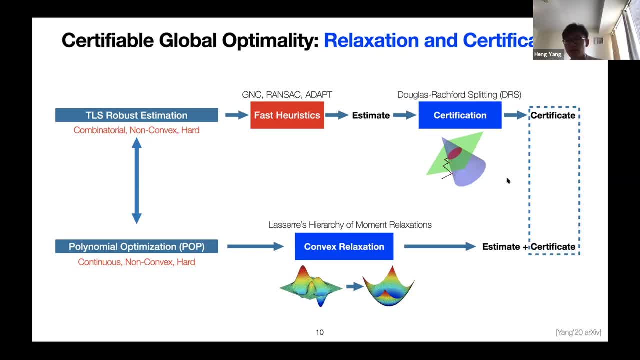 And then what I'm going to stress here is that the certificate is actually a suboptimality gap, which will basically tells you the distance between your estimate and the global optimal solution. And then back to Ender's talk. this gap is also basically the duality gap, or when the gap is zero. 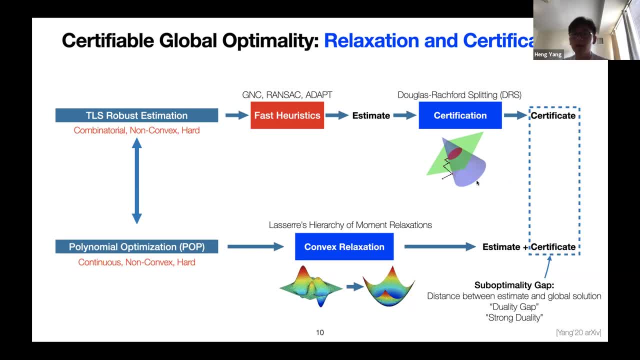 we say that this problem actually has a strong duality. and then, for a more fancy view or for more precise view of these two, two lines of designing certifiable algorithms, the convex relaxation is actually the primal perspective which we're going to, which we relax and non-convex problem directly and we solve the convex problem. 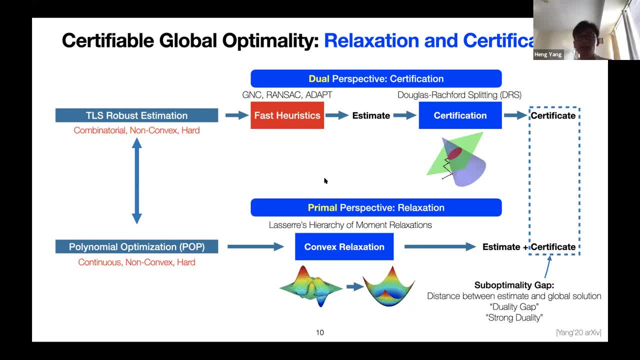 And then the dual view is actually doing certification which has given any result. Can we claim something about this estimate? Can we say that this estimate is global optimal or not global optimal? Okay, So these are really the very high level to overview of this, of certifiably robust geometric perception. 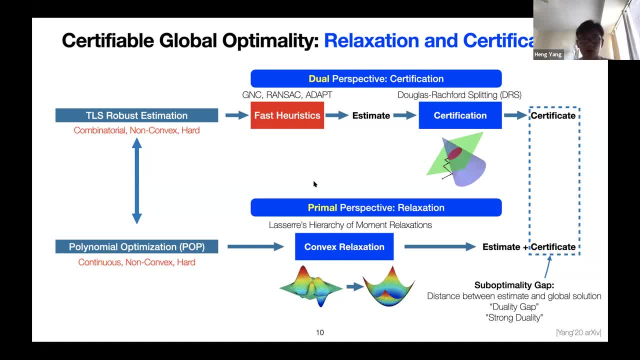 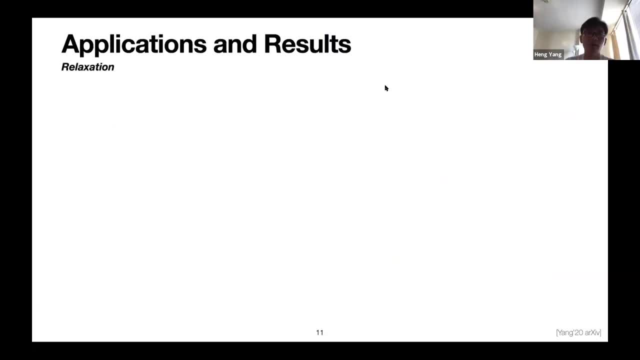 I'm not going to talk about the technical details of each of these blocks, And you know, later I'll point you to the correct references. but now I'm going to show some promising results of these two lines of research. So the first result I'm going to show is: how well does relaxation perform in the presence of outliers? 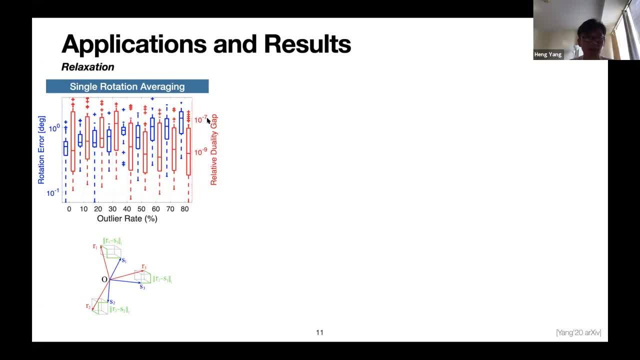 So in here I'm showing a plot where on the X axis I'm showing an increasing number of outliers and on the left axis, which is highlighted in blue, I'm showing the rotation estimation arrow in degrees. and on the right hand side. 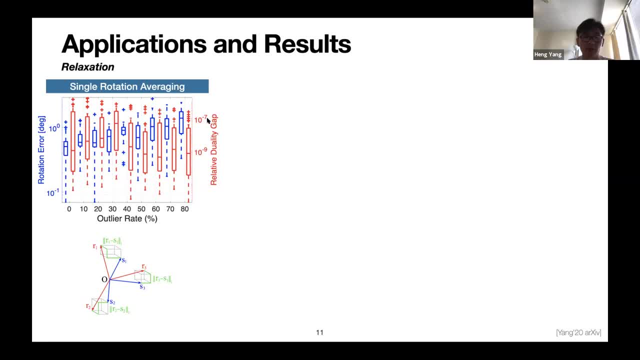 I'm on the right axis. I'm showing the relative duality gap. all the you can take it as suboptimality gap of the estimate with respect to global optimal solution. So this problem I'm showing here is called single rotation averaging, using the TLS, robust cost. 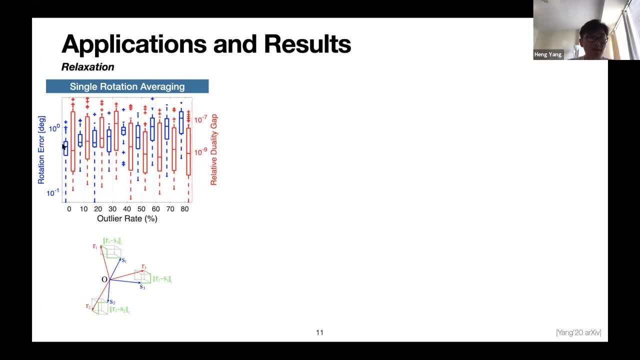 So, as you can see this, this relaxation performs quite well in terms of rotation arrow. The rotation arrow is usually below one degrees and at most it can be five degrees. So it's basically it's very accurate and, more importantly, you see that by solving the SDP, 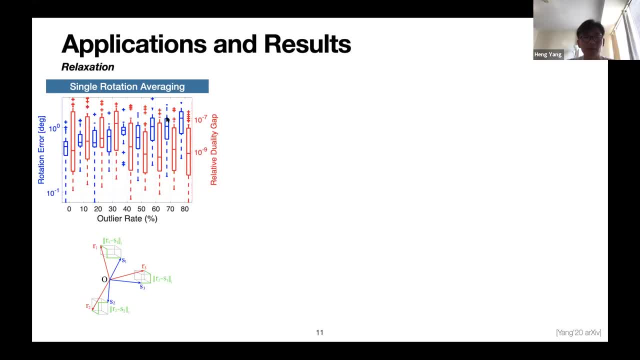 we get the relative duality gap, and the duality gap is usually very, very small. It's 10 to the power of minus seven or minus six or even smaller. So which means that you know your, your solution or your estimate is only a very 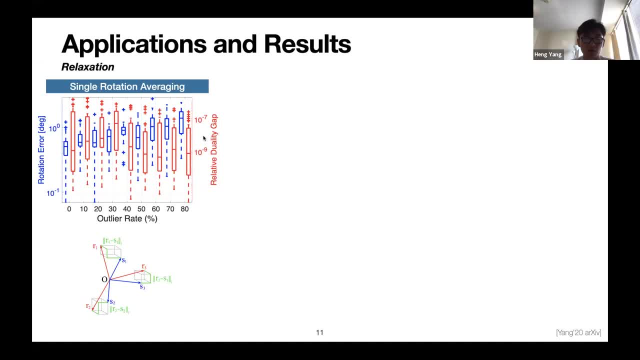 very, very tiny distance away from the global optimal solution, or numerically you can take it as zero. So this basically tells you: you know the old solution, your estimate is the global optimal estimate. And then I'm showing similar results for shape alignment and measure registration. 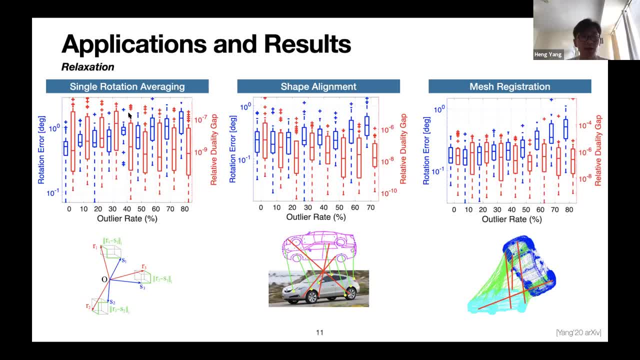 which are actually more complicated, more complicated applications and single rotation averaging, And you will, you actually encounter these problems in robotic perception. So a similar results carry over to these more more complex, more complex experiments. You see that the rotation arrow is very tiny. 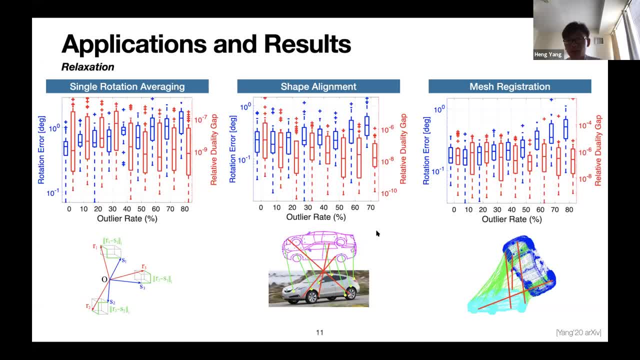 And then the relative duality gap is super small, Although sometimes, you know, there does exist cases where the- when you have a very high ally rate, the solution, the relative duality gap, can be non-zero. in this case, in in the rest circle. 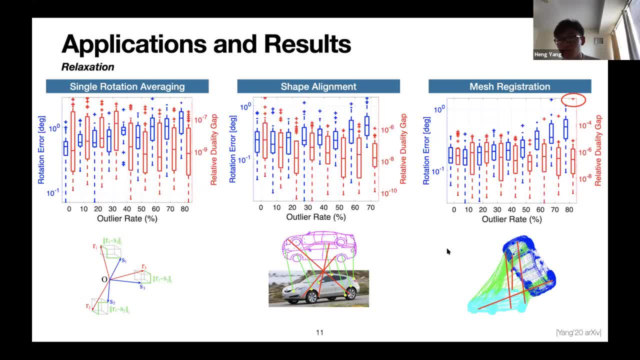 I'm showing in a case where you have a duality gap, that's a 10 to the power of minus two, I guess, which is small, but not not zero. But in that case you still see that rotation arrow is actually very small. 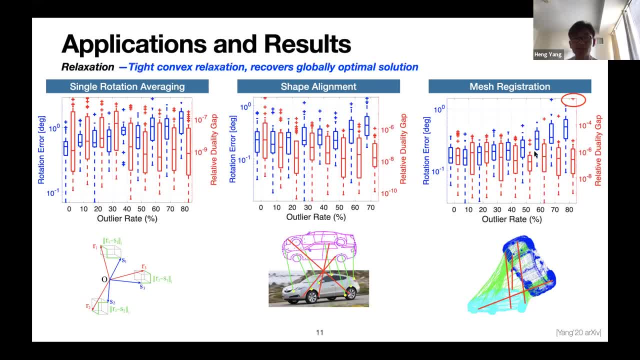 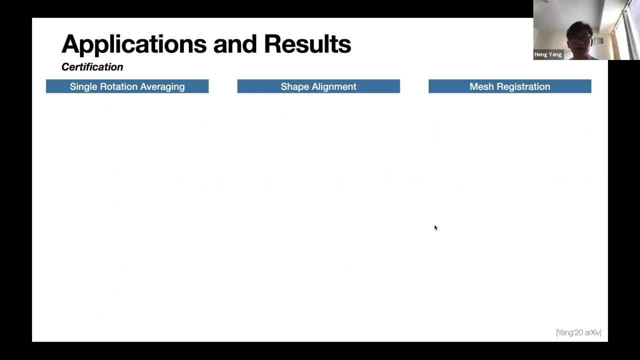 So basically the takeaway here is we have achieved a tight convex relaxation for a different whole, for a whole spectrum of geometric perception problems. And you know, in these relaxations we can actually recover the global optimal solution. And you have. you also recover a certificate using by. 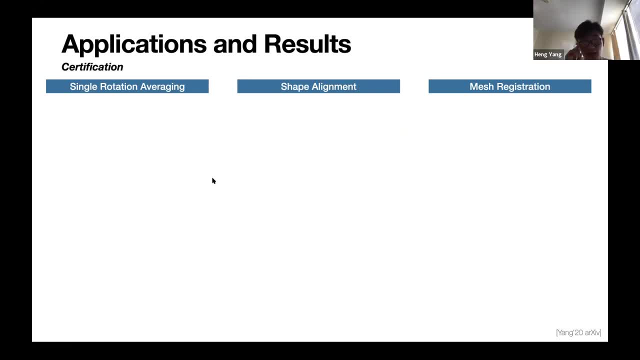 by looking at the duality gap And then on the on the on the other line of designing certified perception is as a, as a show, which is doing certification. So certification is different than relaxation, Basically, you know, in the certification. 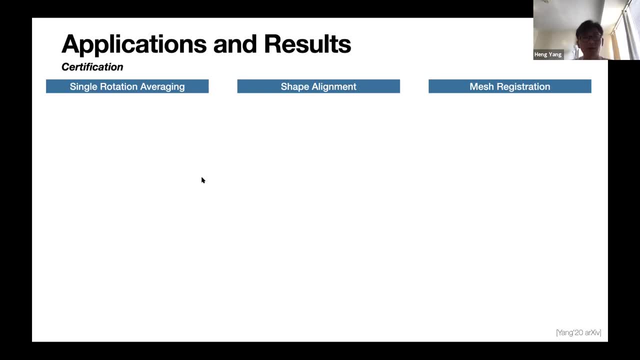 you actually have two steps Now. in the first step, you solve the TOS problem directly using RANSAC or GNC- these, these heuristics that do not offer you guarantees- And then you're going to, you know, add another layer of these heuristics to try to give them certificates. 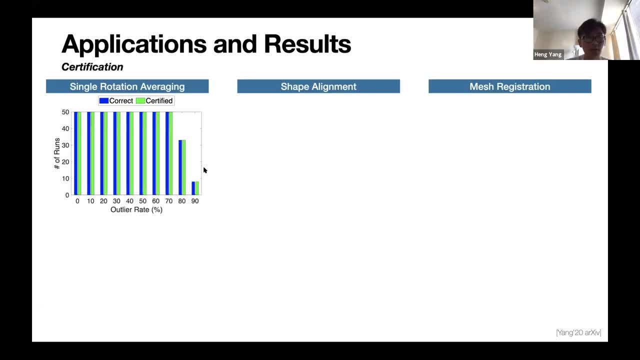 So in this case, where I'm showing results in in in two bars of different colors, So in the blue bar I'm showing results that I run you, I run GNC, And since these are synthetic results, synthetic data sets, 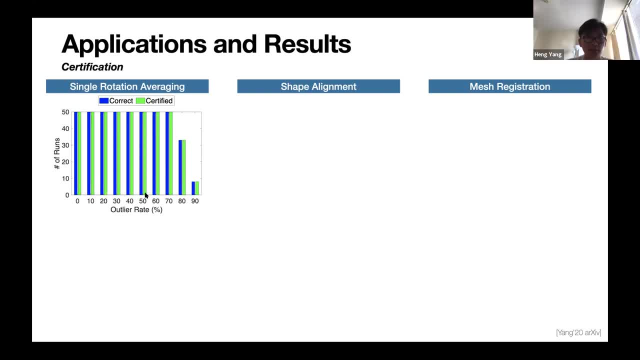 I can. I know which ones are actually the global optimal solution. So the these blue bars showcase that empirically. if I run random runs, for you know, for for 40,, for 50 times, how many times do GNC or RANSAC give me the correct solution or the 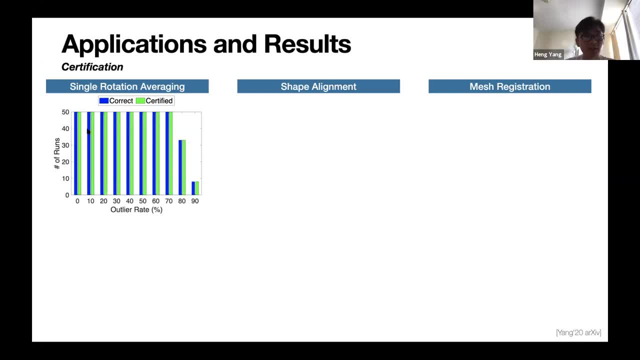 global optimal solution. And then the green bar shows that for each of these solutions can I certify them as correct or incorrect. So you will see that for all the correct solutions, for all the correct estimates, our DRS certification pipeline was able to certify. 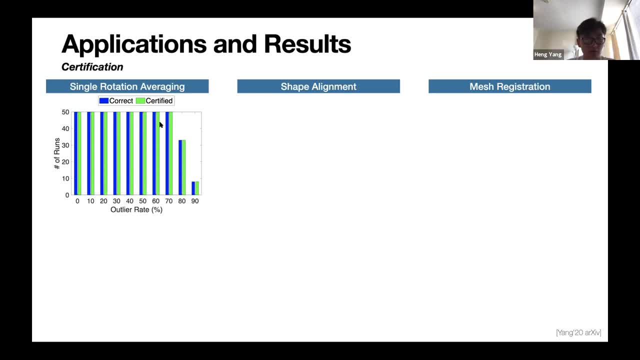 to provide the correct certificate for these solutions And then, more importantly, when the GNC actually fails, they- you know their estimates- will not be certified. So this gives you a way of detecting, of detecting wrong solutions in RANSAC or GNC. 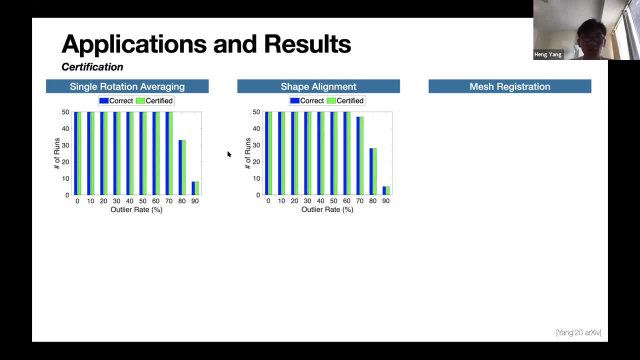 And similarly I'm showing the results of shape alignment or a mesh restoration. You see that the same results, the same results, the same results, the beautiful results carry over to shape alignment and mesh restoration. We were able to certify all correct solutions. 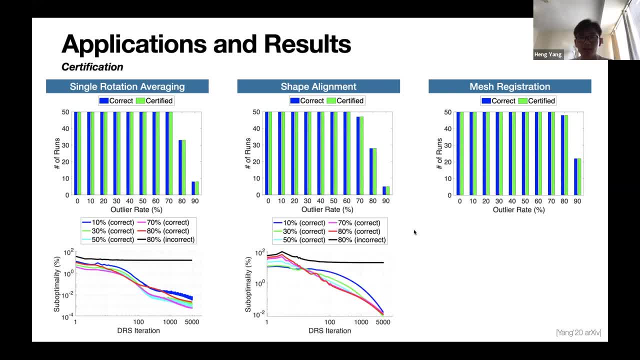 and we were able to project all wrong solutions. And as a as another you know- metric of showing the success of the certification, I'm plotting the sub-opinion gap with respect to the iterations of Doppler's Rashful Splitting. 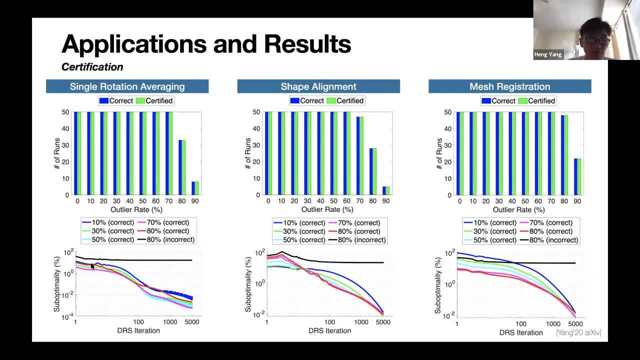 which is DRS, And you'll see that for these, for these correct solutions, the, the, the certification was able to to drive down the sub-opinion gap below 1%, or you know 0.1%, Really fast. 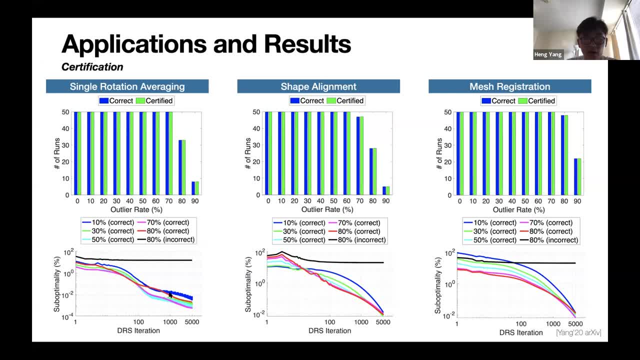 usually within 100, 100 errations or 1000, 1000 iterations. And on the other hand, when you, when you give an incorrect solution or incorrect estimate to the certification pipeline, the certification, the sub sub-opinion gap will actually saturate also very fast. 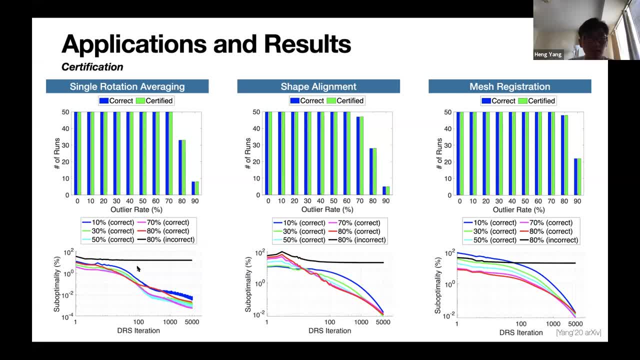 So you see, there's this. there's this very clear bifurcation of correct solutions and incorrect solutions. So correct solutions will give you a sub-alternative gap of below 1% or 0.1%, And then incorrect solutions- its sub-alternative will saturate above 10%. So this gives you also a very 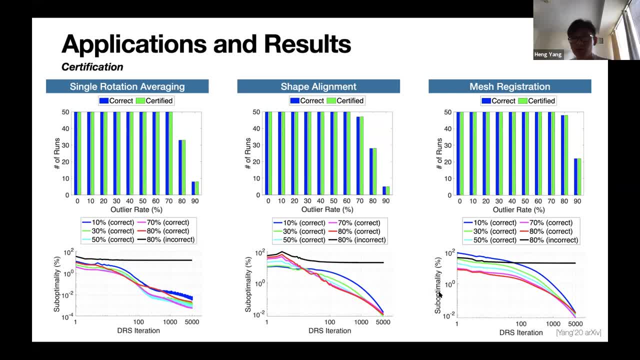 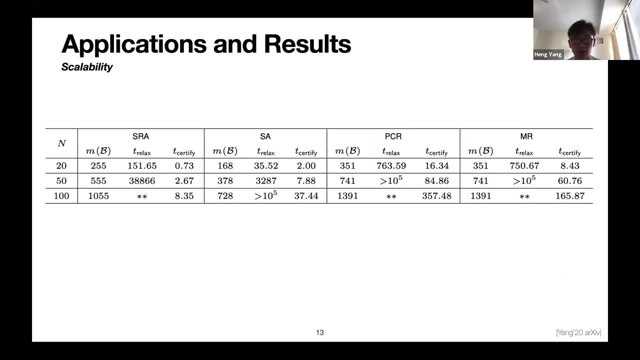 clear idea of when to accept a solution and when to reject the solution, And then you know. the takeaway here is we were able to certify correct solutions and reject incorrect solutions. And lastly, I want to show the scalability of convex relaxations. So usually people will say that 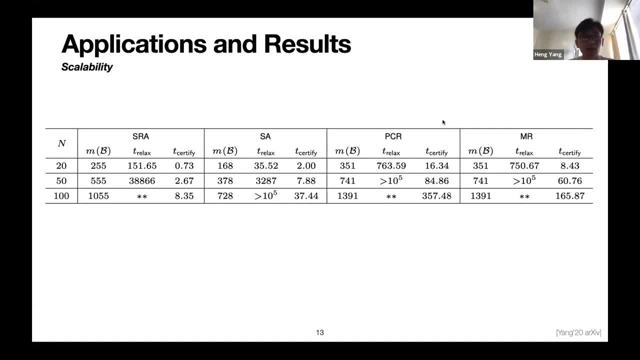 convex relaxations involve solving a large-scale STP and they will not be scalable to real-size problems. but here I'm showing that this statement is partially true. So in this table here I showed the n is number of measurements for each of the previous. 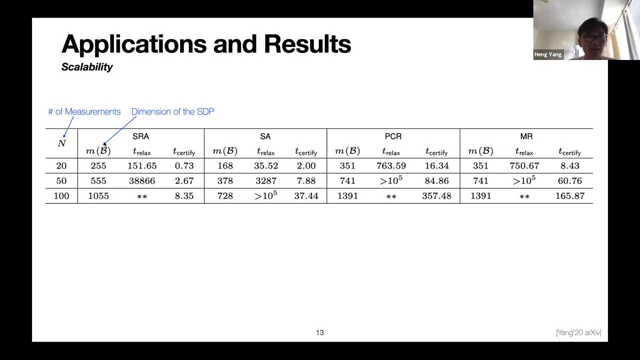 problems that I talked about. And then this n is a dimension of the STP, And then the T equals the mean of the dimension of the STP. So we can estimate the motion by assuming that the mass of negative Claire, even then S equals theogen underlyingieni in a state S cross. 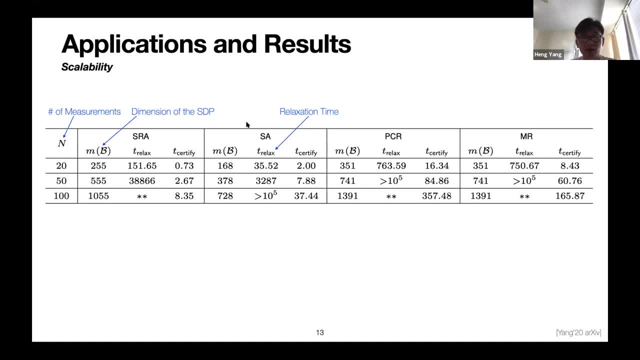 The SOs, leading to the gain of positive Claire. even then, S equals gustFine, So we can estimate T-RELAX is a time that's used to solve the STP directly, for example using MOSAC, which is a commercial state-of-the-art IP solver. 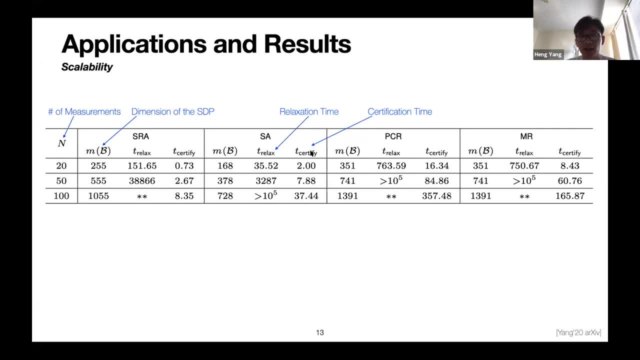 for solving STPs And then the CERTIFY. the T-CERTIFY is a time that's needed to perform certification. So basically, I run GNC first and then I give the. I try to certify the solution of GNC And then SRA, SA, PCR, MR are just shorthand. 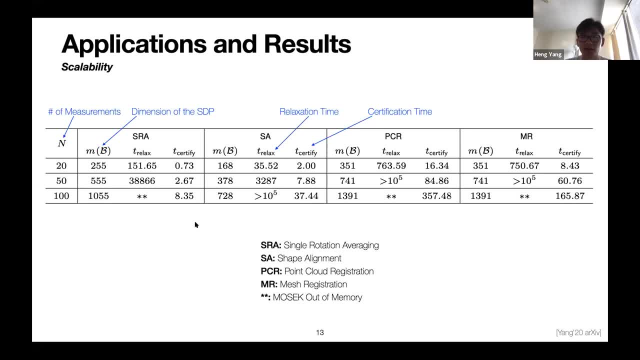 for four different applications, And the double star means that the cases when MOSAC, the STP solver, runs out of memory, And you see that when N is very small, which is 20, this is far away from real size problems- You can still solve the STP. 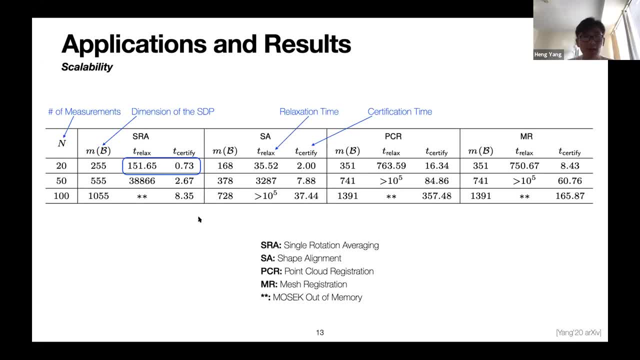 but compare. if you don't solve the STP directly but you're trying to do the certification of the solution, then you end up with a much faster pipeline that only takes you less than one second or a couple of seconds. But then, when it goes to 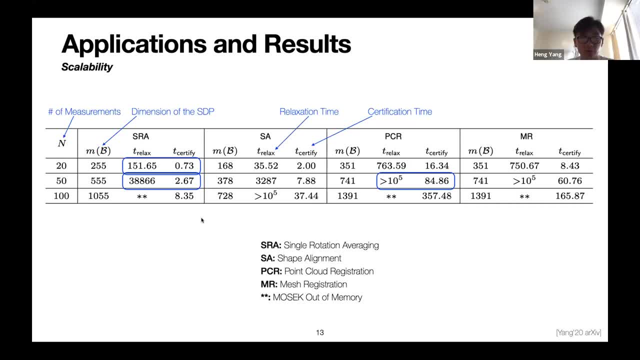 larger size problems, when you have, for example, N equal to 50, then you can still solve the STPs. but it will take you a few hours or even one day to solve this STP, which no one will do that in practice. 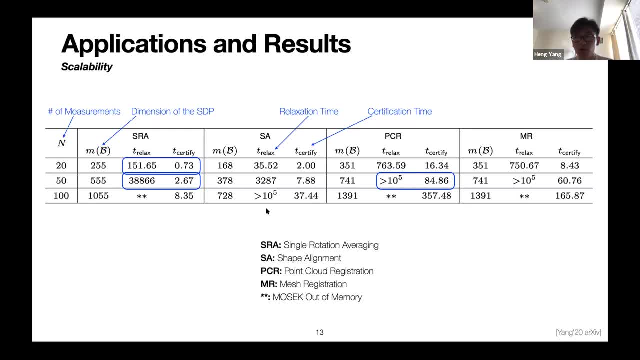 But certification can still be wrong in a reasonable amount of time, Not close to real time, but this is very promising. You see a reduction of time, probably a thousand times or faster. And then when we go to N equal to 100, which is a problem of realistic size, 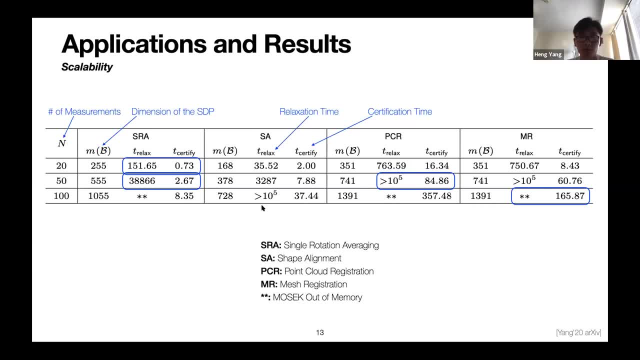 the STPs will basically be not implementable. You just cannot solve it, you cannot squeeze it into the memory of your computer, But then when you do certification, you can still do it in a couple of minutes or a couple of seconds. So this is really promising, as I see. 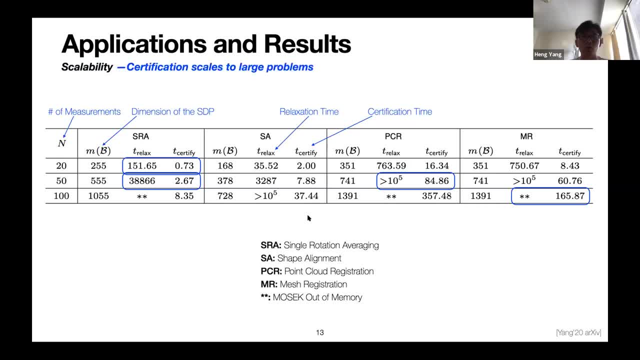 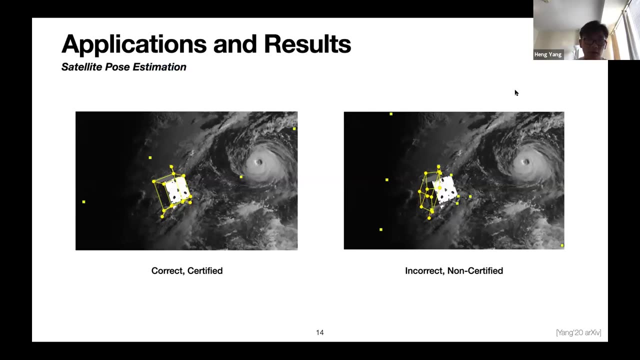 certification skills, large problems And also in certification. we're not completely abandoned previous solvers such as RANSAC or GNC. You're actually leveraging their performance And I'm showing. next I'm gonna show two examples of applying these certifiable perception algorithms. 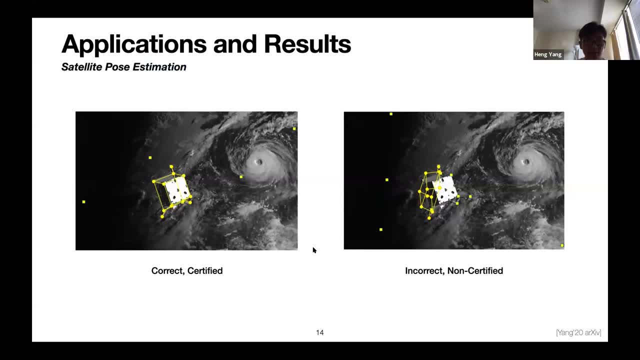 to real world applications such as: the first example is satellite pulse estimation, Thanks to TJ for providing the datasets. So in the left image I'm showing a solution that's correct and also certified, And on the right hand side you do see that the GNC actually converges. 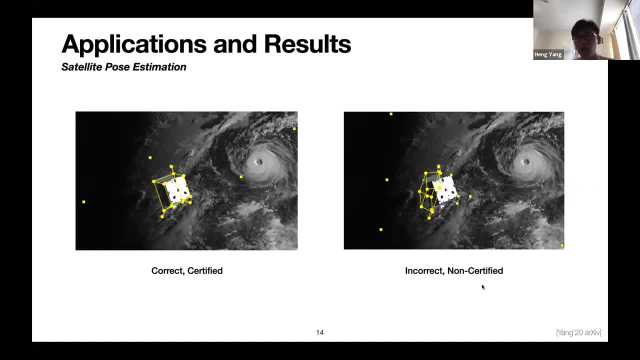 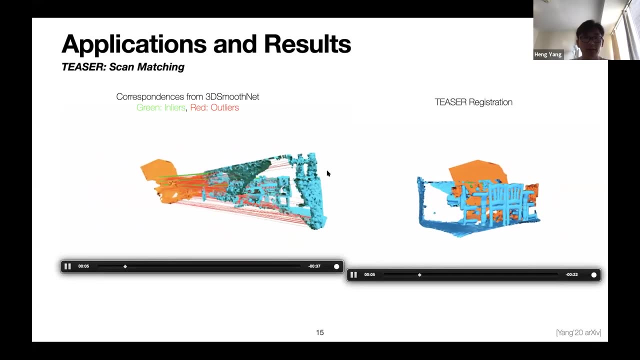 to a local minima, which gives you an incorrect estimate, but our certification algorithm was able to declare this as a failure case, So you were able to reject this solution And in the teaser case, which is a point- cloud registration- we show that the teaser can actually run on problems. 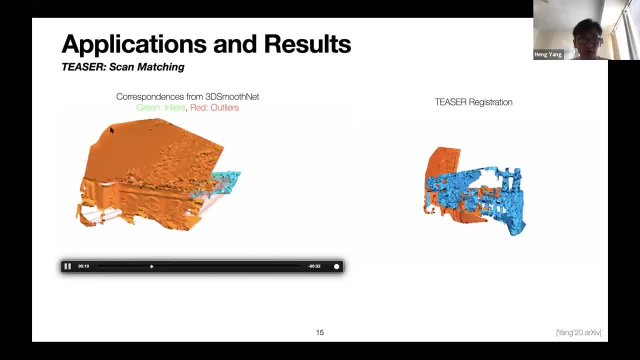 of really large size. In here on the left video I'm showing two scans with correspondences obtained from a deep neural network. of course 3D smooth. It gives you a lot of outliers, as shown by these red lines, but then teaser is super robust to these outliers. 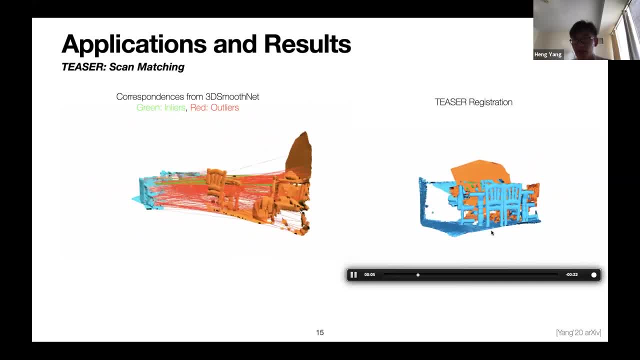 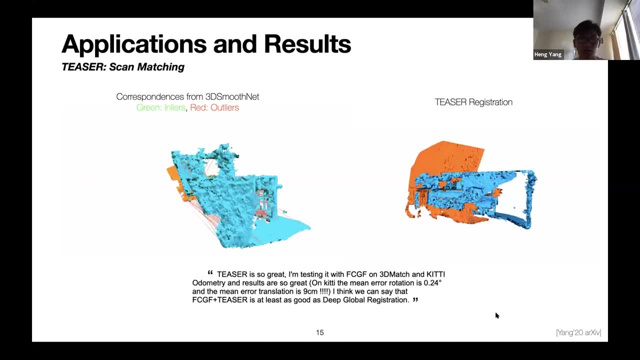 It can give you a very accurate estimate And it also will tell you this estimation is correct in the sense of correct global optimization. And as I'm showing a quote here by someone else running our algorithm- you see that teaser, although it's a handcrafted algorithm. 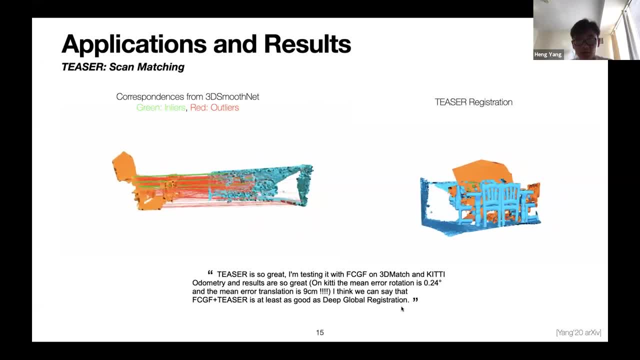 without end-to-end learning, people will comment that the teaser is really so great And it's at least as good as deep neural registration, which is a state-of-the-art deep learning pipeline which just came out of this year's CVPR. 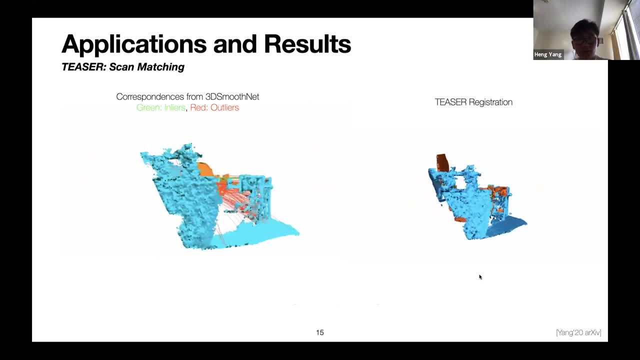 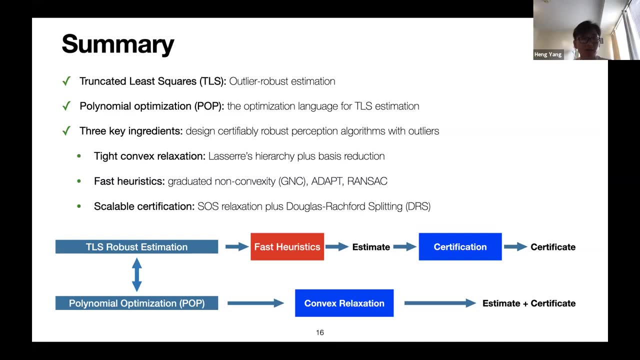 So we are really proud of this work And eventually I'm gonna show a summary of this recent results. So three of these key things to remember is that, first of all, we use the truncated least squares. That's the outlier, robust estimation. 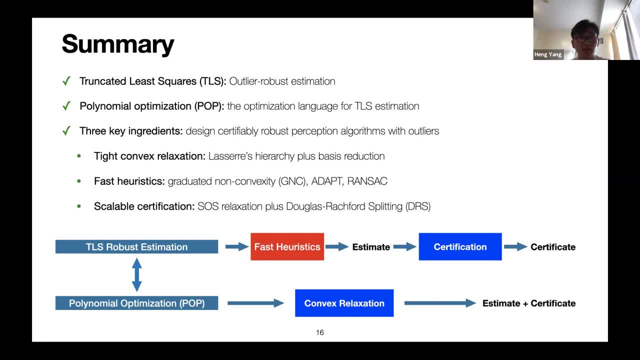 that will kill these outliers. And then, second, is we bring in the tool of polynomial optimization, which is the optimization language for TLS estimation. And then the key thing is that, in order to design a certifiable, robust pipeline, we need three key ingredients. 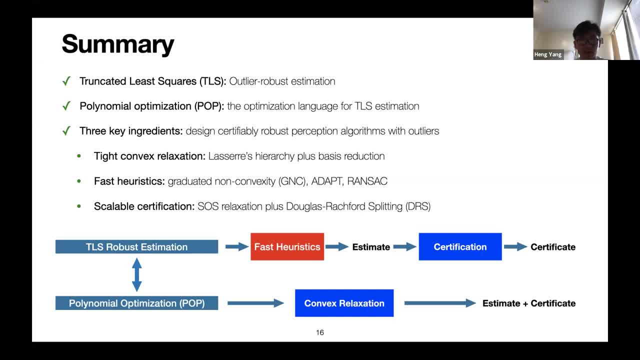 So the first ingredient is that you need to have a tight convex relaxation- In this case it's the series hierarchy- And then we also need a fast heuristics in order to do certification. So imagine that your fast heuristics just gives you garbage. 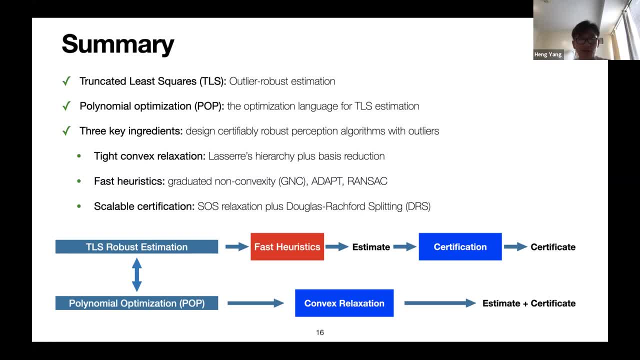 Then the certification will not do anything right, Because every time you give it a wrong solution it will tell you it's wrong, And then this doesn't help for real work performance. So these fast heuristics with very good performances are, from my point of view, 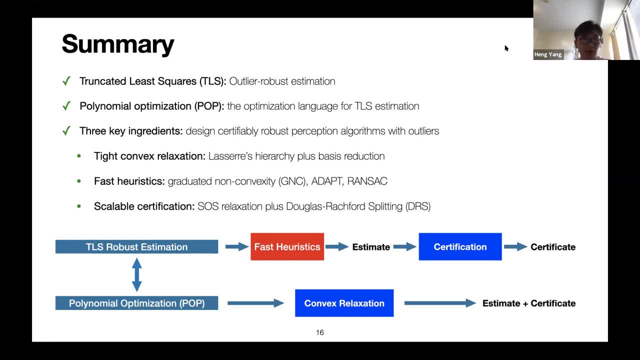 is also very important for certifiable perception. And then the last thing is a scalable certification that actually can outperform existing SDB solvers by leveraging the structure of the problem. And then this line here, this picture here, this line here. 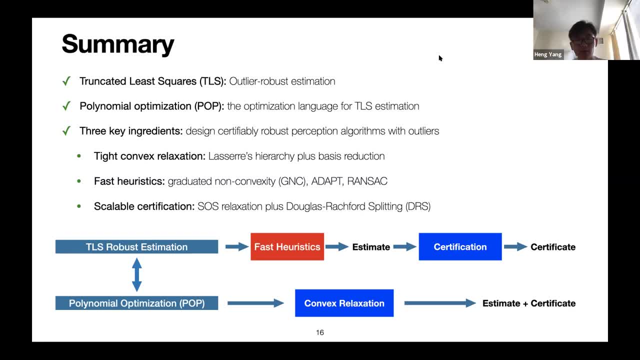 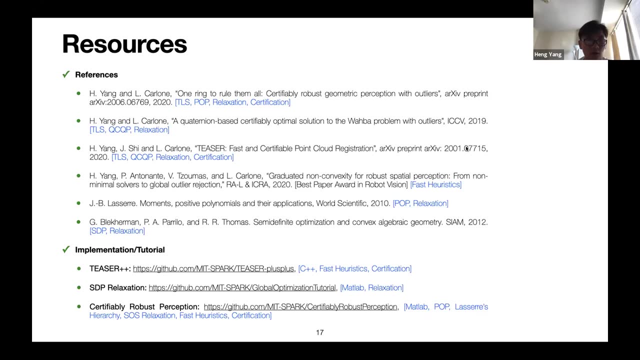 here exactly tells you the two lines of research. One line is directly doing relaxation and the second line is we perform fast heuristics and then we do certification. So in the end I'll show you some references and implementation and tutorial that's probably useful for people. 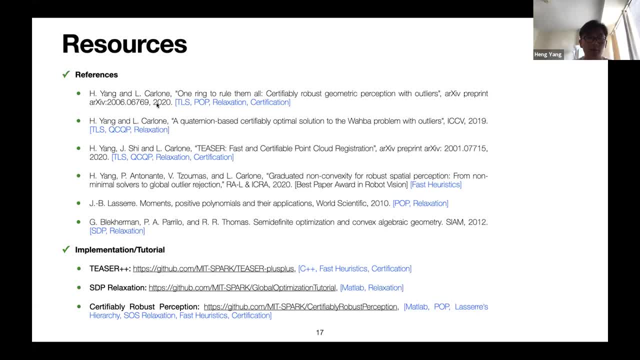 who are interested in the technical details. So the first reference is the result that just came out, which is like one month ago. This probably will be the go-to reference to read if you want to know more about this Lassier hierarchy and its application to. 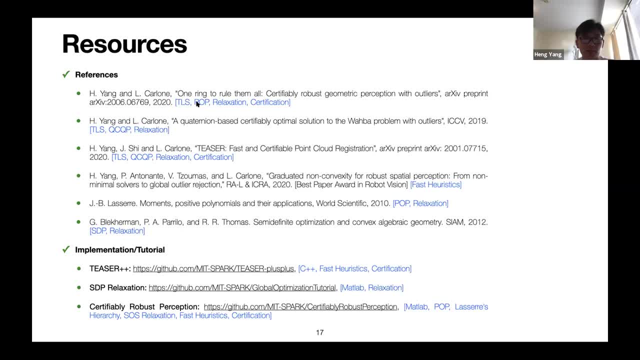 geometric perception And a few other results that in the blue lines. I comment about the keywords of these references And the last two books, one by Lassier and one by Pablo, and Blackerman and Thomas. I think these are two great books. that has been the source of 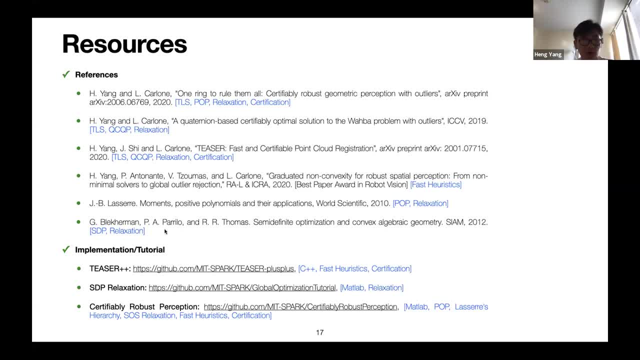 inspiration for me to do certified perception. I'll probably recommend these two books If you want to know. you know the one-on-one of these: SDP and pure polynomial optimization, relaxation And lastly, for some implementation, we have TESA++, We have SDP relaxation tutorial. 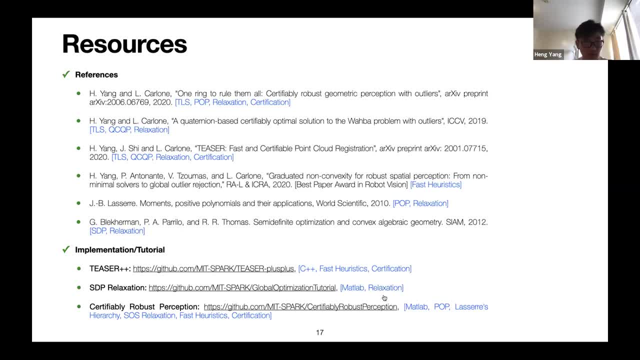 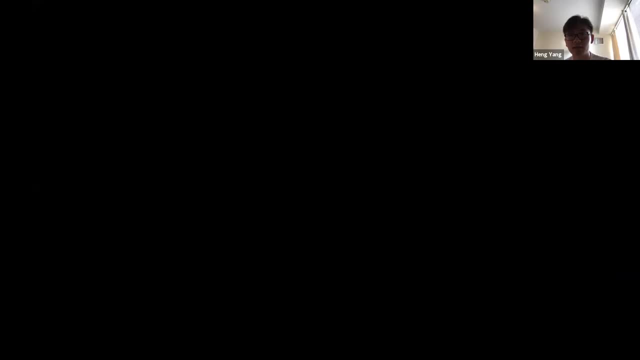 from last year's ICCV workshop. And then we have the. I'll release the certified robust perception code very soon on this. on this link It's currently empty, but it will be populated later. I think that's it for now, I think. 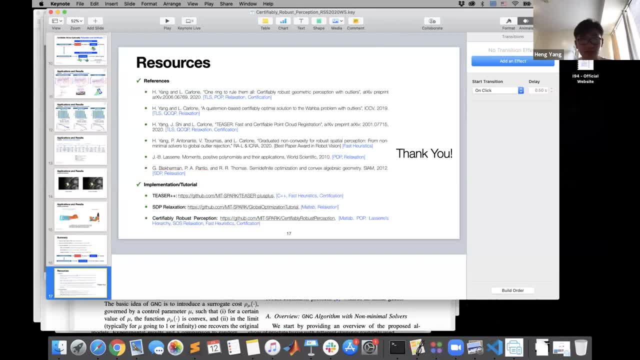 Yeah, I think I can take any questions, Thanks. Thanks, It was. yeah, it was very interesting actually And these tools are very powerful. I do have questions for you, but maybe let's start with the Maolin's questions on the on the chat. I think he's asking about the role. you know what happens if you have. 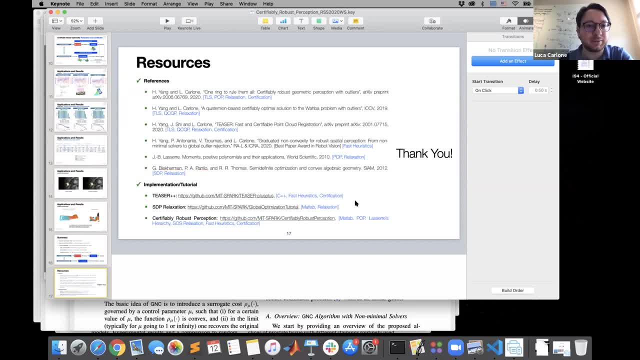 full certification. what does that mean And does it happen in practice? Full certification, Yeah. Does full certification mean that you know if you have? you know if you have full certification. does that mean that when you have an incorrect solution, you can certify it? I think, I think. 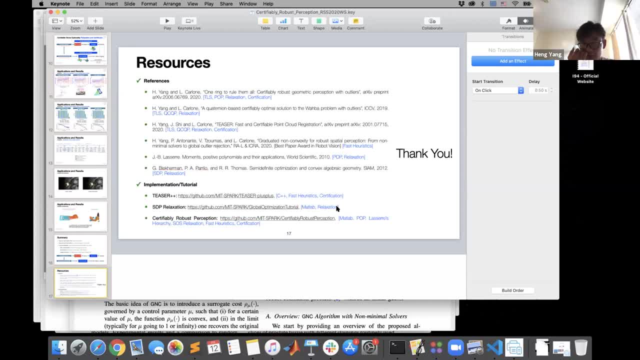 in that case, yeah, full certification. I can say that, if you're, if you're, if you're, if your input to your, to the, to the algorithm is well conditioned or good, which means basically means that when you have enough inliers, that can define, that can define a very good global 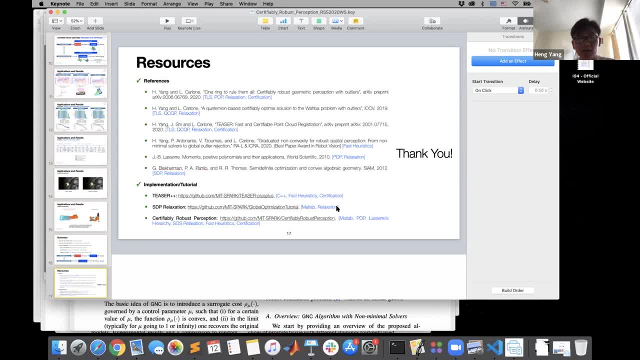 optimal solution, then it will never happen in practice, But it does happen. very rare, Right, Right. So there's multiple sorts ofнем advertisers I think of that you know, like, for example, when your feature correspondences are simply garbage. you know when you have. 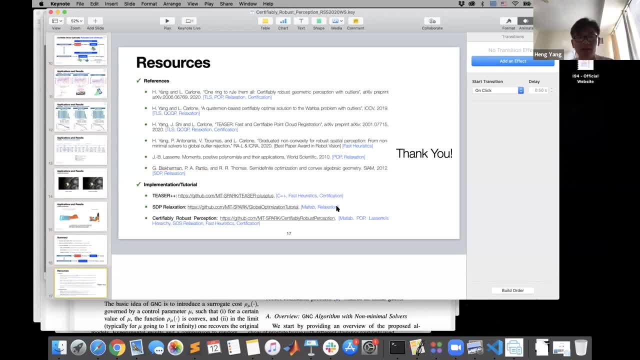 a feature correspondences, that's all our lives. that doesn't have any, doesn't have any in lures, Then you know in that case the global optimal solution is not the ground to the solution that you want. So in in the teaser paper we have a, we have this concept of what's called an estimation. 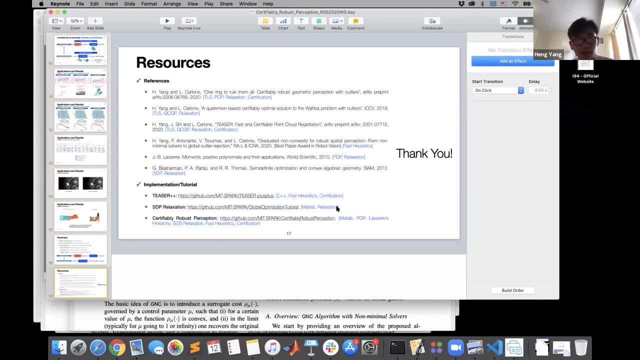 contract which tells you theoretically. Theoretically tells you when, when, the global optimal solution is the solution that you want. So false certification, you know. in short, false certification rarely exists, but you know. false certification means that you know, if you can certify the solution, then it already means that the solution is globally optimal. 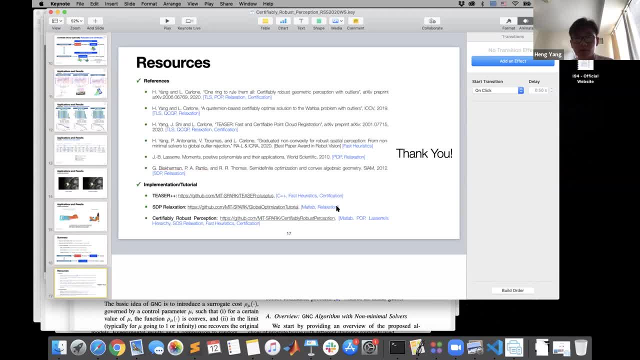 Then it remains. the question remains is: is the globally optimal solution the solution that you want? So false certification basically means that the global optimal solution is not the solution that you want. Yeah, I'm not sure if this answers the question. 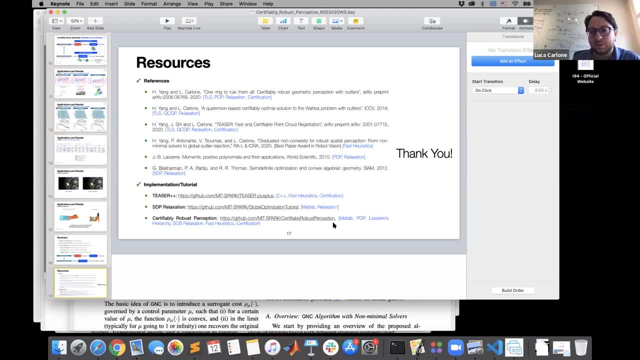 I think that's a very important perspective. It would follow up, like you know, if Marin has more questions. I invite him to follow up. Maybe one thing that can be useful also for the audience is to. so you were hinting to the fact that with this laser hierarchy, with this fancy relaxation, you get all the time zero duality gap, you get essentially strong duality. 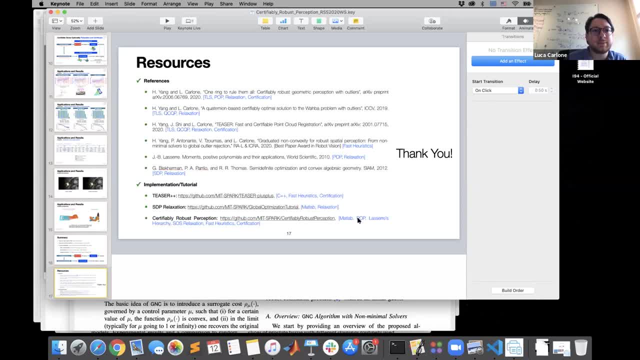 Can you comment on when this strong duality fails, Like you know, in these problems without pliers, we know, you know, TJ told us that, et cetera- At some point, like you know, some intractability will kick in, so we'll not be able to solve all the problems in polynomial time. 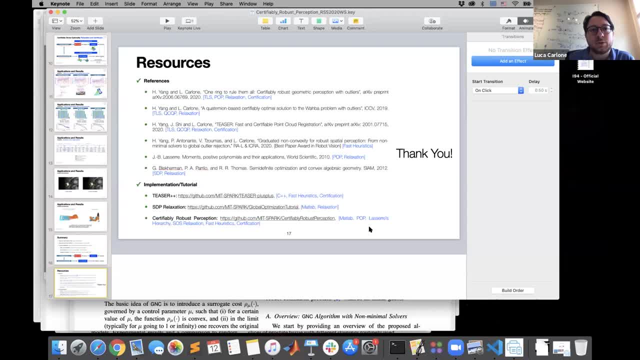 Do you have an insight on what is the root cause of, like you know, when the duality- essentially strong duality- fails? Yeah, yeah, That's a very good point, I think. I think, from my experience, I think strong duality, so I think I have this intuition that strong duality holds when you have a very strong, globally optimal solution. 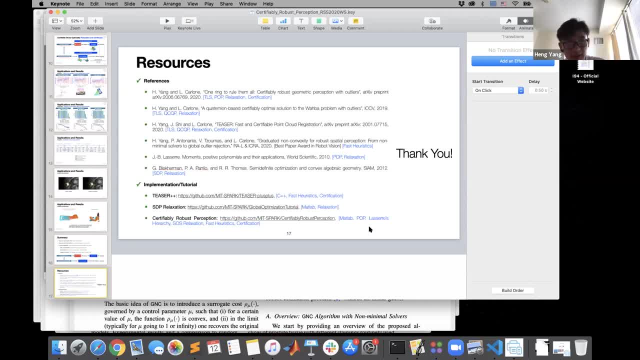 So you know, when I say it, I say a strong, global, global, optimal solution, by by meaning that this optimal solution is not ambiguous. So we do, we do see that in this, in this. you know, for example, when you do, when you do mesh registration, right, usually you have, you just have these point to line and point to plane correspondences. 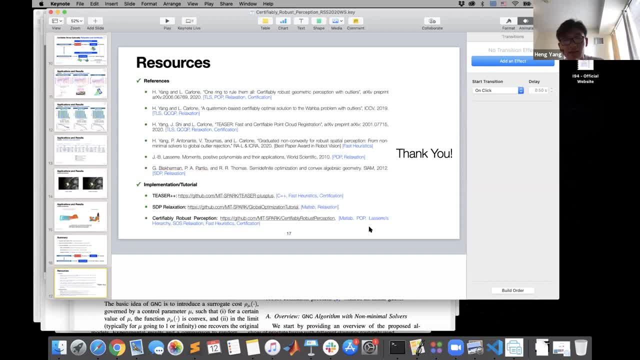 So in that case the relaxation is actually not tight. But if you add a little bit more information to into the solution you will get a. you have a very, very good kind of. you know, in this case the relaxation is not very tight. So in that case the relaxation is actually not tight. But if you add a little bit more information to in into these solutions, then you, you will, that you will be able to. you know that's a very, very good point, right. 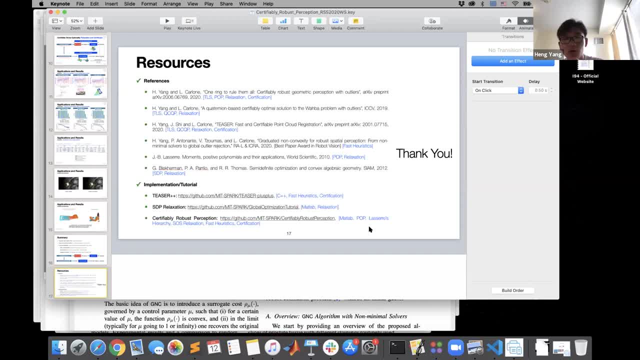 So I think the solution is always, it's true into these correspondences, For example, you know, if you can add, you know, the surface normals, estimated normals as an additional registration cues to these problems, then the relaxation will become super tight. 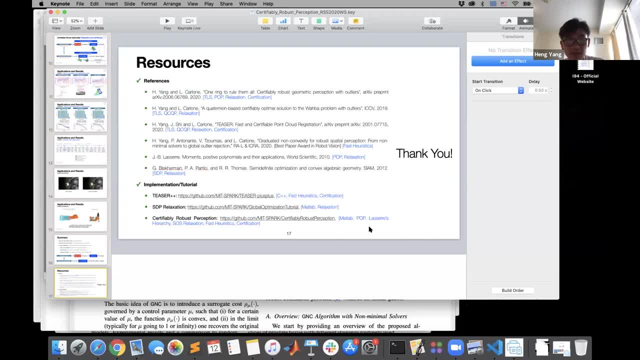 So, you know, this tiny example, you know, gives us the insight that you know, in order to have strong drafty hold, you want a very unique and a very strong global optimal solution. And then, on the other hand, if you don't have this strong global optimal solution, 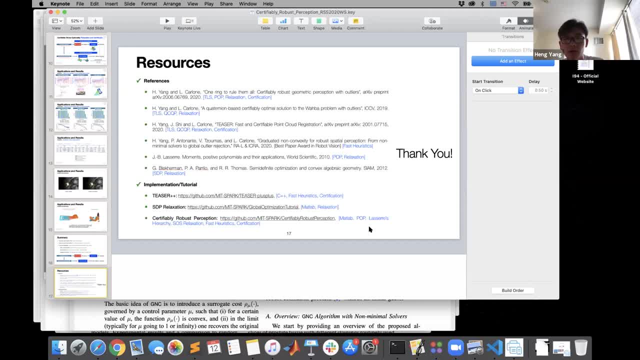 then, after solving the relaxation, you'll get a solution that's not rank, one which basically tells you the solution is ambiguous. You know the global optimal solution is embedded in the solution of the SCP, but it's just not so clear because your data is not perfect. 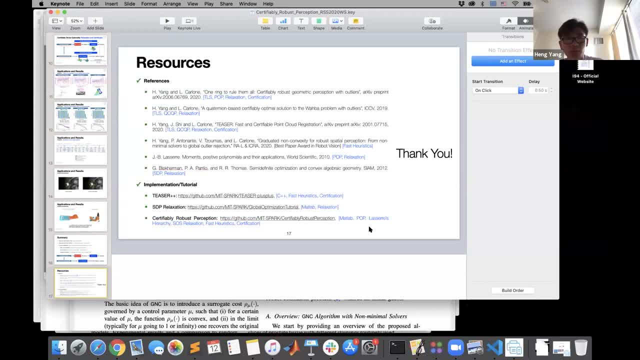 So you know. so the perfect data means you know more visual cues, such as surface normals, or it can be more inliers and less outliers. So these are really just, I think, the intrinsic, intrinsics of this problem. So to make a, to design a tight relaxation, 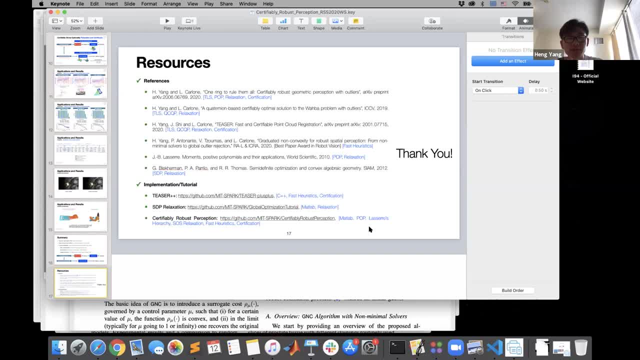 you need enough inliers and you also need a very distinguished, a very distinguishive, very distinguished registration cues, like visual cues, like point to point correspondence instead of point to plane or point to line or point to image. So these, these, for example, point to two. 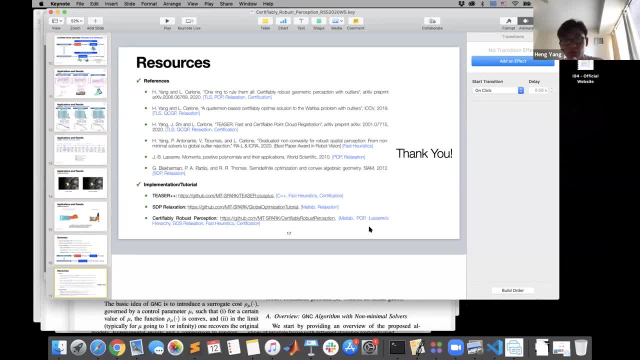 two D to three D sort of certifiable perception is more challenging than three D to three D. The reason is because from two D to three D, the projection actually gives you more ambiguity to this problem. So that's why I think you know these. 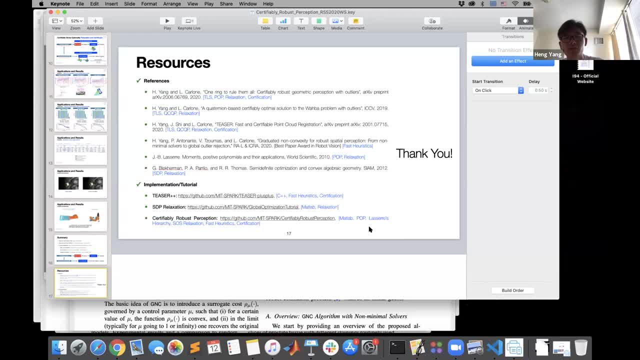 these relaxations can be made tight if you have enough information of the inliers or of the problem of the ground truth. I think that's my, that's my intuition about it. Thanks, Thanks. I will stop you here because we have like a few more questions. 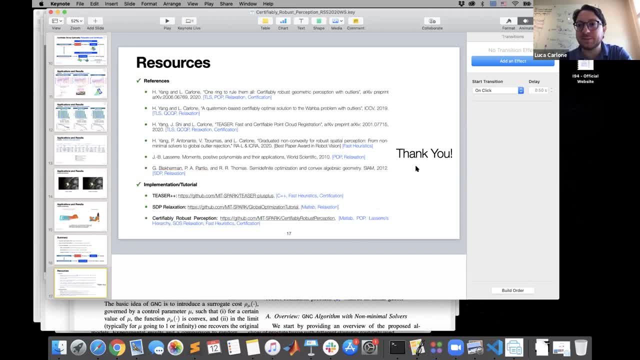 and I will ask you too if you have any questions. We have like around four or five questions. I will ask you to have, like you know, a short reply to each one, if we can. So Sriya, she's asking if you can tell a little bit more. 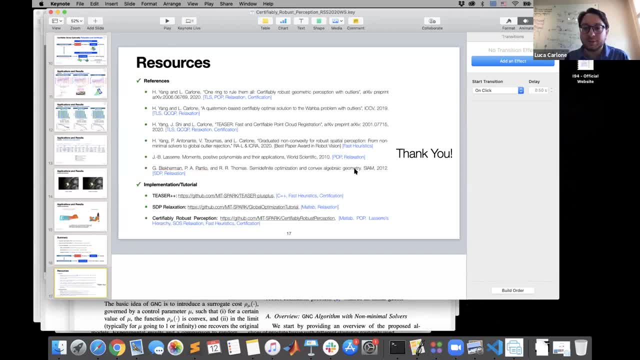 about the interaction between noise and outliers and in particular from the TLS. you have two hyper parameters, One, I think, is the beta, which is the noise, and the epsilon, And the question, I think, how these hyper parameters are affecting the problem. 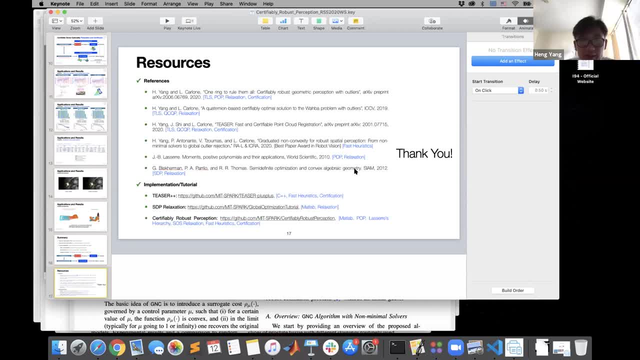 Yeah, I see, I see the chats Right And, in particular, sensitivity to noise, I guess, is the question. Okay, So, by the way, do we want to see which the beta? what is the beta? So the beta beta here? yeah, 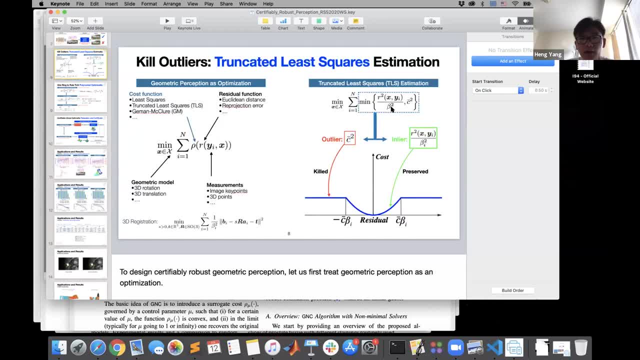 beta here is basically the noise. You can take beta here as the, for example, the standard deviation of the noise. And then the C bar square is, you know, is basically saying how, how, how large of a resistance is. So you know. 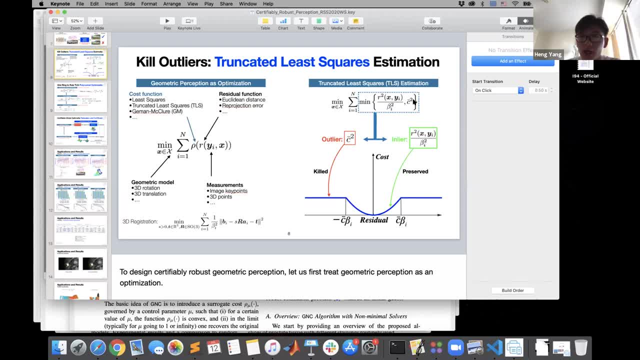 if you're taking the noise ratio above this standard deviation, will you consider it as an inlier? For example, three Sigma, right? So you know, in, in in one dimensional. usually, if the noise is Gaussian distribution, then away from three Sigma. 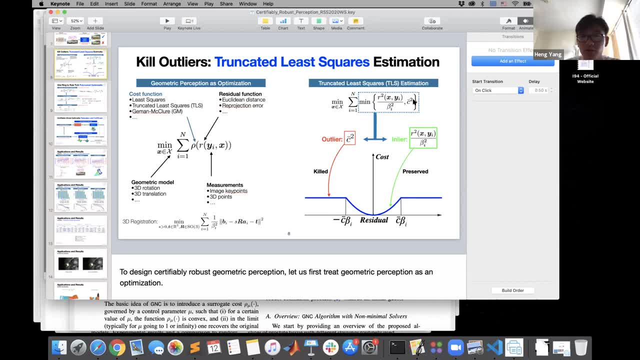 you will think that this is an outlier. So in that case you can set beta to be the standard deviation. then you can set C bar square to be three, for example, then all nine. that in that case it will. So this is basically the interaction of noise and outliers. 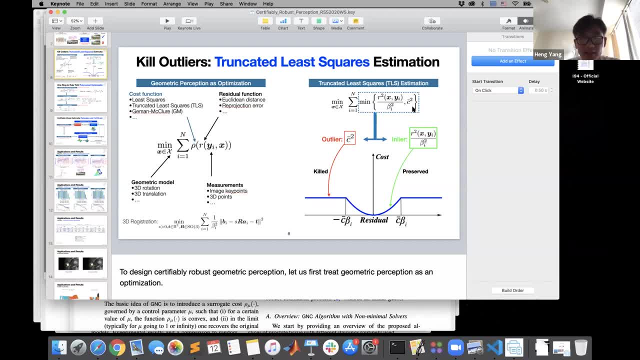 So you, these are these uh hyper parameters really are not not really that sensitive in in terms of uh real app. in terms of uh empirical performance, We found that it performs quite well. uh, you know. 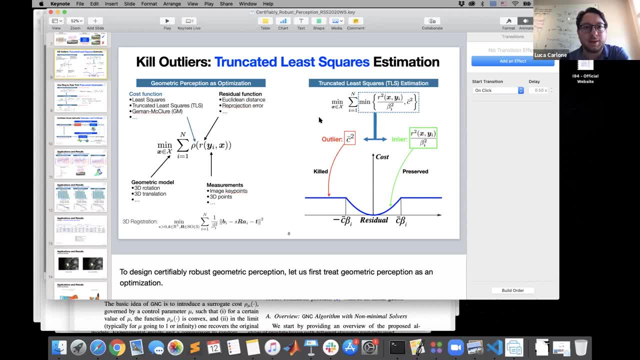 within some large range. I do have a related question from Kasra. We're seeing uh focusing on outlier rates can be misleading uh from intuition and bigger results. You know the distribution of outliers uh influences the hardness. 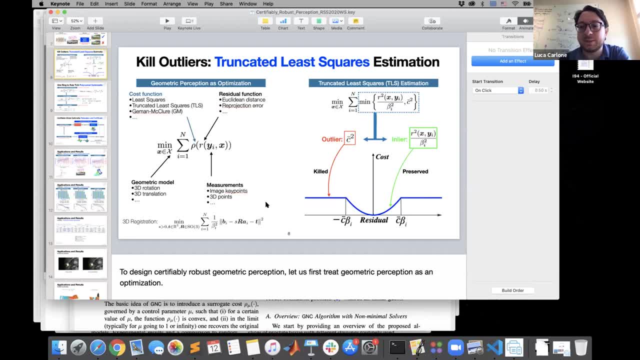 How are you generating your outliers And how sensitive is the performance of these algorithms on the distribution of outliers? That's a great question. Yeah, it's a good, great question. Right now we're just doing random outliers. Yeah, I agree that. uh, you know. 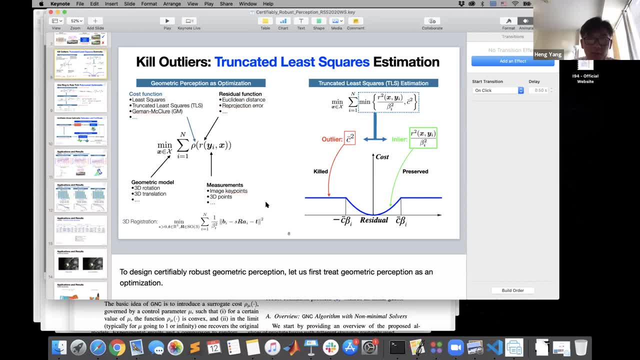 when you have uh adversarial outliers, it's gonna, it's gonna make this problem uh harder, but uh, we haven't explored it yet. Uh, we, we explored it in the Wabaugh case. We explored it in the Wabaugh case, for example. 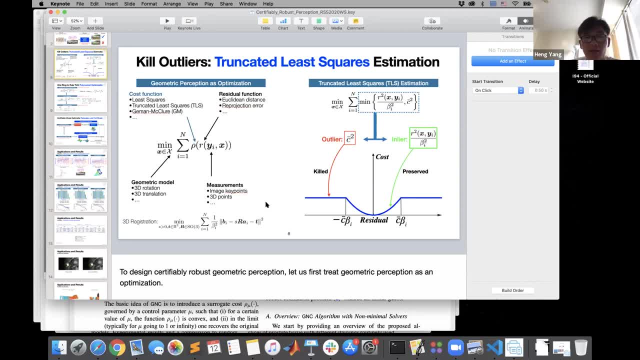 when, the, when you have an uh, a bunch of outliers forming another consensus set. Basically, you'll have two distinguish uh, distinguish uh rotations. that you know. that kind of uh corresponds to uh, a different part of the data. 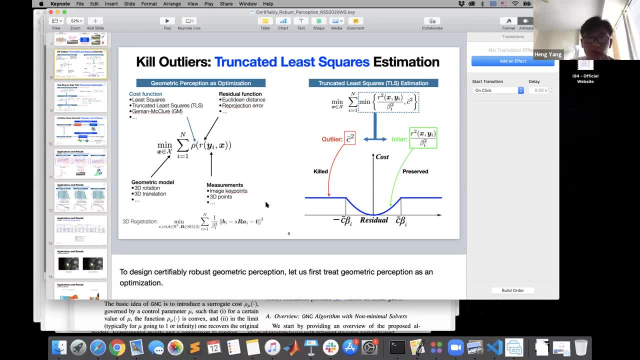 Then you know the the relaxation will still be tight. It'll give you two solutions. One, you know, one solution is corresponding to each of the rotations. So I think it's it's very, it's, it's untapped uh regime, that uh, you know. 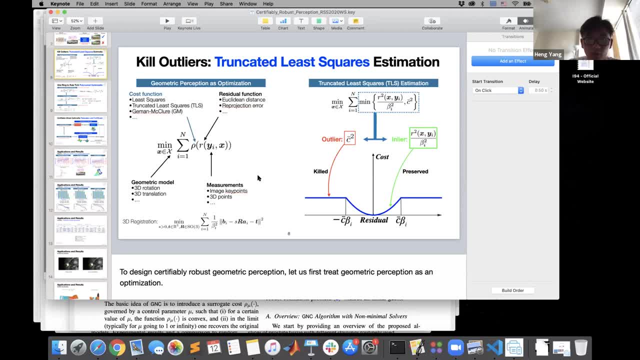 to be honest, we haven't explored too much, but I think the relaxation will will still will give you some, uh, some idea also in in that case, in in the case of adversarial outliers, And also, I would say that, in the teaser++ paper. 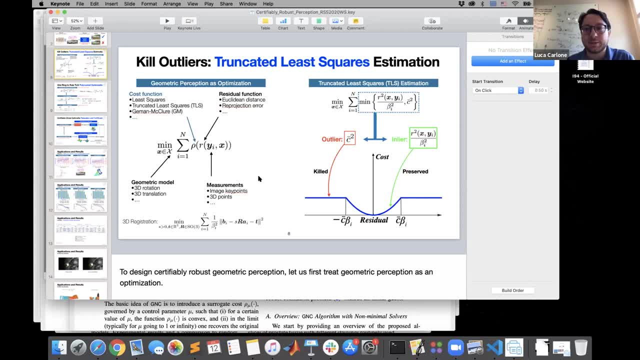 there is some result about. you know which kind of adversarial outliers we can consider. Oh, yes, Yeah, In the estimation contracts. That's right, That's right. So um Kazra is also asking a bunch of good questions actually. 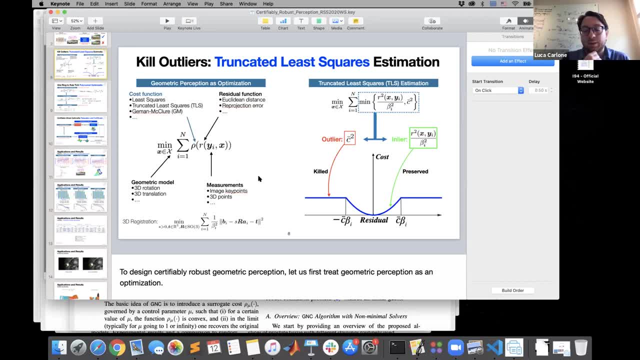 So, um, we discussed a bunch of things right. So, in most of them, um, the observation of strong duality is just a posterior and empirical, for which ones we have, uh, essentially guarantees on, uh, on strong duality a priori. 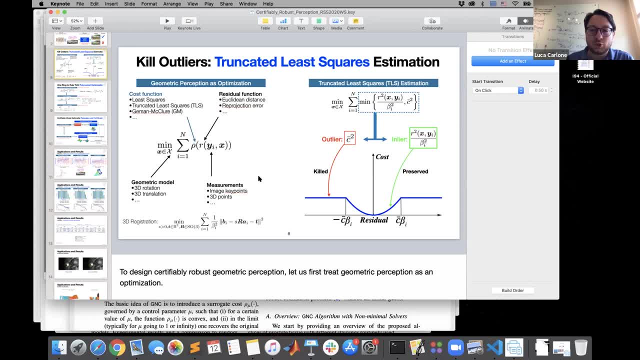 Um, and in SCCing something that we mentioned- rotation averaging, something that we mentioned- Do you want to say a little bit more about the guarantees from LACERA hierarchy? Yeah, So, uh, so yeah, a posteriori, uh, a priori, guarantees we do have for some of them. 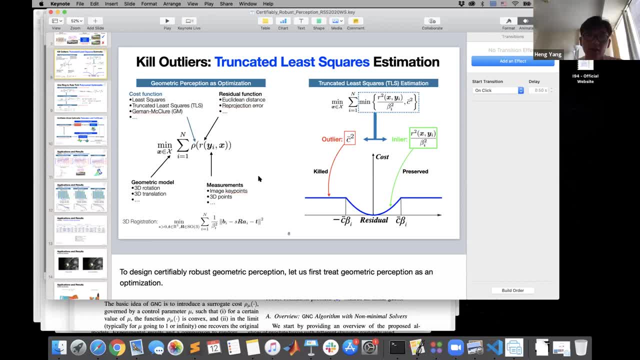 Uh, you know, for example, for the last year's ICCV paper, the, the paper that uh uh TJ talked about. In that one we have theoretical guarantees on the case where you don't have. you have zero outliers and zero noise. 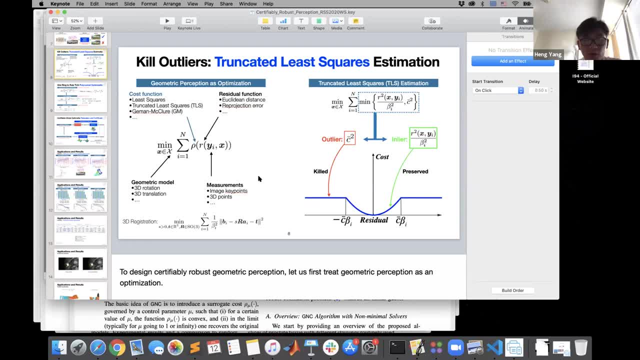 And you know, we all it, it will, it can be extended to the case of small, uh, small noise. But in these, uh, in all the examples that I talked about today, uh, right now, the, the, the, the, the guarantees are purely empirical. 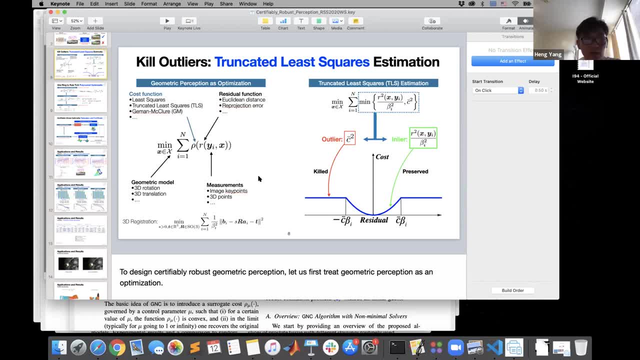 Uh, but I do believe that uh, some of these problems, uh, you know you will be able to prove that uh strong duality will hold. uh, when the noise is, uh, is kind of, uh, is is small within some range. 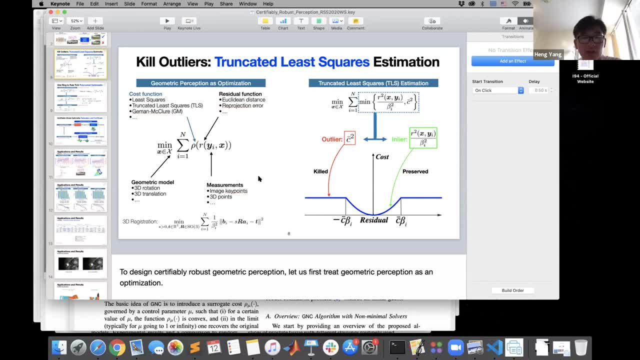 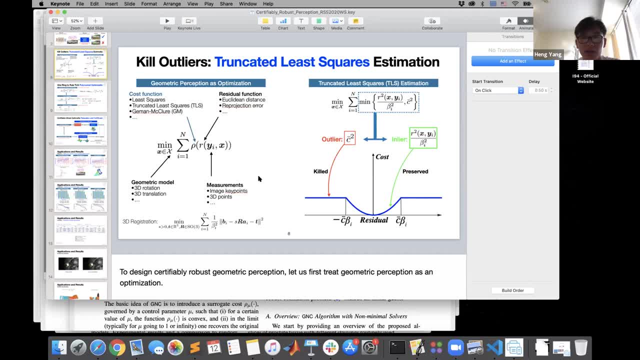 how, if you can implement the hierarchy high enough, Sometimes the hierarchy when the hierarchy is high, too high, you just, uh, you cannot solve the STP, So you will not know, uh, if the relaxation is tight. but they have theoretical guarantees. 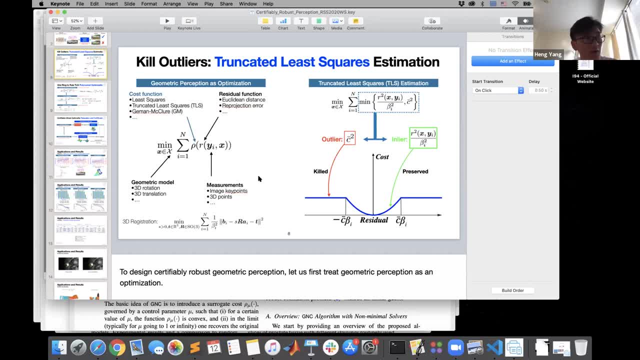 on when the relaxation will be tight. that, uh, when the hierarchy is high enough, it will always be tight. So so the way I see it is that the hierarchy essentially allowing you to trade off optimality and performance right, You can decide to have the high level of the hierarchy. you pay the price computationally. 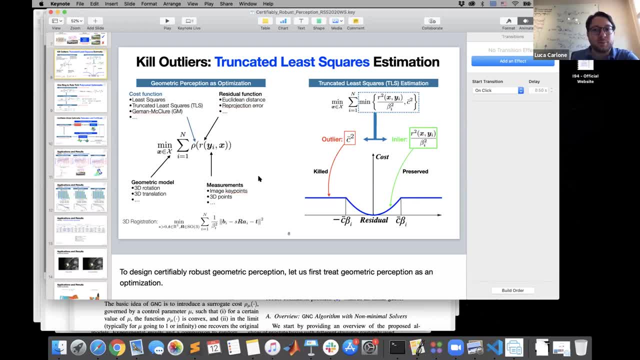 but you get an optimal solution. or you can, like you know, maybe perform a lower order of the relaxation, You can have faster solution, but maybe you lose a little bit of tightness, right, Yes, Yes, A little bit of the tightness, but you know, uh, maybe the tightness doesn't really matter. 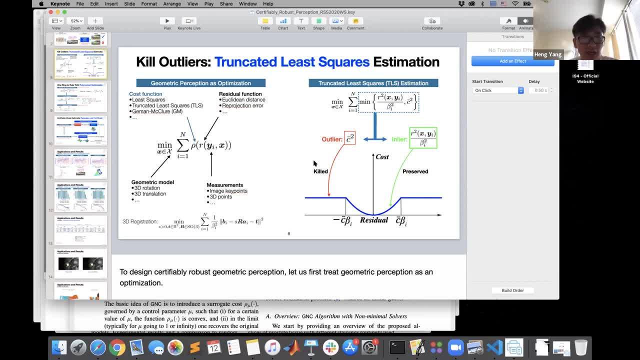 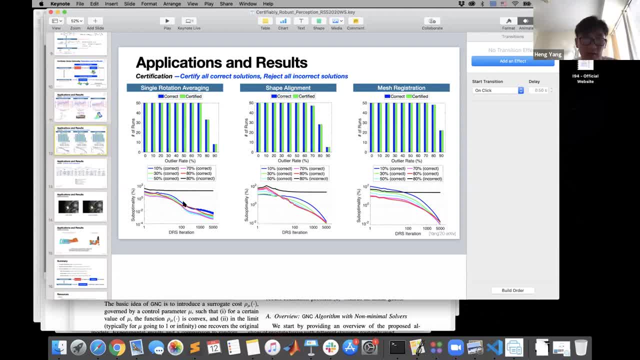 This is going to be: uh uh, uh, uh, uh, uh. um, uh uh uh uh. Certainly uh very distinguishive in in terms of incorrect solutions and and uh correct solutions. 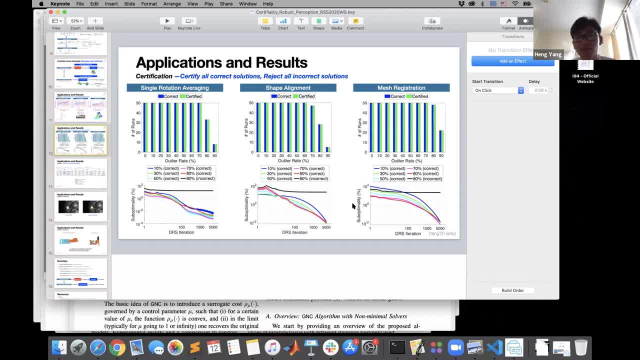 Um, when you do certification, this type of uh, even though you don't have very uh perfect, uh strong duality, it might not necessarily matter. Okay, I think this is related to the next question. I think that there are good questions. 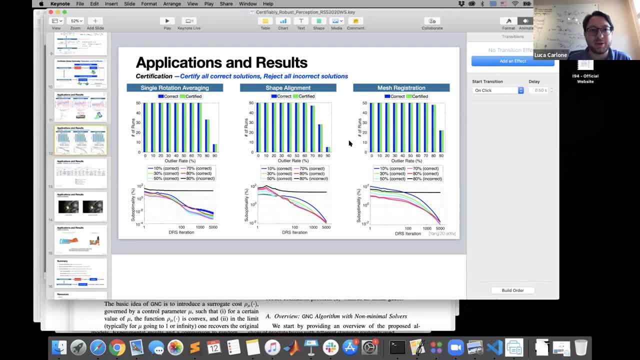 So we'll keep going. there are like probably three more questions, So we'll keep going. I know we are out of time, but uh, you know, um, I think these are really interesting. So, related to what you have said, could we? 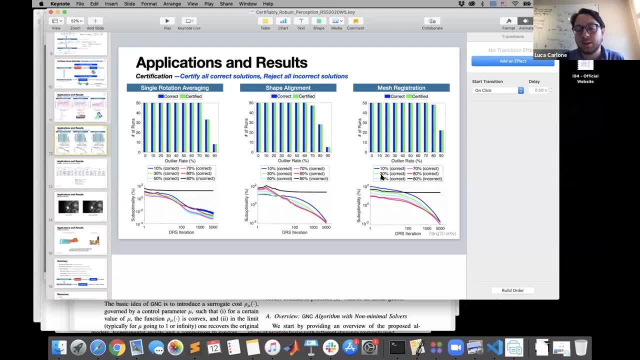 Sorry, you see, because there's also asking: with the certification approach that you have, can you provide the suboptimality gap? also, you do not have strong quality. yes, the certification I think the first question has asked is regarding does the certification rely on empirical tightness? I think that's definitely yes. 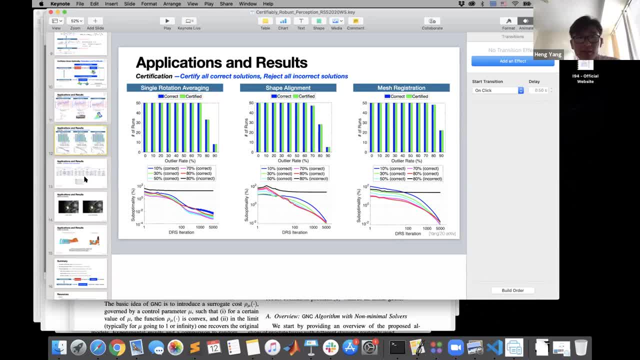 so, if you know, in the certification we are actually certifying the relaxation, we're not certifying the original problem directly. so which means that if you don't have a tight relaxation, then the certification will also not going to work. so because there are primal and dual, so there are, you know, two sides of 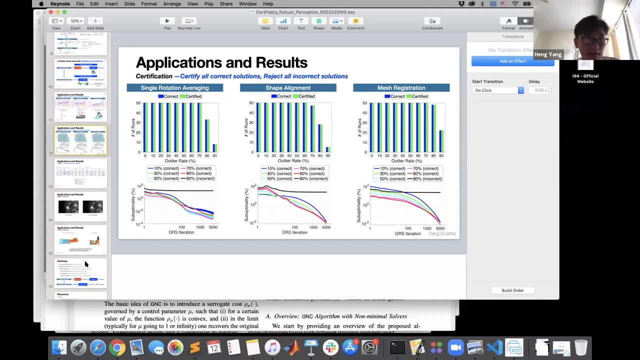 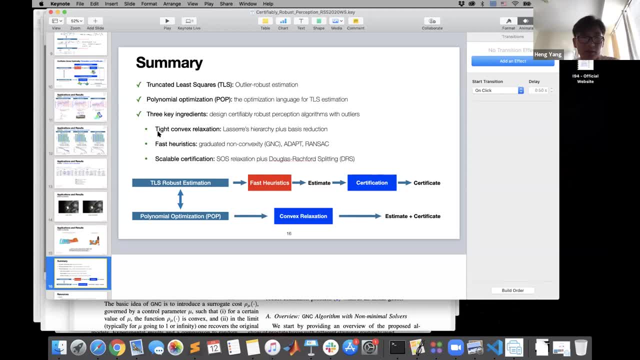 the coin. they are highly rated. so that's why, in the summary, I say that you know the three, three, Q and E, three ingredients are actually. they're all necessary. you know the first of all, you need to have a higher relaxation and then, from the relaxation you can, you can give up more scalable solvers and the 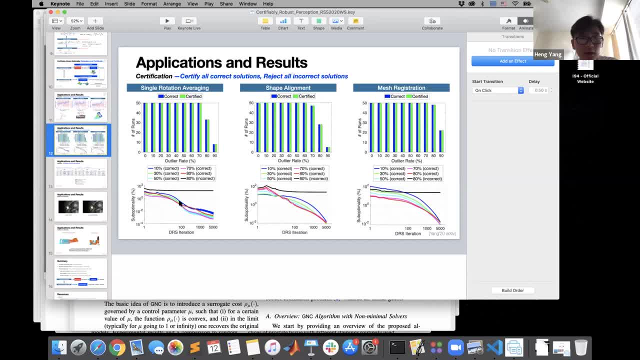 second question is: yes, the yes, even for more scalable. actually, over which one of these benefits about b, b, b does not match drug ability gap and the, and then, of course, the certification. once you check all so different kind of dudes, over which one of these benefits I said? even if you don't have strong via or tide relaxation, the certification will still give you a suboptimality gap. a valid suboptimum cap is always- it's always react. the suboptimity gap is always abound on the only sub b? bb, even though you. 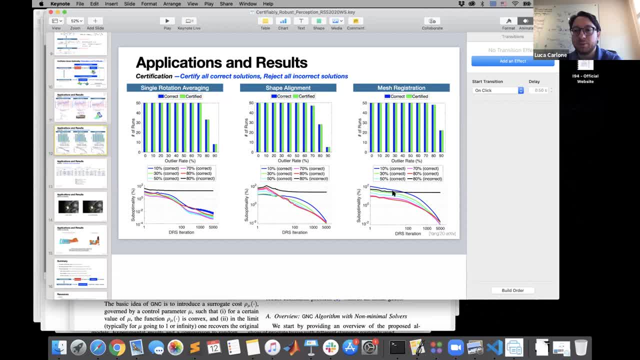 don't have strong to add or a tight relaxation. But did you mention, solving the global optimal is prohibitive in terms of time and resources. Yes, Yeah, this is a very good question. I think yes, the answer is the duality gap is between the estimate and the global optimal. 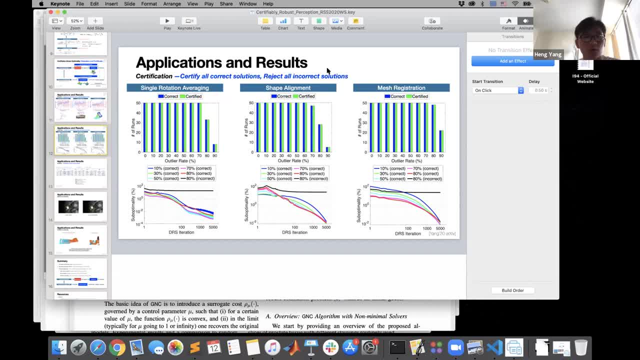 But you are correct that the global optimum is unknown. We don't know the global optimum because the theory prohibits us from knowing computing the true global optimal. But the beautiful theory of Lagrangian duality is that in the certification you actually don't need to know the ground truth. 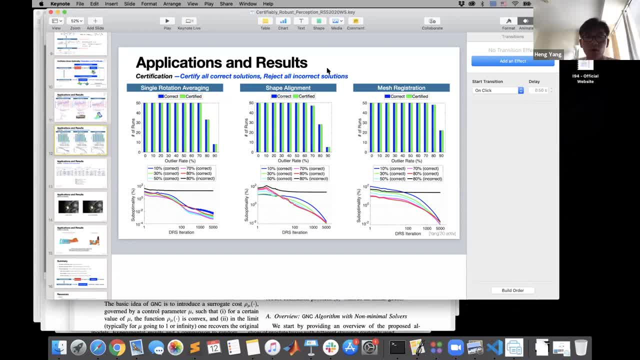 It's like a sandwich: You know the upper bound and you know the lower bound, And then, if the upper bound and lower bound are close enough, then you know that the global optimal solution is sandwiched between these two bounds. So that's why you still get a valid optimality bound. 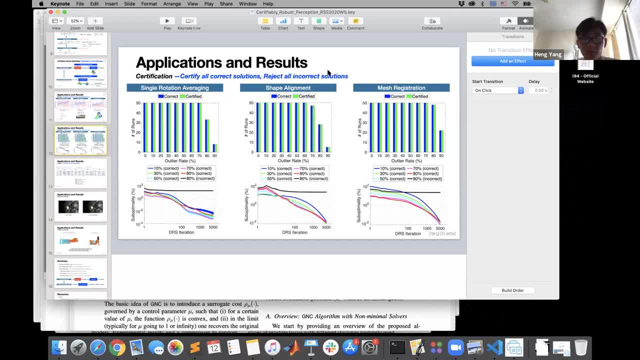 even though you have no idea of the global optimal solution. I think that's the beauty of duality. Okay, great, I think we'll go for the last question Matt is asking. first of all, he's commenting that that's an awesome, very general approach. 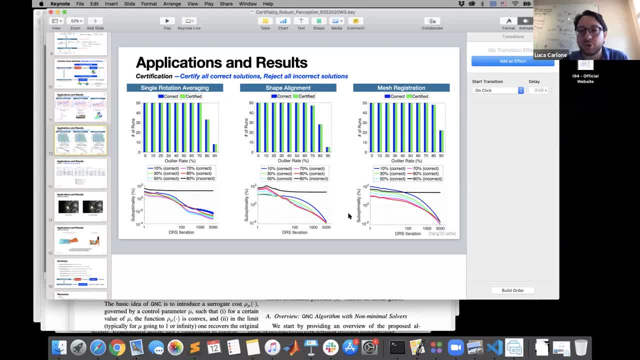 He's asking if you tested these on problems like SLAM or rotation averaging, where the decision variable size grows with the number of measurements And in that case if you can use sparsity or maybe assuming that just a subset of the measurements are outliers. 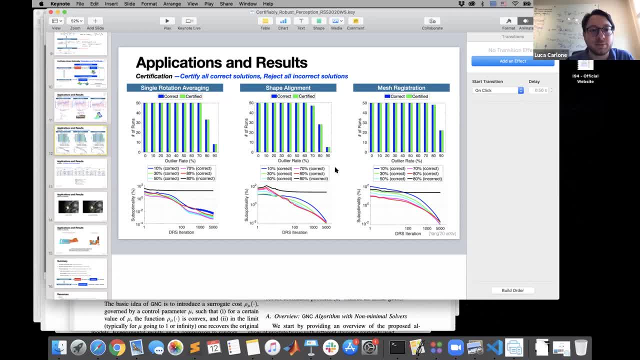 can you make the certification tractable? I think that's another great question. Yes, So I think yes, if you look at the paper, we do use the sparse version of sum of squares relaxation. This is more technical, but I think Matt will be able to understand that. 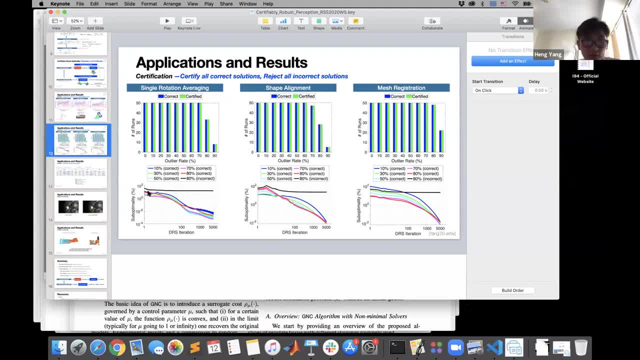 So in order to do the certification. so the certification is the first order method. So you know, first of all the method, although it's a convex problem, but its convergence will depend on the initial guess. So actually, the initial guess is actually obtained from solving a sparse SOS program. 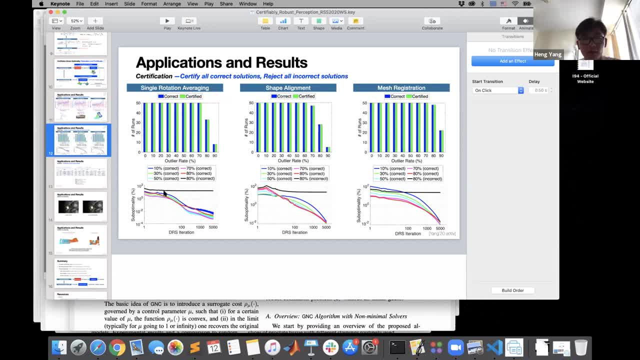 So that initial guess actually bootstrapped the convergence of certification. So I can safely say that without that scalable sum of squares- sparse sum of squares- we will not be able to achieve this amazing scalability of certification. So I do see that sparsity can help a lot in these problems. 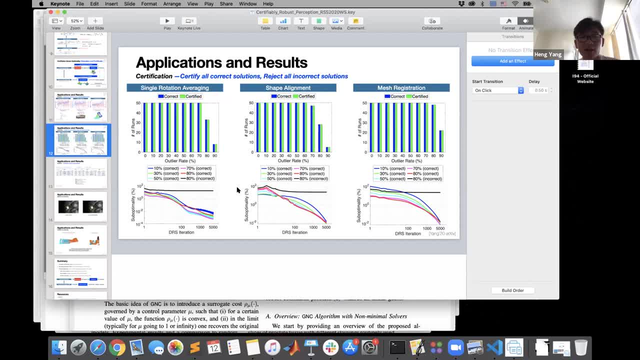 But at the same, on the other hand, sparsity is not enough. So if you just purely rely on sparsity, for example if you directly do a sparse La Silla hierarchy, it's not going to be tight. So that's the takeaway of this. 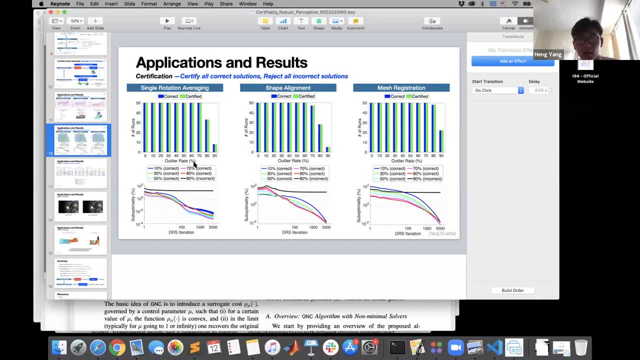 But you know from the again, duality helps. Duality helps Although you have a non-tight relaxation from the sparse SOS, but you can actually utilize that as initial guess for more powerful relaxation, which is dense but can be solved using first order methods. 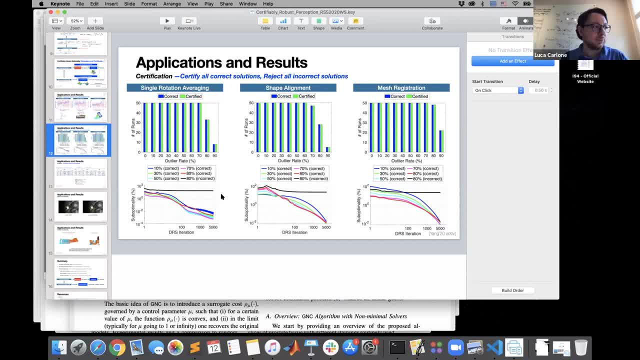 I don't know if that's, Do you think we'll get a scalable? you know we'll get scalable to a level in which you can solve SLAM and rotation averaging. I don't know. I doubt it. It's still going to be the current state of the art of STB solvers. 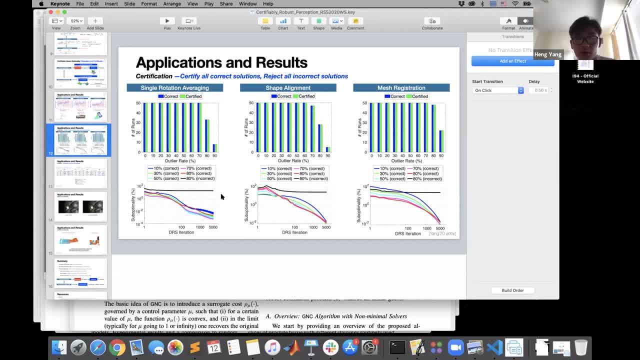 I think it's still going to be on the order of seconds, I think, not milliseconds, So probably will not be real time, but I think it's reasonable. All right, Thank you. so so much. I think we are going to wrap up. 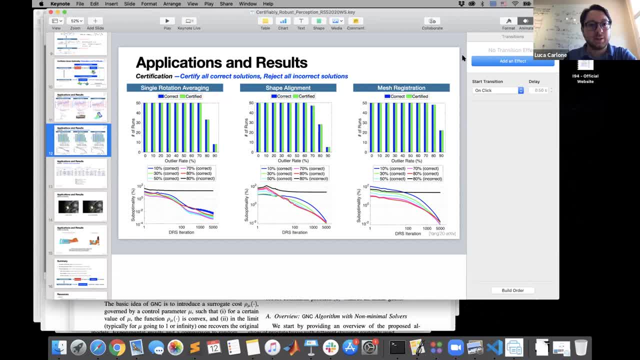 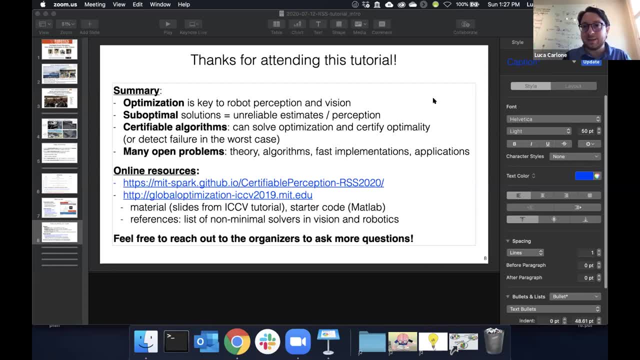 I wanted to show just a final slide to just wrap up. You should see my screen at this point. The final slide, like you know, first of all to thank you all, Thank the attendees, for the patience and, like you know, 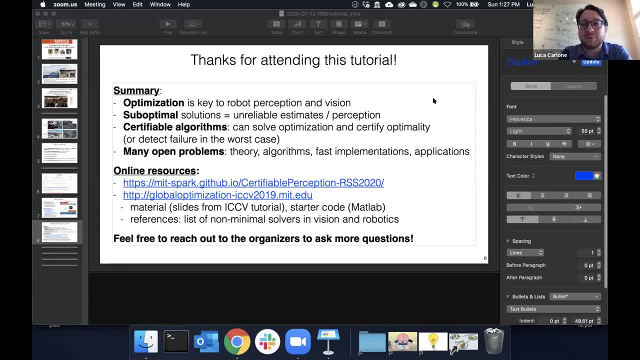 for staying a little bit longer attending this tutorial, Wanted to thank the organizer for giving, like you know, very insightful talks and sharing their experience with global optimization. So, in summary, I think this tutorial is really about four points. really, Like you know, optimization is a key to robot perception and vision. 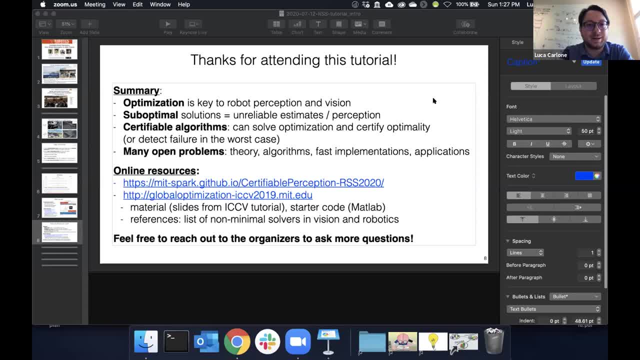 Suboptimal solutions in many cases is the same as unreliable estimates, which is a problem for safety-critical applications, And this is one of the first events that we organized around this idea of certifiable algorithms, which are about solving this optimization problem arising in robot perception and certifying optimality or detecting failure or 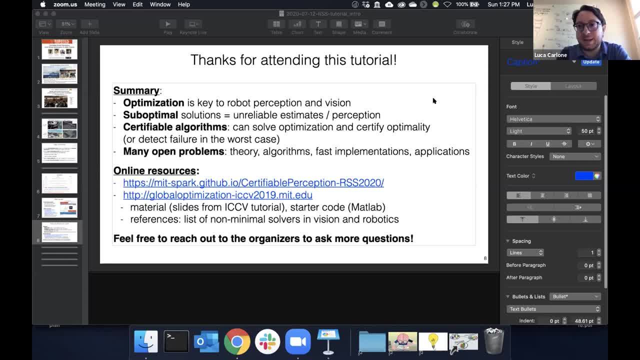 suboptimality in the worst case, And I hope that out of this tutorial you got the point that there are many open problems. There are open problems on the theory side, designing new algorithms. If you want to help us, like you know, also look on, you know. 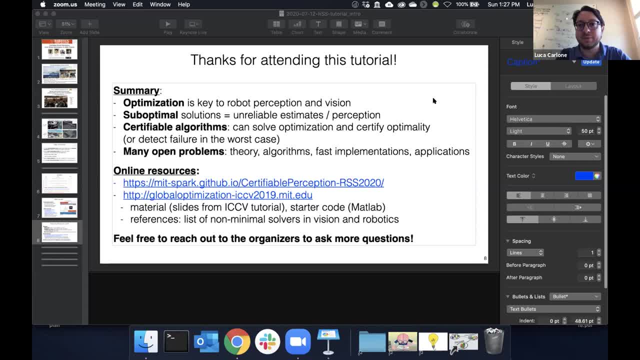 develop very fast implementations to make this run in milliseconds instead of seconds, and even just applying these to common problems, right? So we have a number of online resources. Hank was pointing to some of them. I would say that we kept the RSS tutorial website minimal because you know. 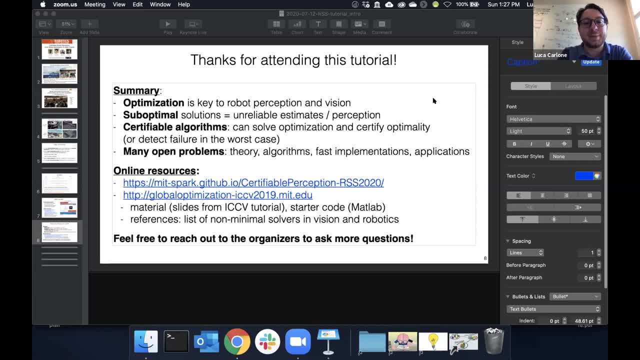 this was embedded on the RSS portal. We could not add much more. You can find even more resources in the ICCV 2019 website. You'll find the slides, You'll find starter code in MATLAB And we're going to keep a list of references of non-minimal solvers in 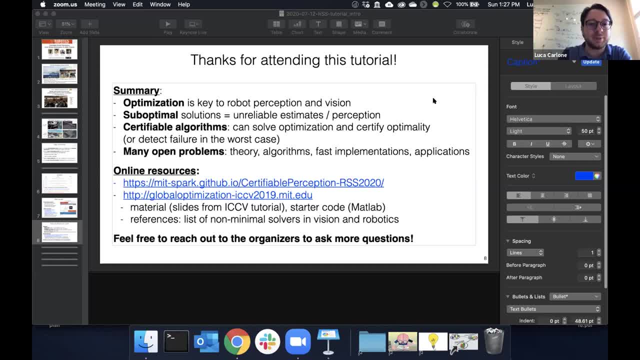 vision and robotics, And we'll keep that updated. So I want to close with a final message saying, like you know, if you're interested in these topics, please- you know- help us And just reach out if you have questions. 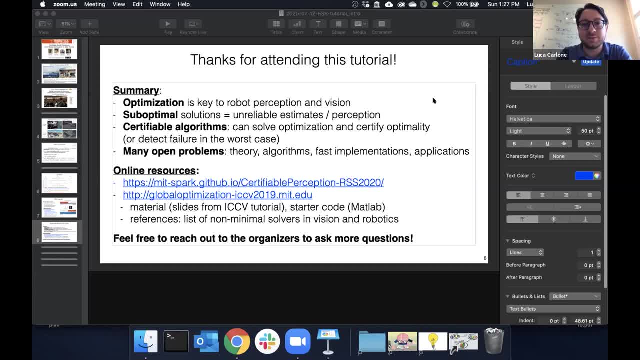 Feel free to reach out to any of the organizers and ask your questions. With this, thanks again to the attendees. Thanks TJ, Thanks Anders, Thanks Hank, And see you guys at the other events for RSS. Thank you, Thank you, Luca.